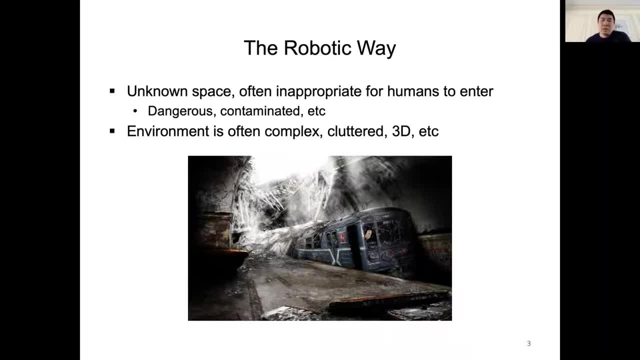 to collect sensor data for us to analyze the space. okay, so as of today, autonomous exploration is still harder than human operators doing it by carrying the sensors your backpack, or hold it by hand, or mount it to a vehicle to drive it manually through the space. that's still easier. 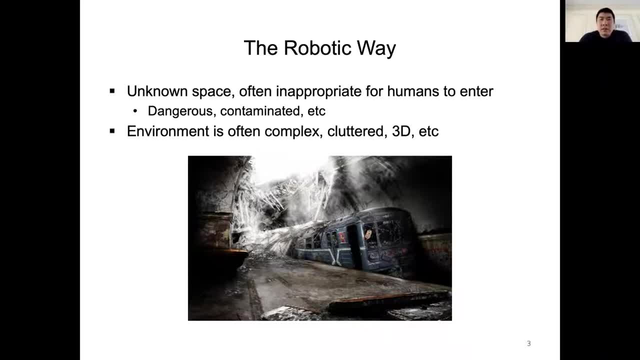 as of today. hopefully that will change. but today, the reason of sending autonomous robots to map and explore spaces, it's mostly because because of the danger, um, so the problem is a hard problem, especially if we are exploring environments that are very complex structurally, structurally cluttered, 3d. so we'll get back to this point of how the problem is difficult. but 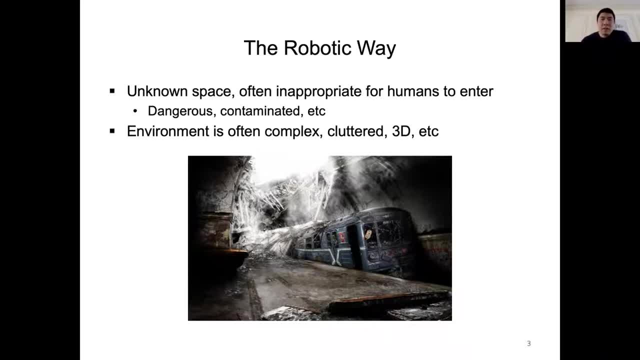 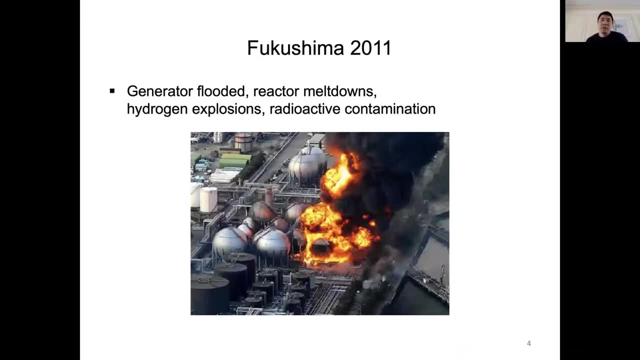 let's take a look at some of the other problems that we're looking at today. so let's take a look at the at a realistic of civil application as a use case of the technology. so this is the fukushima nuclear plant. in 2011, disaster happened: generators flooded in the basement. 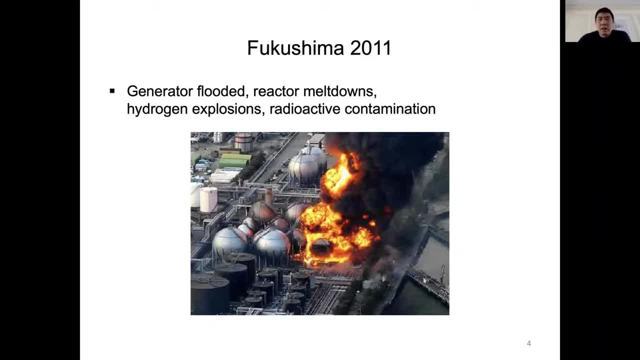 uh reactors melted down and radioactive contamination spread all over the place. so this is a widely used example of the darpa humanoid challenge used as an example a few years ago. um, the humanoid challenge motive was motivated that um, by the time that the disaster happened or right before the disaster happened, if there was a humanoid robot to be sent into the basement. 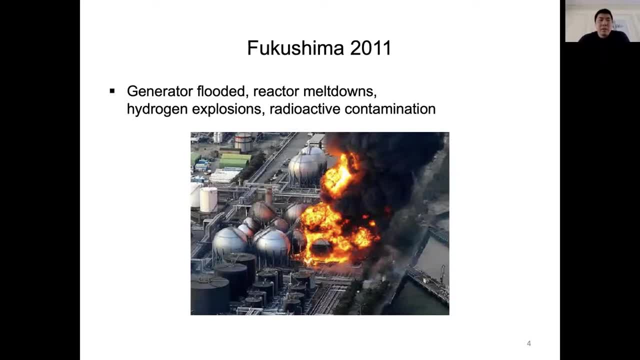 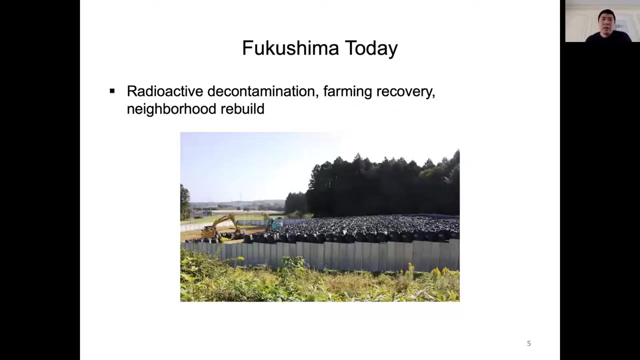 to close a few valves, the disaster could be stopped or largely mitigated. so we are talking about exploration today, we are giving a different story. we are looking at the impact of the disaster. um, now, what we can see is that the state of korea is having a great 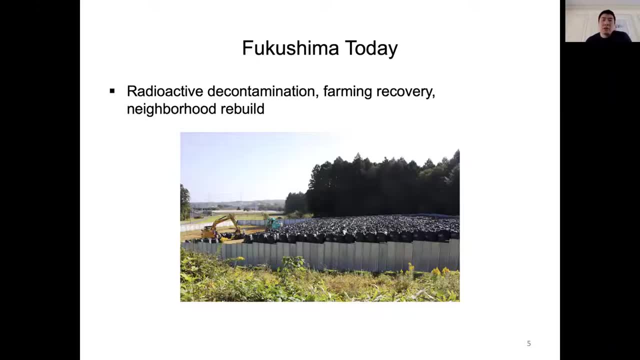 impact and it's not something that's going to really be lost, but it is beinguvved in and with a lot of theBut the the. the fact is that if today, if we look at this area, 10 years after, like today, over the period of 10 years, the government has spent tremendous. 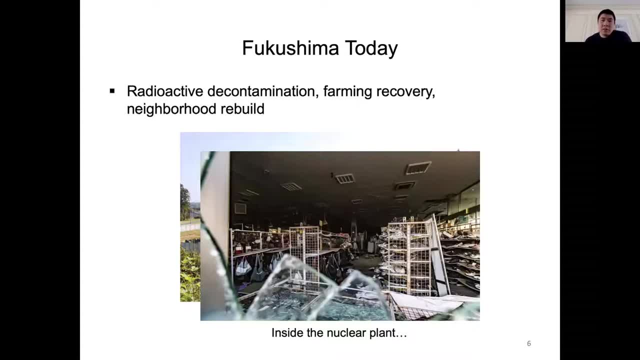 amount of effort to rescue this area, to review radioactive contamination, to resume farming and to areas are completely unknown to the outside world. Nobody knows the situation in there, Nobody knows how to enter the space. even So, this is the exact example as a use case. 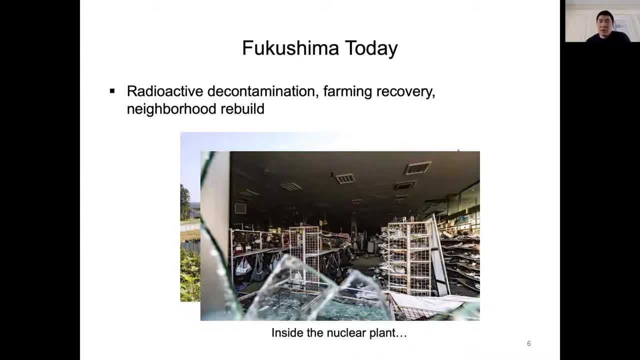 that autonomously exploring systems could be sent into the space to scout, to map and to collect additional sensor data. okay, So for whatever sensors that we can install on the robot, we can let them carry along by the robot to collect the data from them. 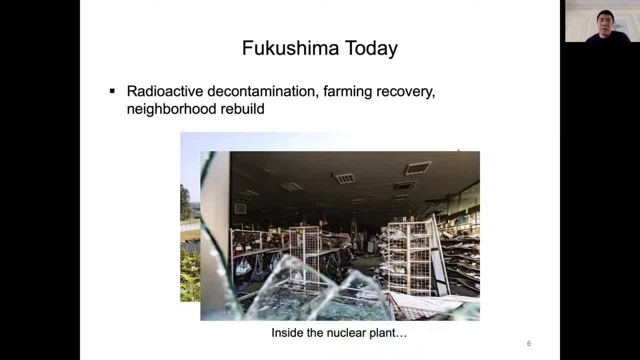 And later on we can embed the data onto the map to get additional information for people to analyze the space and hopefully that opens the door for somebody to enter the space to start cleaning up the space. okay, So this is a realistic use case. 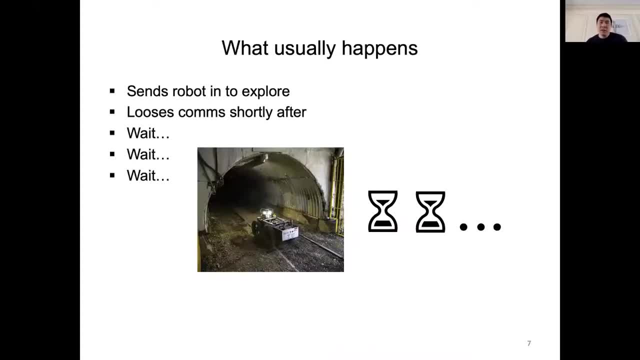 We are all roboticists. We are eager to do this even today. We want to send these autonomously exploring systems to autonomously map and scale all by themselves, And we are expecting them to come back at some point to bring us the full map of the environment. 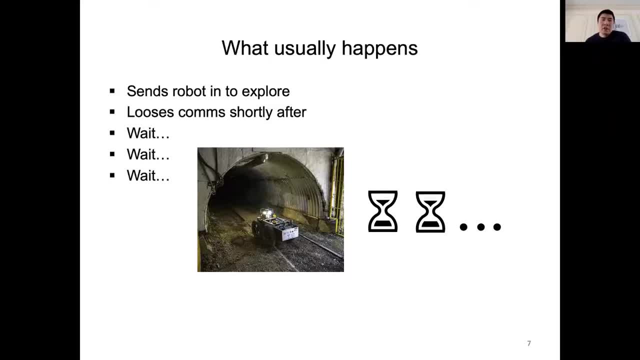 The realistic. the situation is not that optimistic. okay, This is the situation today. If you send these systems to autonomously explorer, this is what happens usually Once it gets in. Okay, we cannot go in with them because the spaces it has some kind of dangers for us to go in. 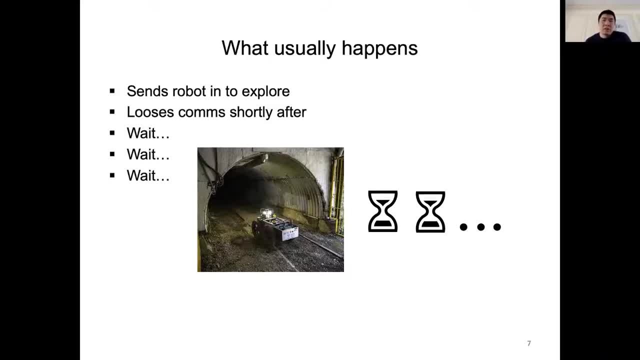 so the systems go in and shortly after they lose the communications to the outside, because the communications is something that we we usually cannot rely on at all time. that's just the way it is. so from there we don't know what it's doing. it may be still exploring, it may get stuck at some. 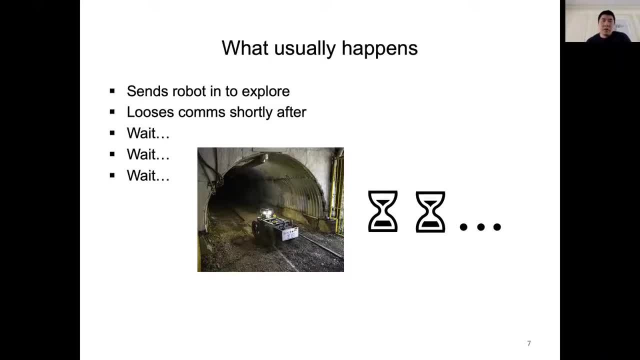 point. but we don't know. we can only hope that it will still come out at some point, and if it does come out, that's great. we have the data. but otherwise we wait hours after hours. at some point we say, okay, this is the way it is okay, so that's the overall behavior as a system and we 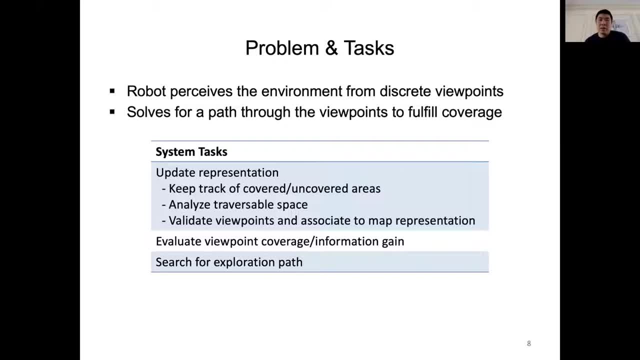 are talking about the exploration problem today. so let's try to look at the problem from- uh, theoretical perspective. let's try to understand the difficulty of the problem from a theoretical perspective. So first let me say a few words about the problem modeling, because the problem 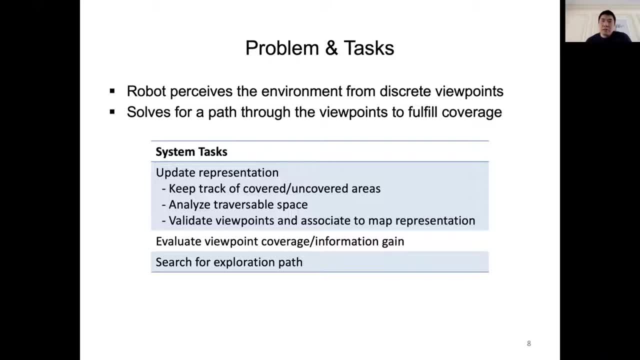 is discretized. In reality, the vehicle moves continuously through the environment and today's sensors have a relatively high frequency, usually from 10 hertz to 50 hertz. even So, it's almost that the vehicle moves continuously through the environment and it collects high frame rate. 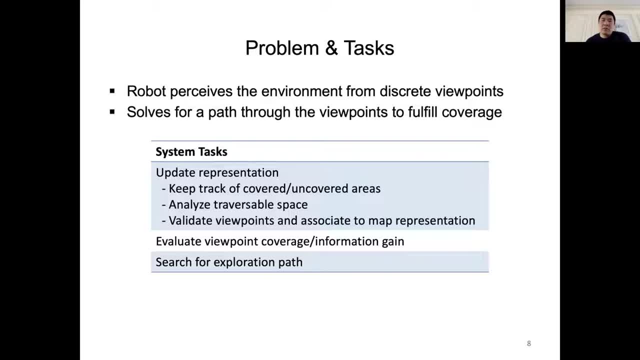 sensor data. It constantly scans or perceives the environment. the high frame rate, It's almost that it continuously covers the environment. But to be able to model the problem mathematically, we model the problem with discretized viewpoints. So the vehicle goes to. 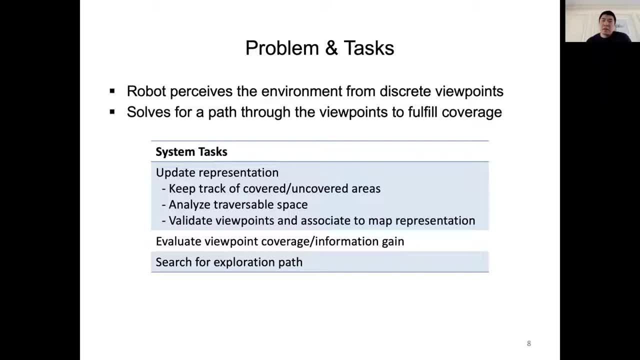 each of these viewpoints and it takes the sensor data and it perceives the environment from these discretized viewpoints. So, with that said, the exploration problem is a planning problem. It plans these viewpoints in the environment for the vehicle to go to each of. 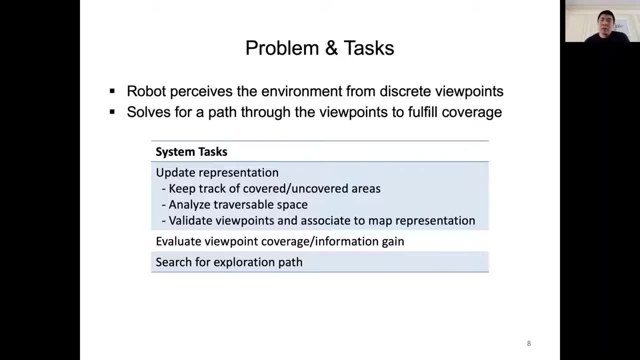 these viewpoints, So it takes sensor data and to cover the environment. The combination of this sensor data collected from these viewpoints basically covers the full environment. So from a systems perspective, there are several tasks that needs to be fulfilled for the system to autonomously explore and to map, So there has to be a representation of the environment that 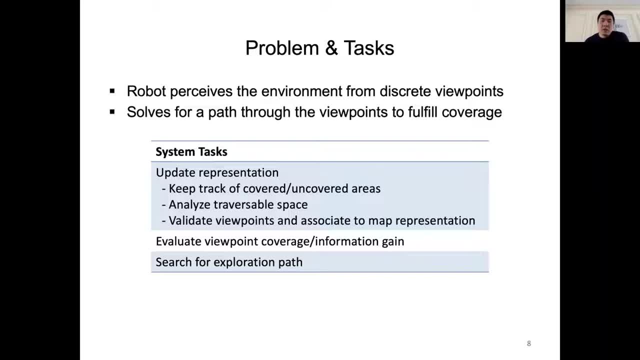 has to be constantly updated, it through the round. for us to keep track of the covered areas, the uncovered areas, The system has to be able to analyze the traversable terrain. for ground vehicles, For aerial vehicle, there's no need to analyze the traversable terrain, but there is a need. 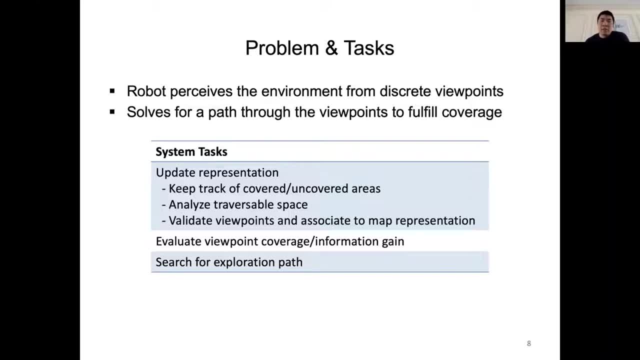 of analyzing the traversable space, Because for aerial vehicles it does not have to care. This part of the terrain is traversable and this part of the terrain is not, So everything that they see is an obstacle. But for ground vehicle it has to actively segment out. 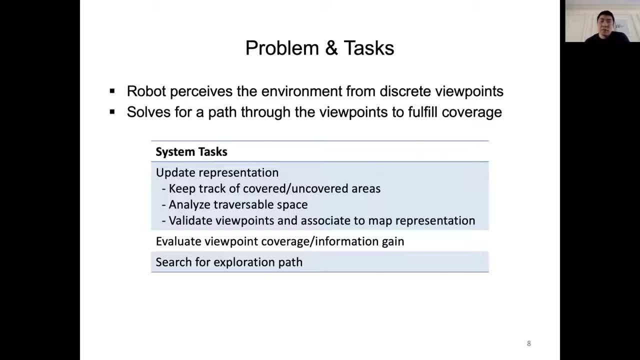 the traversable terrain from the non-traversable terrain. So this process is called terrain traversability analysis. So ground vehicle needs terrain traversability analysis. The system needs to be able to estimate the coverage from these viewpoints or to compute the information gain And from there 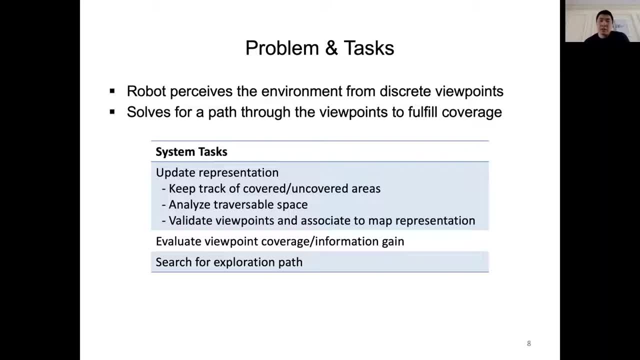 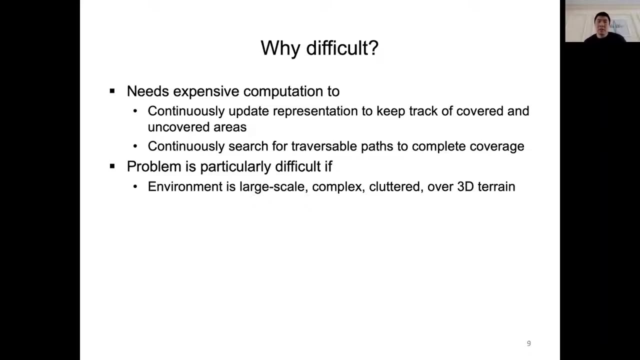 it searches this representation for the exploration path. So this is the whole process happening in the system, in the exploration process. Why is this a hard problem? Because there are two steps that need to happen continuously through the whole course of the exploration. First, 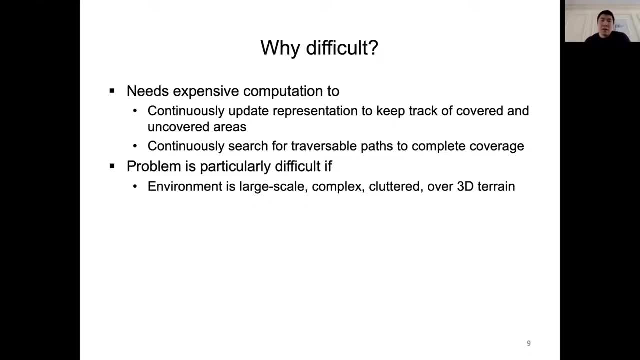 this system has to constantly update the representation of the environment to keep track of the covered and uncovered areas. Then it needs to search this representation for a traversable path to guide the vehicle through the environment to fulfill the coverage, And these two steps have to run constantly through the whole course. 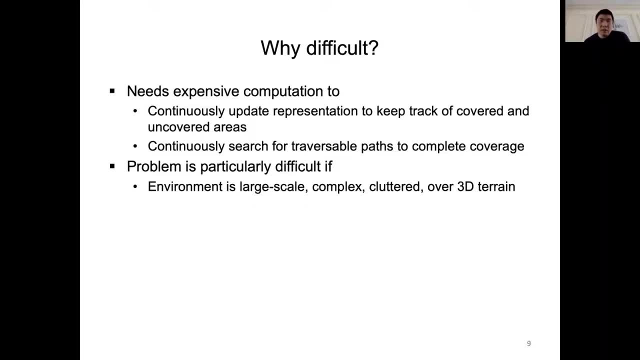 It's really not that you update the representation and you do one-time search So that you get a path. then you follow this path from the beginning to the end and now the coverage is done. It's really not that case, because the exploration process itself is a recurring process. 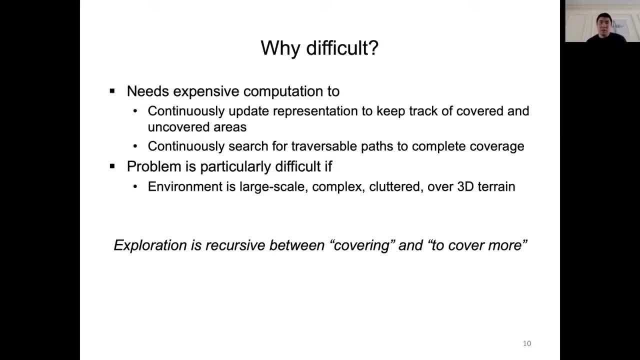 Okay, but let me briefly explain this point. The exploration is recursive between covering and to cover more because, as we're talking about exploration, it assumes the environment is unknown. It does not have any prior about the environment. Upon the system starts, it only sees a small area, basically around the sensor, and that's the environment that they know. 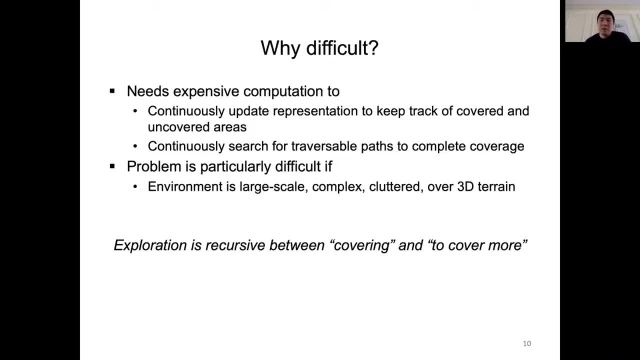 And from there, based on that data, it makes a plan to go to cover the environment that it has seen so far, which is a small area. But as it goes, it gradually sees more structures, It gradually figures out more layout of the environment. 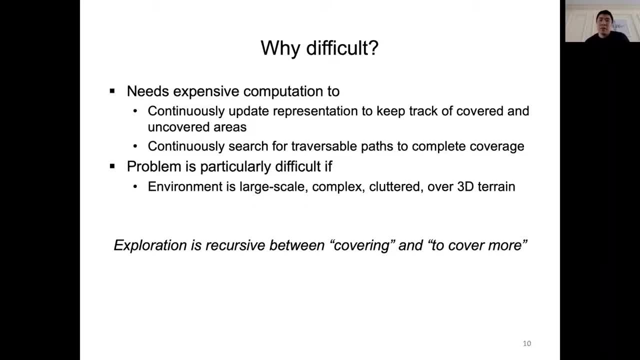 And from there it has to constantly update the representation and to constantly replant, update the path to cover the structure that it has seen so far, Because it gradually, Because it gradually sees more and more structures, more and more layout in the environment. 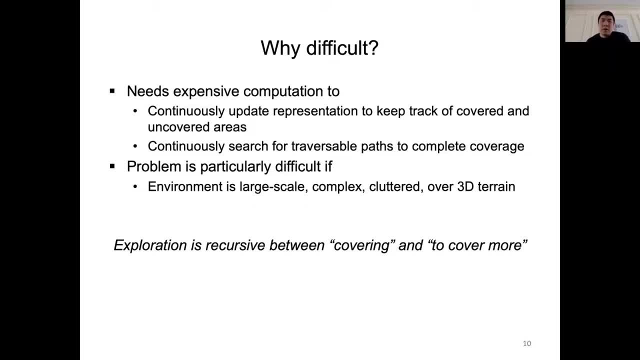 So this process has to recur until at some point, all the structures in the environment are covered and that's the end of the exploration. So you see, these two steps has to run all the time, from the beginning to the end, And it's a time consuming process. 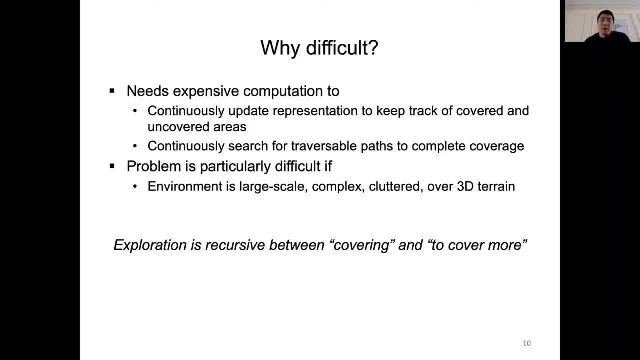 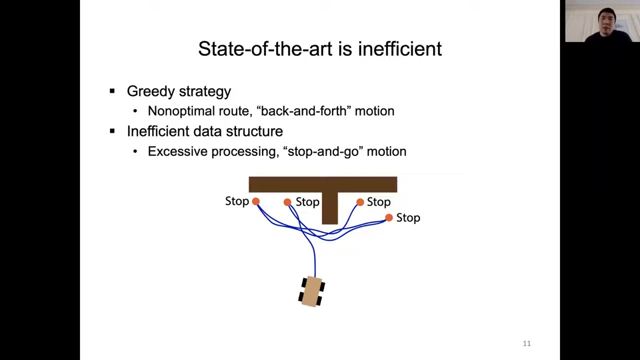 Especially if the environment is large scale or structurally complex, cluttered or over 3D terrain. the problem is particularly hard. Now, how is the state of the art doing? In general, I can probably summarize: state of the art is not efficient enough in exploration mainly because of two reasons. 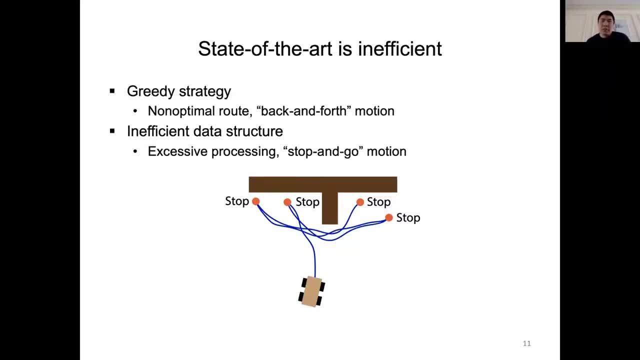 The first: a lot of these data. The second: a lot of these state of the art methods. use greedy strategies. so instead of optimizing the whole exploration path, it's only looking for an instant viewpoint or a few viewpoints, and it connects a short path through these a few viewpoints and optimize the short path to do the coverage in the vicinity of the vehicle. 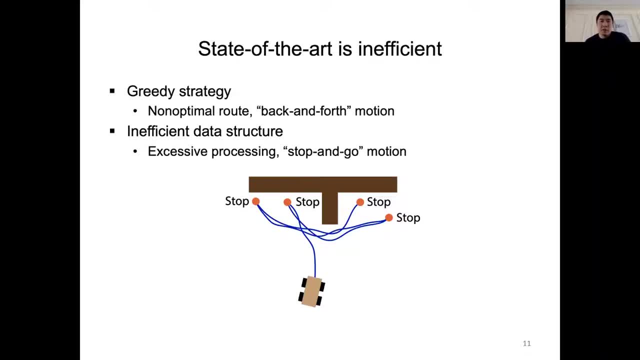 So the greedy strategy is ultimately myopic. The symptom with greedy strategy is it often gives us this back and forth motion Because it's myopic. it does not have a global picture from the past perspective. what happens is it usually comes to one place to explore, but it cannot explore that area fully. it goes to somewhere else. 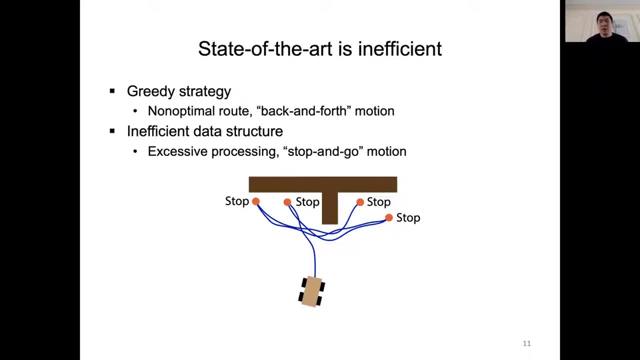 Then later on it goes somewhere else. Now it has to come back to cover more, but even that it may or may not cover it fully. So it comes here, it goes there and it comes back in the force and that reduces the efficiency of the overall exploration. 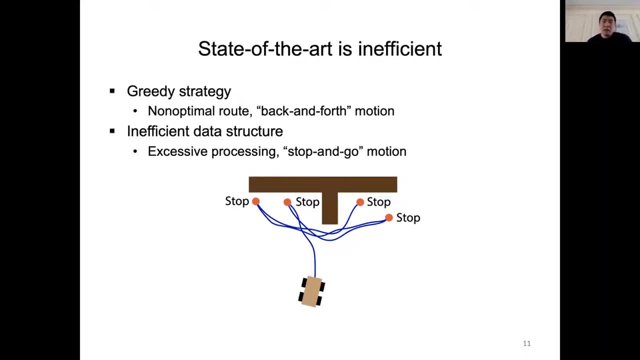 A lot of the methods don't use an efficient enough data structure. so the problem is a hard problem. It needs excessive processing. But if the data structure itself is not efficient enough, imagine this is online algorithm. the vehicle has to move continuously in the environment to do the coverage. 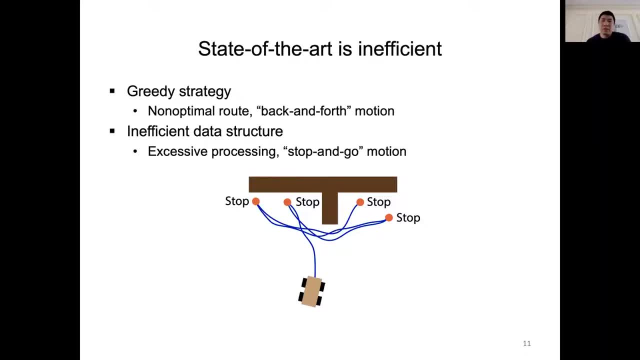 If it takes 10 seconds for the algorithm to come up with a path, the vehicle has to wait in there for the path to come out. If it takes one minute, the vehicle has to wait for probably almost a minute, So a lot of the time because of the 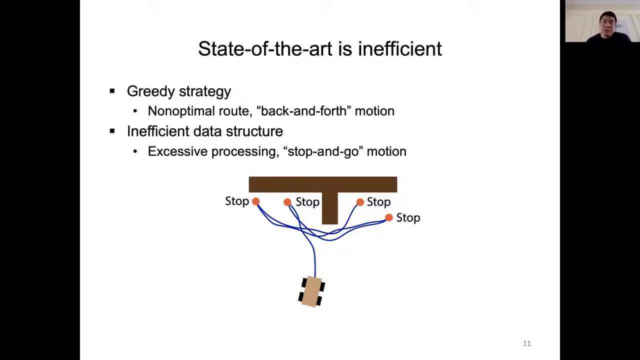 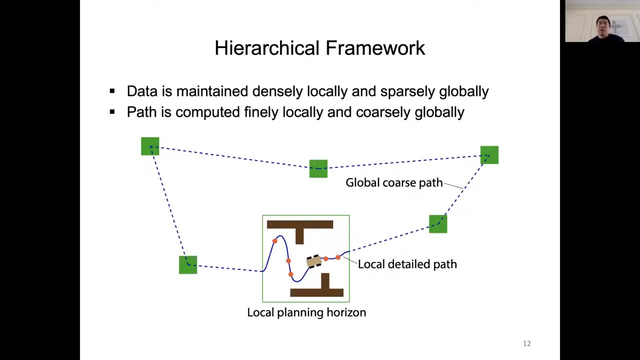 inefficient data structure. the vehicle stops and goes in the environment, and that limits the overall efficiency of the exploration. Okay, So this is a quick overview of the state of the art methods. So here is our exploration framework We started work from more than a year ago, and the purpose of this framework is 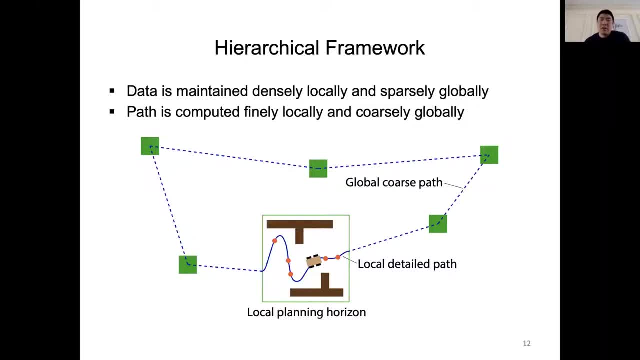 basically to push the limit of the efficiency in exploration. So if you look at this framework, this is a hierarchical framework with two levels in the data structure. We have first a local area which is in this, in this big green box, which is what we call the local planning horizon. The local planning horizon is an area surrounding the vehicle and it moves along the vehicle In this local planning horizon. 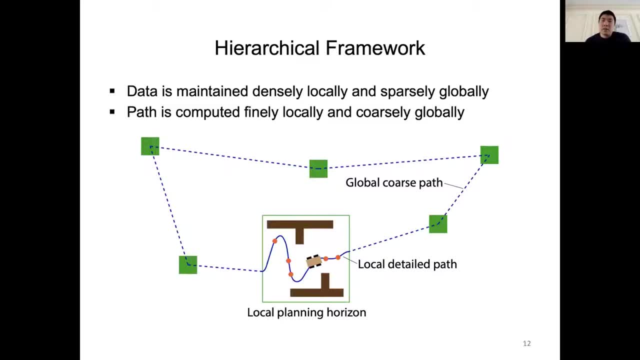 we maintain the data densely and we compute a detailed exploration path within the local planning horizon, But out of the local planning horizon, in the global scale, along this dashed blue line which is a global path, so that's our global environment. we maintain the data sparsely, only in these small green blocks. 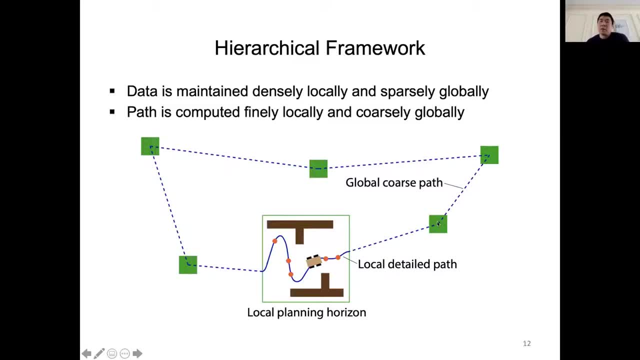 Okay, so these, these, these little green blocks are where the information is stored. So I'll get to this point later in the in the talk, because this is a important representation in our framework. but for now, let's let's understand: the little green blocks are where the information is stored and the little green blocks basically mean those areas are not fully explored. they need more coverage or more. 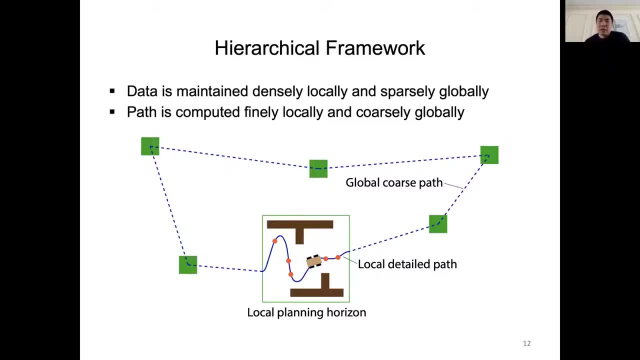 exploration in the future. Okay, so it's. it's kind of putting a mark in the environment to say, okay, I have to come back here to explore more at these little green blocks. Okay, so, at the global scale, we maintain data sparsely in these little green blocks. we compute a very chorus path through these green blocks. 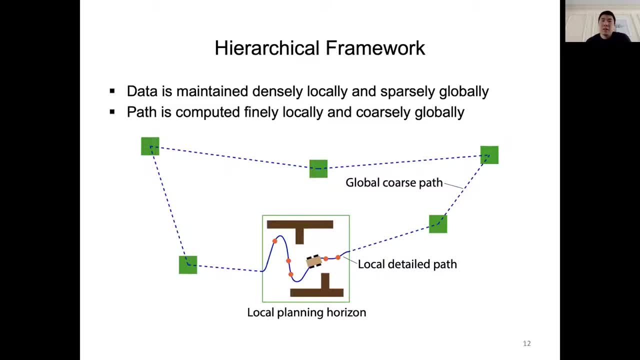 our global path. so the whole inside behind this framework is in the vicinity of the vehicle, close to the vehicle. we need to maintain dense data. we need to compute detailed paths because that's helpful with the navigation, but at the global scale it's not necessary to maintain the data at that density. 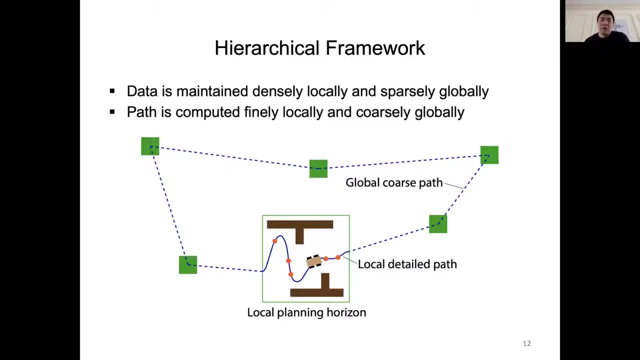 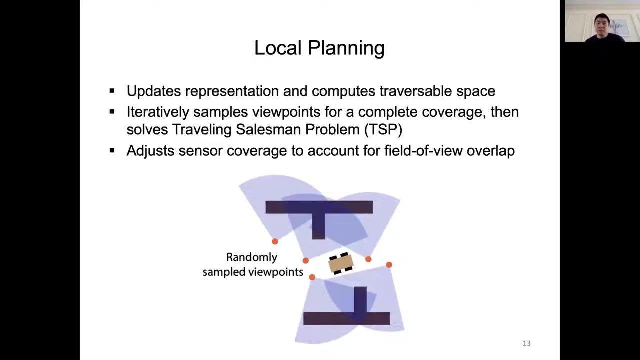 We seriously turn down the resolution, use sparse representation and trade it off for computational efficiency. Okay, so that's the whole inside behind this framework. Now, in the next few slides, I'll briefly talk about the processing at the two levels. So here is the processing at the local level, which we call local planning. The local planning. 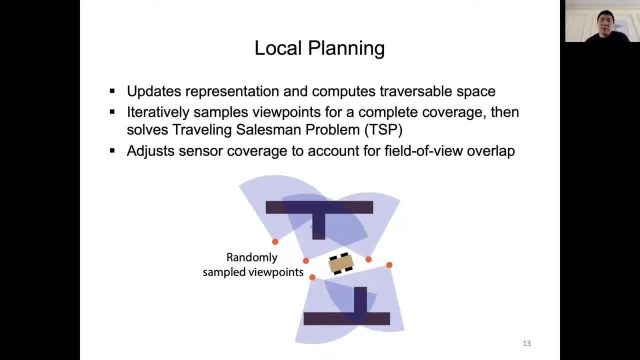 is to compute a set of viewpoints and paths through these viewpoints to fulfill sensor coverage around the local planning horizon. The local planning process is a recursive, random sampling process. It's iterative. we sample multiple sets of the viewpoints and each set, the combination of viewpoints, fulfill a complete coverage of the structures around the local planning horizon. 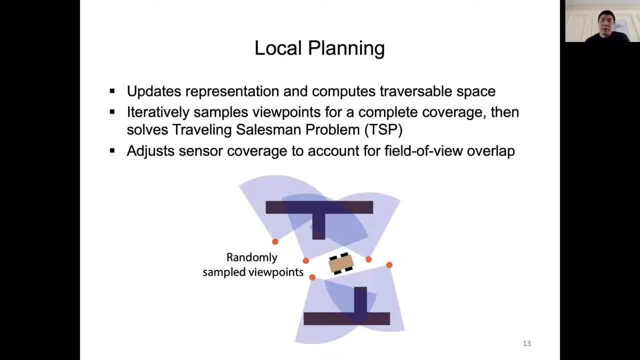 So the algorithm samples a set of viewpoints to make sure that there is a full coverage, and it samples more sets of viewpoints For each set. solves the traveling salesman problem to find the tour through these viewpoints and in the end it picks the tour that has the shortest path. okay, so one characteristic in the local planning problem. 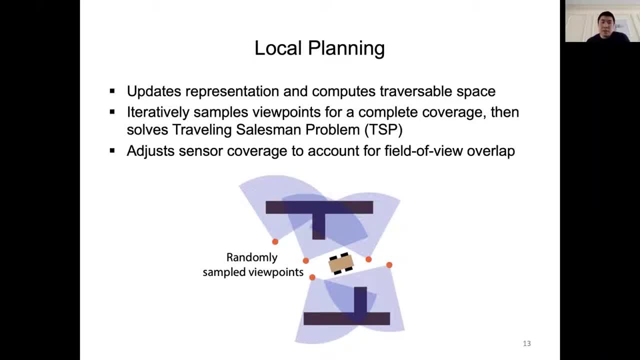 that is worth to mention is there are sensor field of view overlaps in between these viewpoints, because if you look at the structure in the environment, it can be seen by multiple viewpoints. so this characteristic results in what we call the sub modularity of the problem. and dealing with the sub modularity, or the sensor field of your overlap, takes a little bit more. 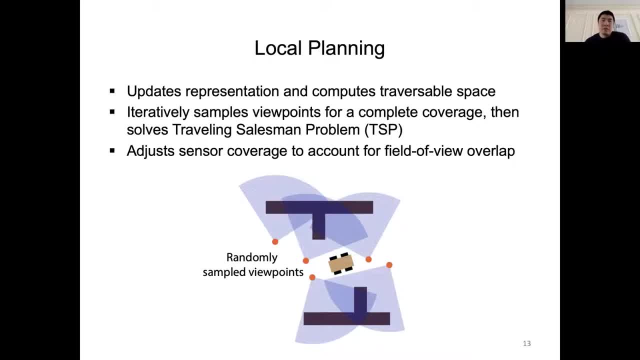 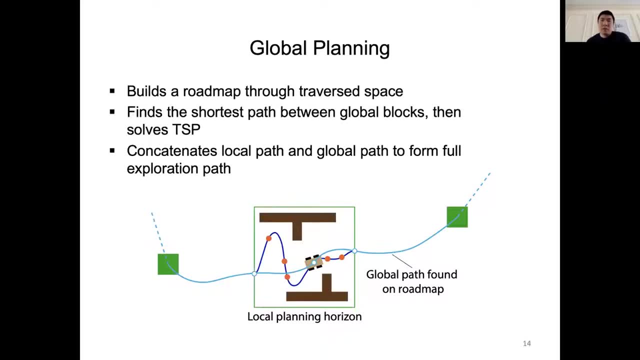 processing in the local planning of process. okay, the global planning builds a map through the traversal space. as a vehicle moves through the environment, that gradually develops a road map which is basically a graph, and this graph indicates the traversable space through the global environment. then on this road map, we search the shortest passes. 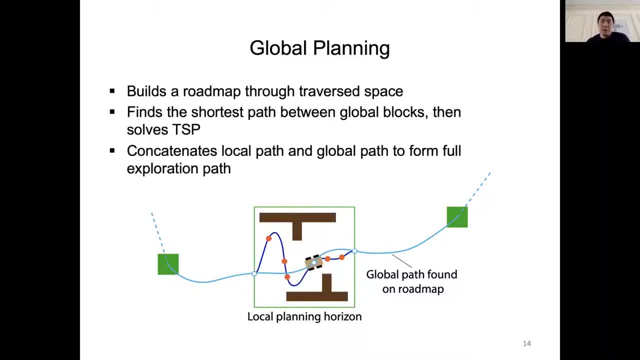 in between these little green blocks. remember, these little green blocks are where the information is stored and they are the areas that need more coverage. so we we search the shortest path in between every pair of the little green blocks, then then we solve the traveling salesman problem, again as a global scale. uh, to get a tour through these little green blocks. 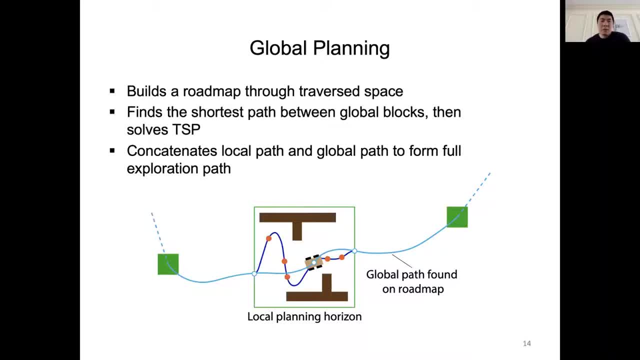 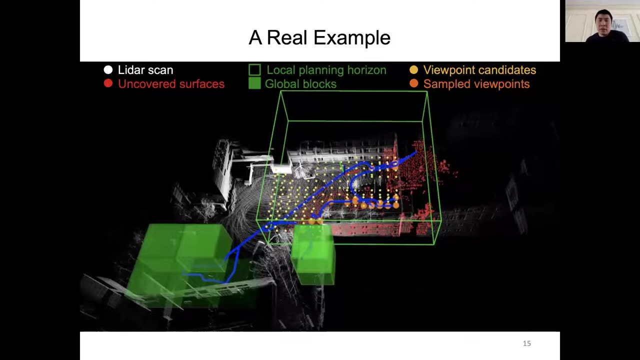 then the the local paths and the global paths are connected on the boundary of the local planning horizon. so that gave us the overall exploration path. okay, so that's um an overview of of the technical procedure. let's use this real example to understand this exploration process a little bit better. so this is real data from aerial vehicle exploring a few buildings on the. 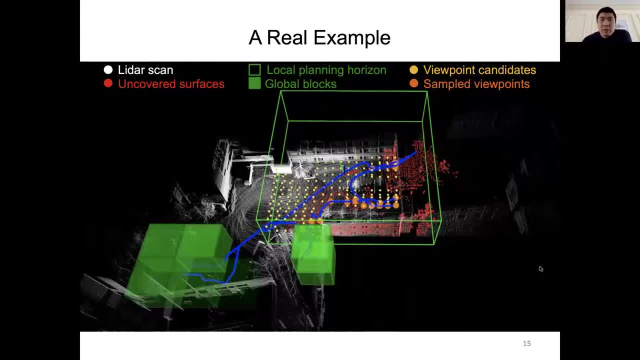 university campus. so this, this big, this big green box here is basically the local planning horizon, and these smaller green blocks are are where the information is stored. um, the blue path is the exploration path, obviously. so if we look at this, this green box, this local planning horizon, we see these little orange dots, you know. 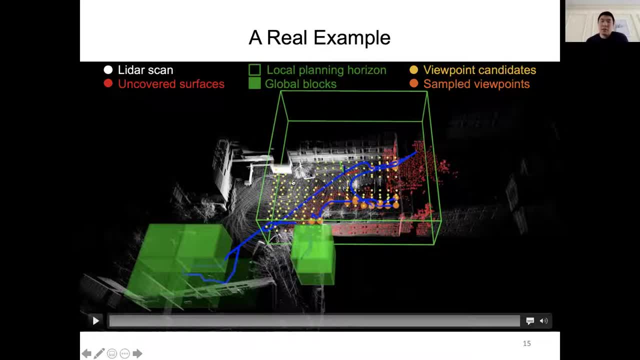 great pattern. so so these little, uh, so these little yellow dots, not orange dots, these yellow dots are what we call the viewpoint candidates. so we we evenly distribute the viewpoint candidates, our grid pattern, in the local planning horizon and in the traversable space. okay then, when we randomly sample the viewpoints, we randomly 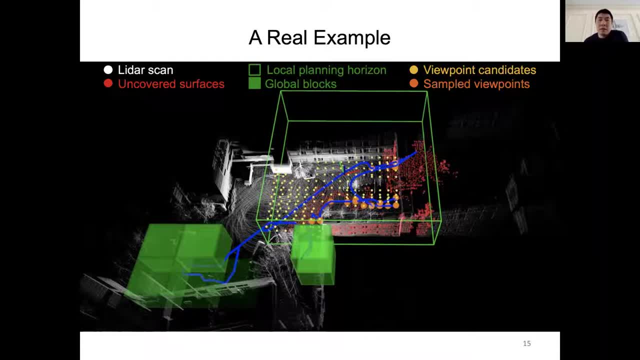 pick them from the viewpoint candidates. if you look at these bigger orange dots here along the path that's the run randomly sampled viewpoints. we we basically randomly pick them from the viewpoint candidates on the grid and these selected or or sampled viewpoints, or these bigger orange dots, are the sampled viewpoints. those are the points that the vehicle 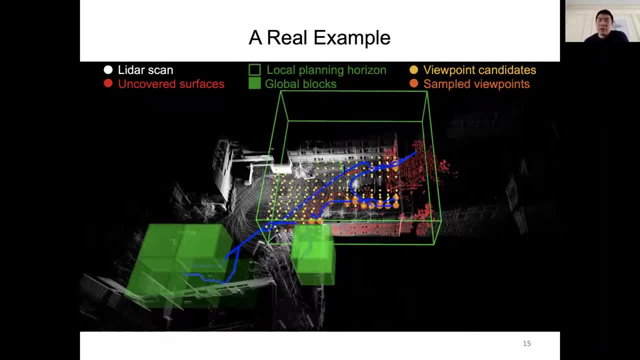 should go to to collect the sensor data and the combination of the sensor data from these bigger orange dots- uh cover the whole environment. then from there we can put a path through these sampled. so let's watch this video. this is aerial vehicle exploring to the right side, um. 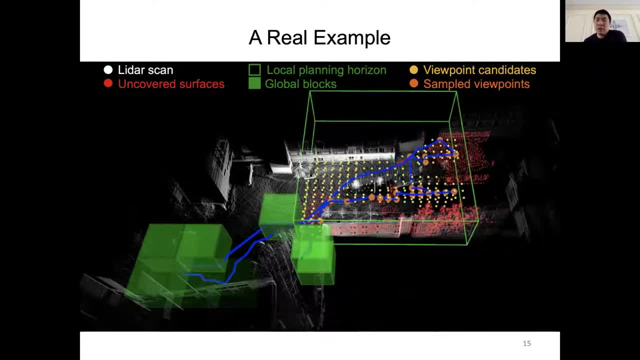 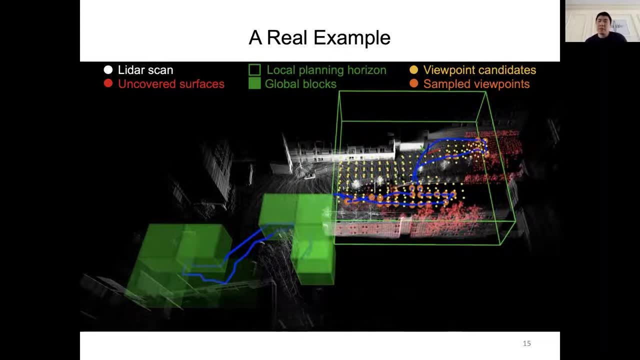 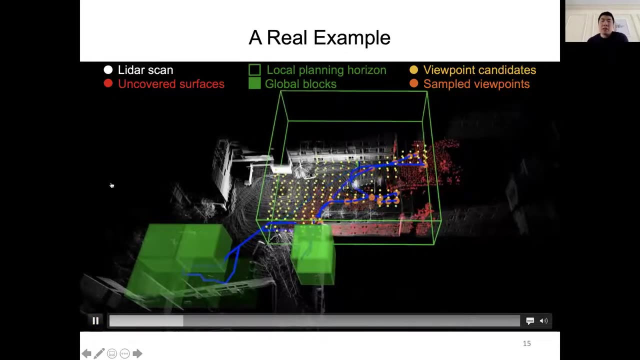 the re-planning is one hertz, so every second you see, the representation is updated, it's extending to the right side and the paths is replanned to the right side. okay, so let's watch this process one more time, and this time let's pay attention to these little green. 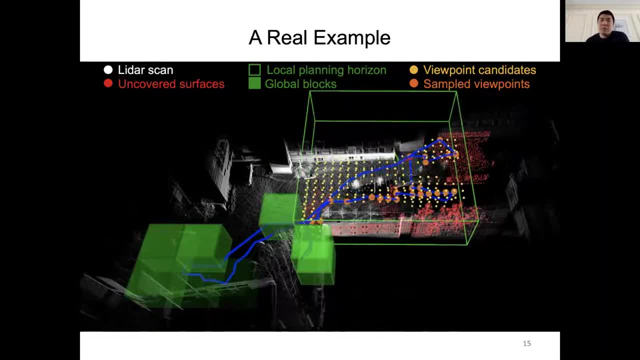 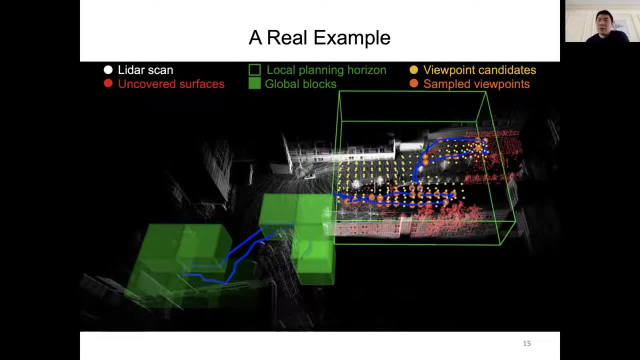 blocks. so we said the these little green blocks are where the information is stored. they are the area that needs further exploration, right? so let's see how they are generated. they are actually generated from the local planning horizon. they are left behind as a vehicle explores if there are areas. 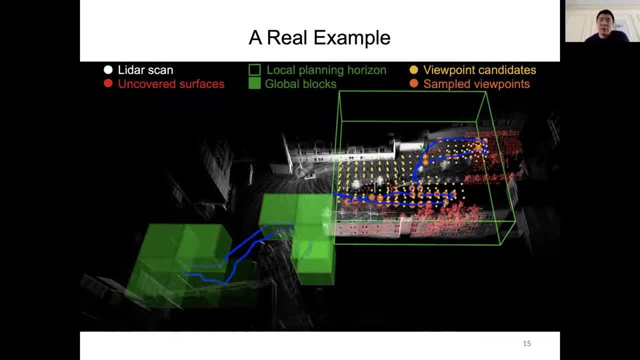 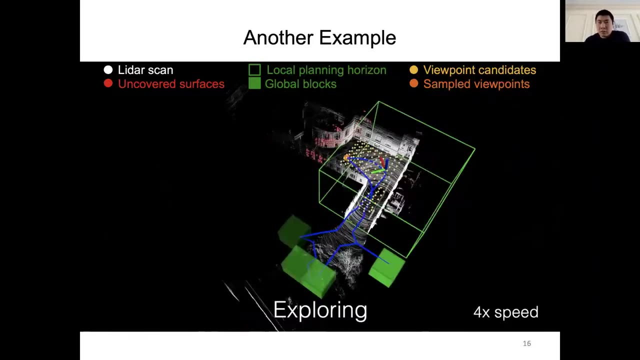 along the way that are not fully explored. the algorithm leaves these little green blocks behind and to remember that it needs to come back at some point to explore more. okay, so here is. here is another example. um, that i want to, that i want to show, and while we watch this example, 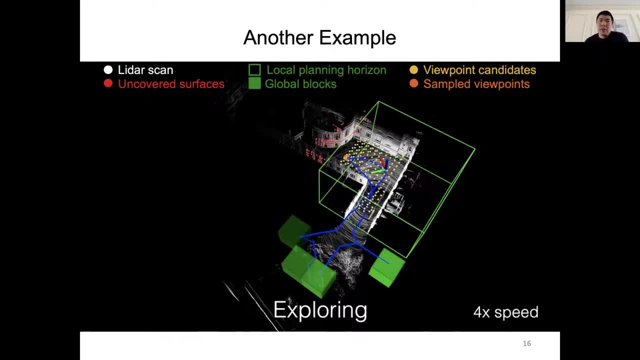 i want to explain an important phenomenon, which is exploration versus relocation, because if you explore a realistic environment, it actually often has intersections in it. when you're at an intersection, you can only pick a branch to explore. that's the only way to do it. you have to pick one and once you go in to explore that branch. 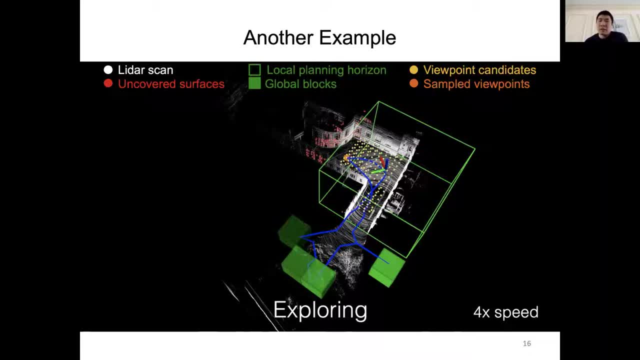 and that branch is fully explored. you need to come back, to relocate yourself back to the intersection and from there you can explore the other branches. okay, so this video is about that: this area with these little green blocks, and this is where the intersection is. okay, the vehicle is exploring. 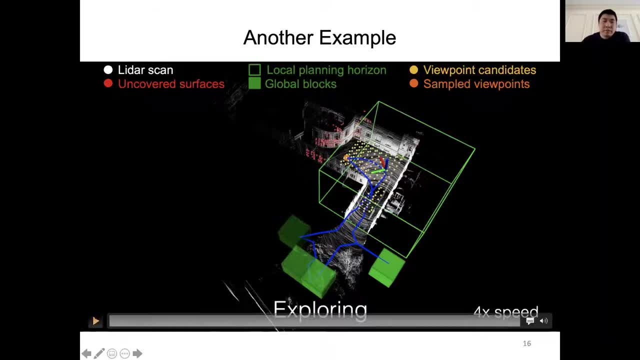 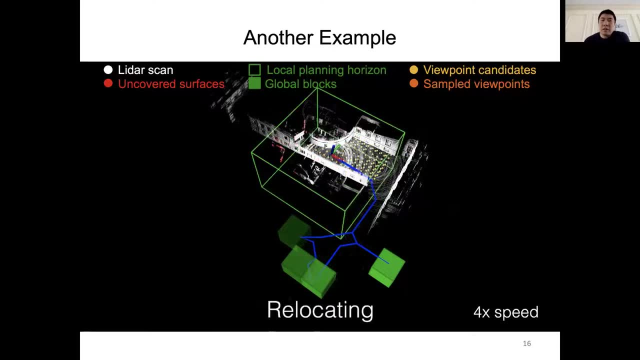 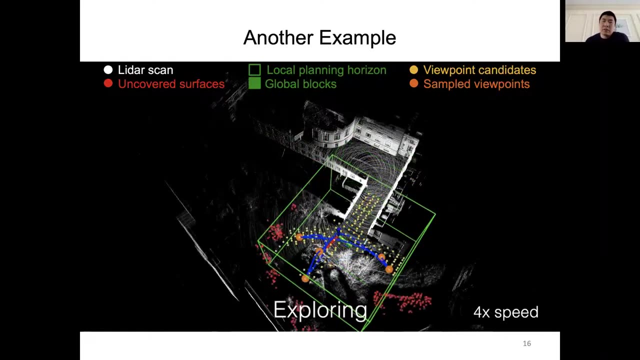 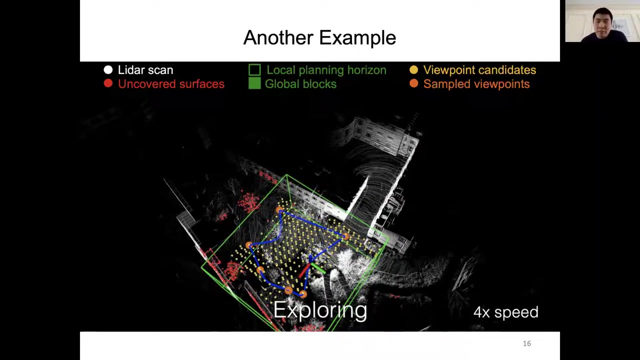 through this branch to to here and that's the dead end. okay, now we're seeing the vehicle is approaching the dead end. now that whole branch is fully explored, it's relocating its back itself back to the intersection. and once it gets to the intersection, it starts to see these orange dots. the orange dots indicates the uncovered surfaces. 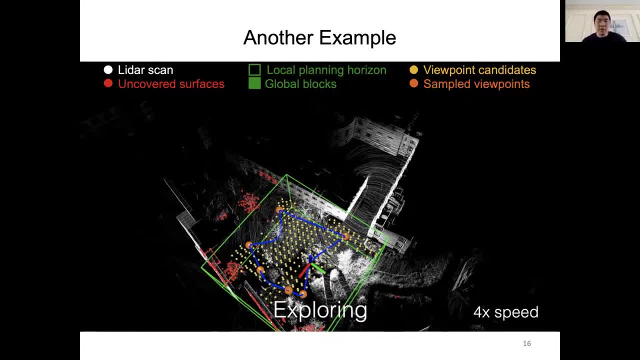 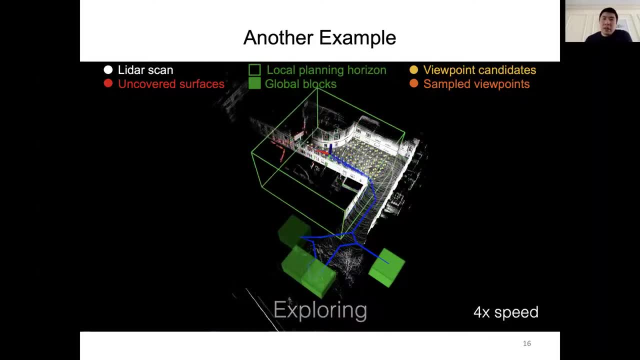 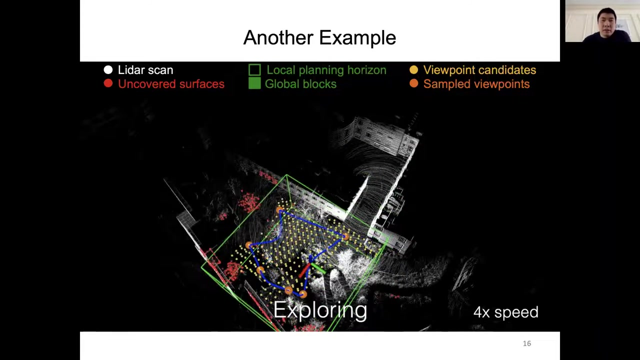 and from there the exploration resumes. okay, so one more time. um, right now the vehicle is exploring to the, to the end of that branch, and it's relocating its back to the intersection, basically getting itself back to these little green blocks. and once it gets there, it starts to see more of these red points, which means that now 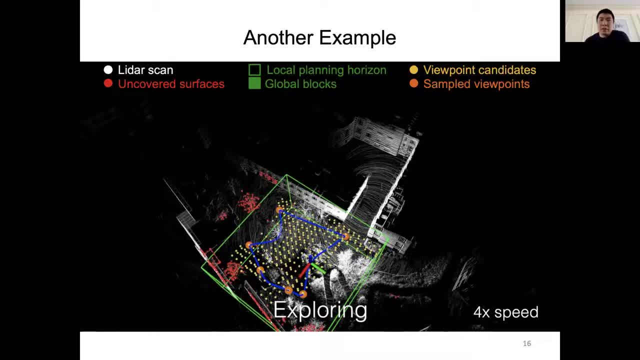 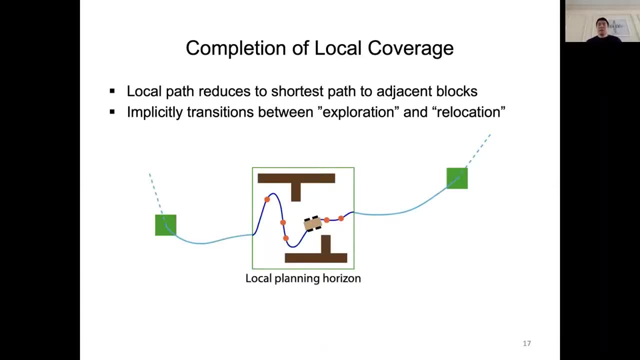 it sees more uncovered surfaces and they start the covering process already and you see that the influence of the vehicle activities is stronger at some point. okay, there, i don't know if you can see that, uh, the chrome thezenita that is here showing the yellow point. um, so this, the white point, is this area. 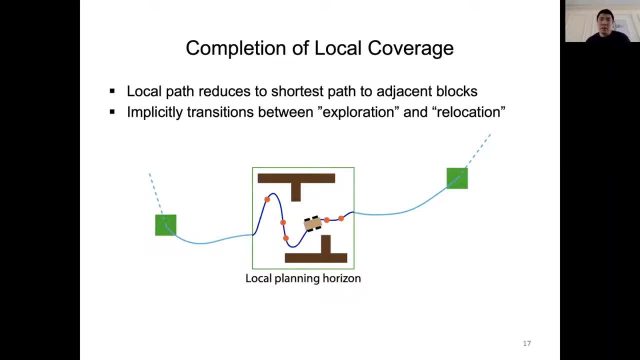 uh, here, and you can see that now, this chain here, the little yellow over here, signals this side of the car. so this is the front difícil, then the one on the right side of the Series 3. up there is the hill, the other one that runs at 1.8m. 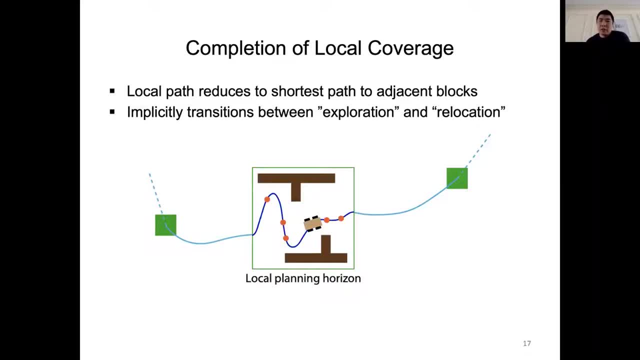 University of MarylandOT needs to be covered in the local planning algorithm. If you look at these two brown things here, these two brown structures, those are the structures that need to be explored. So the local planning algorithm places these arch stars along the path and it plans the detailed. 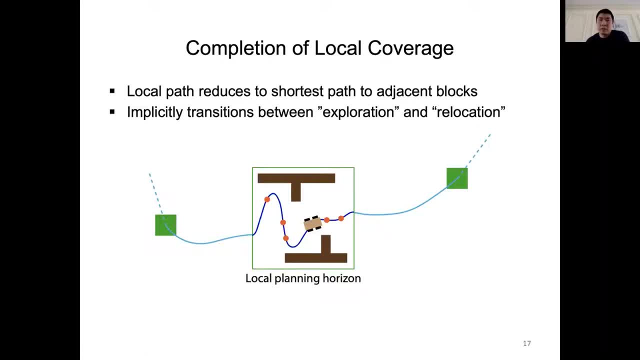 exploration paths to cover the structures in the local planning algorithm. But once it gets to the dead end, that whole branch is covered. There is nothing more to cover. The local planning algorithm basically degenerates. There are no more viewpoints along the local path, This local pass. 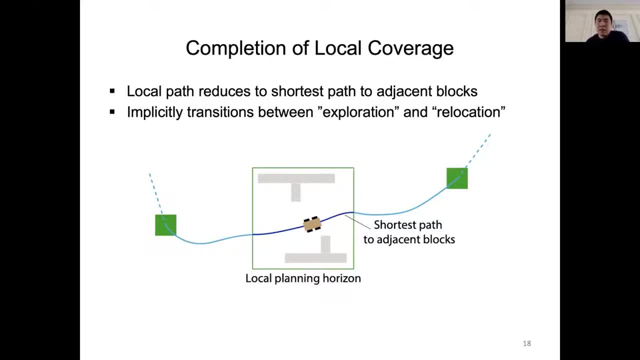 basically reduces to the shortest path that connects from the vehicle here, from the vehicle to the boundary of the local planning horizon and from there it connects Basically, that's the goal to the task of three tracks. You can see the two tracks 사�镜 Под bearded and the male for historical facts inils. 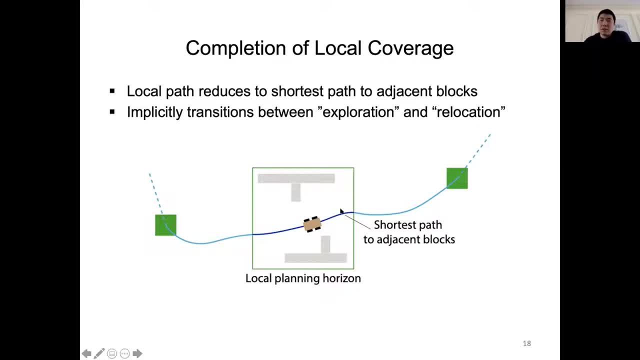 global path and through the global path it connects to the next green block. okay, so the local path reduced to the shortest path, so the local planning or the boundary, and from there it connects to the next little green block on the global path. remember we said that the little green blocks are. 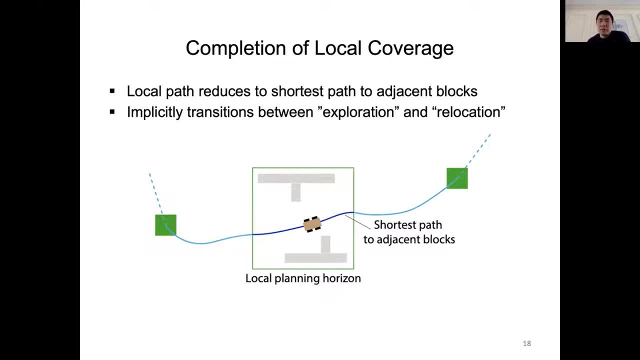 they are important in this framework. they mean not fully covered areas and they need to be covered more. so what happens is the vehicle is basically guided through this path to relocate itself to the next little green block on the global path, and once it gets there, it starts to. 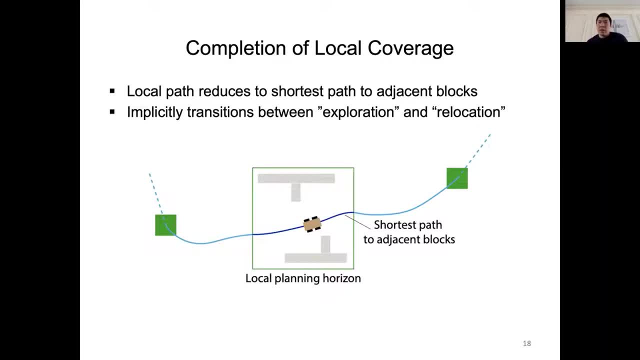 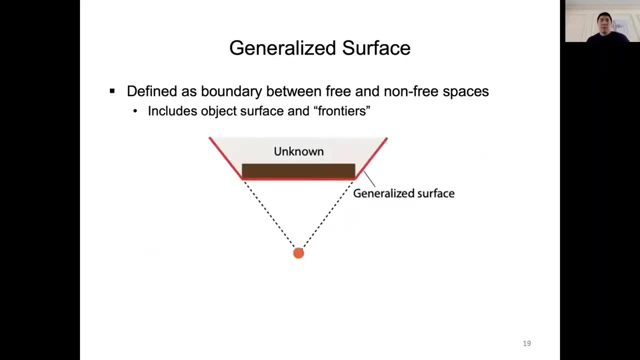 see more uncovered structures and the explorer, the nominal exploration process, resumes. okay, um. so here are a couple more details, uh, about the framework, before we, um, look at the results. so one um one detail is the definition of surface. in our system we define surface as generalized surface. the generalized surface is basically the boundary between free. 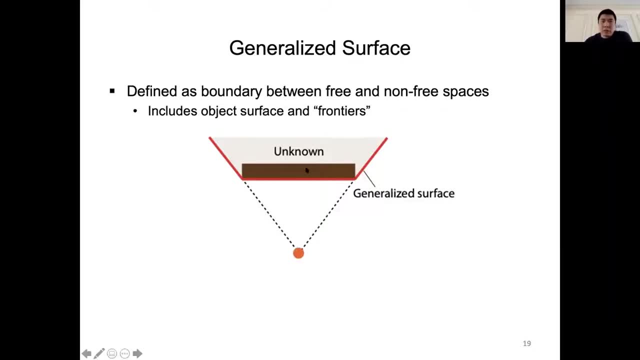 space and non-free space. so if you look at this object, which is this, this brown structure, when the sensor sees from, when the sensor sees the structure from one direction, it sees the front surface, which is this part on the red line, but there is also an unknown space behind the unknown. 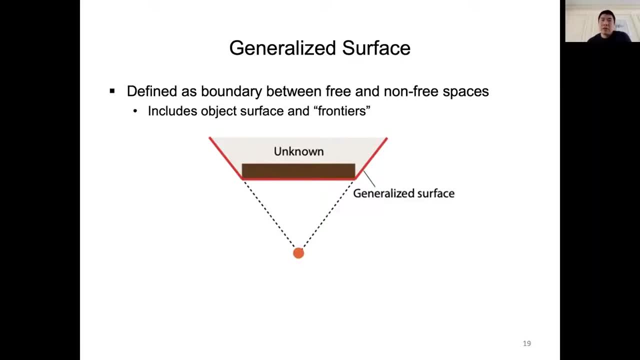 space basically means we don't know what's there. it could be occupied, it could be free, but we don't know. okay, now the definition of the generalized surface includes the boundary between the unknown and the free. okay, so this, this part, basically, is also included as the generalized surface. 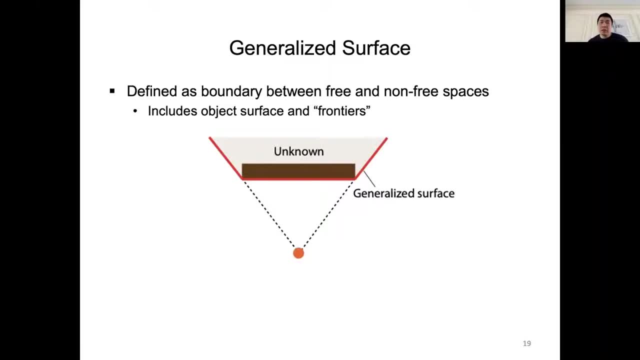 if you look at the traditional frontier-based exploration, the frontiers are defined as the boundary between unknown space and free space actually. so basically just the these two parts on the two sides that's used by the traditional frontier-based exploration to explore. basically, the frontier-based exploration is guided by these two little parts on the two sides, but ours include 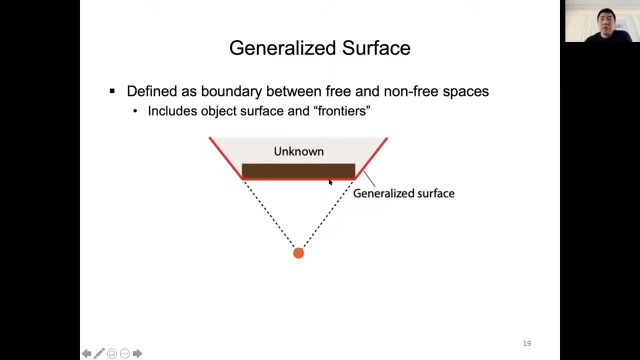 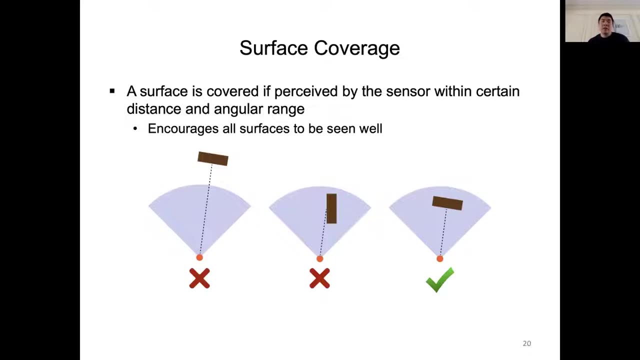 this, this front surface in the front of the object. okay then now, based on the definition of the generalized surface, here is our criteria for a surface to be covered. so this coverage criteria. it's unique to us. this criteria is not there in the traditional frontier-based exploration. so this criteria is defined based on our observation that 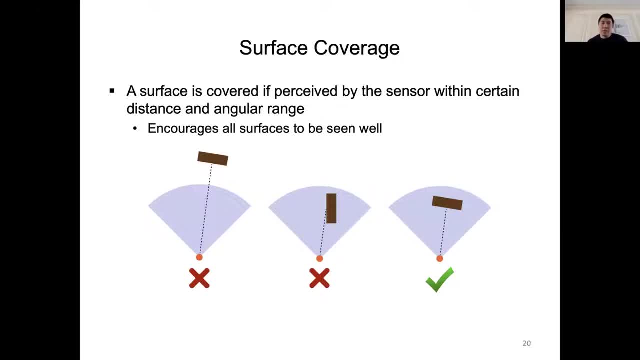 today's sensors can usually see quite far away. if you look at our system, the 3d lidar in our system can see up to 100 meters, but when it sees from that far it does not necessarily see well enough. so this criteria is to encourage the system to approach all the structures in the environment. 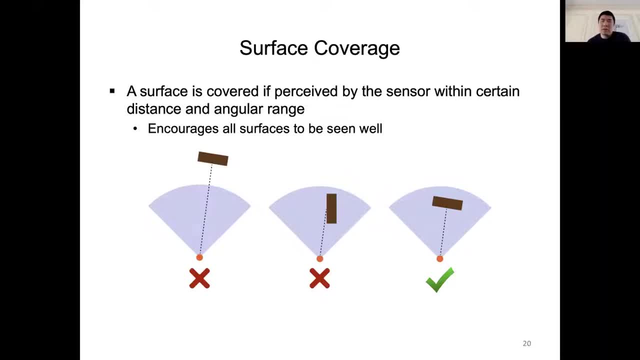 to see them well, within certain distance and within certain angular range. okay, so at this point let me recap on what i said. the exploration process itself is a recurring process because as the system starts, i only see the small area, and from there, that small area is enough for it to do, to come up with one plan. and when the vehicle follows the path, 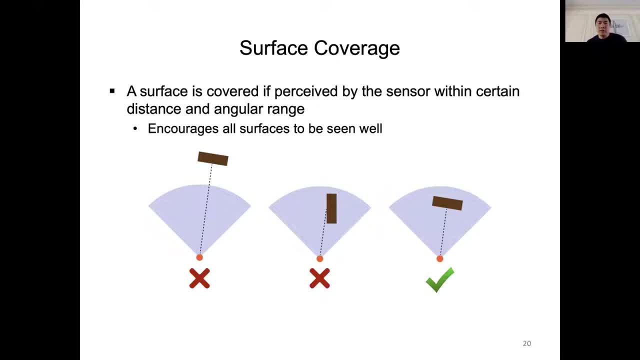 to explore that small area. it gradually sees more structures in the environment. it sees them, but then there are multiply. so the information on the map that isει skps étaient y, the representation that replans to approach half the fact that ert hogy k oxygen. 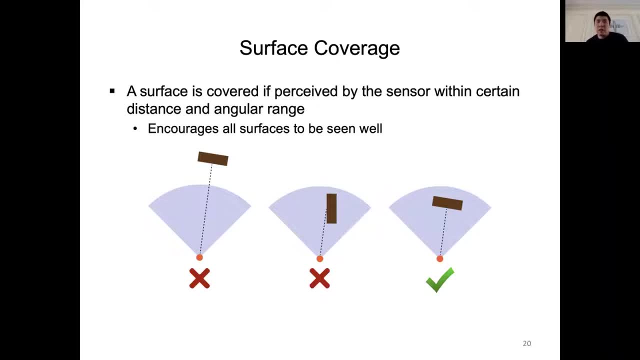 பรד�도 phут, peninsula, nimalbut an apathetic representation that it re-plans to approach these structures that have been seen so far, these structures that to cover them, and along the way of covering these structures, there is ever weight of. 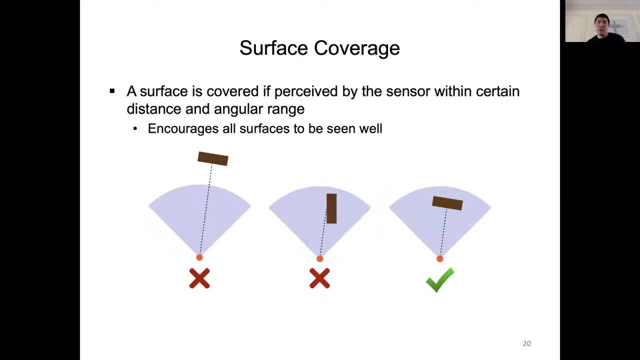 covering these structures. there are even more structures in the environment, so gradually it stays that they beach more, it tries to cover more, and that when it tries to cover more, it sees even more more. as it tries to cover more, it sees even more. so this is how the recurrent happens. until at some point the whole structure is firmly on how it went. until at some point the whole structure, the whole environment is time-LANED, structural. the whole environment is time-landed until exactly when it starts to surge. we are even more tired as it starts. 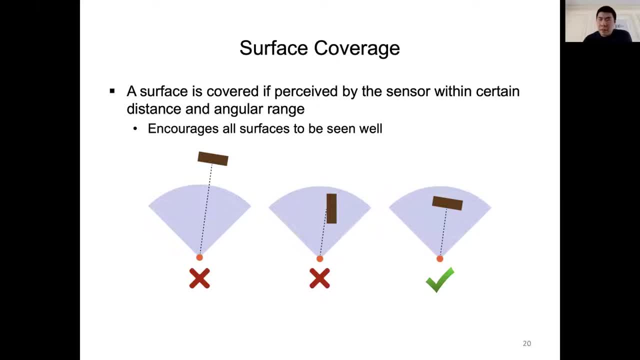 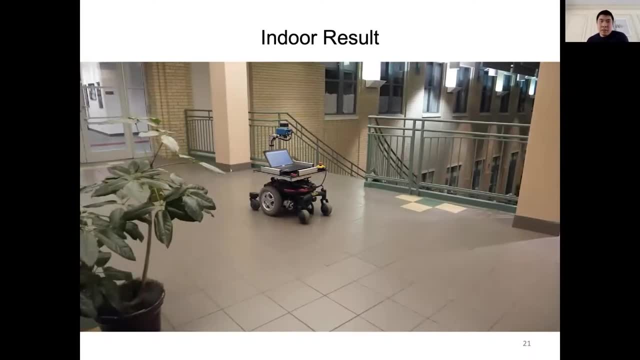 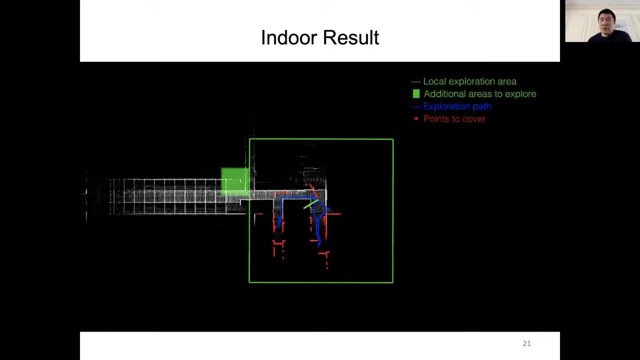 the environment is covered and the exploration terminates. Okay, so that's about the technical part. Let's look at some of our results. Here is a result of exploring a large indoor area starting from a building on CME campus. It's exploring through another two buildings. 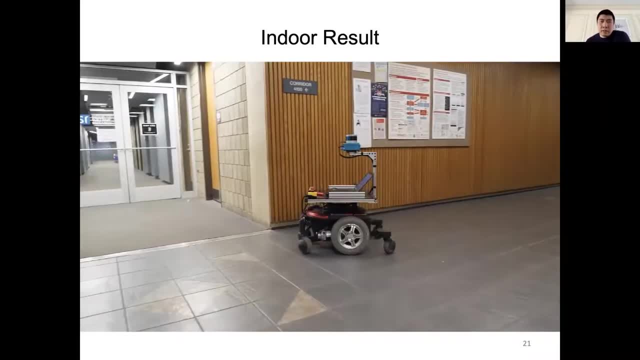 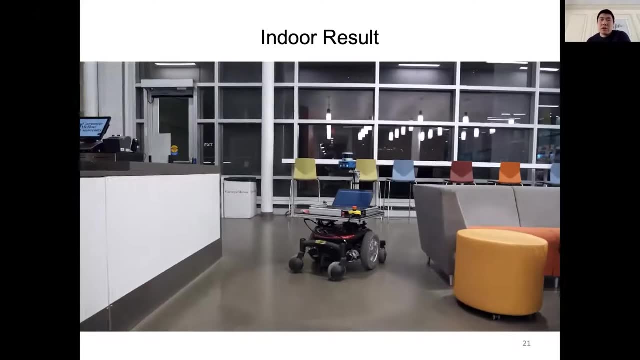 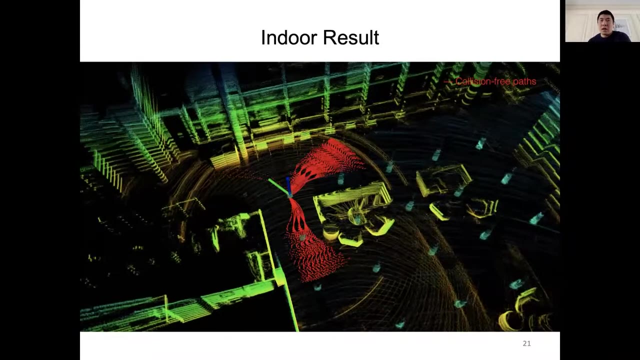 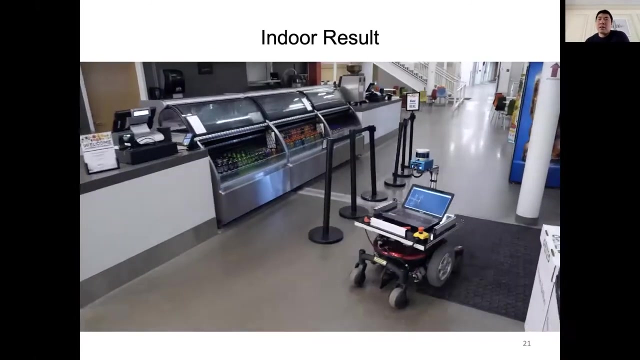 through connected hallways. So an environment like this is a typical indoor environment. It has mostly long and straight corridors connected through some of the larger dining lobby areas. This has a few typical difficulties or challenges, as in most of the indoor environment, And the challenges have to do with glass. 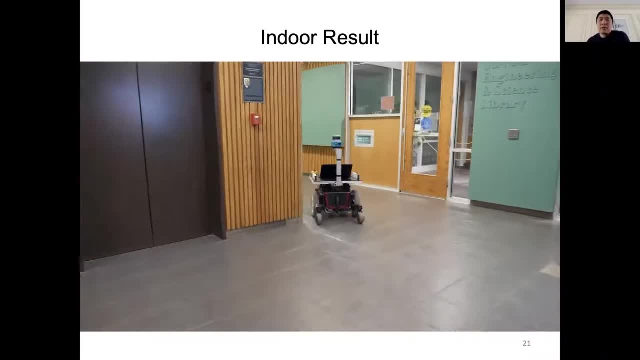 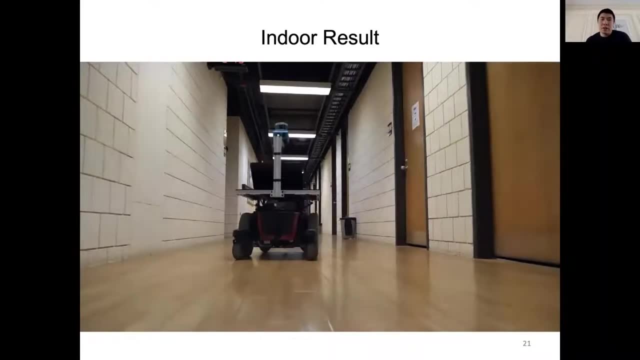 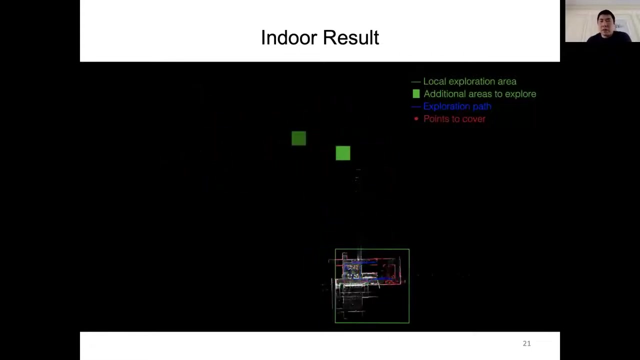 and scene structures. So in a few seconds we will see the whole exploration process actually right here. This is the whole exploration process And I want you to pay attention to these little green blocks. These little green blocks are left behind by the vehicle. 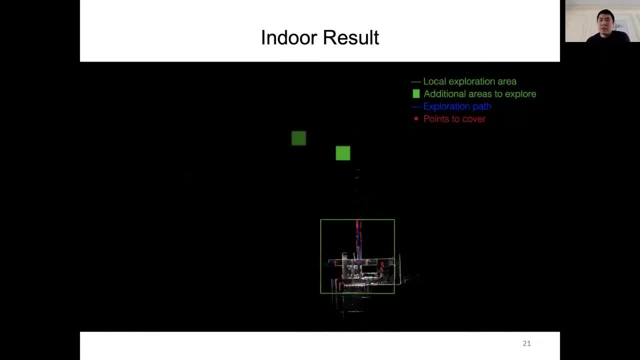 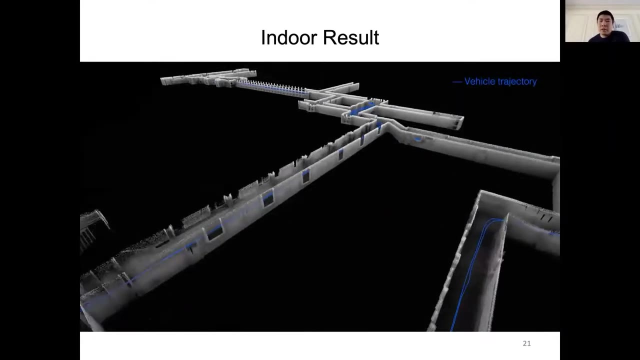 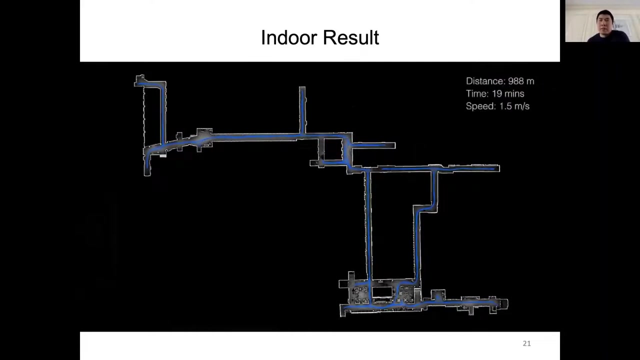 As it explores it determines those areas need more exploration, So it marks them down and later on it will come back to them to explore more to clean up these green blocks. Okay, So that's the overall map of the exploration. The whole process has about eight kilometer of travel. 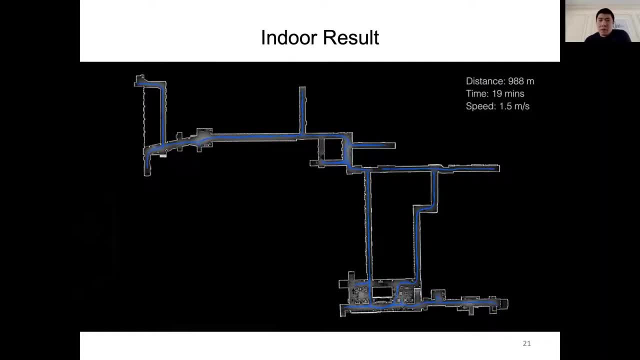 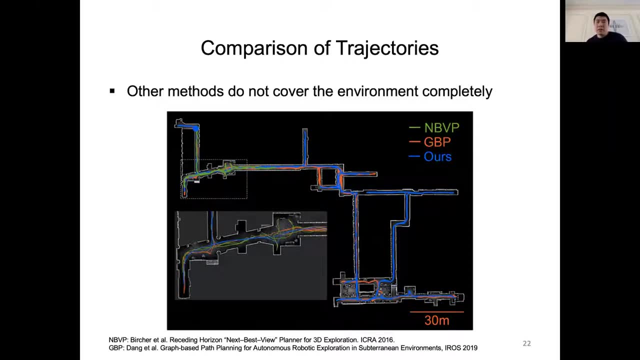 over almost 20 minutes. Okay, So here are some comparisons to the state-of-the-art methods. we're comparing to two other methods. The one is called MBVP- It means Neck Best View Planner, which is from ETH, And the GBP method is. 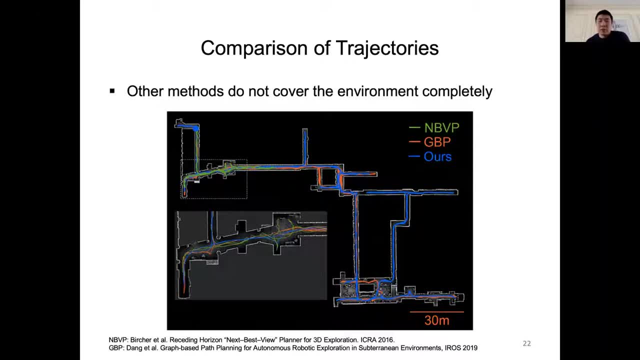 it's called graph-based path planning for autonomous exploration And it's from University of Nevada. So the MBVP method uses an RRT data structure in the back, It considers the nodes on the RRT as the viewpoints and it selects the best branch in the RRT. 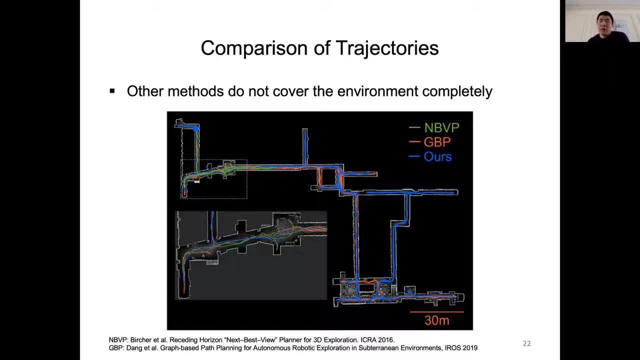 So, while this is sad, this is a typical greedy strategy, because it's selecting the best branch, The branch is the best branch And the branch only has a few viewpoints on it. So it's greedy and it's mild. The GBP method is sort of an extension of the MBVP method. 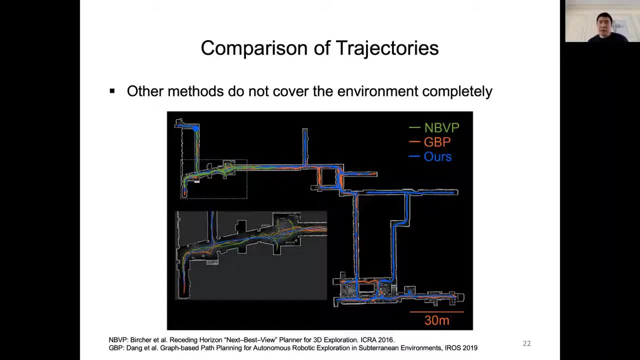 because the MBVP method has some limitations in dealing with very, very large environments. Now the GBP method uses it has two levels running side by side at the same time And it uses heuristics to switch in between these two modules. So one module is basically like that, one module is basically like the other one. 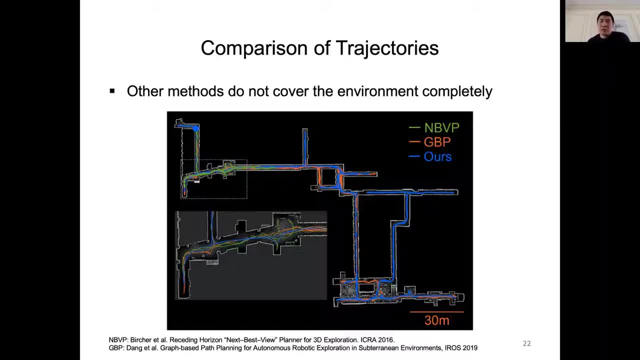 basically the NBBP method for local exploration, but the other module develops a dense graph through the whole environment for relocating the vehicle. So our framework has a capability of relocating the vehicle. That's not unique to us. The GBP method can also relocate the vehicle. 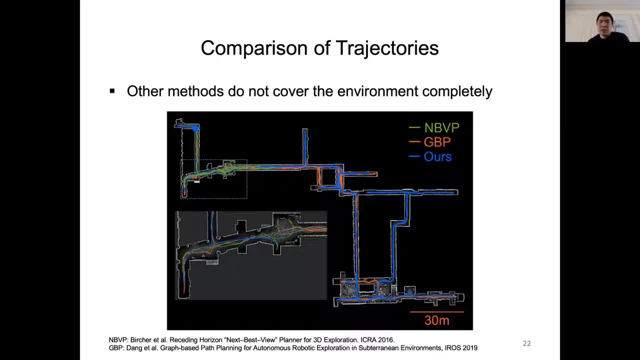 but the way that it does this is to use career steps to actively switch in between the two modules. The vehicle has to either be exploring or be relocating. It has to be explicitly in either one of them. Now our framework is made in this way that the relocation process basically 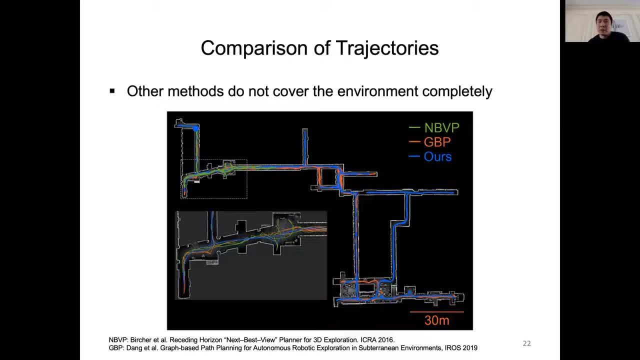 is a degenerate case of the nominal exploration. When the local planning problem degenerates, it starts the relocation and there is no heuristic to actively switch in between modules. So if you look at this result, ours, which is in blue, covers the whole environment. 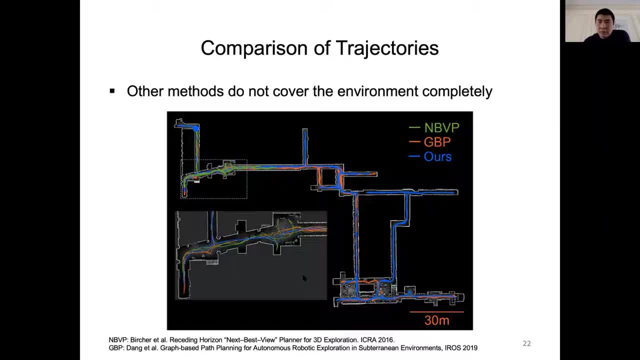 but the other two mess some areas Like this area on the global map. they're messed by both the other two methods And if you look at this zoom in picture in picture, and if you look at the green trajectory and the orange trajectory, you see some back and forth motion in there which limits the 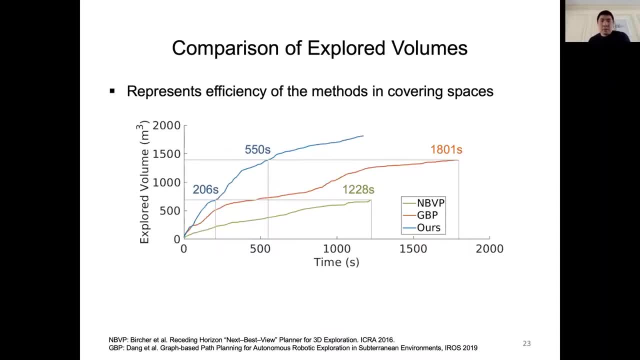 efficiency of the exploration. So here is a comparison of the exploration efficiency as the volume explored with respect to time, because the other two mess didn't explore the whole area. We basically take the amount of volume from their coverage at the end of their run. 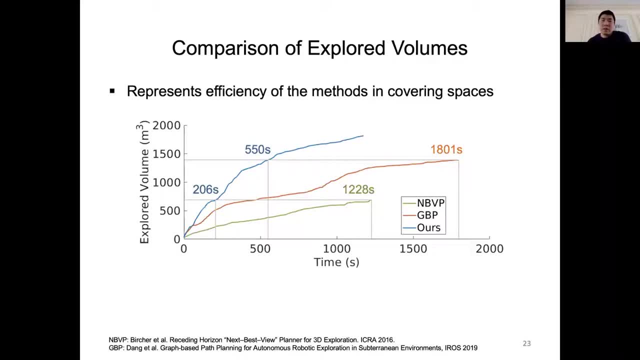 and we compare to our profile. So even though they can take different paths, the volume can be from different areas in the environment- We basically just compare the volume. That's how we do it And for the MBVP method it takes about 12, 28 seconds to. 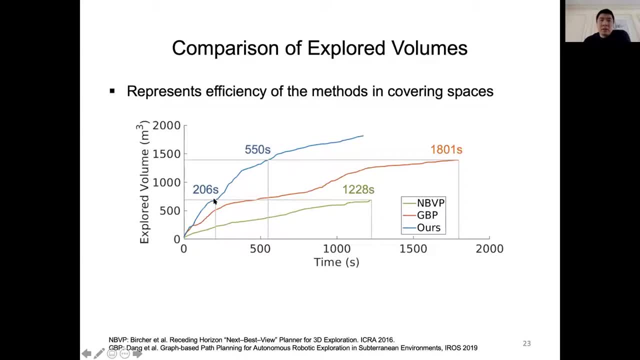 cover the amount of volume that we covered in 206 seconds, And for the GBV method it takes 18.01 seconds to explore the volume that we exploring for 50 seconds. So in both cases we are a couple more times efficient. Okay, Then here is the comparison of the run time. 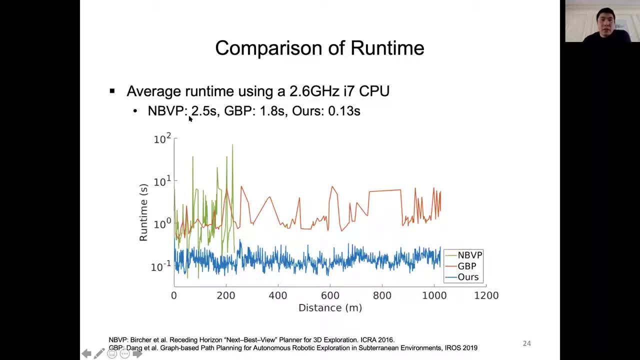 If you look at the MBVP method, the average run time for the algorithm to compute a path is 2.5 seconds. The GBV method is 1.8 seconds. Ours is much faster- It's the order of magnitude faster, because we use this efficient data structure in the global scale to seriously. 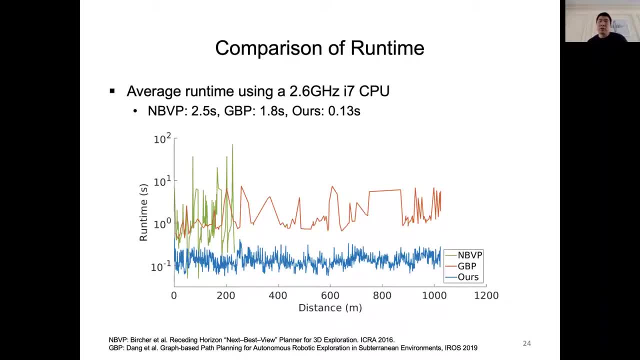 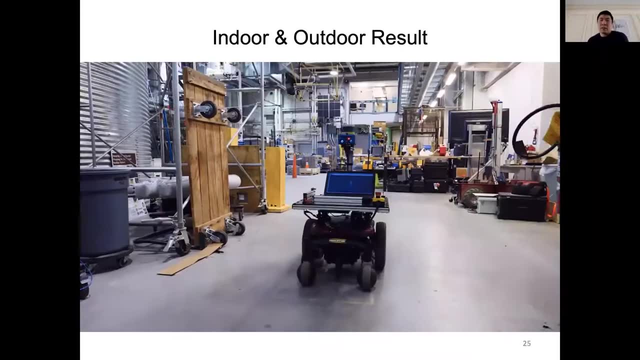 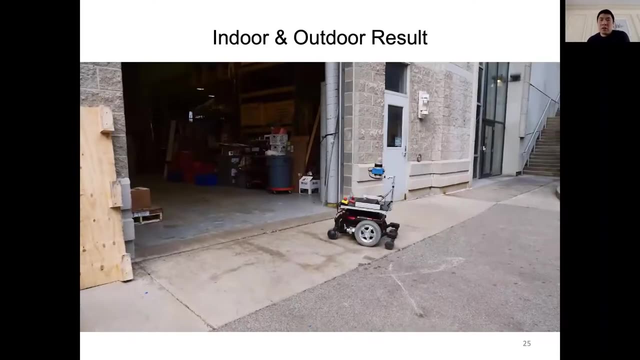 turn down the resolution at the global scale and trial for computational efficiency, And that really helps. OK, Here is another result from indoor and outdoor environments. It starts from indoor environment, which is a high bay near a building. Now it's exploring this outdoor space, which is over a very 3D terrain. If you notice the area, it's looks a lot. like a해서 simulator. you know, It's kind of like a big depression That and it looks like it's a very large knoll by pressure. but it's actually because when you switch to a surfaces if you don't pick a expositionוא. 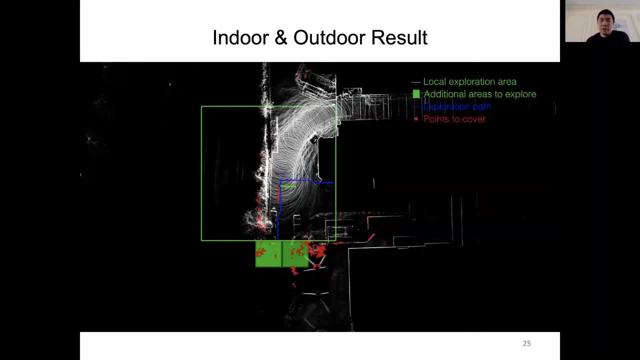 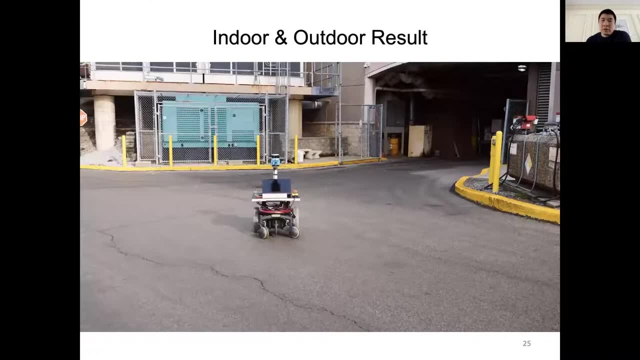 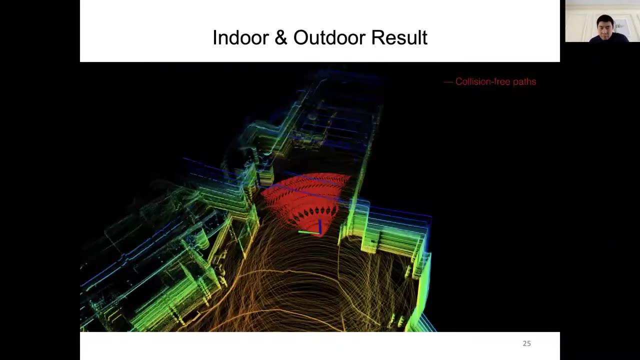 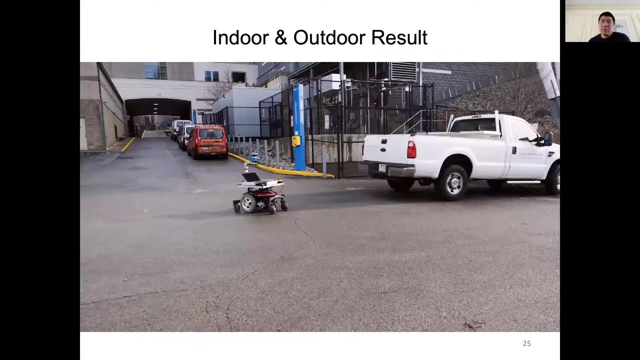 will happen. the spectra, everything goes. area is on slope, So the vehicle is going to the bottom of that area and it will go up to the top of the area. So an environment like this, it's an interesting environment. It has a big 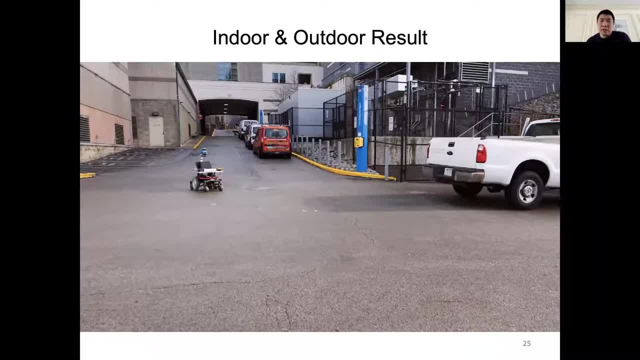 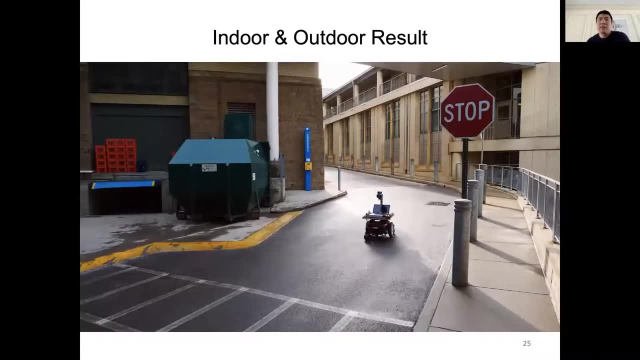 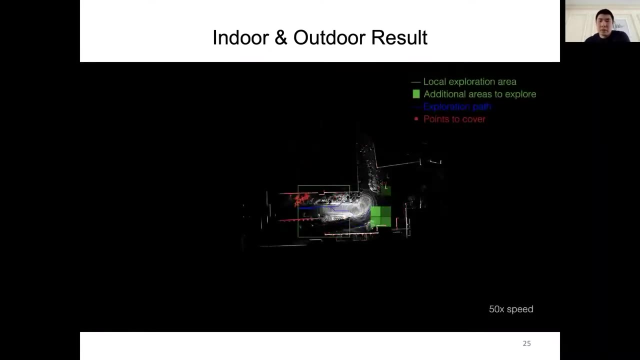 intersection in the middle and a few branches connected to the intersection into different directions. So this is the environment that we can really see how the exploration versus relocation works. So this is the overall exploration process, right, This area where these little green blocks are, that's the intersection area and a few branches are. 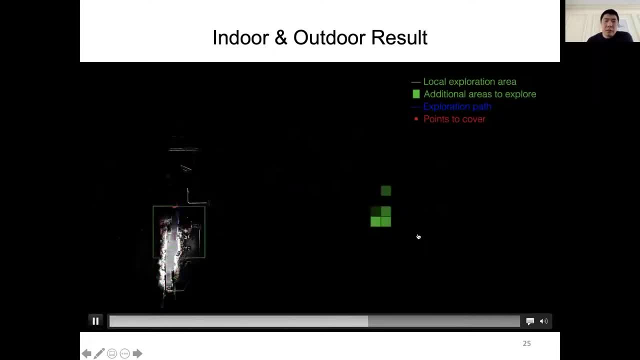 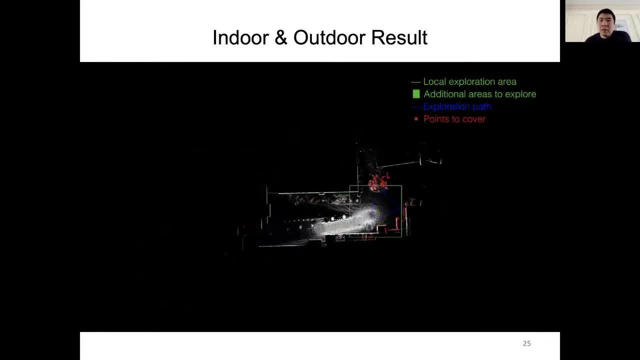 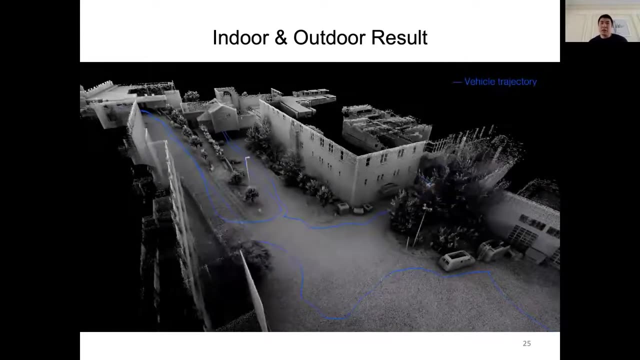 connected through that area. So right now the vehicle is exploring to the left, now it's down, it's relocating back to the intersection, now it's exploring another branch and relocating back, and now it's exploring to the right side. Actually it's a little fast, but you can see how it relocates. 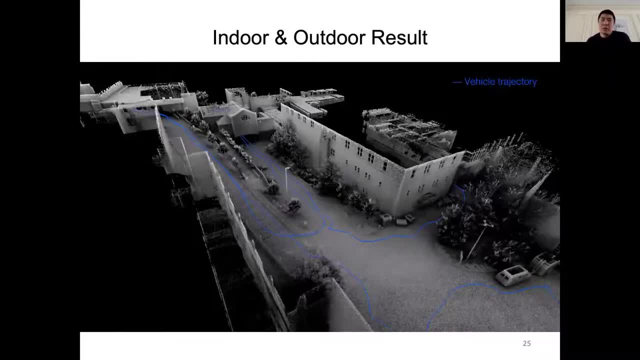 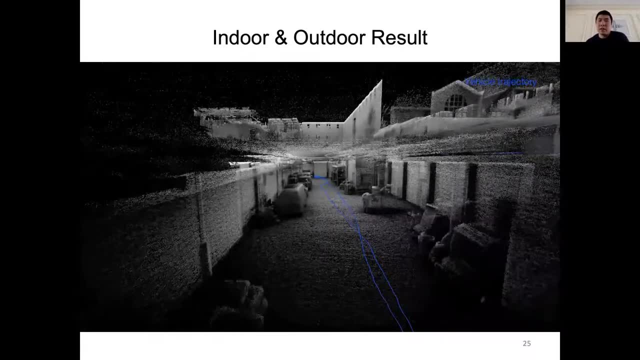 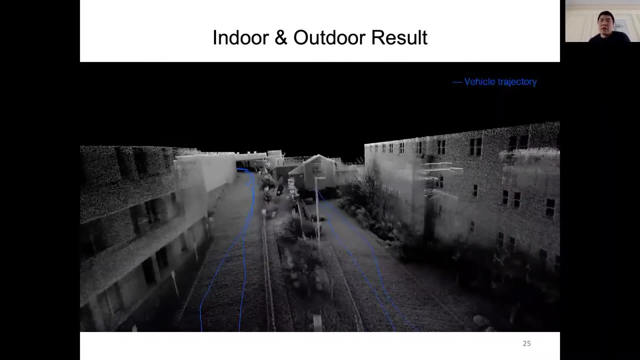 itself back into force, back to the intersection, because there are these little green blocks and you just go back there and once it gets there, it starts exploring again into other branches. okay, So here is the overall map build through the exploration run We run online. 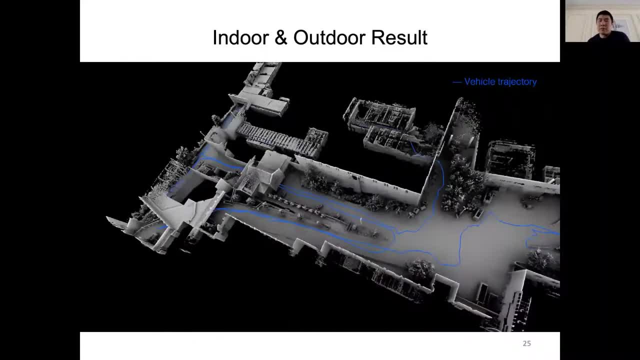 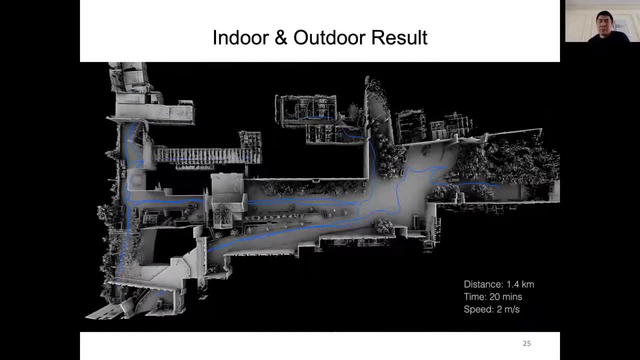 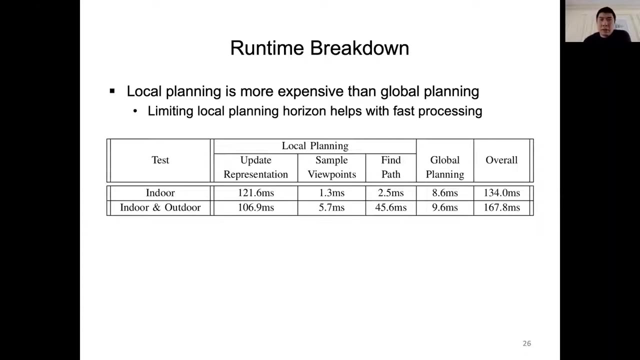 SLAM algorithm to develop the map. there's no post-processing. Overall, the traverse is about 1.4 kilometers and over 20 minutes. okay, Here is runtime breakdown. We want to look at this local planning time as a whole. basically these through. 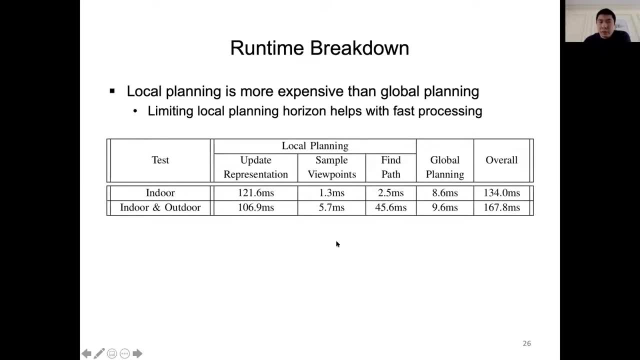 these three columns together and if we look at the numbers here, these numbers are much larger than the global planning time. okay, The local planning time together is more than an order of magnitude than the global planning time because, as we said, the data efficient. 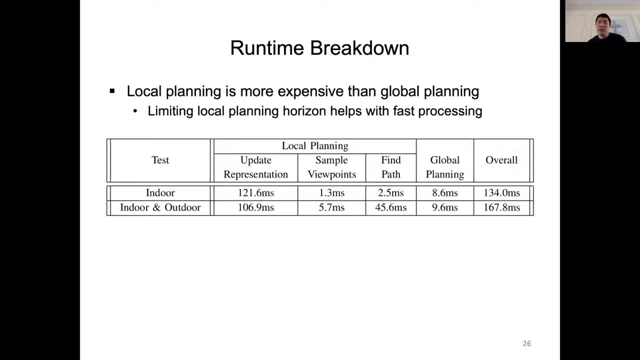 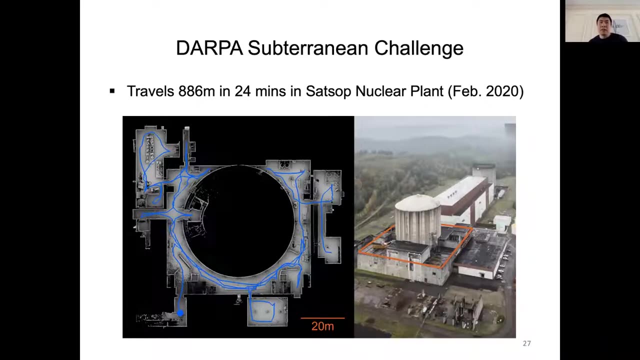 representation as a global scale, seriously turns down the resolution and trade it off for computational speed. okay, So this is a proof of that. So the last result is from DARPA Subterranean Challenge The CMU team is teaming up with. 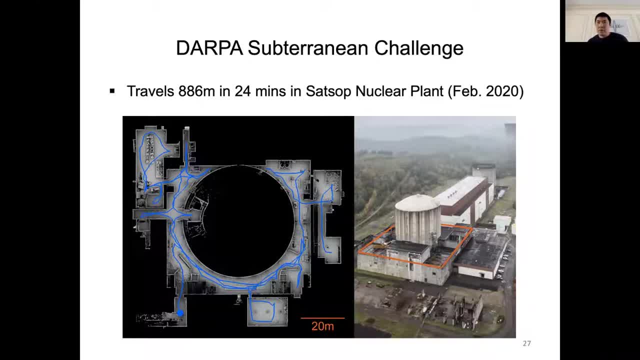 the University of Washington. Anyway, the CMU team is attending in the DARPA Subterranean Challenge and this is the result from the February of last year, which is what we call the urban circuit. It happened in an unused nuclear plant in Washington state and our system explored. 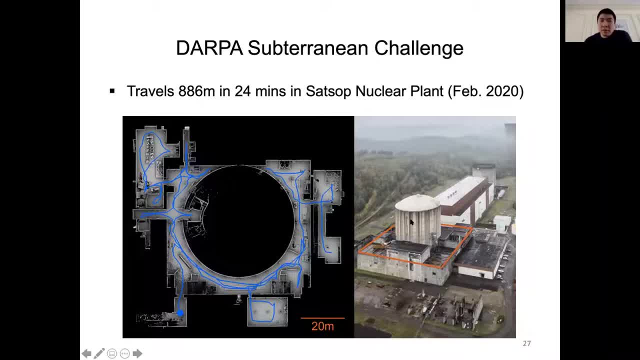 that whole floor. If you look at this square, that's where this whole floor is, and this is really a competition round, so nobody is allowed to enter the space. Only robots are allowed to enter the space, and for this particular round it's fully autonomous. 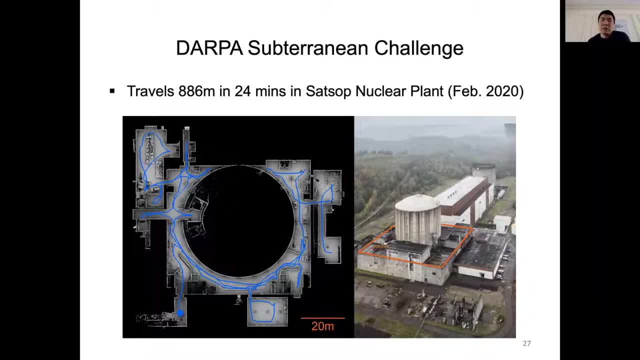 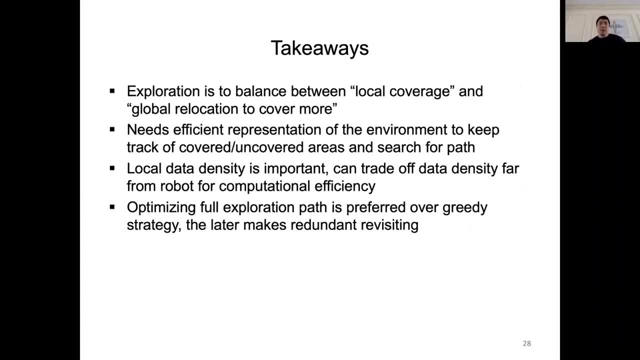 We let it explore all by itself and they covered this whole environment in 886 meters in 24 minutes. okay, So a few takes away before we finish up the talk. Exploration: to our understanding, it's a balance between local coverage and the global relocation to cover more, because the real 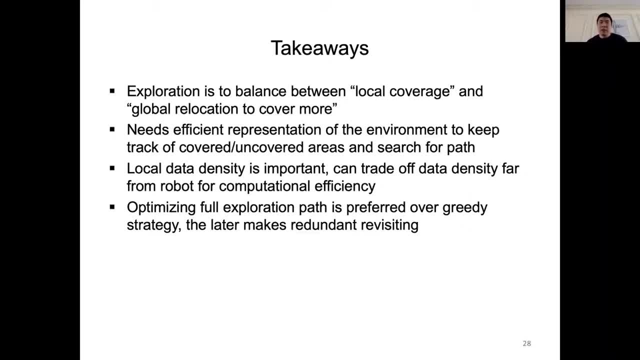 environment is often convoluted with intersections, It's hard to cover it in one shot. As the vehicle moves along, it covers everything. That is usually not the case. It has to leave these areas behind and it has to memorize them so that it relocates itself back to cover more in those areas. 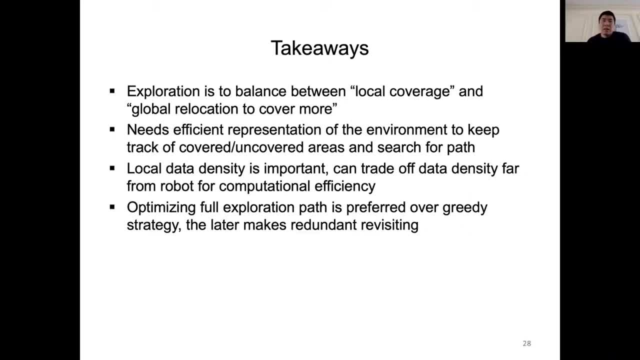 That's usually where the what the reality is. Having an efficient representation of the environment helps, because this whole exploration process has to constantly update the representation, search the representation for the past. Being able to efficiently do these two things- to update the representation and to update the past- helps with the exploration efficiency okay. 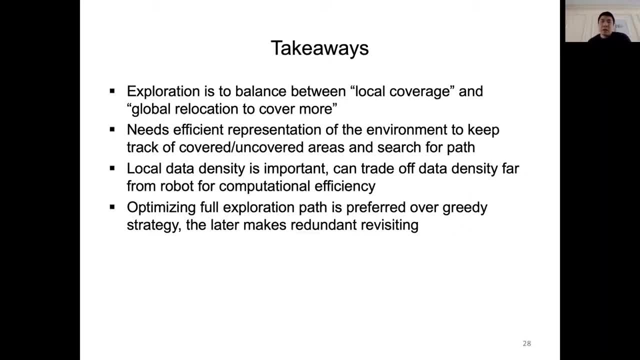 Having dense data and a detailed path close to the vehicle, in the vicinity of the vehicle, helps not just for exploration, It helps to almost all the navigation problems. but when it is far from the vehicle, in the global scale, for example, it may not be necessary to maintain the data at that. 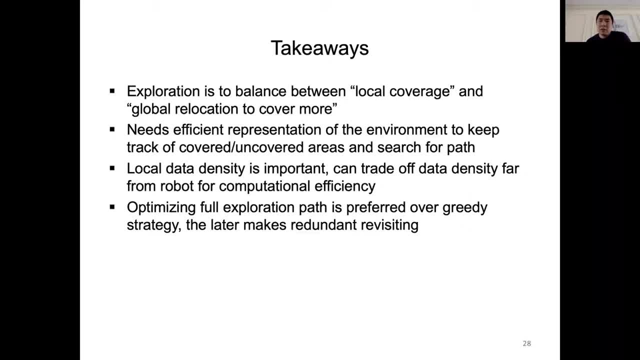 density. There is a possibility to turn down the data density to use an efficient representation and trade off the data density for competition efficiency. okay, Optimizing the full path is always preferred over greedy strategy On exploration. the greedy strategy often gives us this back and forth motion and redundant revisiting. 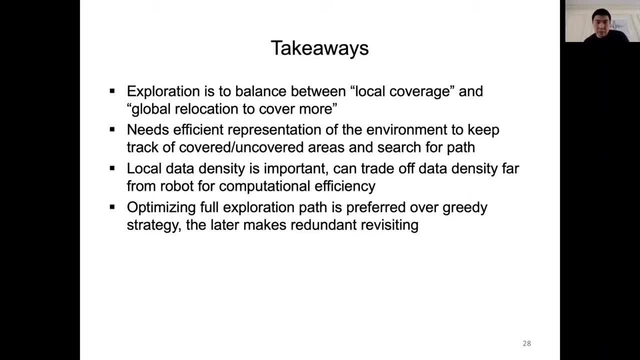 which limits the efficiency of the exploration. The greedy strategy is my op-ed. If we can optimize the full path, we always prefer to optimize the full path. okay, So this is getting to the end of the talk, but before we finish up, I want to briefly introduce our open source website. 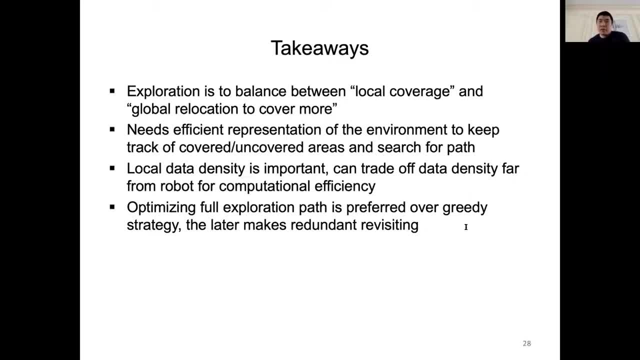 So our algorithms are being open sourced- not completely yet. It still takes us a couple more months to open source everything, especially these exploration algorithms, But today we have this development environment, open source, which is an environment for people to develop and to benchmark exploration algorithms, And you can use it for developing. 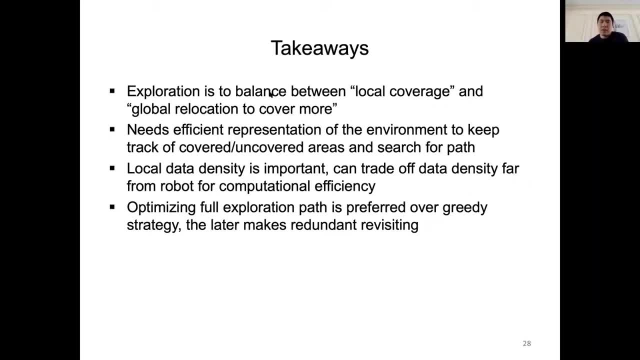 full exploration systems as well. okay, So I'll talk about that. So, if you look at this development environment itself as a simulation environment, the idea is you can use these simulation environments- this one is simul campus, by the way. you can't use these simulation environments to develop and develop. 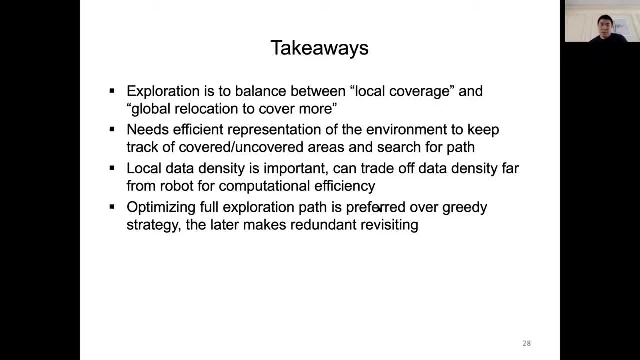 into benchmark exploration algorithms in Office, but then you can use the same repository to integrate the system around the Unreal robot. okay, So these are the five challenges, five challenging simulation environments. Each of them has some challenges And so we separated, we classify the challenges. 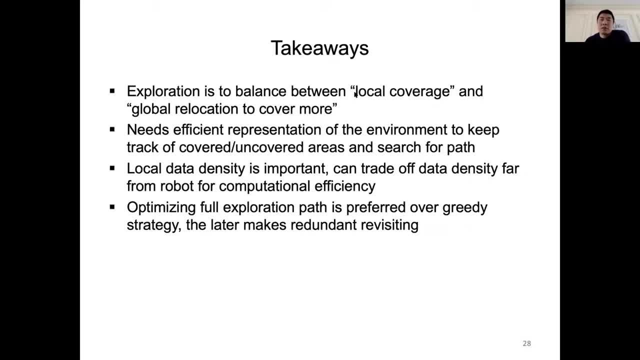 into large-scale, common-looted, multi-storage under-looting terrain, cluttered environments, scene structures, and these five environments all have their own difficulties in them. okay, Then, this repository has a few basic navigation modules, from clear avoidance to terrain analysis. 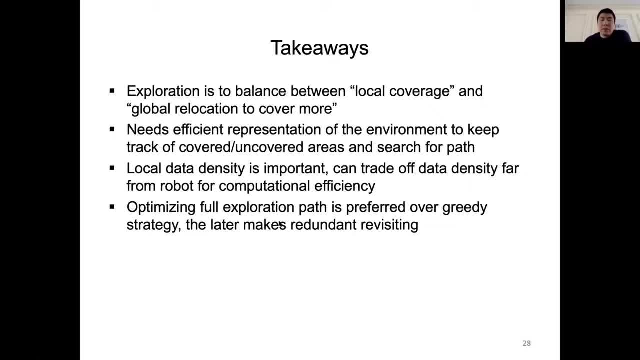 What we're seeing here is the local planner output. The local planner in our system is for clear avoidance. These yellow passes are the clear free passes. And here are the terrain analysis output: Green is traversable, red is non-traversable. So and here are some visualization tools. okay. 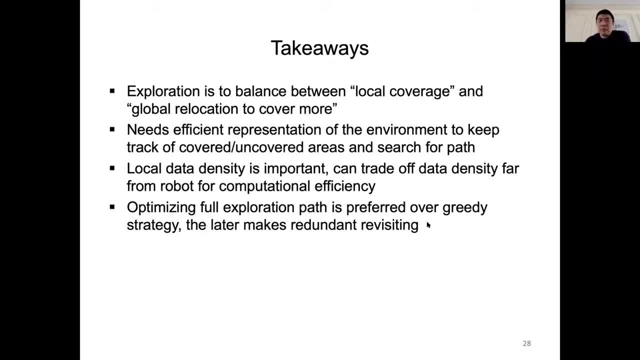 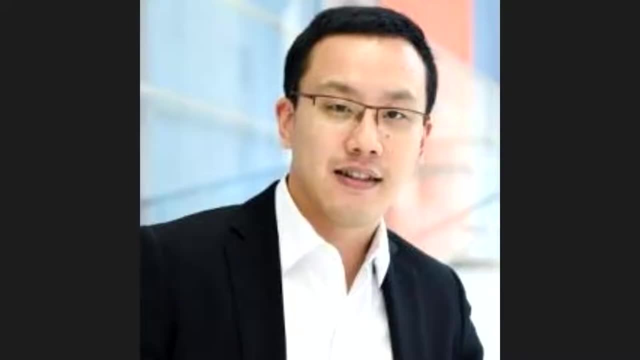 So if you look at the system diagram, this repository- Sorry to interrupt, I'm not seeing the, I'm just seeing your takeaway slide. if you're showing the video, Yeah, same here, I think-. Okay, sorry. Okay, I have to go back to the top then. 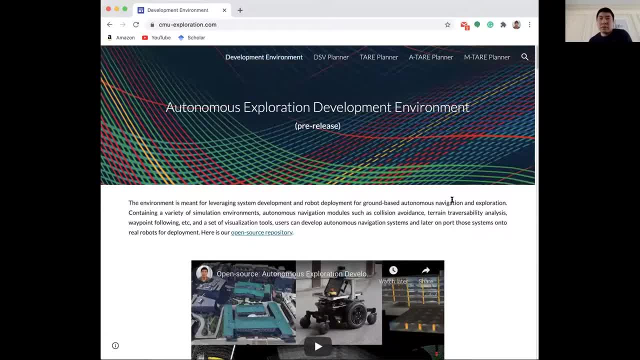 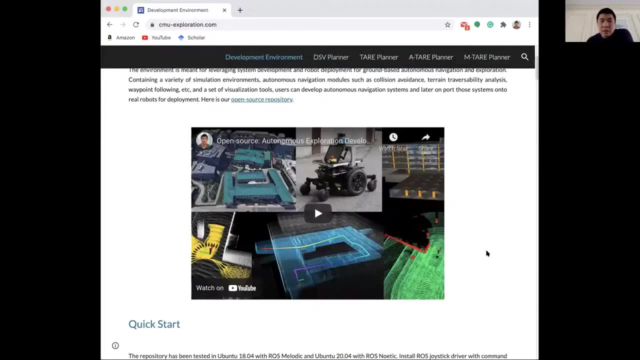 So here is our open source website. We are still in the process of open sourcing all of the algorithm, but this development environment is there. These two, these are few- still need some more time. So here are the environments. There are five challenging environments. 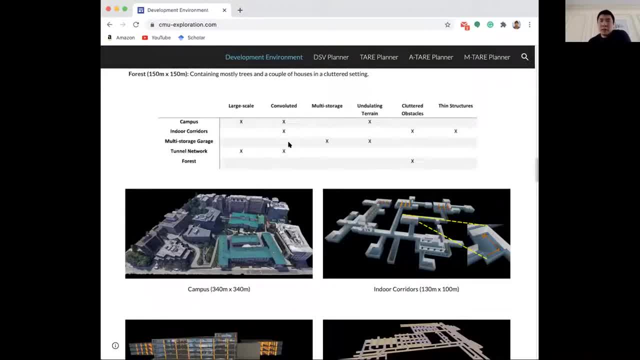 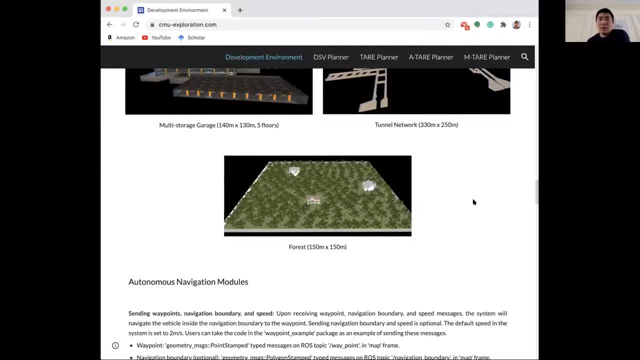 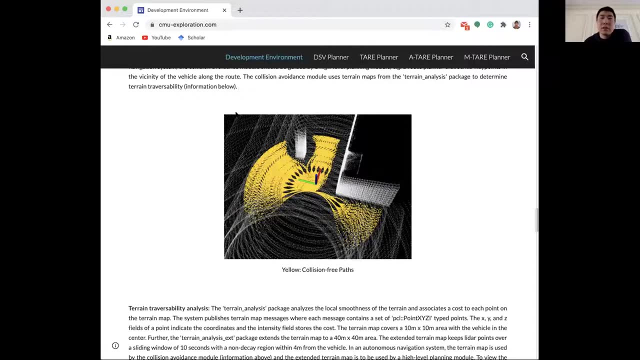 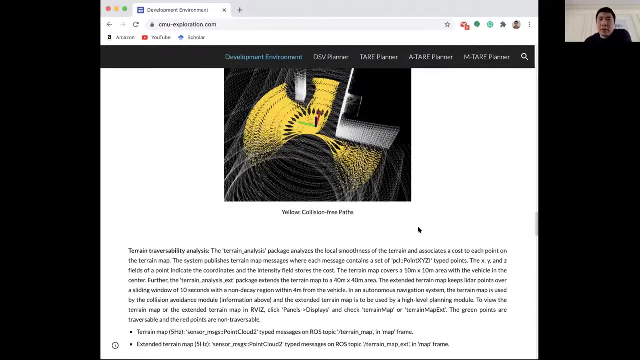 and here are the challenges that we put in the design of these environments. So this repository has some basic navigation modules. This is local clear avoidance. The yellow passes are the clear free passes going around obstacles. These white points are the obstacles. The green is analysis output. green is traversable. 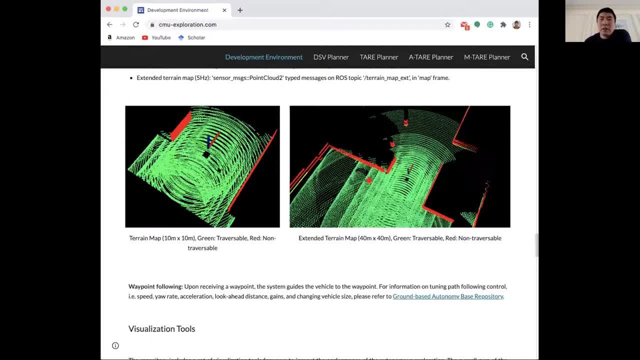 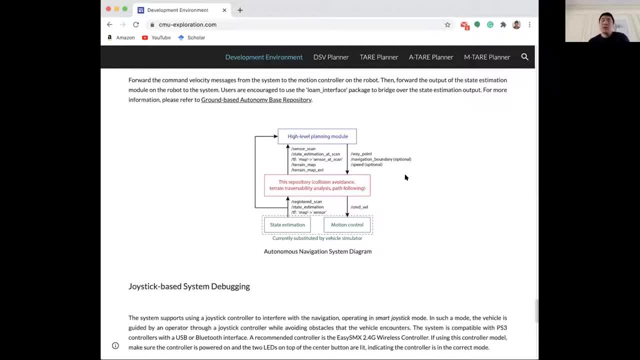 red is non-traversable. So if you and it has some visualization tools, okay. So if you look at the system diagram, this repository or this system is basically mid-layer in a full robot navigation system. You can use that to develop navigation algorithm. 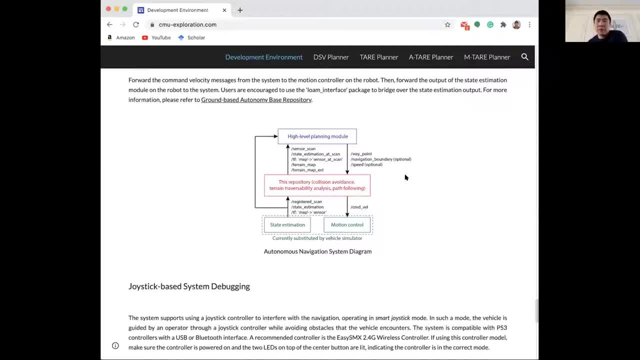 especially exploration algorithm and you can benchmark the simulation. but if you use this repository to integrate full navigation system, this will be the mid-layer in the system. It connects to the bottom layer, which is state estimation motor controller, and the upper layer, the top layer. 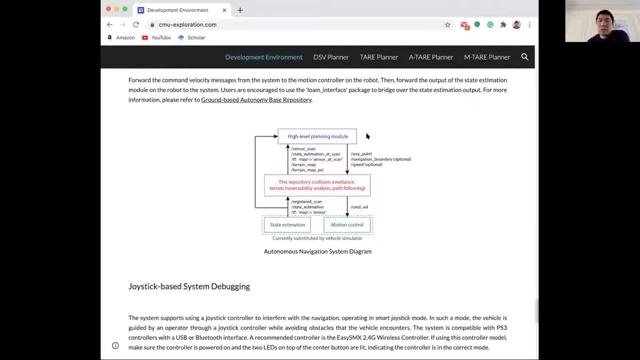 is the high-level planning algorithm. So this is really to help people to develop the high-level planning algorithm. If you don't work on exploration but you develop other high-level planning algorithms, that's the same. You place it here and you interface with the mid-layer. 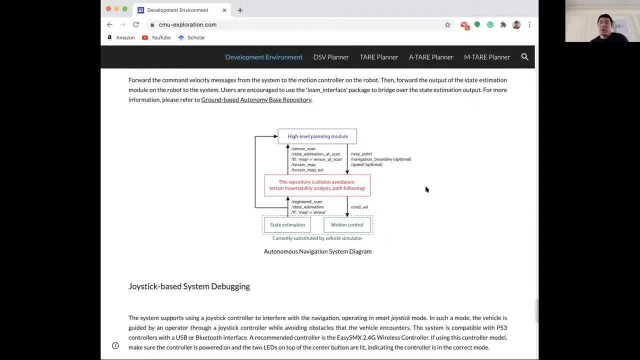 and the mid-layer has all the interfaces to the upper layer and to the bottom layer to take the state estimation and to control the vehicle. Basically, if you send a waypoint to the middle layer, it will take care of it. It will bring the vehicle to that point, okay. 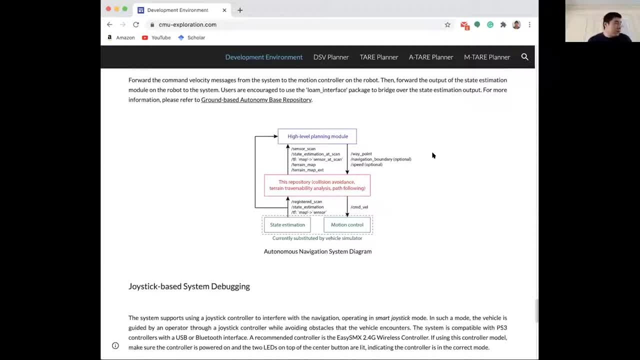 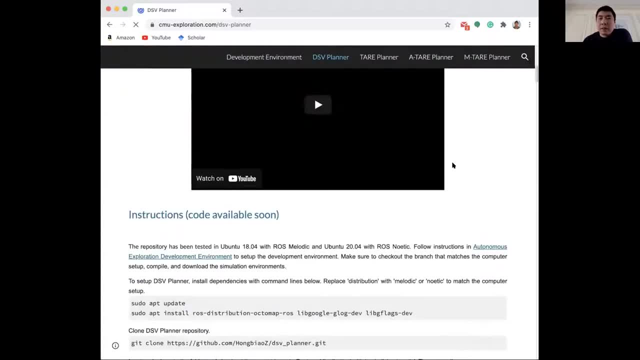 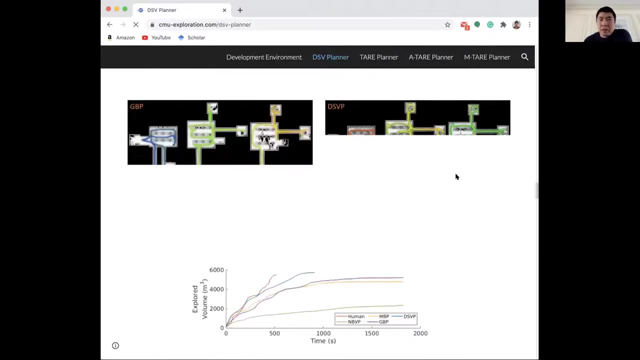 So, but what I want to quickly mention here is another point, because we have a lot of time As we benchmark in this simulation environment, and while we benchmark, we also ask a person, we ask a human operator, to drive through the environment. 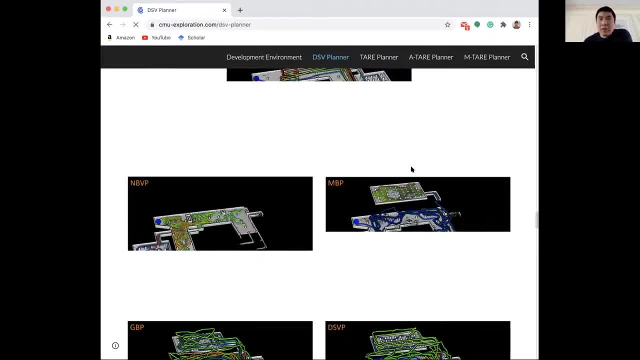 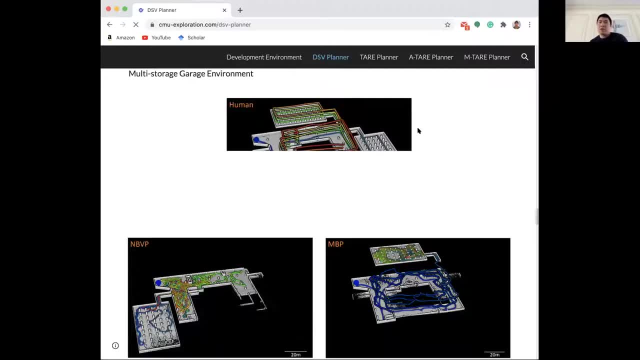 Okay, so these are the results. This is a human drive through about 10 rounds through the same environment, So this path is not theoretically the best, but almost the best. We really cannot make it better ourselves as human driving. Okay, If you look at the path, it looks very neat. 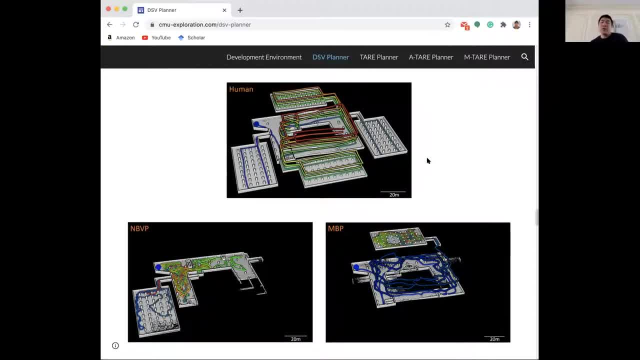 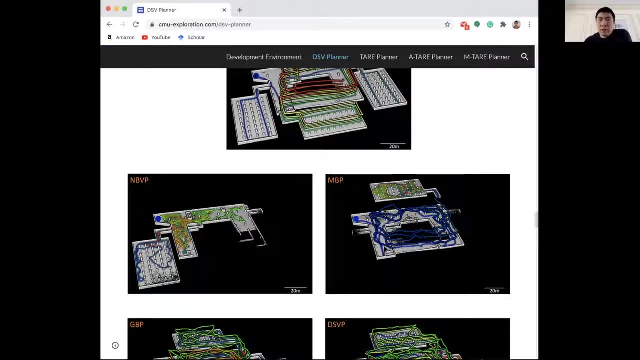 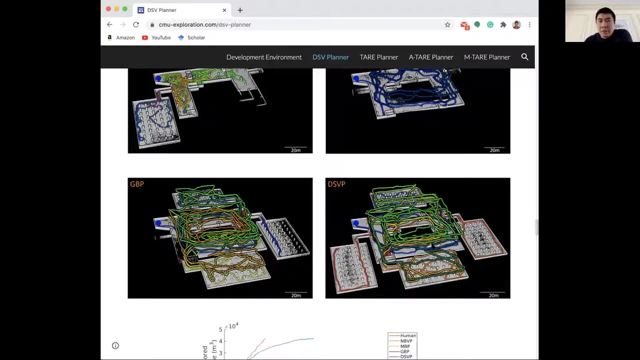 and you don't feel that you can do much better from there. Okay, The current state of the art algorithm are not doing very well. We don't have to pay too much attention to them, but this is our result, which is still irregular compared to the human result. 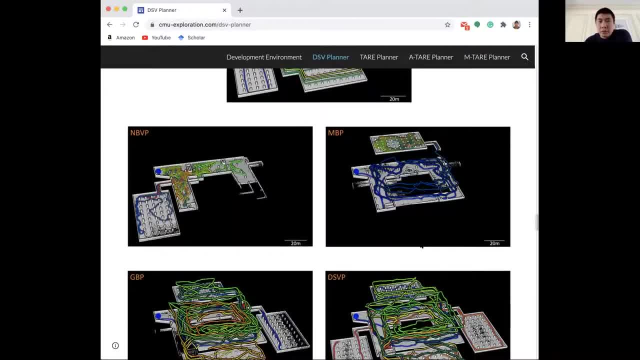 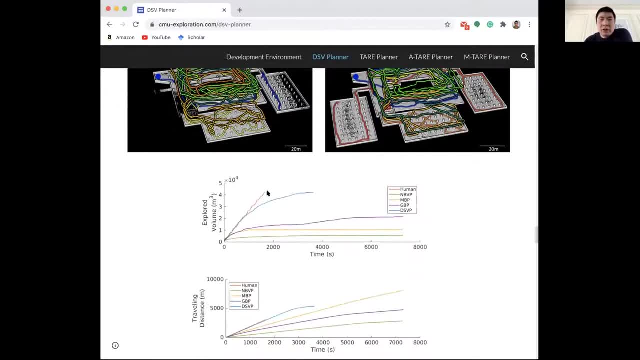 which is here It looks much better. And if you look more carefully, it still has some redundant revisiting. okay, And if you look at the efficiency comparison, the human drive is still much better, especially at the second half. If you look at the first half. 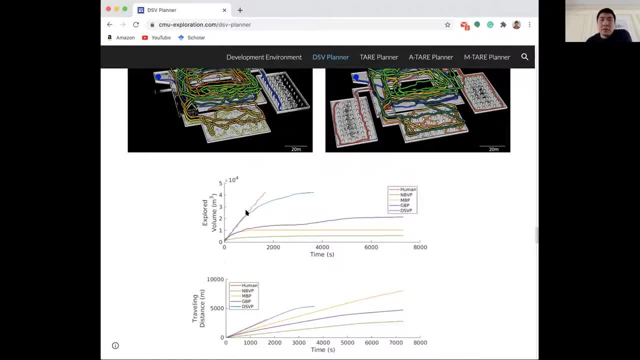 our algorithm is doing almost at the same level, or sometimes even better than the human drive, But in the second half the efficiency drops because it's still not as efficient to use the global picture And, by the way, it does not have the global picture. 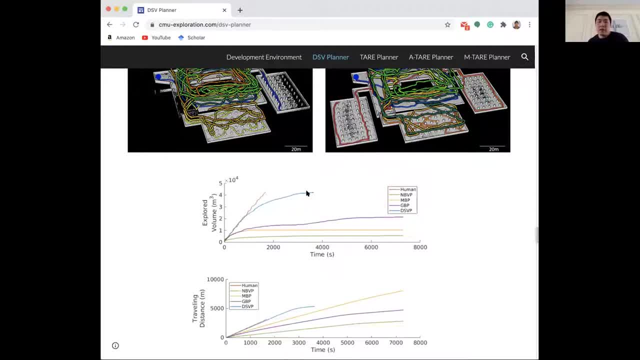 because it has to. it has to explore, to gradually figure out the layout. Now the human drive. it's practiced through 10 rounds. It basically knows everything about the environment. So this triggers us to think what we can do further to maximally bring this blue result. 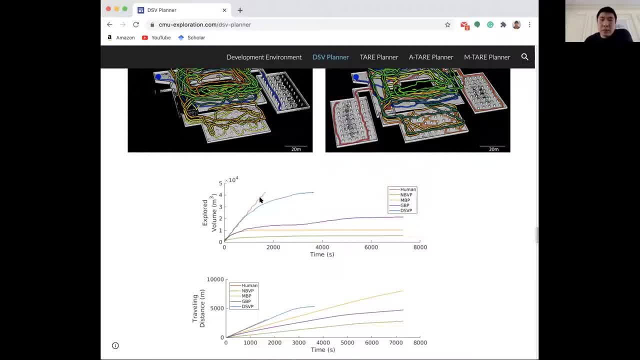 this blue curve to the left side to approach this red one which is the human drive. We won't get exactly there, That's not possible, probably, but we want to bring this blue path, this blue curve, as much as possible to the left side. 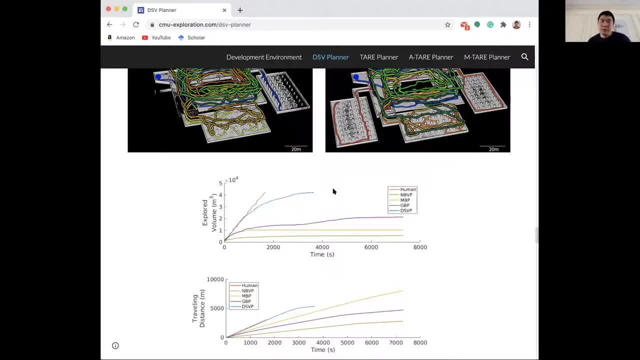 And there are some discussions at CMU with Gino, who is the organizer of the workshop. So we are trying to actively leverage experience and prior, to predict the uncovered or the unseen areas in the environment. Right now our algorithm only uses what has seen so far. 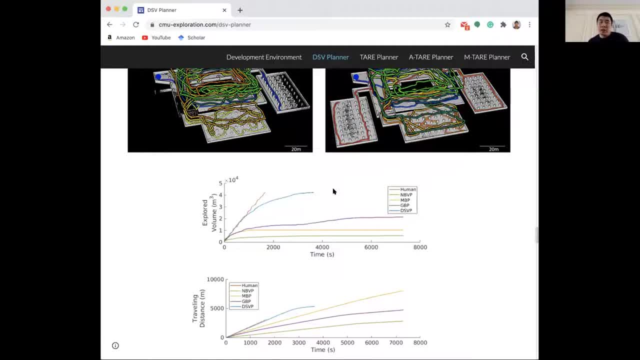 and it's using it quite efficiently And it's using it quite efficiently And it's using it quite efficiently. But for the parts that has not been seen, we don't know anything about it yet, but there is still a chance that you can predict something. 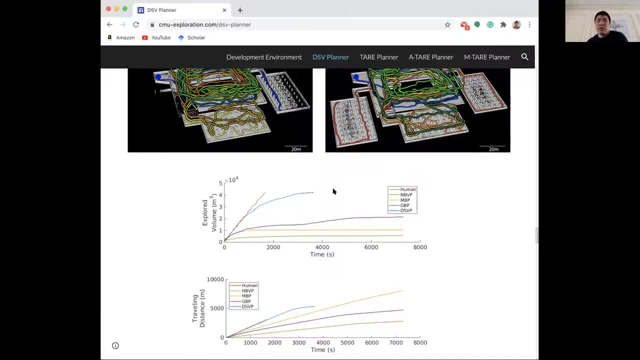 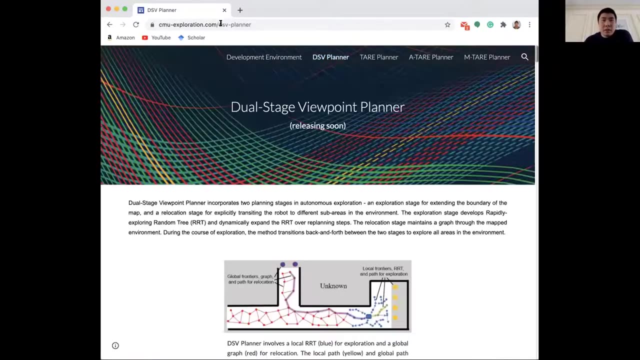 It won't be exactly accurate, but it's still helpful And by doing that we can probably bring this blue path slightly to the left, a little bit, Okay. So that's the end of the talk. Let me share this website and I can answer questions. 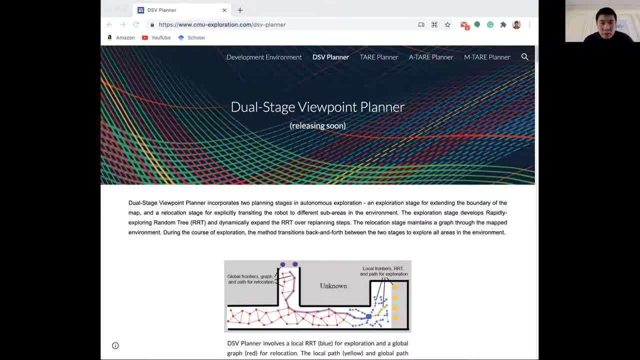 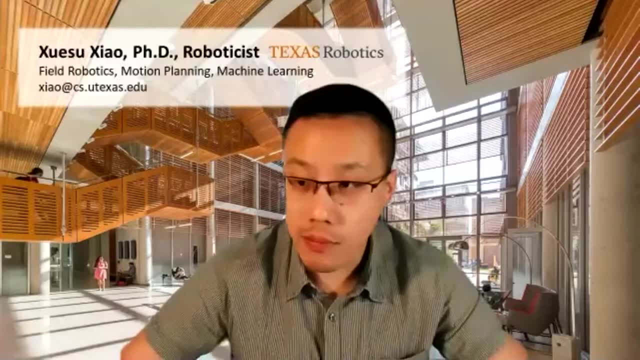 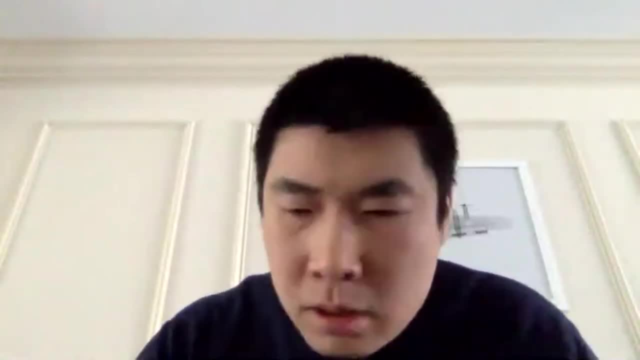 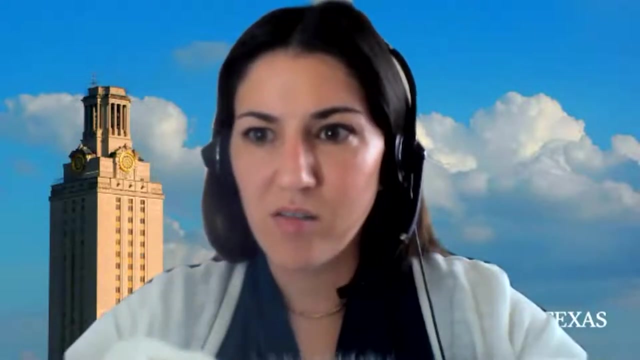 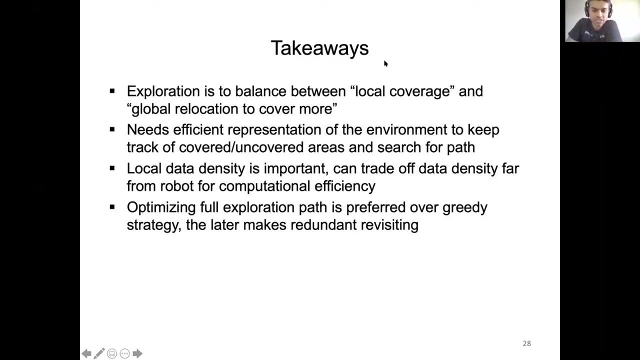 Thank you, Gi. Do we have any questions? I'll share the screen again. Let me send the link. We have Sure you are Any questions? Yeah, Thank you so much for your talk. I have two questions, interrelated questions. uh, with your local repositioning, when you reposition the robot back? 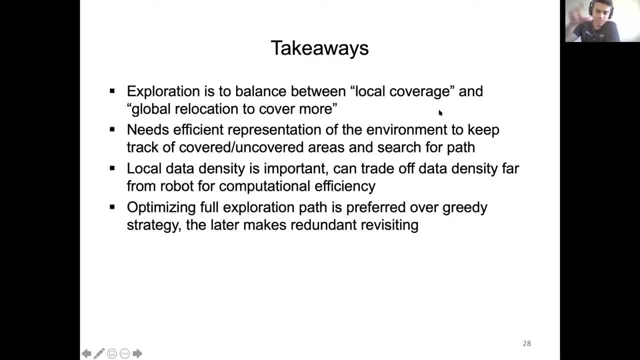 first, when you reposition or back, do you or are you also online re-planning to avoid any obstacles? and secondly, how much your solution relies on consistency of your slam solution. so if there is some drift while you reposition from one part, another part, uh, there can be some drift and how much it affects your solution. 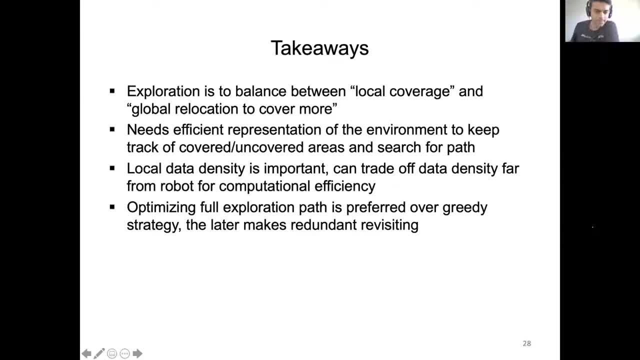 okay, okay, let me answer the second question. i was not exactly clear about the first question, so i need some more explore, more, more of explanation. so the second question: how much does it rely on the slam? uh, so we have the simulation environments. if you're testing the five simulation environments that there's no, there's no effect, basically. but in reality, 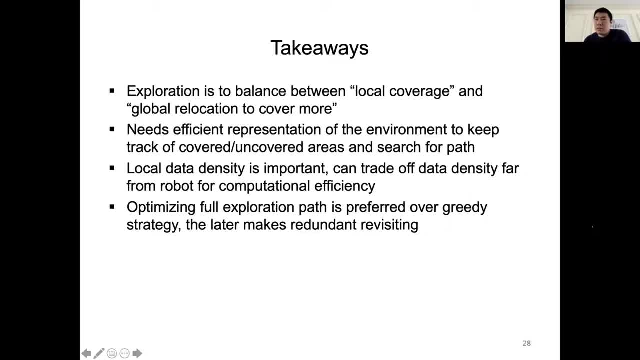 what we have seen is that because we are using the sparse little green block, the sparse representation, that really helps, because if there is a little bit of drift, um, the green, the, the, the sparse representation basically smooths it out. okay, so because you don't care about that much. 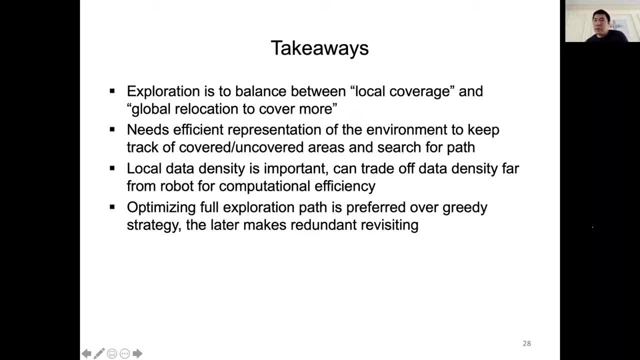 details. as long as that whole area is covered, that's fine. you don't have to cover that another time. if you use a traditional frontiers where you see something slightly shifted, you think that's new and you want to. you want to cover it one more time, right, but there is a there. there is an exception. 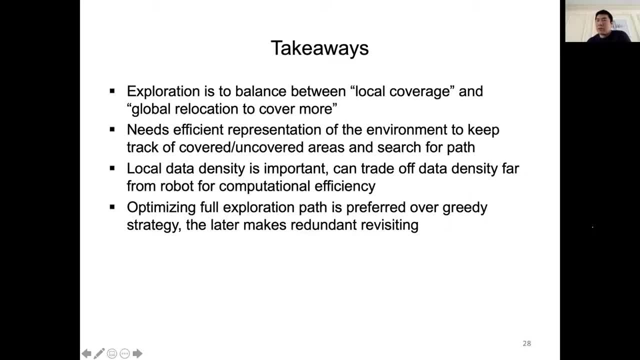 which is, if you go and when you come back, the drift will cross the boundary of the representation. basically, you drift from one block to another block. so that needs some additional work. from software engineering's perspective, we think it's. it's solvable, okay. so, um, for your first question, can you explain a little bit more what the question is? yeah, so when you're 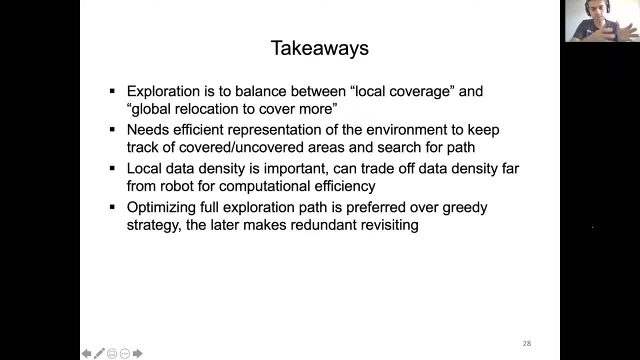 coming back, like you're coming back to one of these green blocks over a long period of time. uh, are you continuously re-planning while you're coming back? so, for example, if a new obstacle appears like, for example, that was not before when you moved forward, like a dynamic, for example? 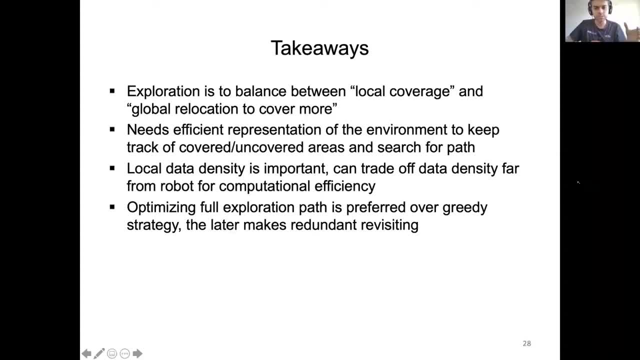 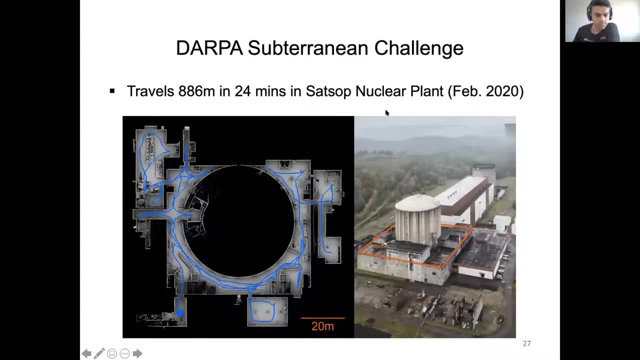 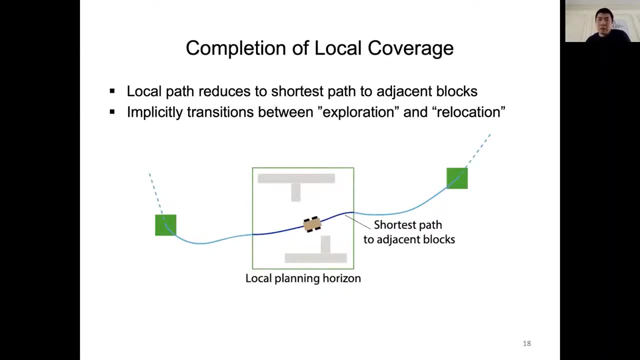 someone parked a car somewhere in your previous path, but will you re-plan around it or will you just follow the path that was set before? let me show that slide. so basically, our re-planning phenomenon, our re-planning phase, is, it's basically a degenerate. 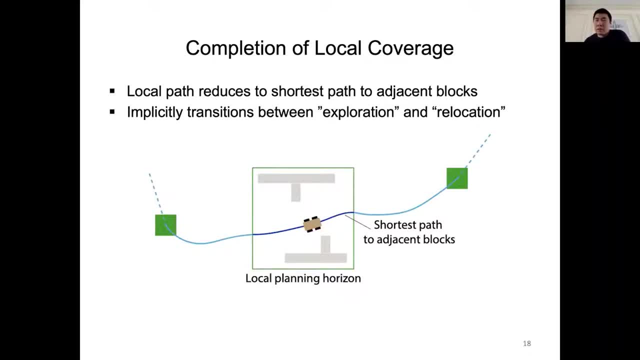 phase of the nominal exploration. so along the way, whenever it sees more structures, this local planning problem reverse back to the nominal, healthy phase and it starts to explore again. okay so, but it's a great question. if you look at the gbp method, they use the heuristics to switch in. 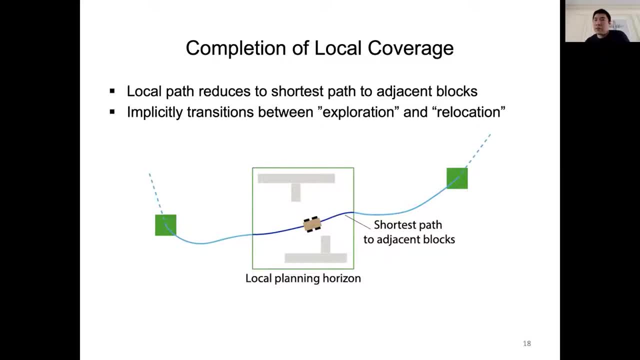 between. so it's either exploring or it's relocating. while it's relocating, it's either relocating, if you, if it actually passes some other areas that are not fully explored, it has to ignore them because it's in the relocation phase. it has, it plans the path and it has to. 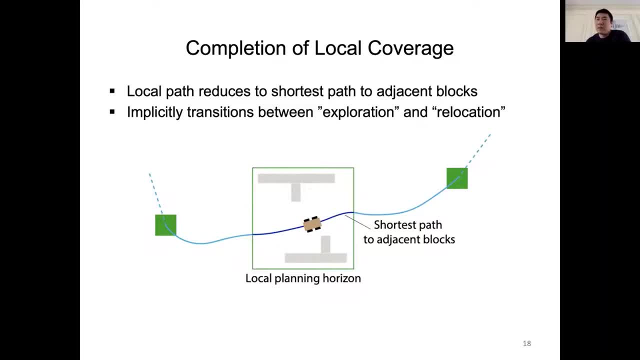 get there, the from there. from there it switches back into the exploration phase. so that method would cause cause that, that problem. so even you see some uncovered areas along the way. it misses them and it has to come back later on to cover those areas. thank you so much. 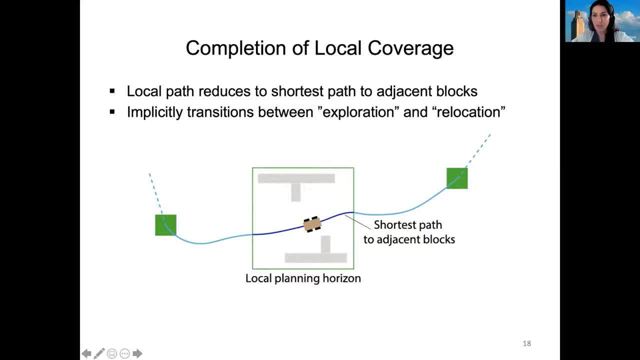 do we have additional questions? i have one, but i'll wait if someone else wants to ask first. yeah, so, hi g, thanks for the nice talk. so i'm not an expert in exploration. i'm just a little bit curious about this green blocks idea you presented. i think that's very interesting. 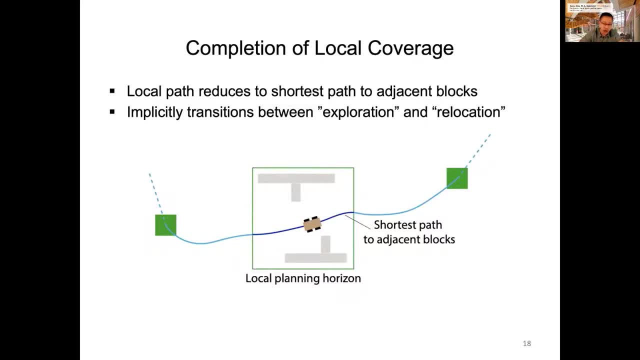 so this is kind of like the the frontier in traditional methods, right? so you know that's unexplored, you mark it down and you come back later. so, um, how does this? your methods like i would say a higher level compared to those traditional, like depth first search or breast first search. so i i see this green block, somehow it looks a little. 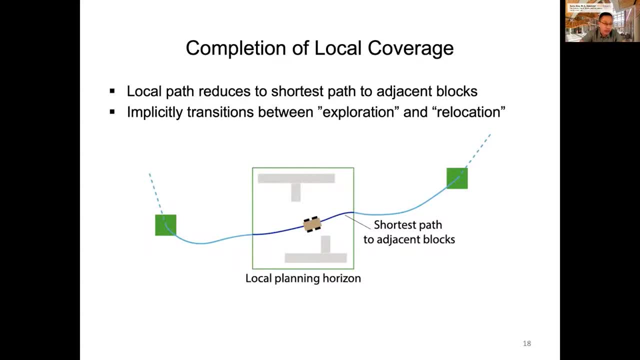 bit like: like you're doing a breadth first search, right, so can you comment on that? uh, we are, we're quite different, but okay, let me explain. if you look at the method itself, uh, from a systems perspective, it has a front side. it has a back data structure to maintain the data. 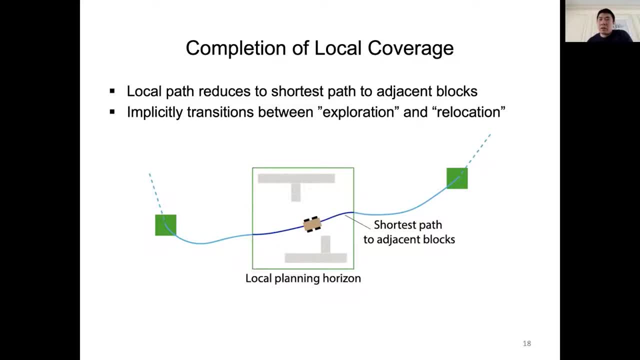 now the depth first search, or so, or or the greedy algorithm to search through the state structure. that's the, the back side, that's to determine which frontier you go to right. the front part is the front side is the frontiers. so there are difference on each side: the frontiers, that's a dense. 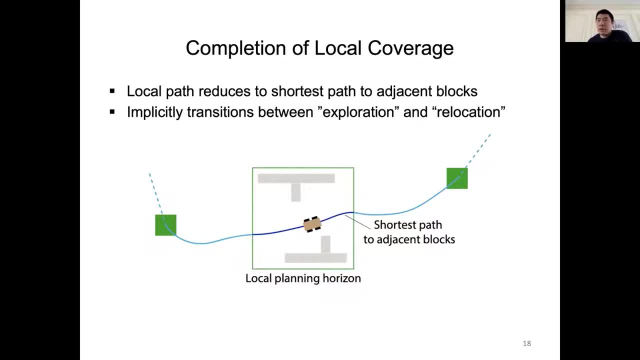 representation if you use the traditional way. it's not that it will not mark down. it will still mark down those areas and it will memorize to come back. but as the the environment gets large, today's computer has just that much resources and it's online algorithm. you have to come up with a pass fastly enough for it to go, otherwise it's. 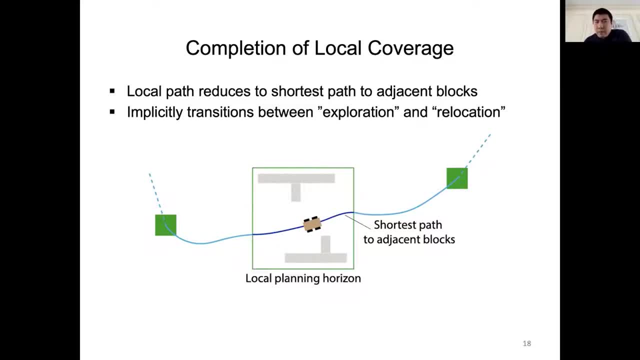 it's stopping there, it's waiting forever. so if you use the dense global representation, it's possible to do it. if you have unlimited computational resources, right. but realistically, if you do it like in our method, i use a sparse representation. it's not marking down, though, in 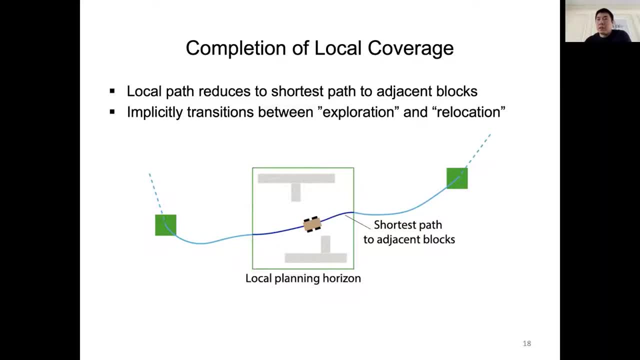 those areas with these dense frontier points, but it's using sparse block, green blocks to mark down in there, which significantly accelerates the processing. so that's, that's the difference. that's mostly for computational reasons, right, that's mostly for computational reasons, because you cannot just process all the data you collect along the way. i think, okay, right, right, that's the. 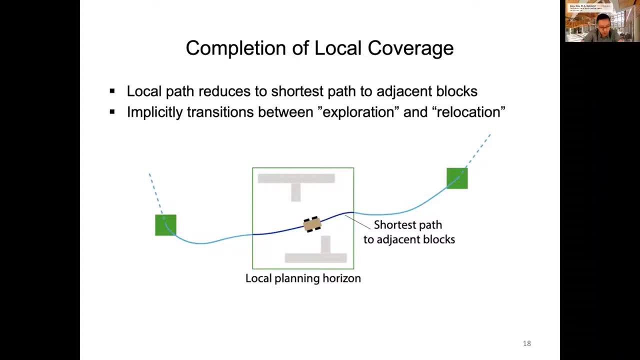 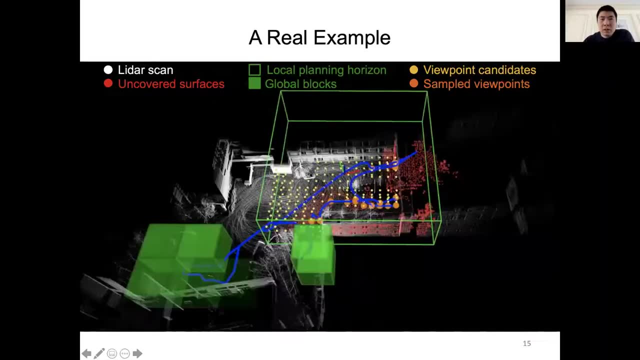 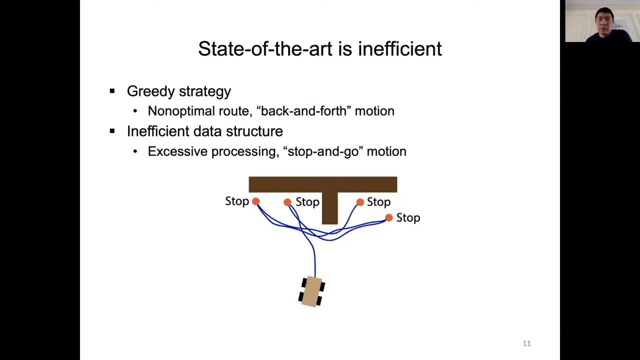 first point. then the second thing is that you need to be very precise in your data collection process. it gets to the second point. so why So? if you look at the Okay, so here, most of the existing methods, they use greedy strategy. 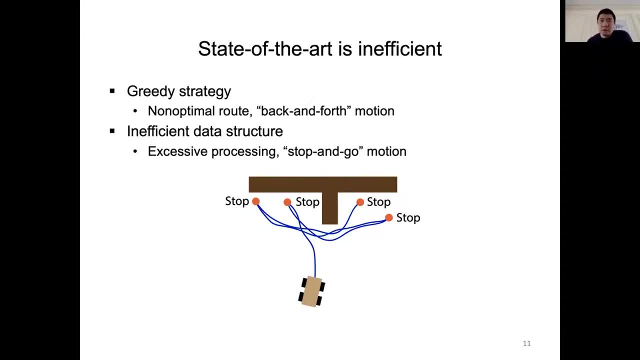 Why do they use greedy strategies? People know greedy strategies are my own paper. they can only get that far, but why do they still use it? It's not that people cannot understand. optimize the whole path is better. everybody understand it, But in reality it's a hard problem. 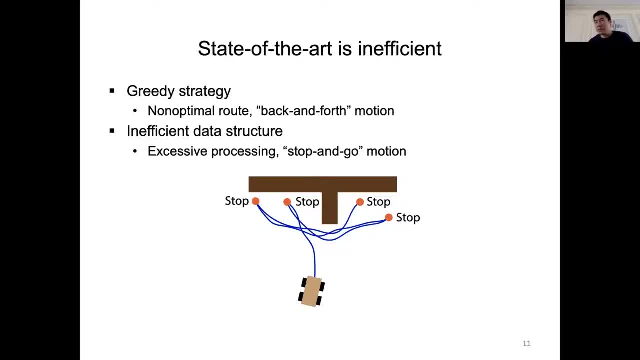 If you can't use greedy strategy, because greedy strategy it's greedy and it's faster, So it gets you something. even you cannot solve the full problem, you can still get something right. So as long as we can do that, that's good enough. 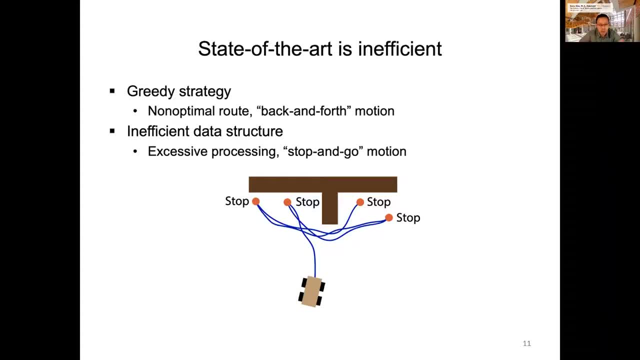 in real time onboard the vehicle. So ours is really that we have this efficient data structure that gave us a lot more computational capability, So that from there we can optimize the whole path, instead of using greedy strategy to just optimize a little bit, that little bit short path that connects to a few points. 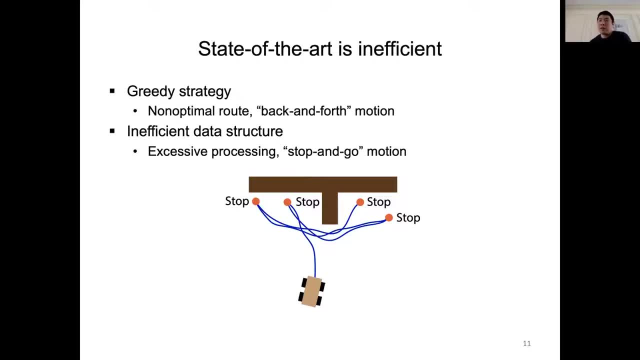 So that's the reason, that's the insight behind seeing we first have efficient data structure that gave us a lot more computational capability, So then we can optimize the full path Sounds good. yeah, I think. thank you. yeah, I have one small question regarding the local planning. 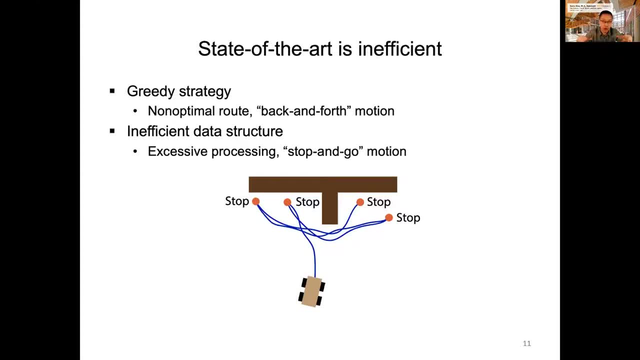 So currently so not. So I'm not sure if you're familiar with the green blocks, but within the local range you generate an evenly distributed grid of candidate viewpoints and then randomly sample among them and then plan a path to cover all of these right. 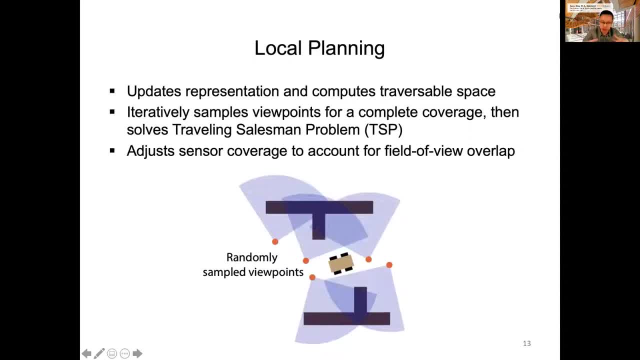 So I'm curious about: so this assumes you have omnidirectional perception, right? You are using a 360 degree LiDAR. So if, for example, you have a limited field of view, like using a depth camera, would that randomly sample procedure be affected? 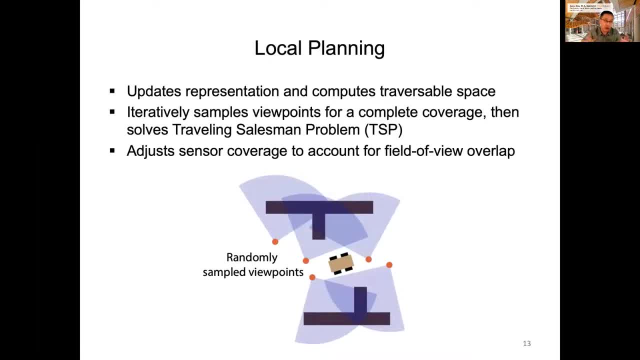 Maybe you need to carefully, but you need to be careful, carefully plan the route and also you need to plan the orientation of the vehicle to cover as many space as possible. Maybe that's like an extension of future work. I'm just curious. 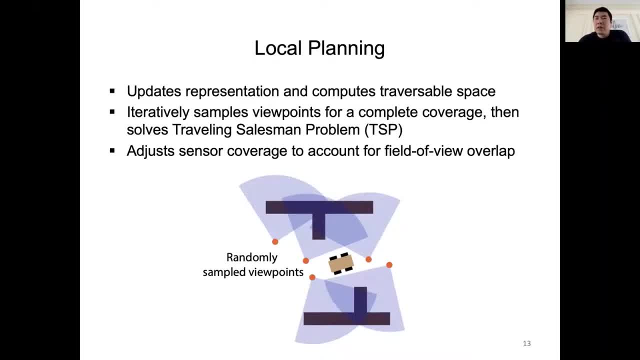 Right, exactly, It will take more computation, for sure, because you're adding one degree of freedom, which is orientation, or a few more actually. So there are ways to accelerate it, because when looking at the surface, you can mostly figure out the norm of the surface. 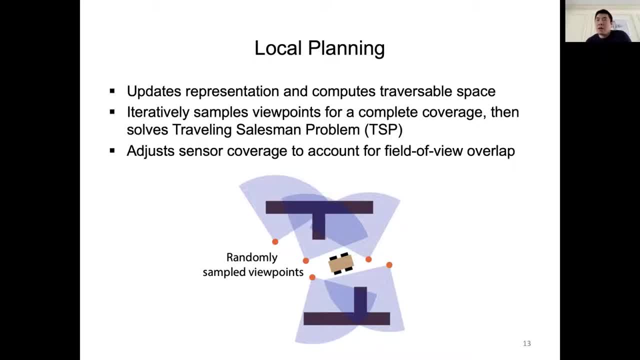 that helps constrain the orientation. By the way, if you build the system really well, the vehicle may not have to spin for the whole vehicle itself. If you put a gimbal on the vehicle, that really helps. right, You can keep it spinning all the time. 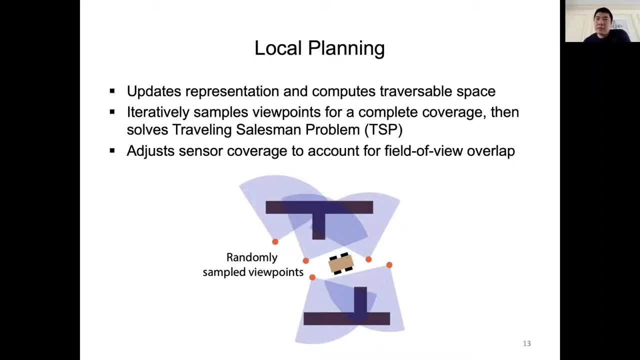 Now it becomes a 360 sensor. Okay, yeah, that makes a lot of sense. yeah, Thank you. Well, I had one short question, if possible, before we move on. Okay, So I have a question for you. I was very curious about the choice. 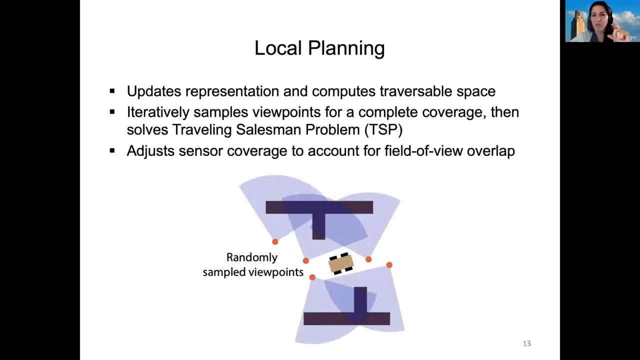 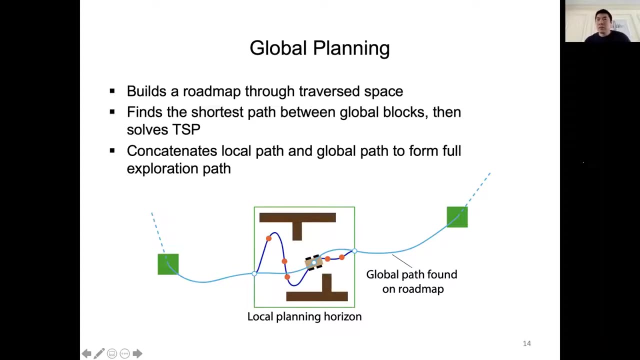 to expand specific, the sparse global blocks. How do you choose which one you will expand next? Because it seems like some of them are close by. some of them might be further away, for example, That's from the global tour. So we have all these hologram blocks. 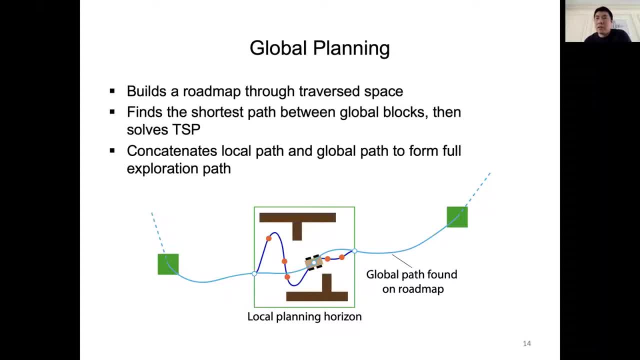 We'll compute the shorter path in between every pair of them, Then we solve this TSL. Okay, So we have all these hologram blocks. We'll compute the shorter path in between every pair of them, Then we solve this TSL. 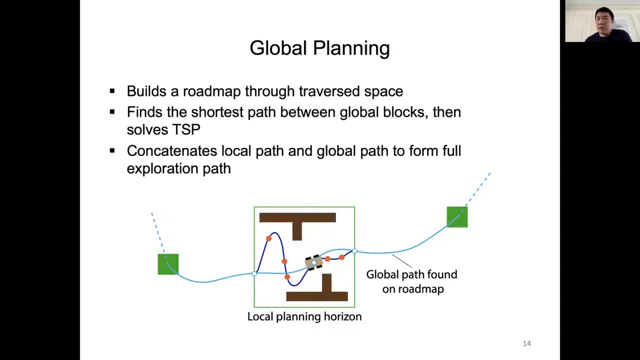 So we have all these hologram blocks. We'll compute the shorter path in between every pair of them. Then we solve this TSL, The traveling salesman problem. Which one that is the closest to us on the tour? That's the one that we go to next. 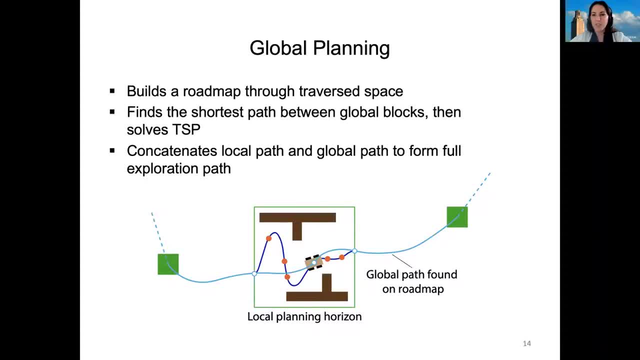 So there is no aspect of heuristically making assumptions about the benefit of expanding a specific node. It's just the shortest path. The idea is the idea is to cover all of them in the shortest time, Not to gain the maximum coverage in the limited amount of time. 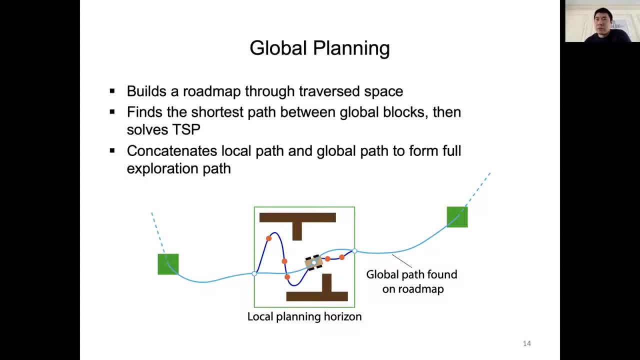 We don't care about the incident coverage. Well, while I'm saying we don't care, we are only seeing that little area from the vehicle because we're not actually predicting the places that are not seen yet. So, for what we know about, 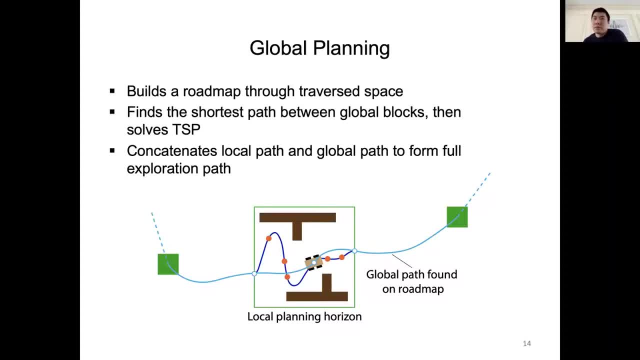 we want to cover them fully in the shortest time. Okay, That's also. you also assume the environment is closed, right, Because you assume the vehicle will come back in a certain amount of time. It can't be open, right. So that's one of the assumptions. 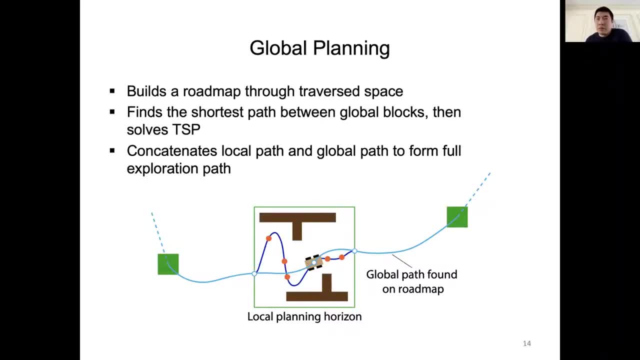 of the current implementation. I'm not sure what open means exactly. It doesn't mean that you don't define an exploration boundary. Yeah, I guess, yeah, You don't define a boundary, I guess, Yeah, yeah. So basically, there's a door going to the outdoor. 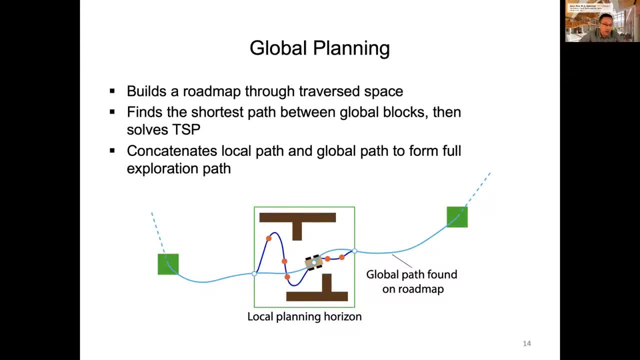 In our system, we have this boundary, We have this coordinate. It will not explore out of the corner. Okay, okay, You have to have it, Otherwise it will run out of battery somewhere. Yeah, exactly. So that's one of the things that we need to be aware of. 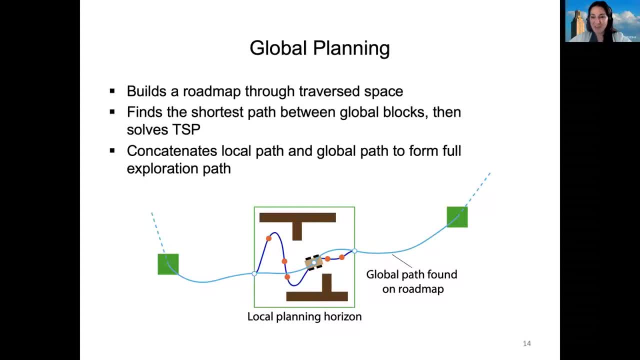 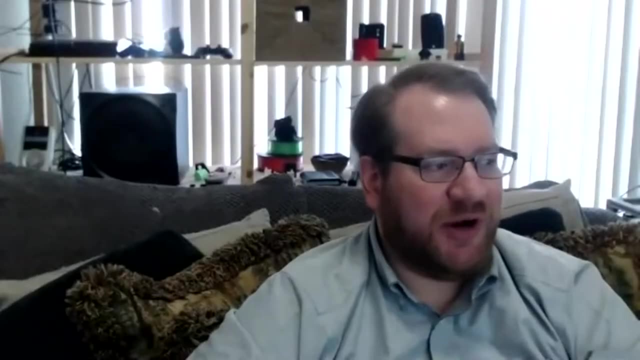 Okay, thank you so much. It was a fascinating talk, And our next session will be chaired by Justin Hart, Thank you, Thank you very much. So, yeah, hi, everyone. We're entering into our last session of papers. I feel like we might as well just jump right into this. 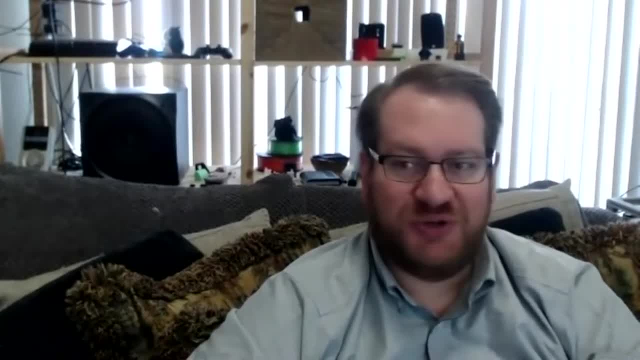 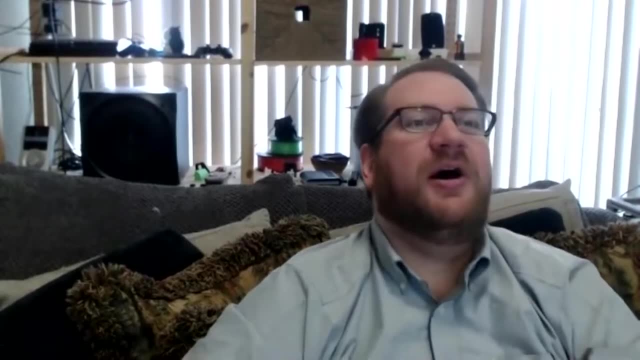 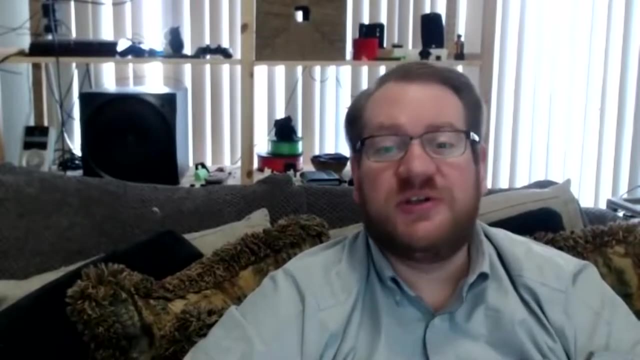 Our first paper is. the lead author is Wei Xu, which is wonderful. Our presenters are Zixiao Wang and Zifan Zhu, And I'm going to go ahead and get this shared. Let's see Screen to optimize for video, which it's not letting me do that. 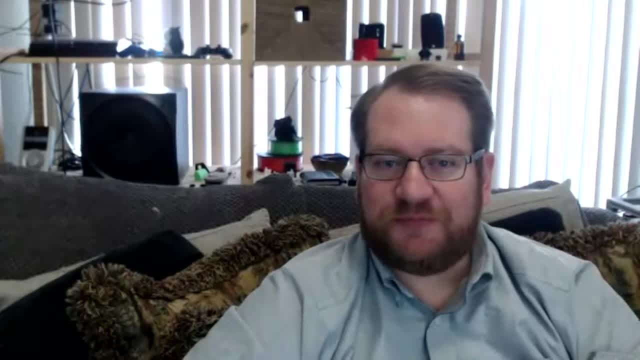 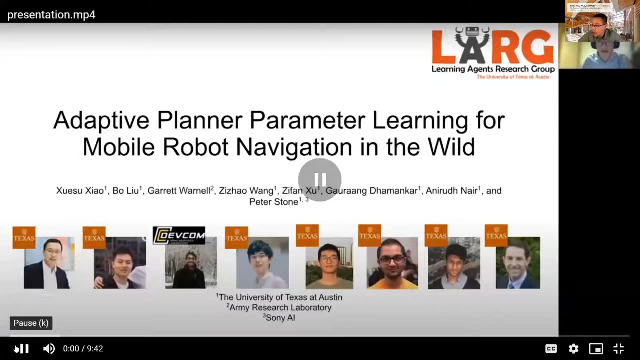 So that is just live share sound. All righty, Justin, can you try again? I think I forgot. I forgot to make you a co-host And now you should be able to do the optimizing for video thing. All right, Let me. let me get that set up. 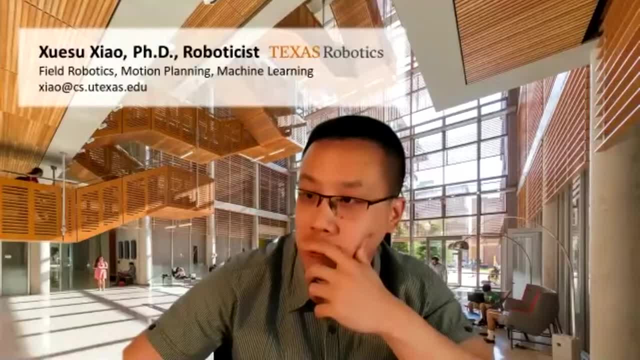 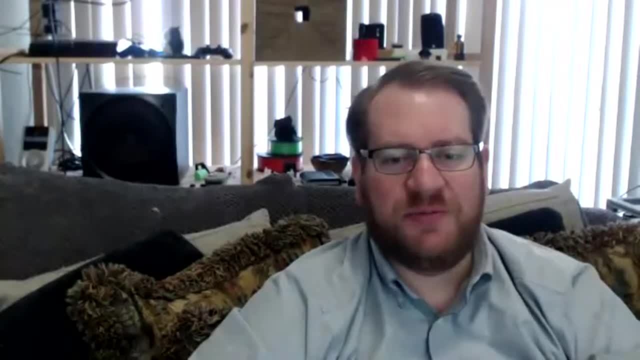 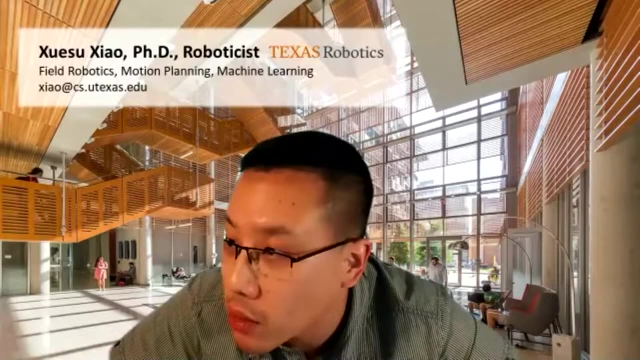 Okay, so stop share share screen. It doesn't give me the optimized video clip option- One sec, I think- just some advanced one. Oh yeah, I think Now you should be able to do it. Oh, now I have it. 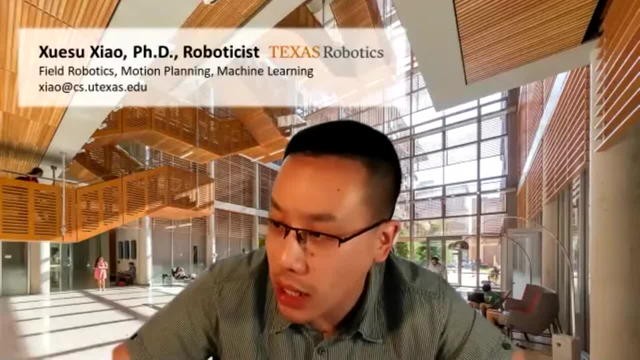 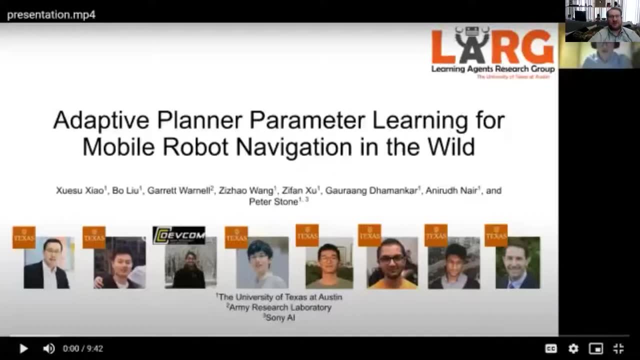 All right, So one participant has to like are allowed to share at one time. I think that's the option you need to do. Yeah, All right, So does everyone see it? Does everyone see the clip? Yes, Yes, Hi everyone. 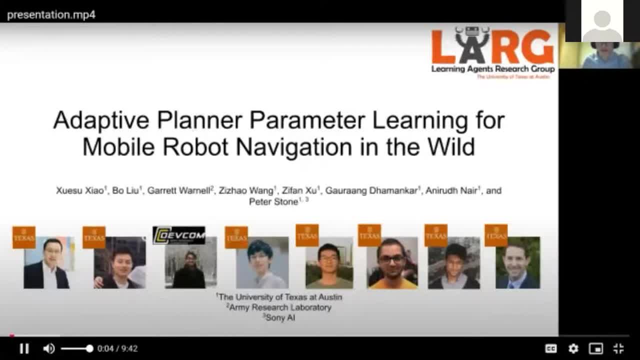 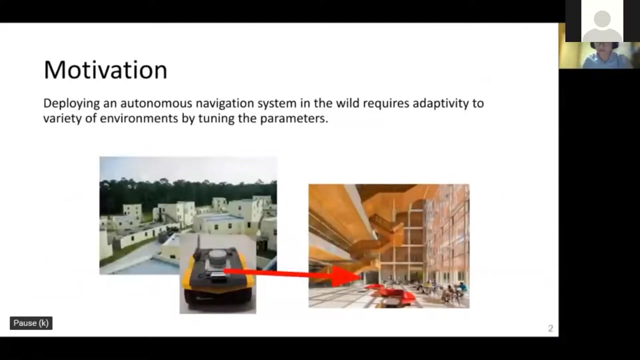 I and my collaborator Zixiao Wang will be presenting our work: adaptive planner: parameter learning for mobile robot navigation in the wired. This work was done by Xue Suzhao. This work is motivated by deploying an autonomous navigation system in the wired. requires adaptability to a variety of environment by tuning the parameters. 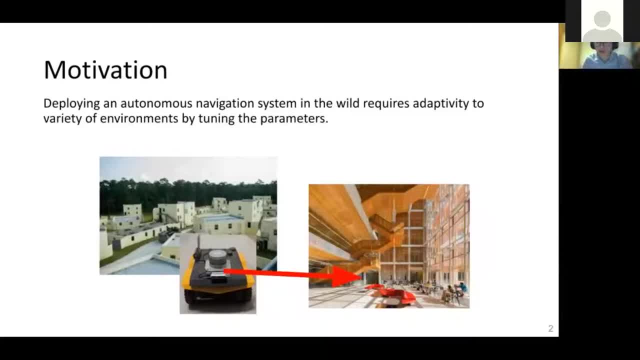 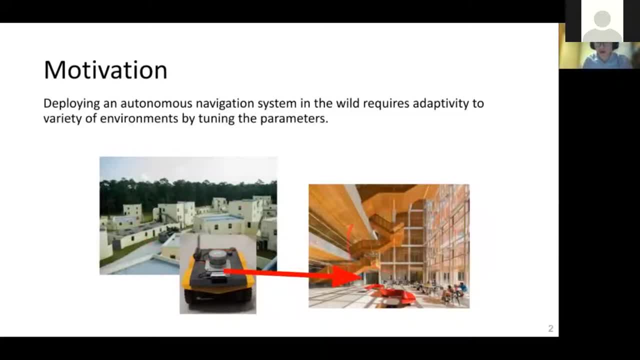 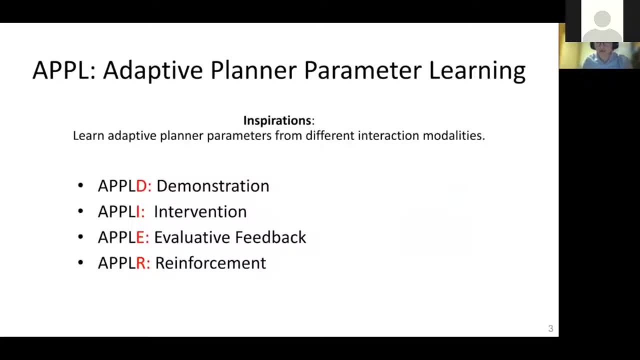 We want to develop to a different environment that really requires the tuning of the parameters. So we propose our learning framework: adaptive planner parameter learning and then adaptive planner parameter from different interaction modalities. We propose the following four different learning frameworks, But the first one, Apple D, learning from demonstration, and Apple I, learning from intervention. 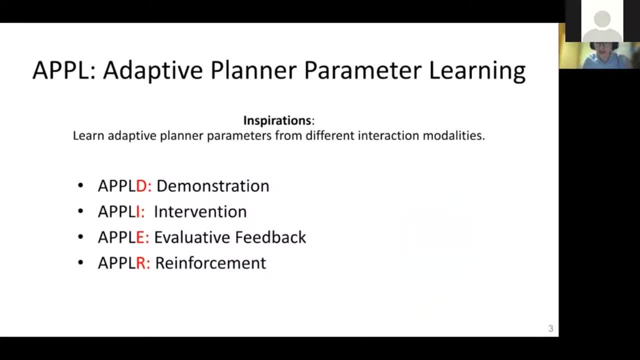 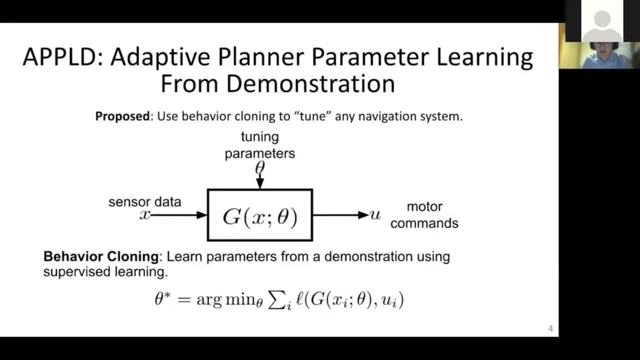 Apple E, learning from evaluating feedback. And finally Apple R, turning from reinforcement. The first is Apple D. The idea of Apple D is to use the behavior cloning to tune any navigation system. So we model the Apple D as a black box. 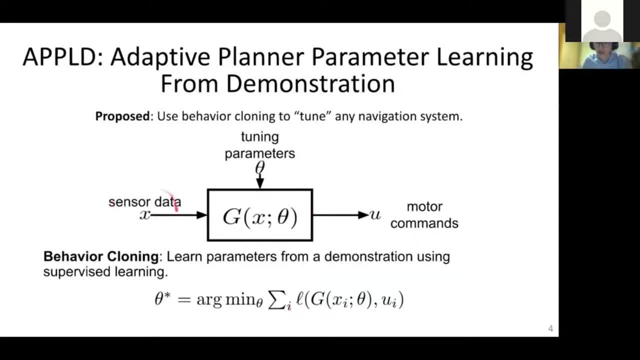 which take in the sensory data as an input and generate the model command to operate the mobile robot. The status of the navigation system is represented by the parameter, So we use the behavior cloning and then some parameters from a demonstration using a supervised learning. The goal of this optimization is to solve. 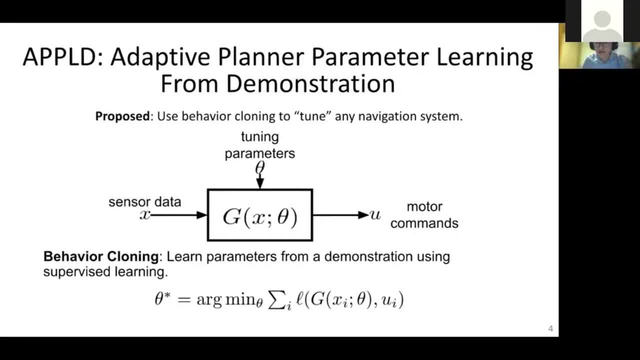 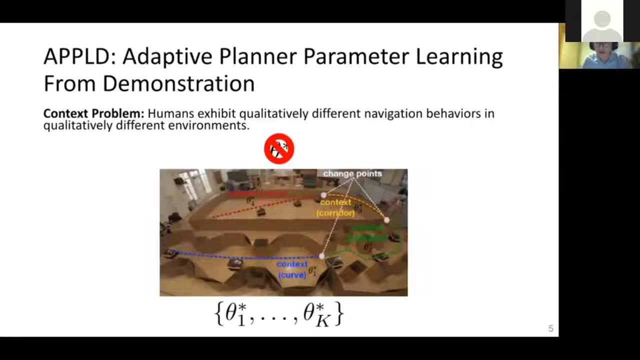 an optimized set of parameters that minimize the loss between the motor command and the motor command generated by the navigation system. And Apple D also deal with the context problem: The human acts with qualitatively different navigation behaviors in qualitatively different environments, For example in one demonstration. 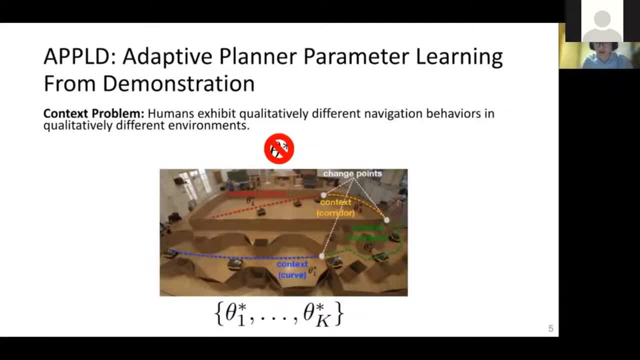 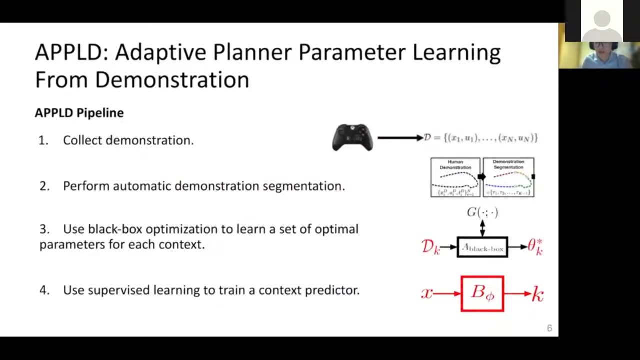 it purely has a different context, that has different navigational behaviors that can be represented by different optimal parameters. So we want to learn the optimal parameter for each of the contexts. So we propose the whole pipeline of the Apple D. First we collect the demonstration. 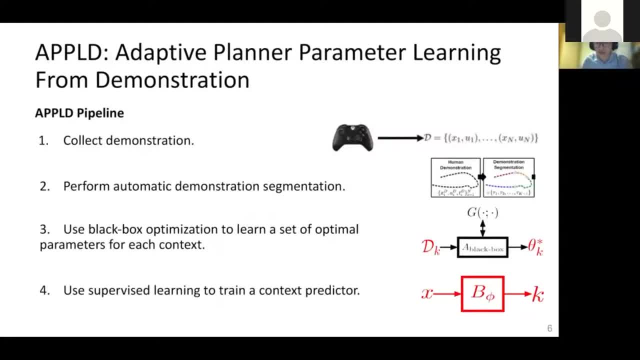 Then we perform an automatic demonstration segmentation, Then we use a pipeline, Then we perform a black box optimization to learn a set of optimal parameters for each of the context And finally we use a supervised learning to train a context predictor. The context predictor: take in the sensory input. 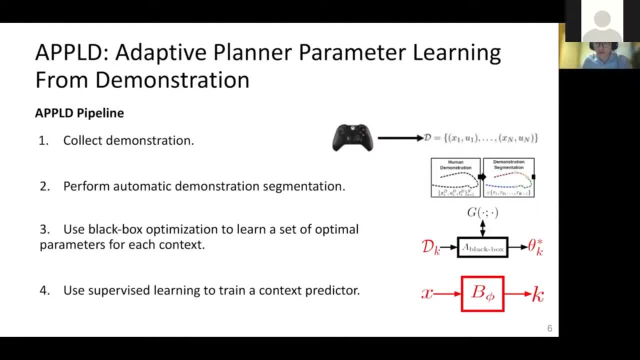 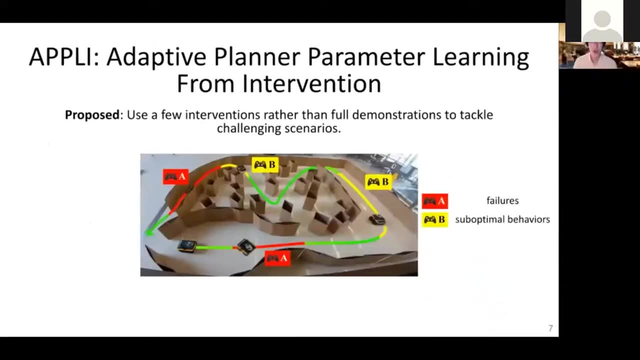 and predict the index of the context, Then it uses the corresponding optimal parameters for this context. The evaluation results of this paper can be found in the official website of this symposium. The next: we introduce Apple I and the input action modality is intervention. 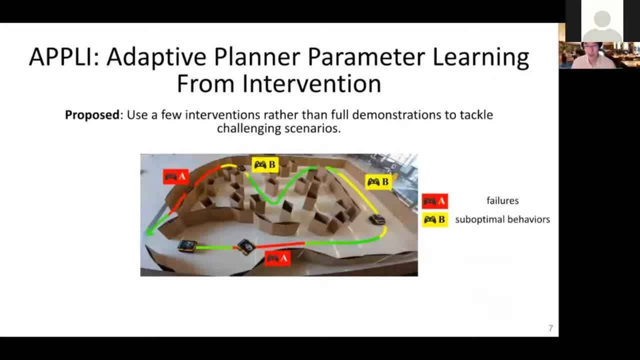 So sometimes the full demonstration is not available And also we find the navigation system with default parameter URE exceeds three kinds of behavior. The green one represents it's working pretty well And the bright one is failure, So sometimes it may get stuck. 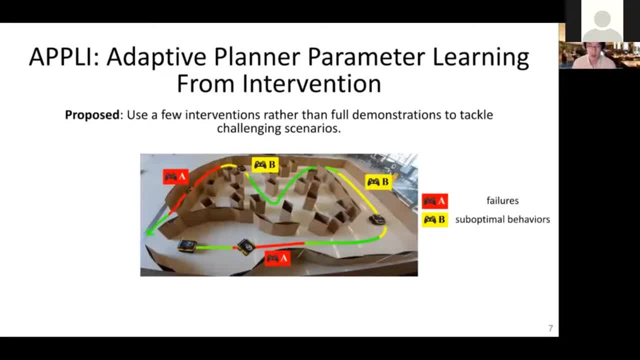 Or it flies with obstacles And sometimes the yellow one is the suboptimal behavior. For example, in this safe open space it may still drive very conservatively and drive too slowly. So in this case, for the failure and for the suboptimal. 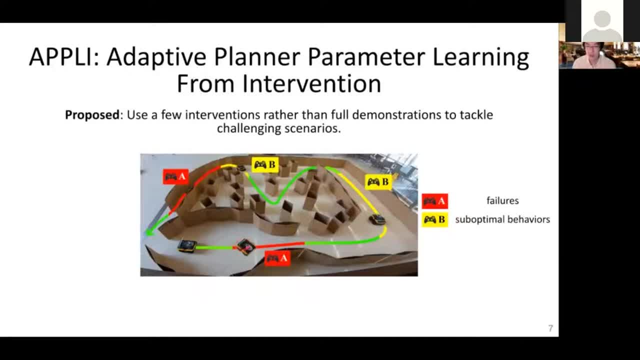 behaviors. we could just reset the robot to the beginning and give a short demo, And in the next slide we'll talk about the intervention, which applies to all the interventions, And for the intervention we will use the same method in Apple D to learn the parameter for them. 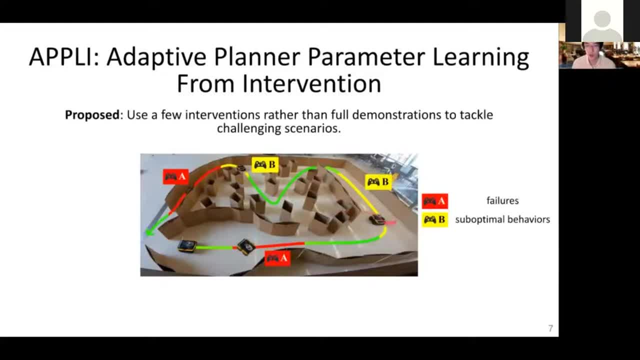 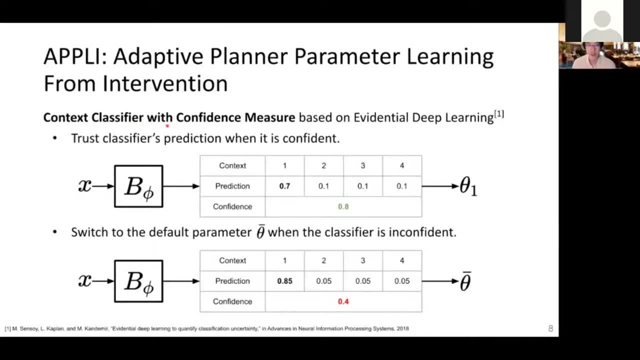 However, we cannot accept those intervention. contacts will generalize to all environments, So in this time we augment the contact classifier with competence measure That is based on the paper Evidential Deep Learning, For example. the context classifier will take the sensor data as input and it outputs the prediction properties for each context. 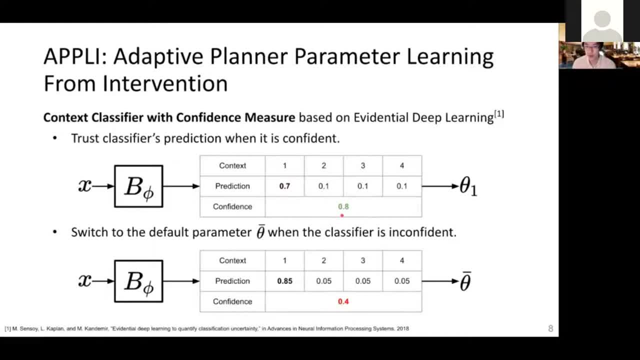 Also, it outputs the confidence and where 1 represents the context classifier is 100% confident about its prediction. So in this time the confidence is very high. So we believe the prediction is correct and we will adopt theta1, which is the parameter for context1.. 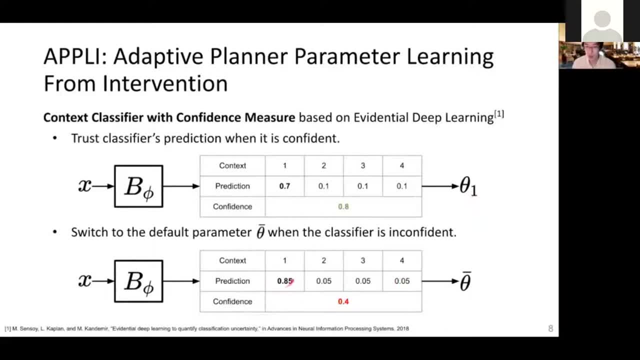 However, in this example, even though the prediction probability is very high, but since the confidence is very low, we will just use the default parameter rather than theta1. Because the default parameter is tuned to work for almost every environment And it should generalize better. 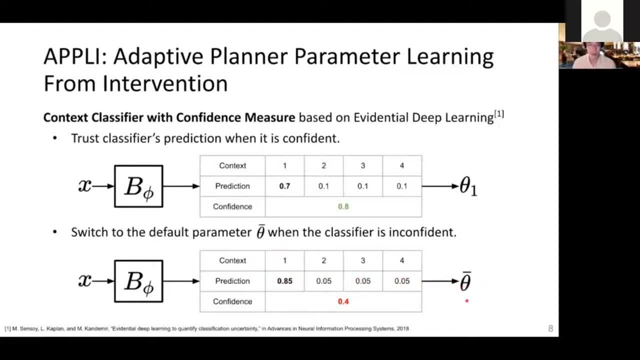 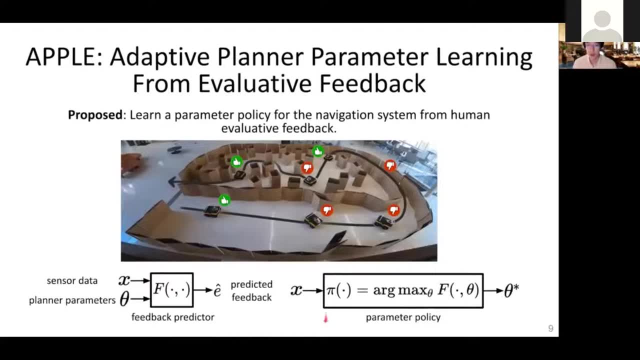 Then this specific parameter, theta1.. And then is our work employee evaluative feedback. So in some case, the supervisor may not be able to, or unwilling to, take control of the robot, So we don't have access to either demonstration or interaction. However, in this case, we could still utilize evaluative feedback from the supervisor. 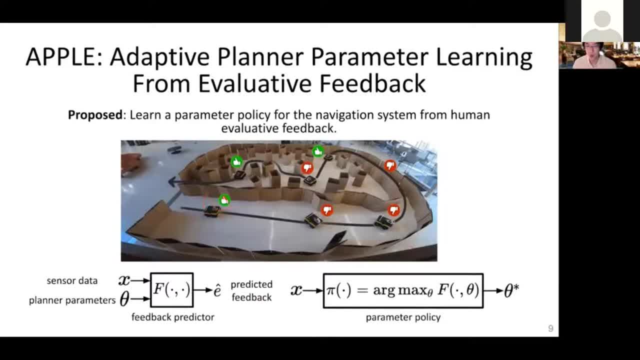 For example, the human may say good job when the robot is working well or say bad job when it gets stuck or collapsed. So in this case we learn a feedback predictor that takes the sensor data and current center parameters as input And we try to predict what kind of evaluative feedback that human will get. 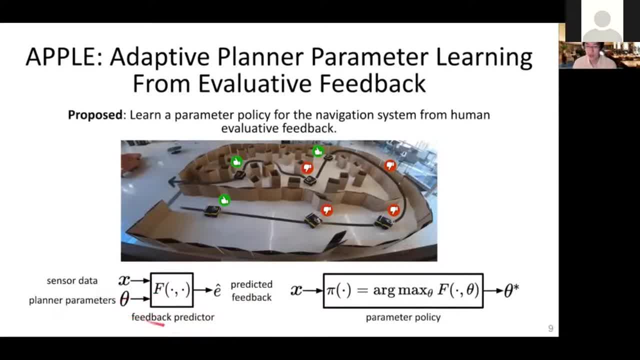 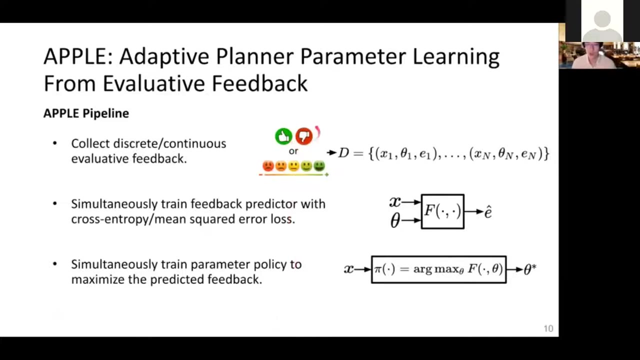 So once we have this feedback predictor, we will also learn a parameter policy where we optimize the performance by trying to select the parameters that will give us the highest probability to receive positive feedback. The whole pipeline is like this. So, even though in the example before we described a discrete evaluative feedback, 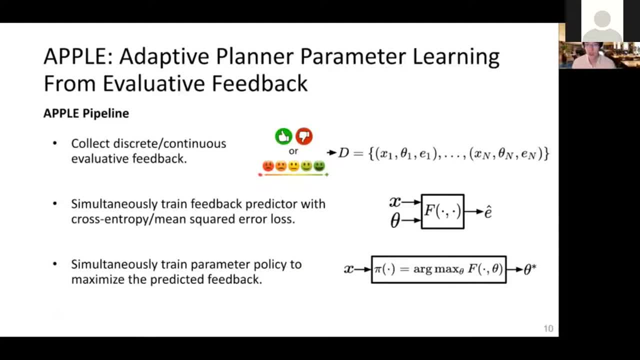 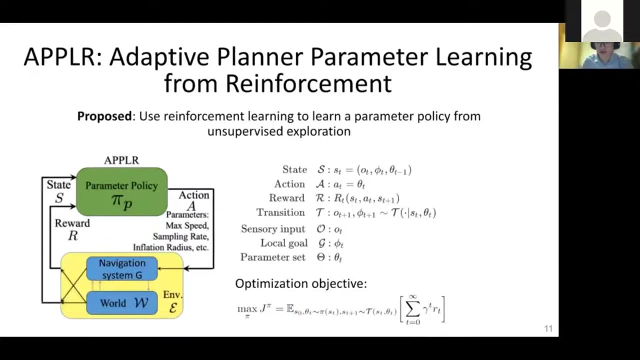 but we also accept continuous one, like a score between 0 and 5.. So simultaneously we will train the feedback predictor and simultaneously we will train the parameter policy to keep improving the performance of Apple R. Finally, we present Apple R. 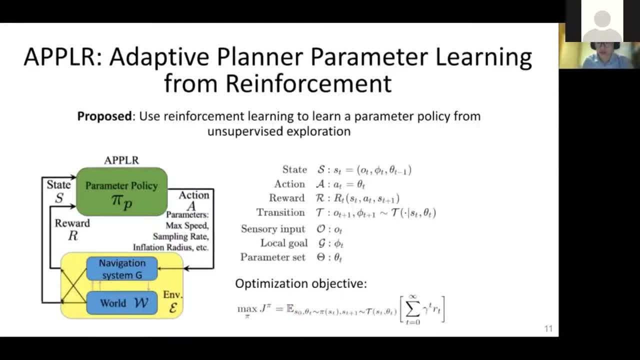 The idea of Apple R is to learn a parameter policy from the reinforcement algorithm. Because Apple R does not limit to the human's knowledge but learns completely from its own exploration, so it's supposed to be more generalized to different environments. We first frame our problem as a Markov division process. 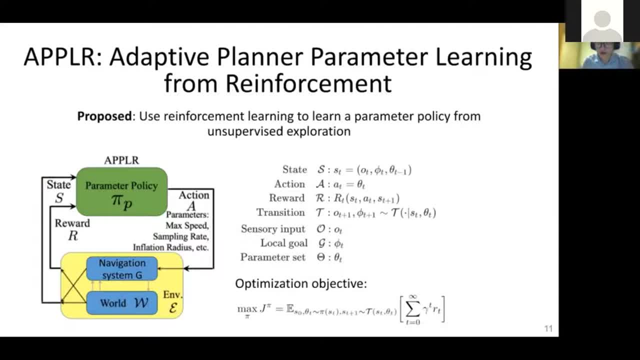 The environment is composed by the navigation system and the physical world. At each of the time step, the environment will take in a set of hyperparameters and the navigation staff will navigate based on the parameter for a fixed time step, for example, 2 seconds, used in this work. 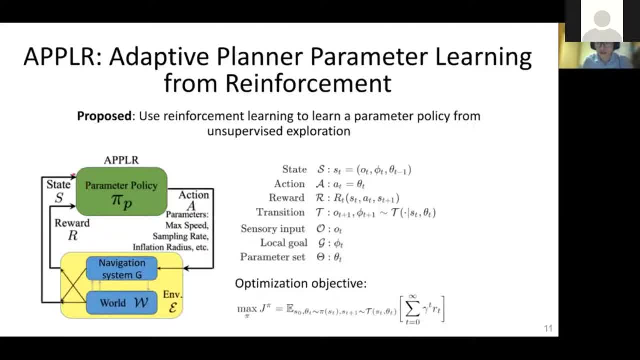 And it will generate the state of the system for the next time step. More specifically, the step is composed of the sensory input, local goal and the parameter set from the last time step, which serves as a short memory. An action is a set of parameters. 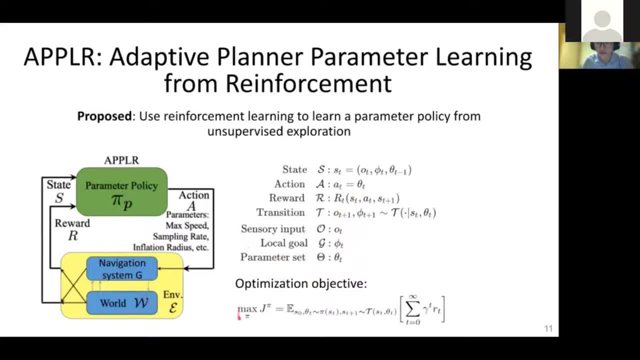 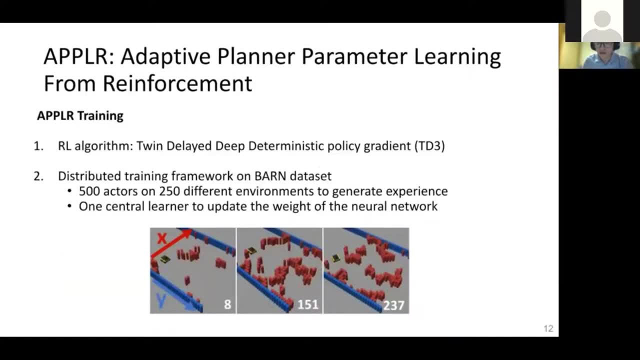 And the optimization objective is to maximize the accumulative reward. And Apple R is trained with the twin-delayed deep deterministic policy gradient, which is also called TD3, which is a state-of-the-art off-policy IOL algorithm that deals with the continuous action space. 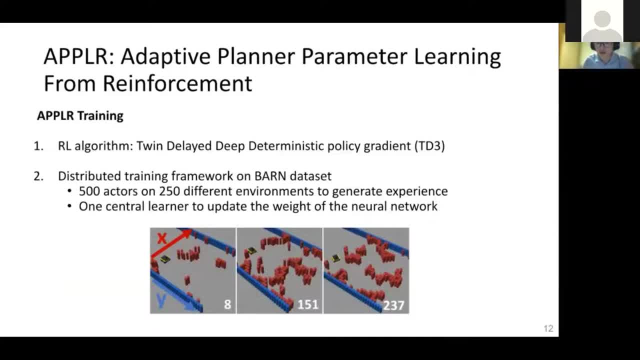 It will also develop the distributed training framework on Born dataset. The figure at the bottom shows three examples of the Born dataset environment with different difficulty levels. We have 500 actors on 250 different environments running parallel. to generalize the environment, to generalize the experiences. 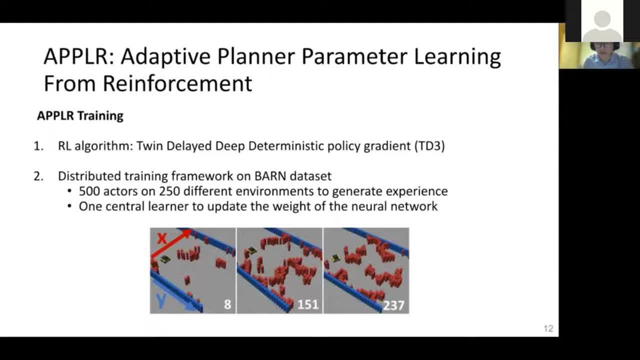 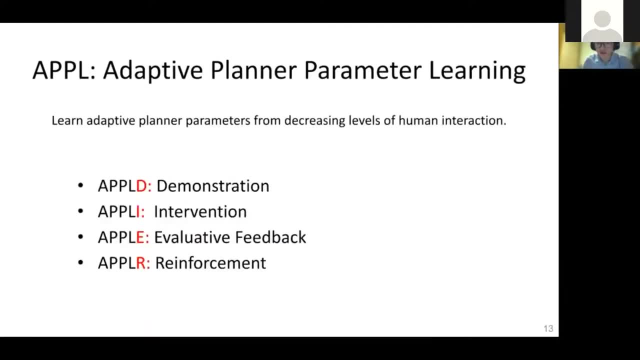 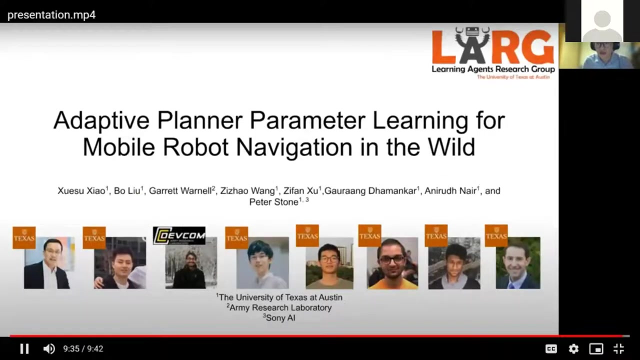 And then we have one central learner to update the weight of the neural network. In summary, we proposed the learning framework of adaptive planner parameter learning. Then we proposed four different learning methods with decreasing level of human interaction. Thanks for listening the presentation. 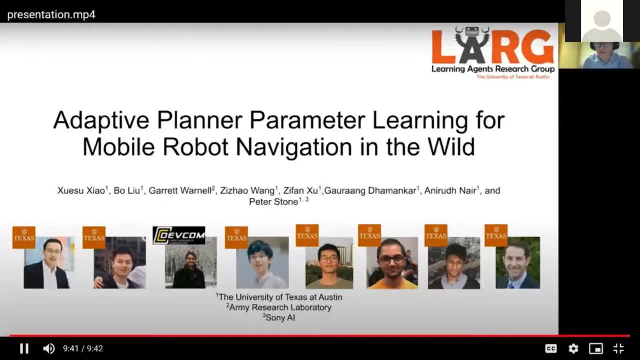 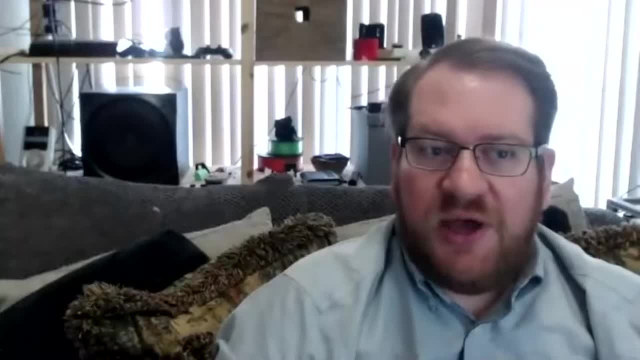 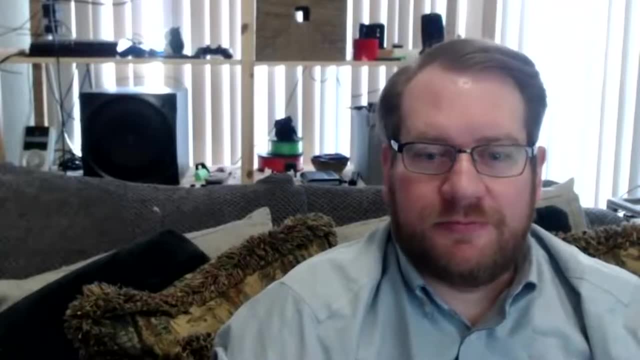 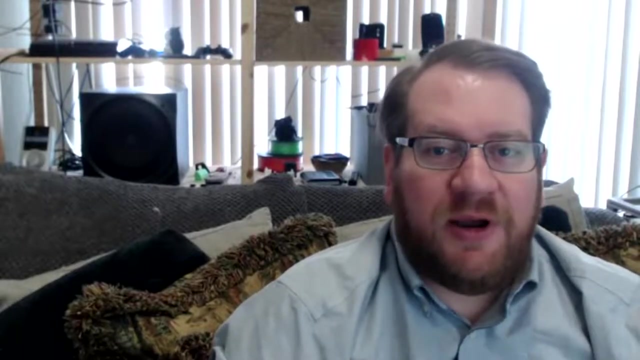 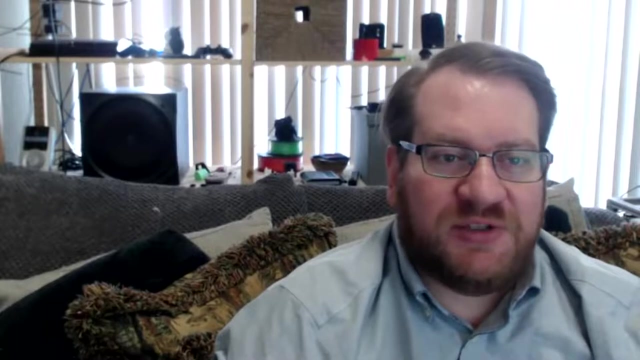 We're happy to take any questions. Thank you, Let's go ahead and open up the floor to questions to our speakers. All right? Well, I have a question. So you have this whole variety of different ways to provide feedback to the robot in order to train it. 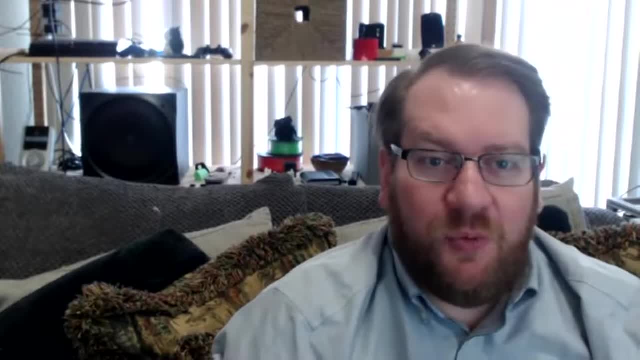 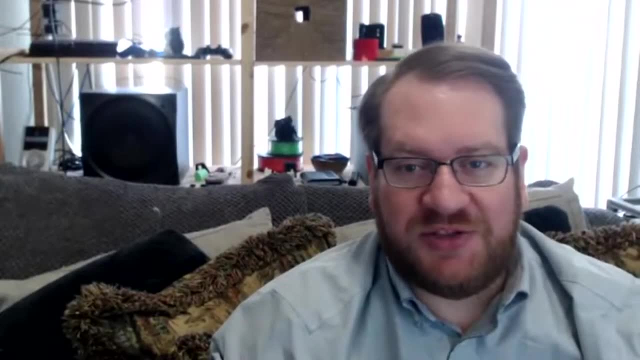 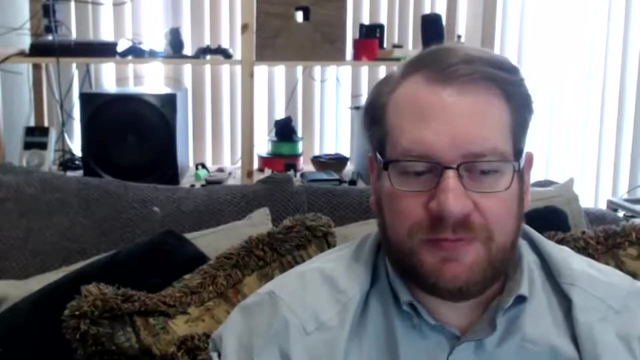 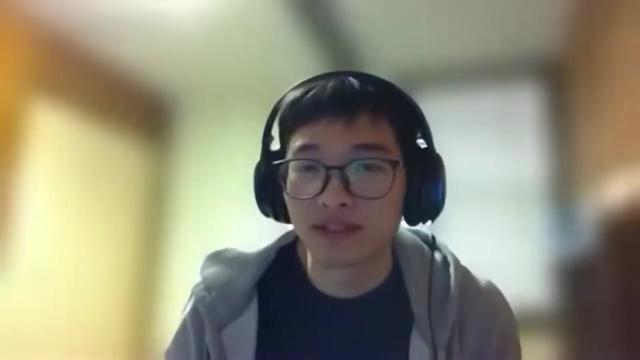 Have you thought of having, like you know, one single? You have this Apple framework, but have you thought of having sort of an overview training system that could accept all these different inputs, And how would that work? We're actually developing a cycle of learning framework. 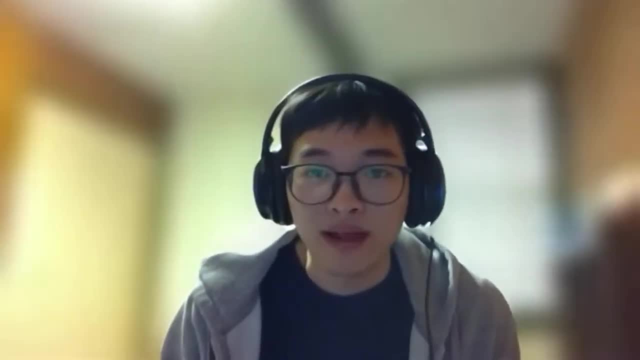 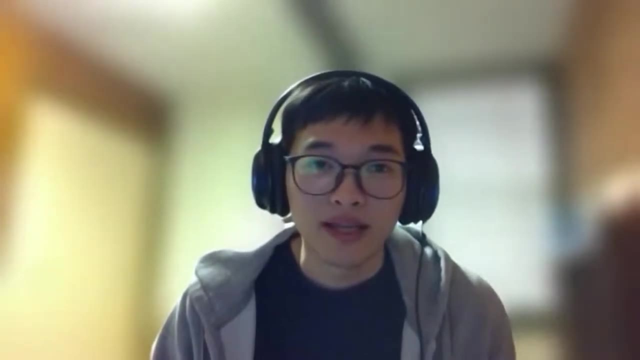 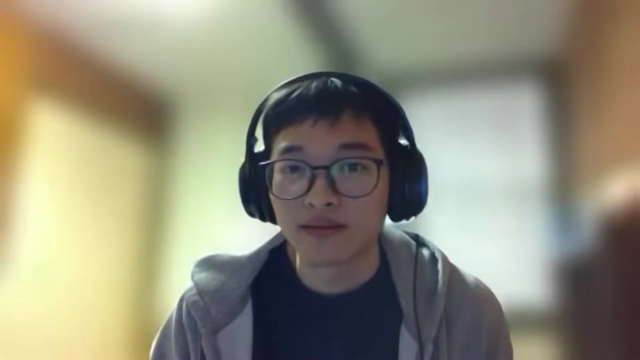 I think all of this learning method, it has the capability to take in the previous method or policy that then could take in any form of input from the human or self-exploration and to improve based on that. So to add on that, for example, 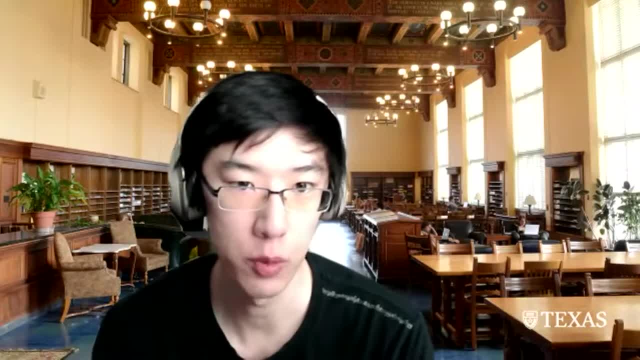 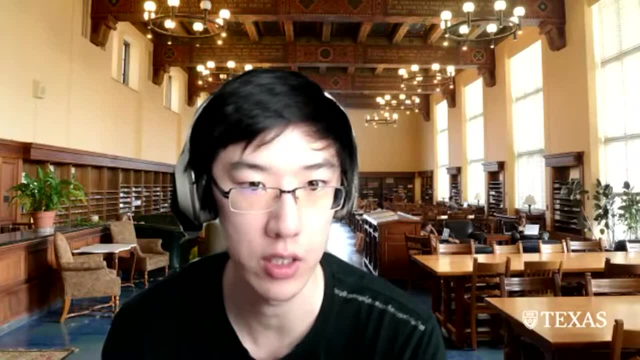 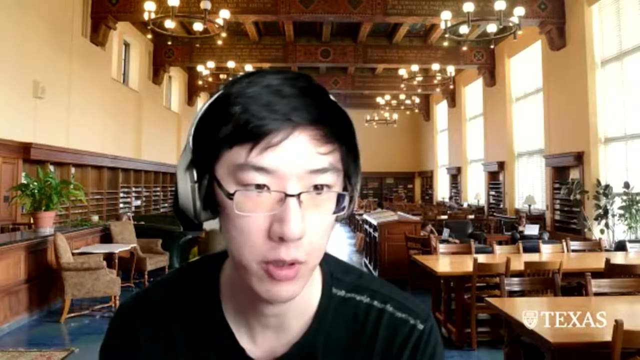 if you have an initial policy that's not working well and you want maybe- Or it's good enough, but you want- to deploy it into an entirely new environment and then it's performance downgraded. So in this case, maybe you can first collect some demonstration. 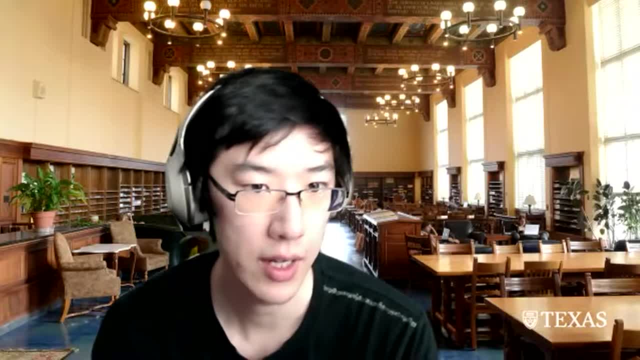 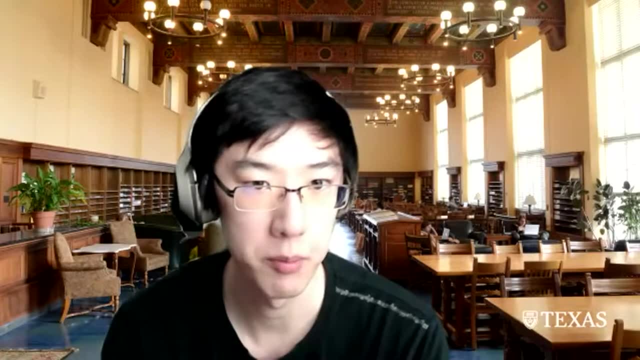 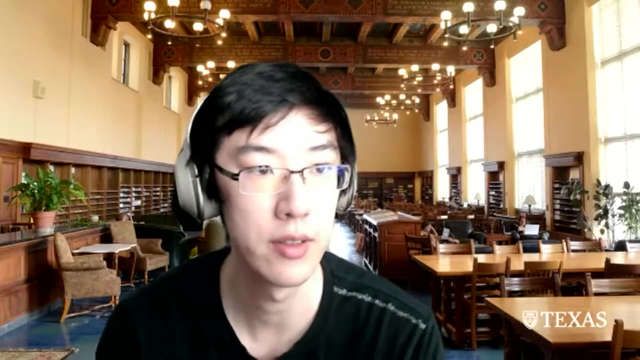 and use Apple T to train that, And after that I think it's basically familiar with a new environment. but still it may Struggle at some place, but just a little portion of the space. So in that case you can use the intervention to correct these behaviors. 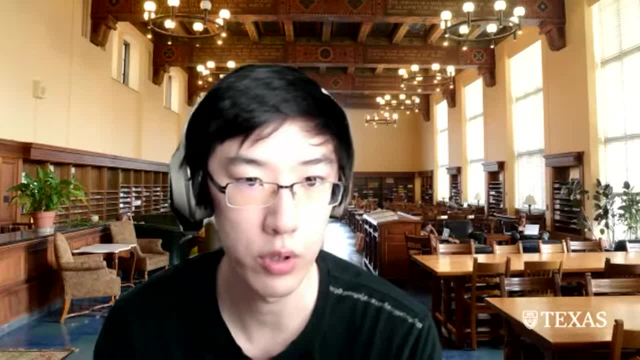 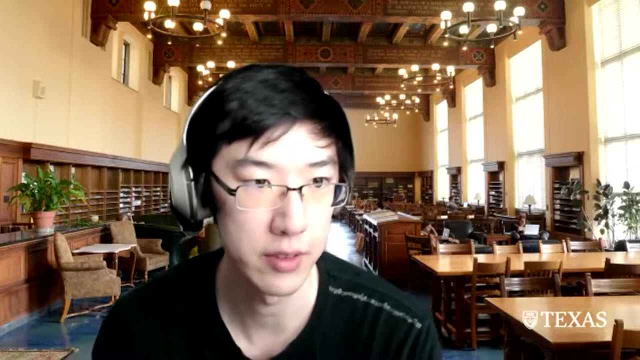 Or further. if you want to improve, you can use evaluative feedback, which is less demanding because you just need to provide some easy feedback like good job, bad job, like that. So, basically, I think you can use this pipeline to. 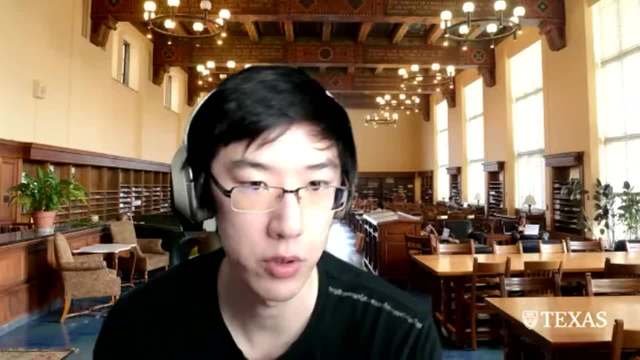 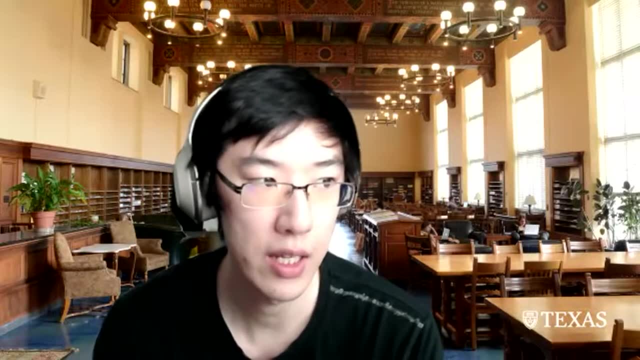 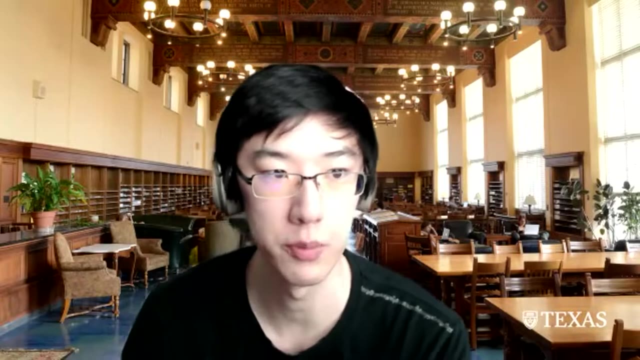 Or even, if you want to further develop, you have a lot of. You have learning model policy from Apple D, Apple I, Apple E, And you can use them as to bootstrap the learning from reinforcement. Oh, sorry, To bootstrap the reinforcement learning. 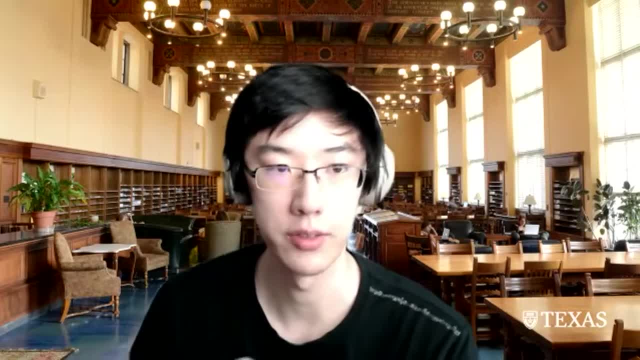 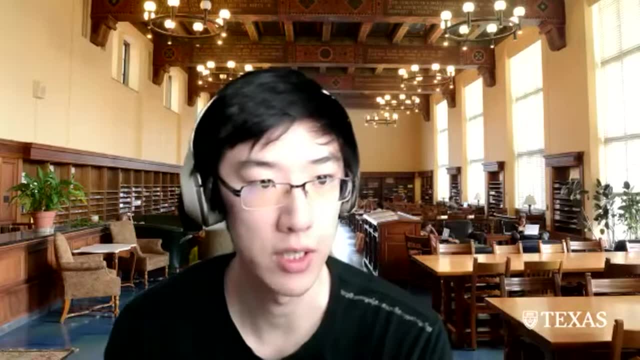 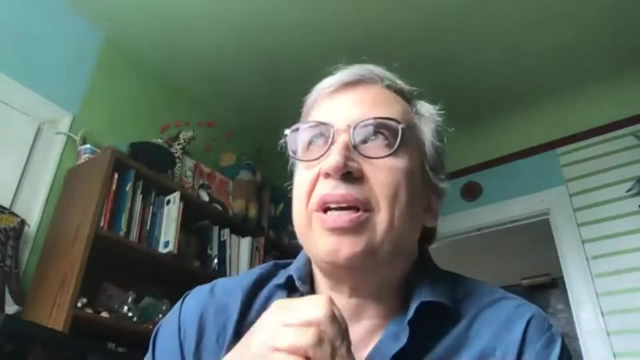 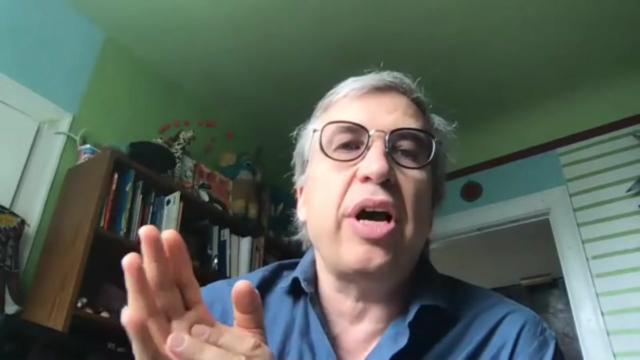 So to further learn better policy? Yeah, Any other questions? Yeah, I have one. So have you thought much about the contextual dependency of the learning from the different people and the people state, And so how you might want to accommodate the fact that? 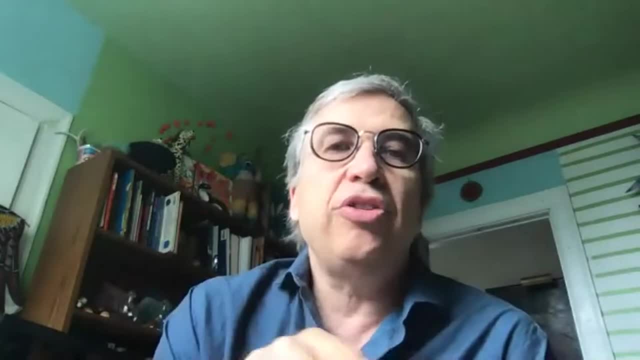 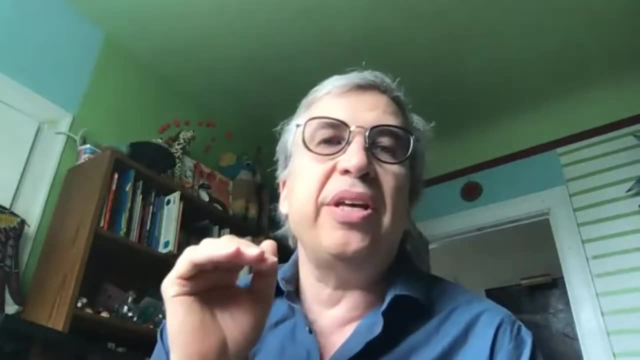 you know I'm in a rush now. I'm not in a rush now. I mean, of course you could query a person and get them to classify themselves into state as the kind of lowest learning level. But if you're in the lowest bar, 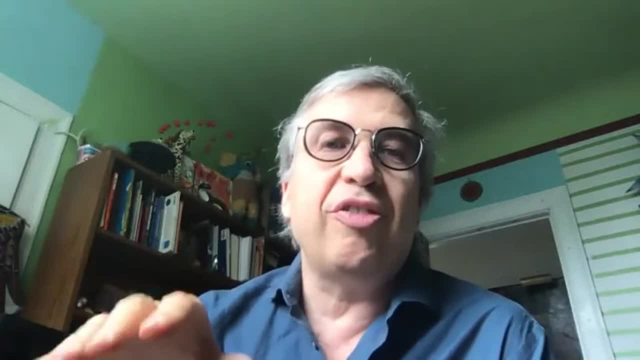 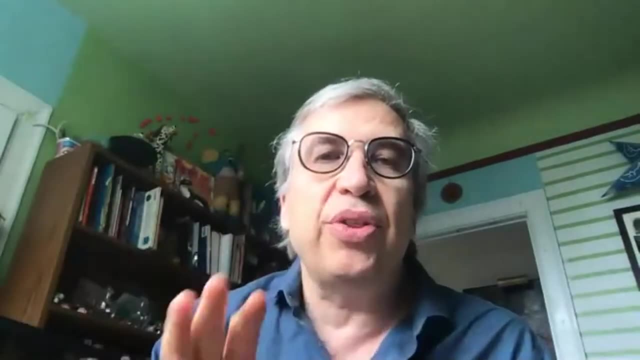 and then you learn parameters are contingent on those classifications. of course, then you have a problem with people not being consistent in how they classify themselves between different people. But so that whole issue of how to deal with different people and the fact that even single individuals have variable 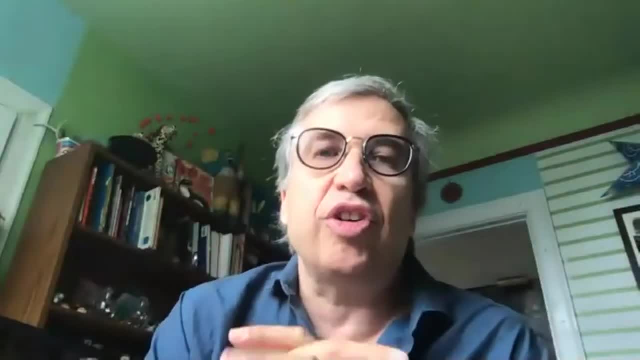 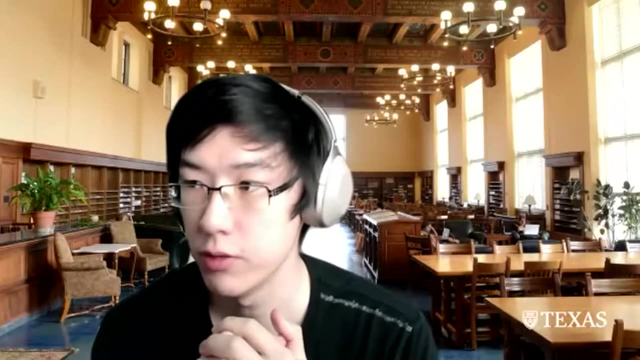 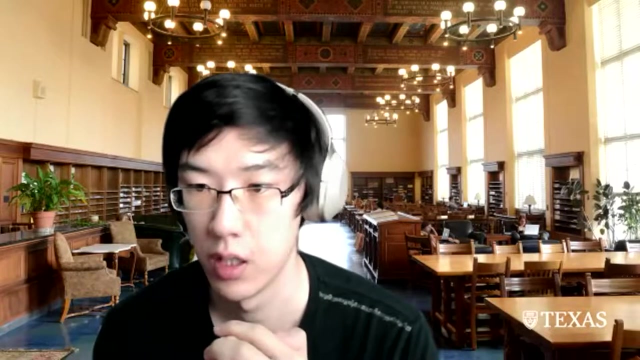 you know in the real world, different speeds and different levels of urgency and things like that. Yeah, that's a very good question. I think in our context, indeed, it's just based on the observations, So maybe one thing will help. is that in the Apple deal? 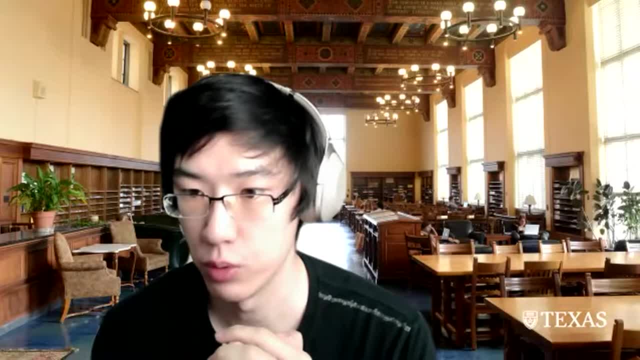 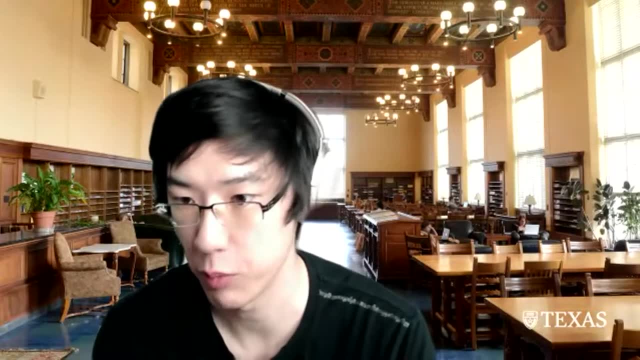 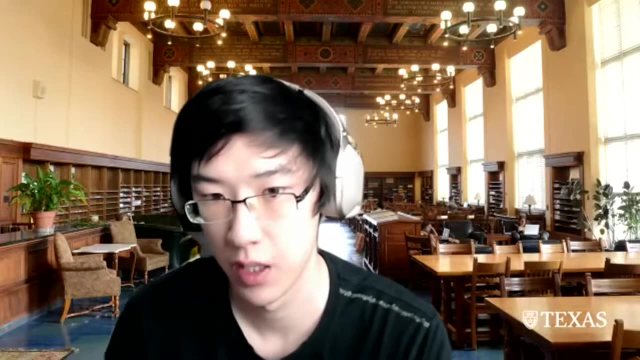 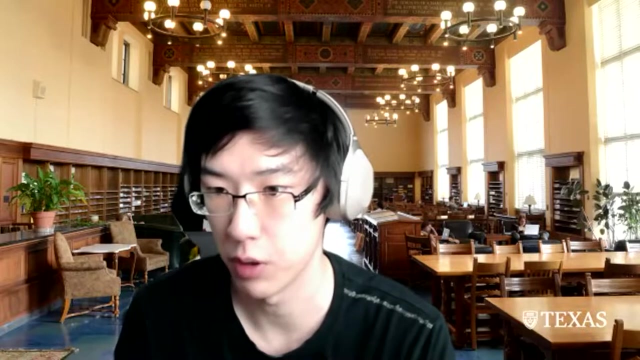 we have a method that will use Bayesian method to detect different modes of driving behaviors. For example, some people may- or a single person may- be conservative and they drive slowly at this time, But sometimes they may drive aggressively and drive very fast, And the Bayesian method will detect those different modes. 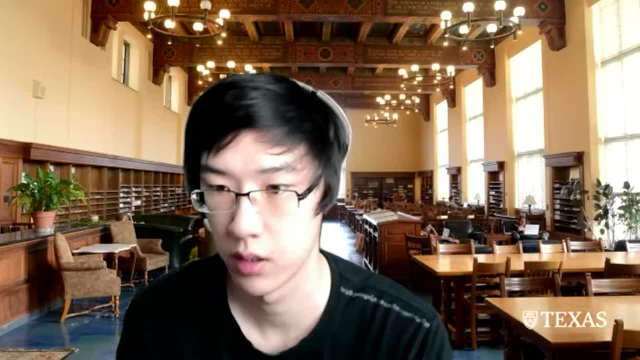 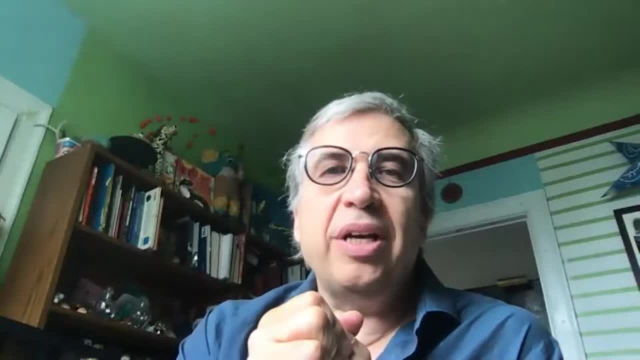 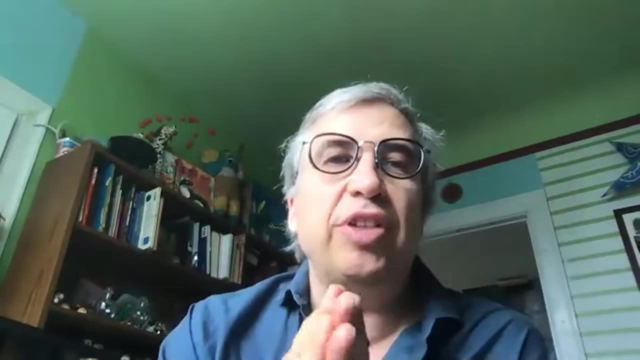 and split them into different contexts. Yeah, I think one tricky thing is sometimes people drive slowly because they're you know. sometimes they drive slowly because they want to drive slowly, And sometimes they drive slowly because they don't feel confident enough or they're bad drivers, right? 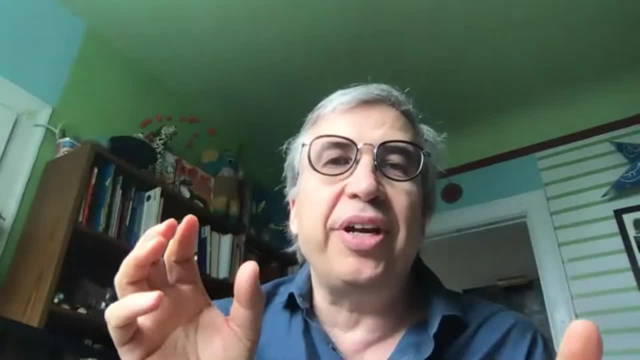 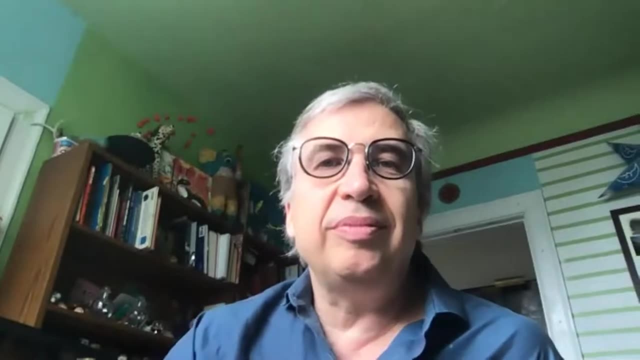 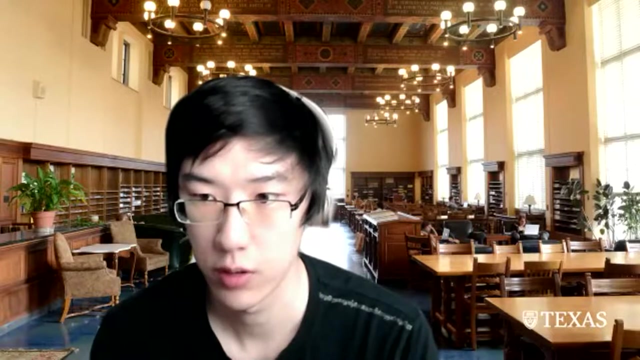 So there's two different sort of hidden variables that their demonstrations are contingent on, And knowing which case it is can be hard and maybe interesting. Yeah, exactly So we also noticed that in our experiment. So sometimes, when Usually the demonstration will help. 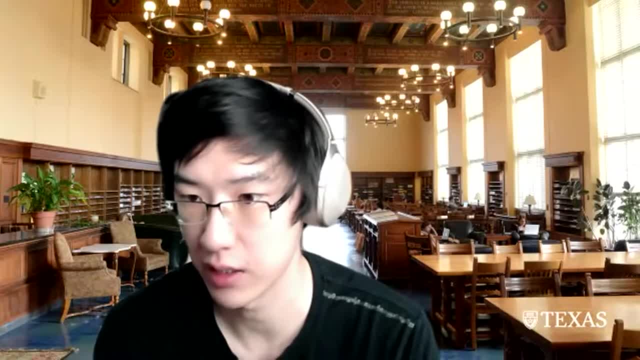 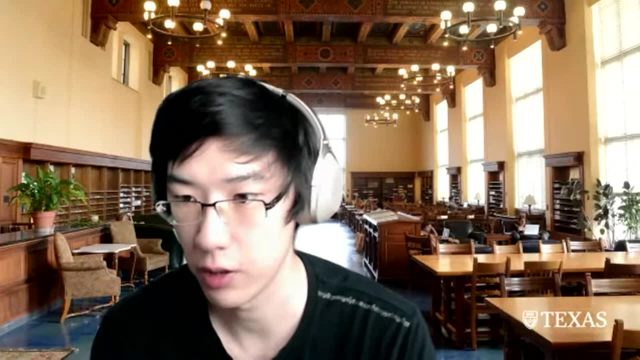 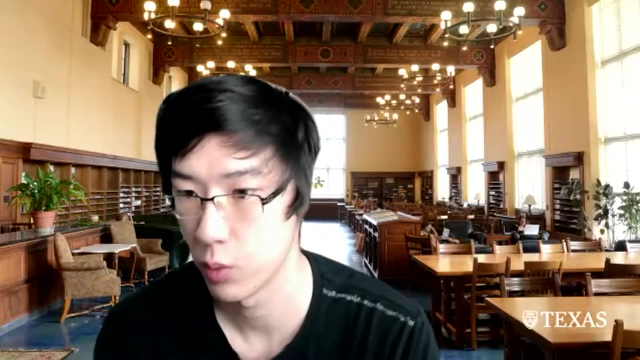 but sometimes they are not confident and drive too slowly and it even harms the performance. So maybe, So after we get all the contexts and their parameters, we can test them, Maybe for the sub-ultimate one. we can just don't use them when we're doing the deployment. 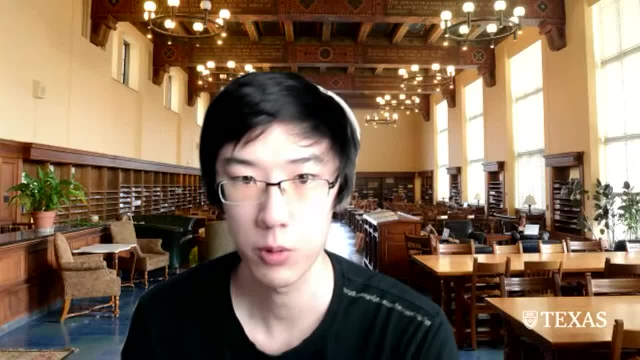 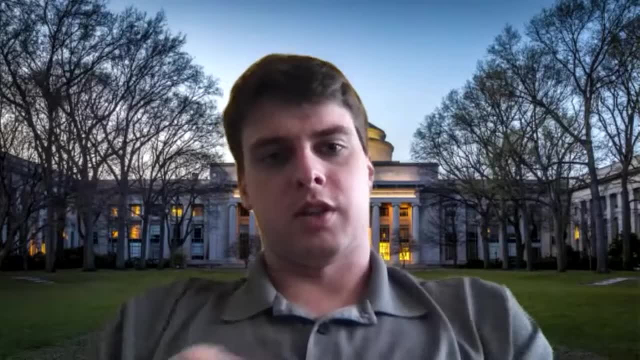 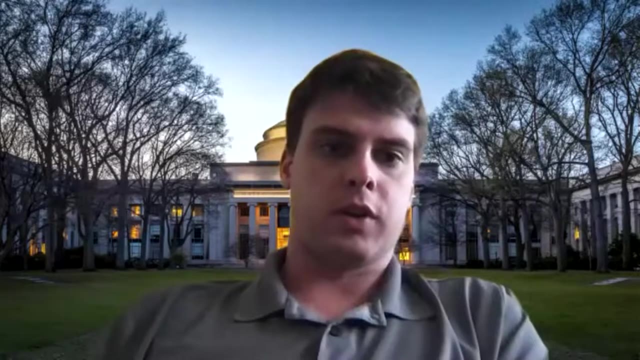 Yeah, Cool, Thanks. I have a question. I'm curious to hear your thoughts on how this idea relates to the field of adaptive control. I think, in particular, you know there's a lot of work in like reinforcement learning, where I think people are going. 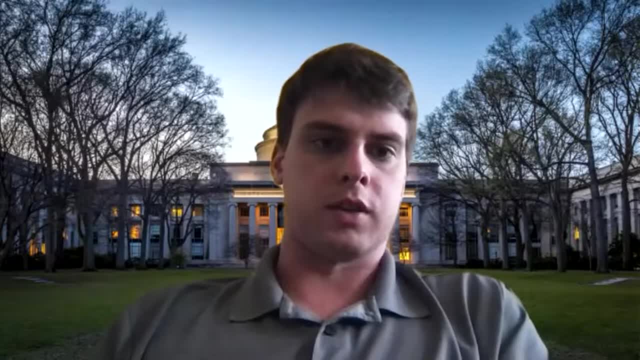 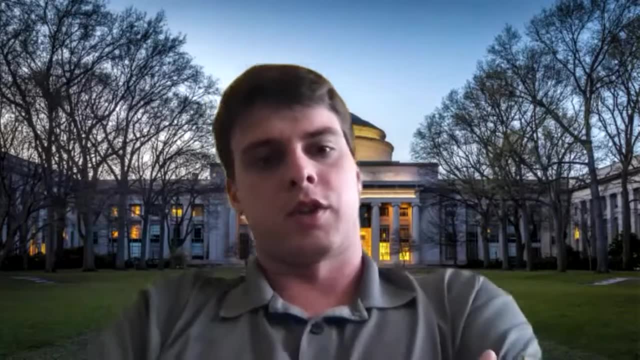 in another extreme of we want to learn a whole policy, where I think in this work it's more like we have a policy and we're trying to learn some parameters to tune it. I'm just curious to kind of hear any relationships between things that maybe have gone on in adaptive control. 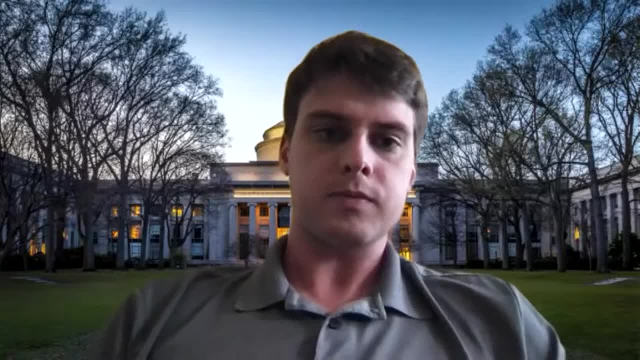 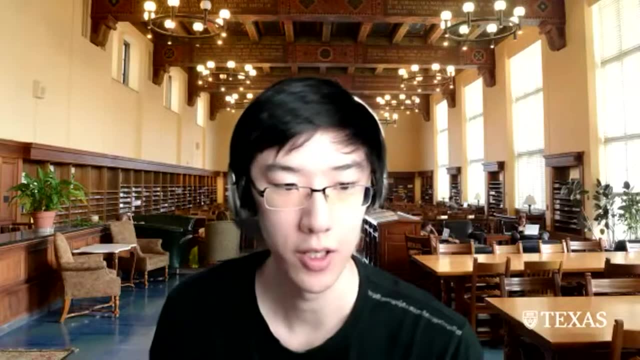 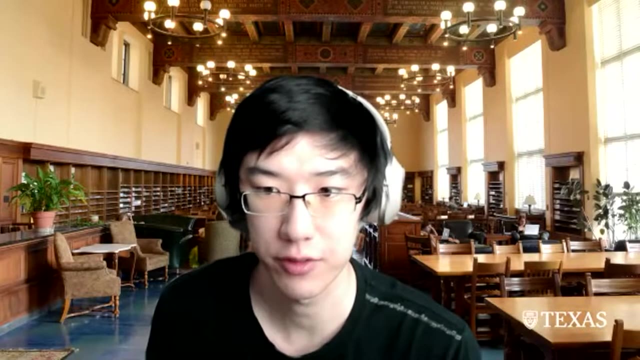 in the past versus what you're doing with planning here. Yeah, that's a good question. So unfortunately I'm not very familiar with that. I'm not familiar with that literature about adaptive control And I have thought adaptive control is where the model 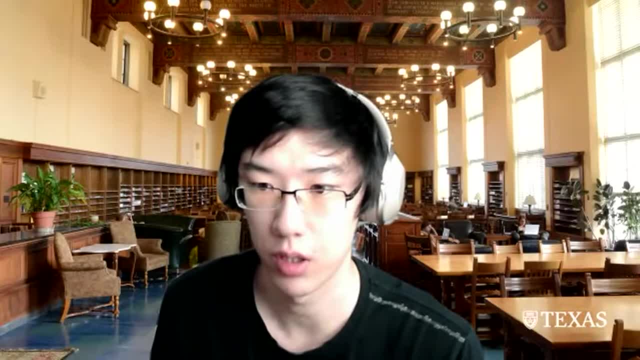 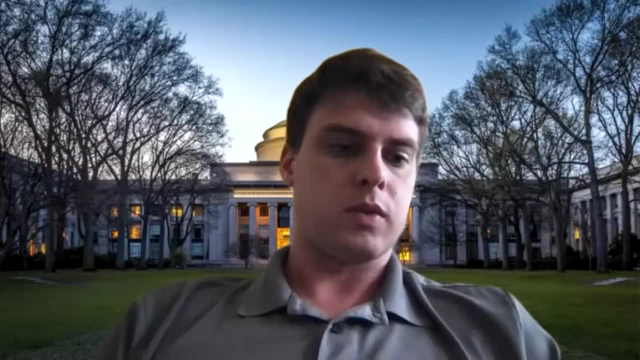 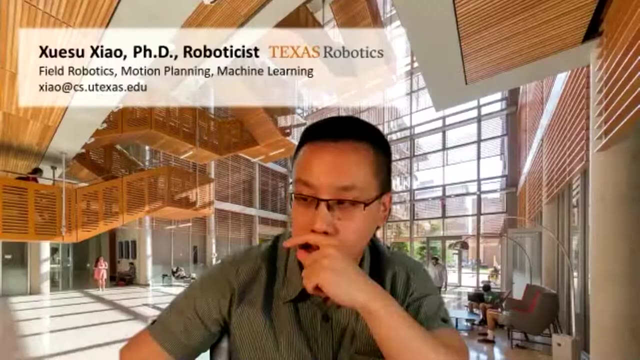 is changing with time, right, Or Potentially you could have that. Yeah, Or you may just not know the model, or you may not know some of the parameters in the model. I guess one thing is here: we are learning the parameters. 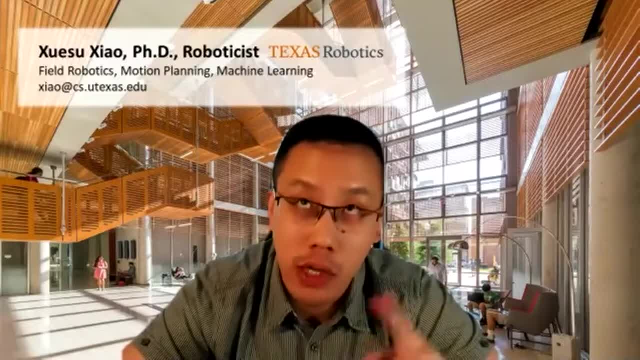 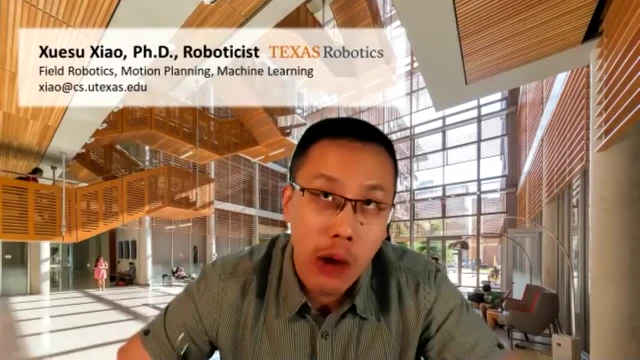 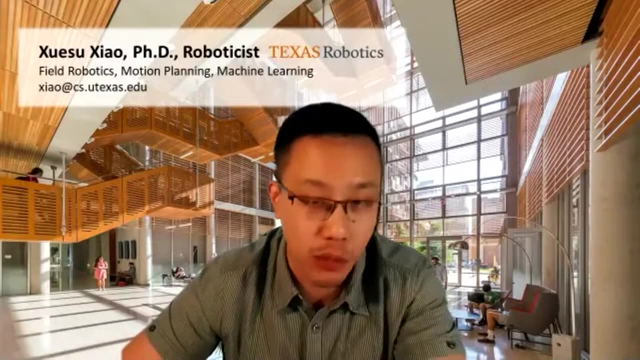 for a planner right, And also from human interactions right. So I would say so it's very similar to the taste of adaptive control, but I would say it's definitely be opposed to the direction of like reinforcement learning, because we do not want to learn an end-to-end motion planner. 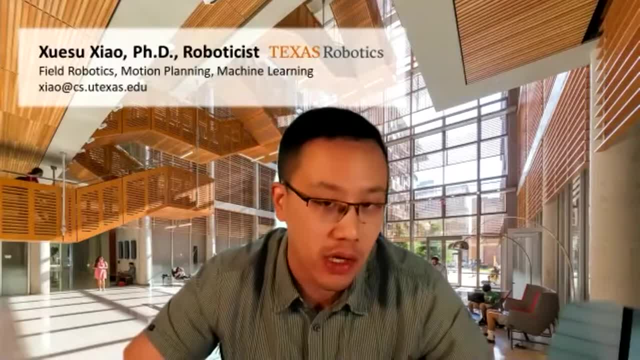 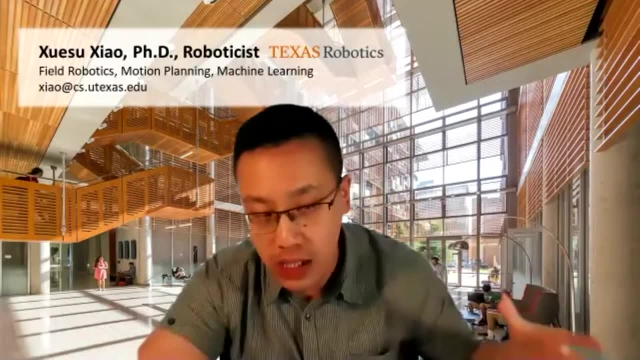 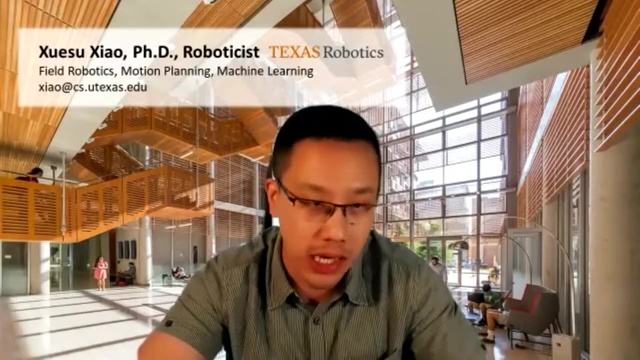 We want to bootstrap on top of all existing motion planners and just to find, like fine tune, the knobs on those classical motion planners to make them better. The idea is because all these advantages of the classical approaches can be inherited, like safety, like assurance, like explainability. 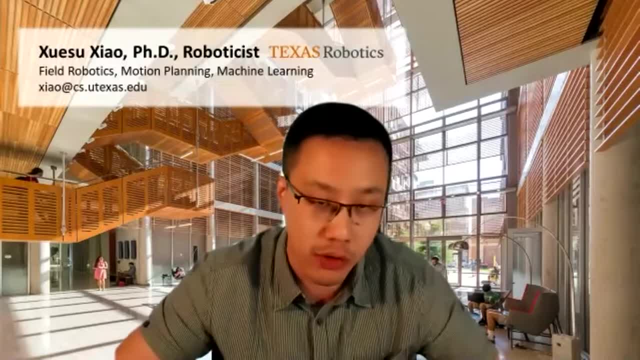 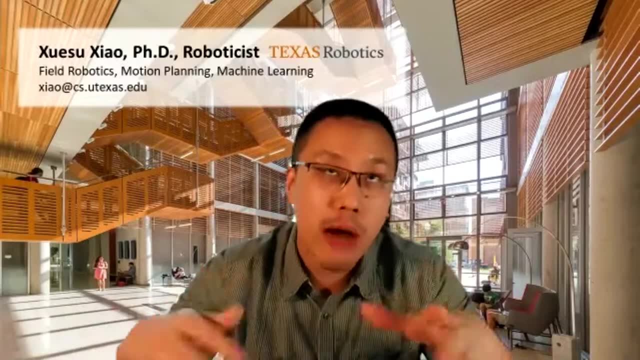 all these kinds of things. We do not want to learn everything from scratch. We learn on top of that. That's kind of like high-level idea why this Apple paradigm can, like I would say like- take the best of both worlds. 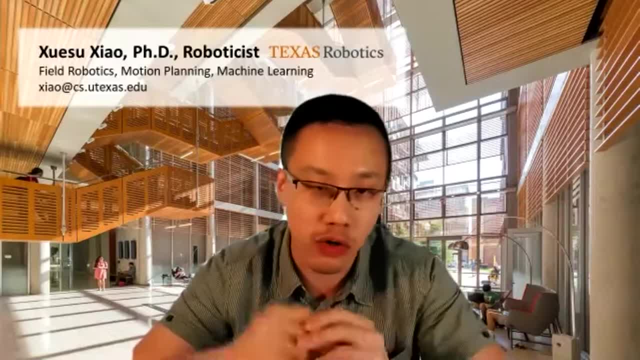 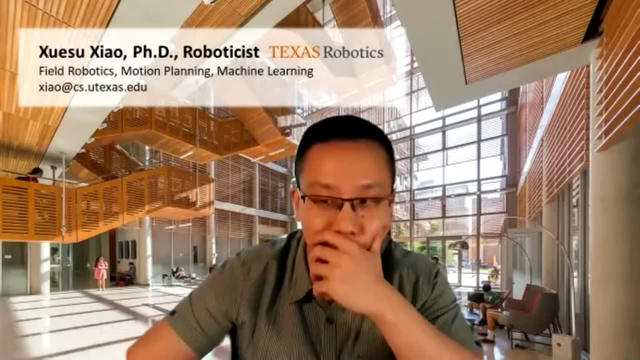 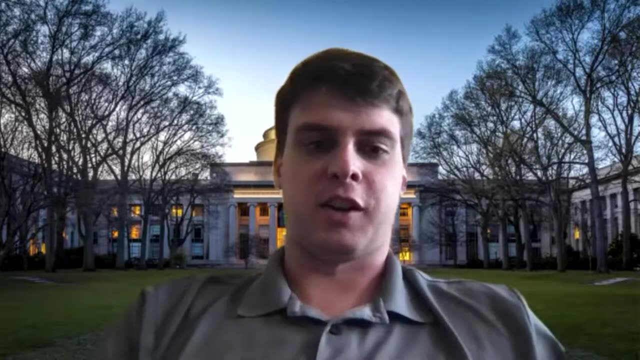 like classical motion planners advantages and also give it the flexibility and adaptivity of learning. That's kind of like a high-level idea. Yeah, that makes sense And I think the way you described it as tuning knobs like makes that connection to adaptive control even more clear. 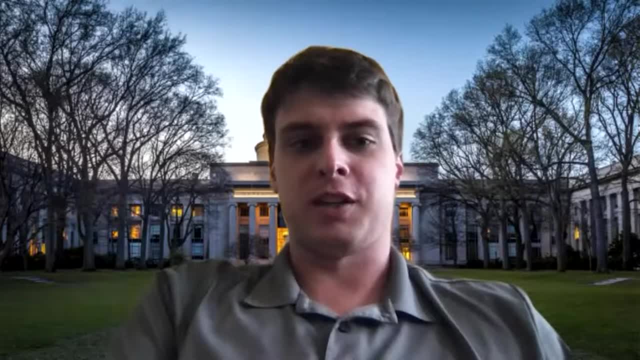 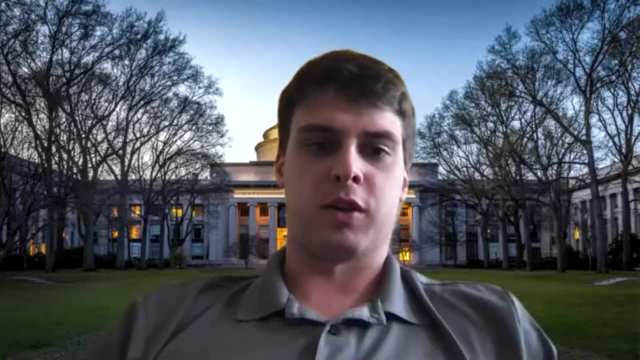 Where, maybe in adaptive control, you have some PID knobs that you just don't know what they are and you want to figure out the best values. So I think it would be cool- maybe something to explore in the future- of how to build that bridge even more. 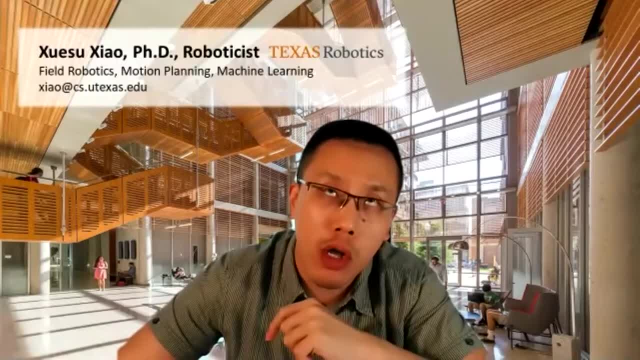 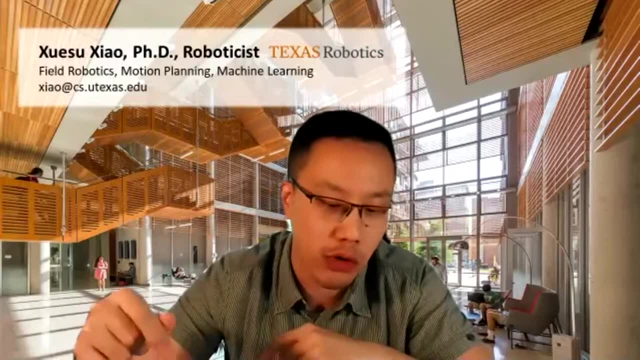 Yeah, definitely, definitely. Yeah, I would say probably from adaptive control. it's more kind of adaptively find those like correct values of those knobs autonomously, right? So we are here, We are trying to leverage human interactions, right. 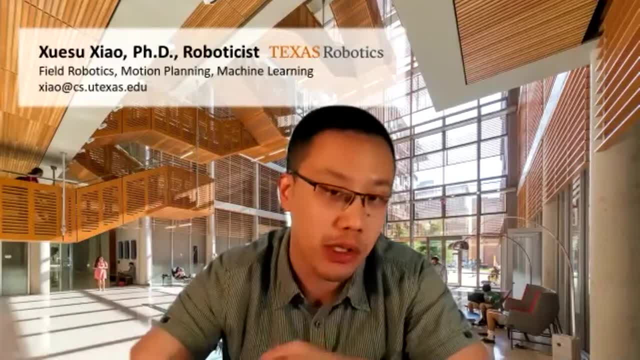 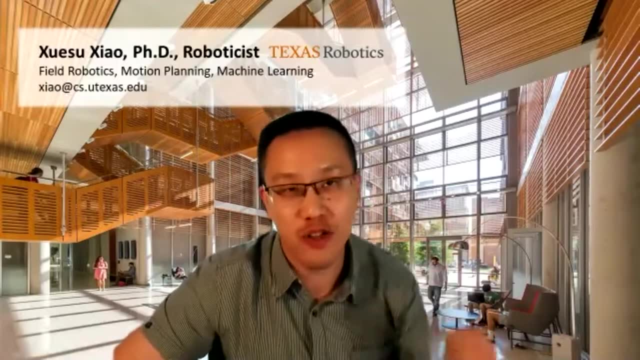 Different modality of interactions, because we are talking at field deployment. When you bring the robot to the field, you may not be expert Like we like as roboticists. we are very good like knob tuners: We can turn the knobs. 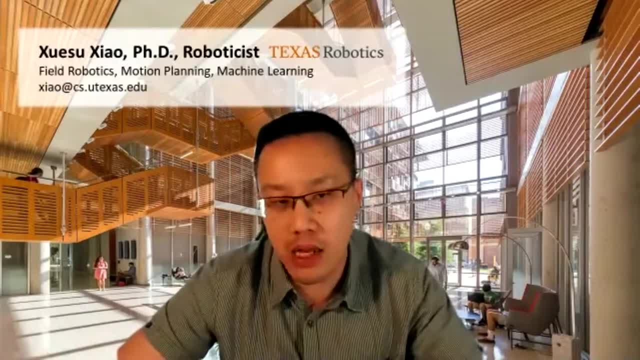 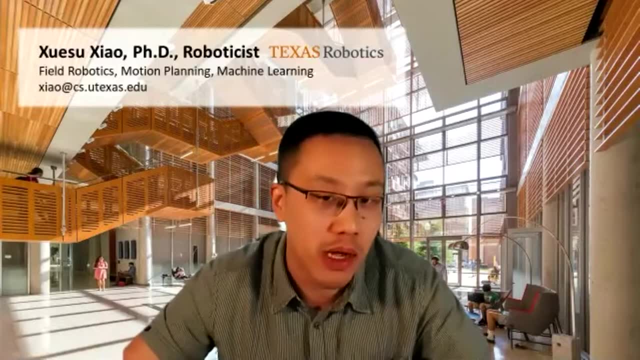 We have all our knowledge right, But not for, like, an end user, like from the general public. They do not know the underlying navigation systems, They do not know how to tune them, But giving them this suite of Apple methods. 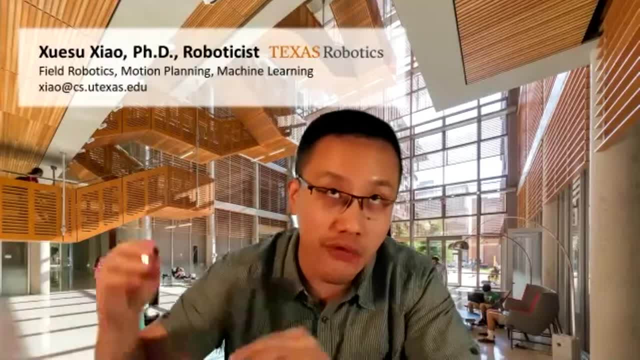 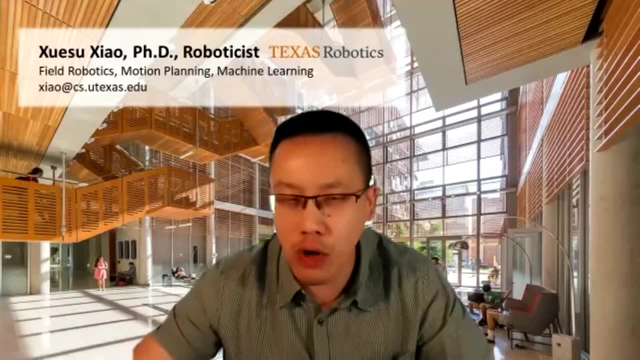 they can just use their like the interaction modalities of their comfort level. Like some are gamers, They can tally, operate like very easily. Some are not willing to take control of the moving robot using the joystick, Maybe just evaluate feedback. 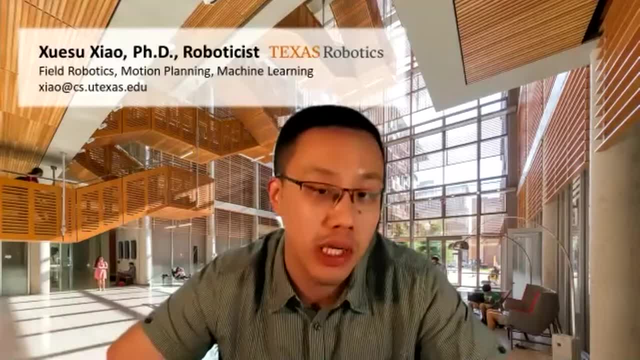 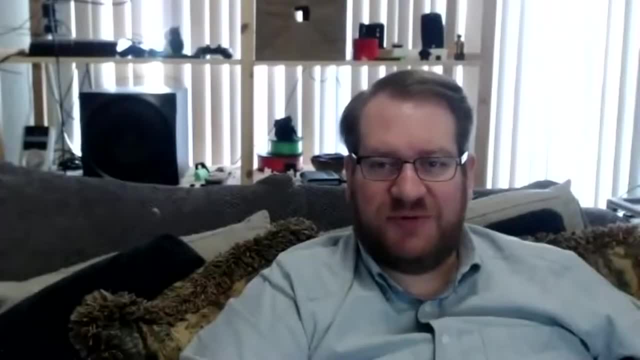 Good, bad, good bad, very good, very bad. That can also be leveraged in the field. Well, I hate to cut off a good discussion, but we're slightly behind schedule, So let's, let's, let's jump into our next talk. 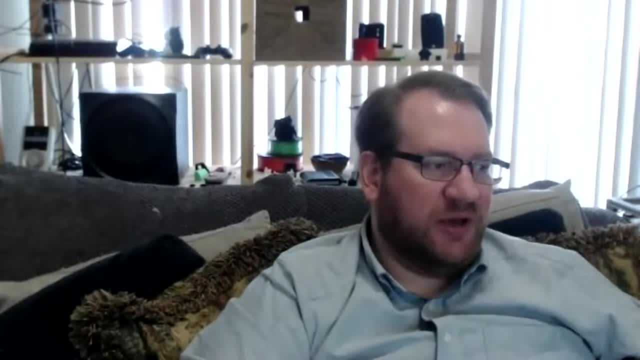 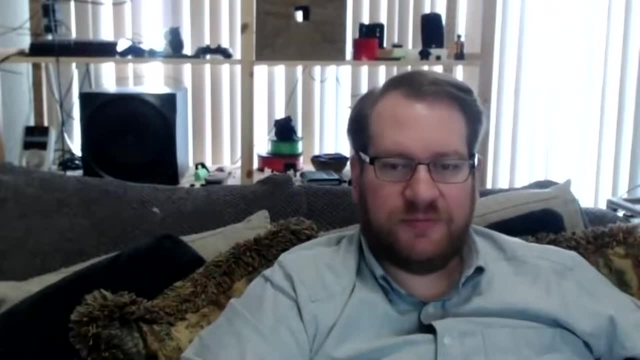 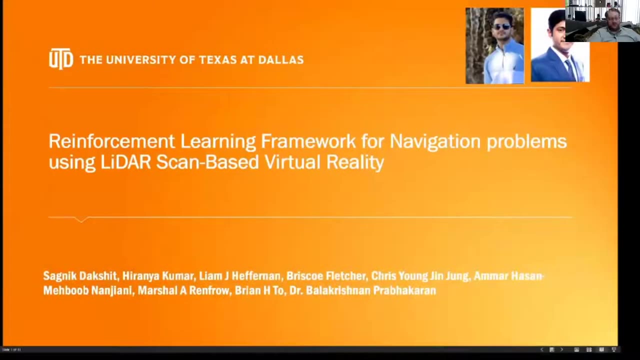 Our presenters are Shagnik Dakshet and Kiranya Kumar, And I'm going to go ahead and queue up this video. Hello everyone, My name is Shagnik Dakshet And today Kiranya Kumar, and I am going to present our work. 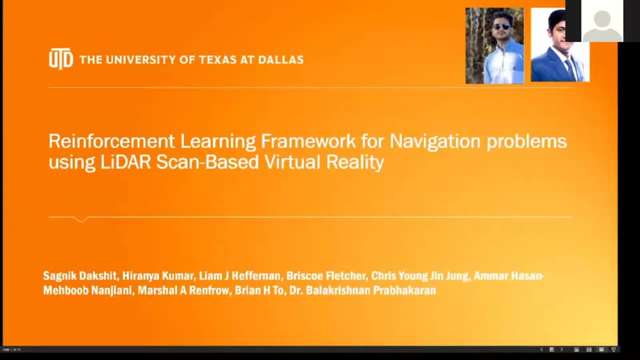 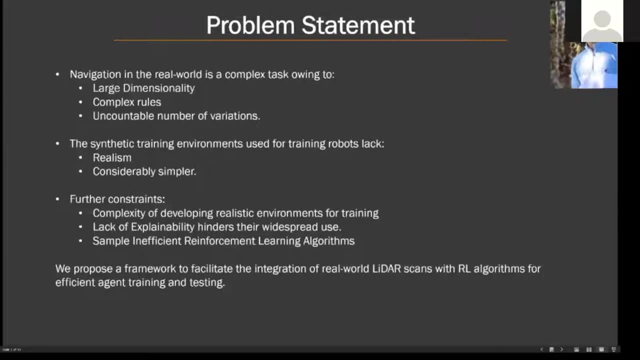 on reinforcement learning framework for navigation problems using LiDAR scan-based virtual reality. Navigation in the real world is a complex task owing to a number of problems such as large dimensionality, complex rule set and uncountable number of variations. Research in the same has made significant improvement. 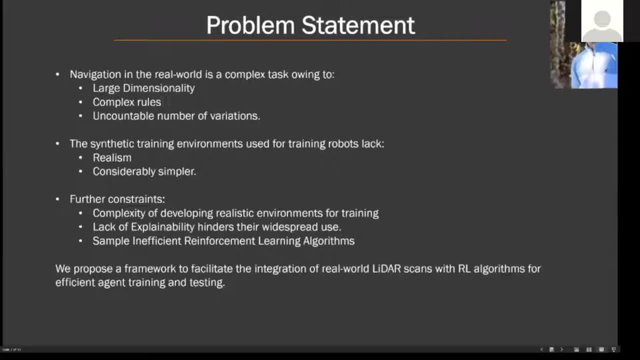 in training agents to perform automated tasks such as navigation. However, the state-of-the-art methods like reinforcement learning and imitation learning are limited by sample inefficiency and extensive computational resources. The black-box nature of such algorithms make it harder for society to accept. 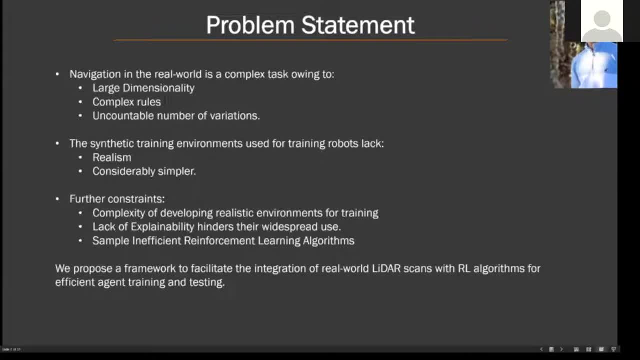 Furthermore, the synthetic environment used to train agents is considerably simpler and does not always represent the real world, which affects the deployment performance in the real world, which consequently hinders their widespread acceptance. We propose a framework to facilitate the integration of real-world LiDAR scans. 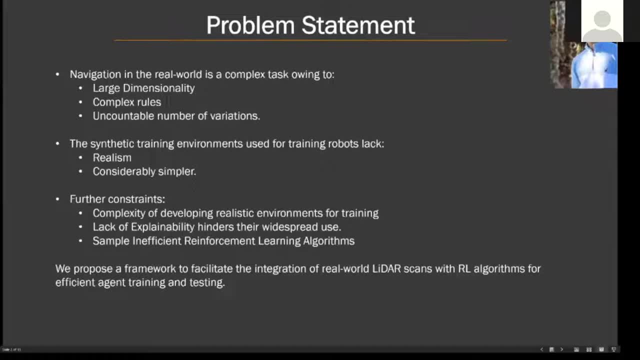 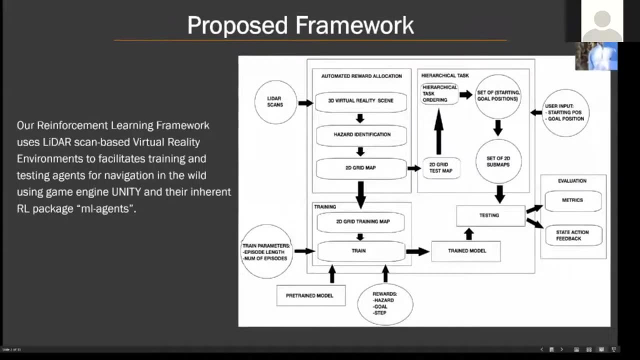 with reinforcement learning algorithms for efficient agent training and testing. We use LiDAR scans to articulately reconstruct real-world scenes in virtual reality. The depth information of the point cloud data is used to identify hazards and traversable paths by thresholding. this is from the motivation that, in bird's eye view, 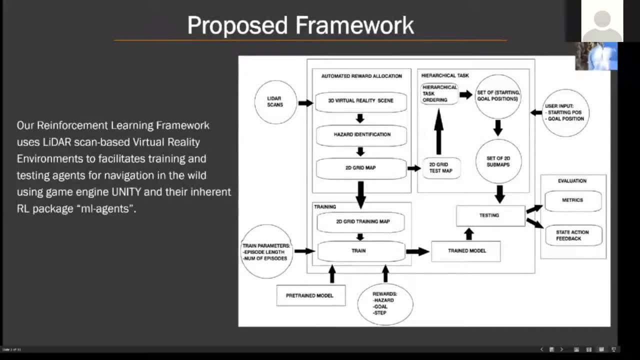 buildings and objects have a lower depth value in comparison to traversable paths. With this approach, we convert the 3D scans to 2D grid world. Once the hazards are identified, we mark and allocate reward values taken as user input, automatically to all hazards and traversable areas. 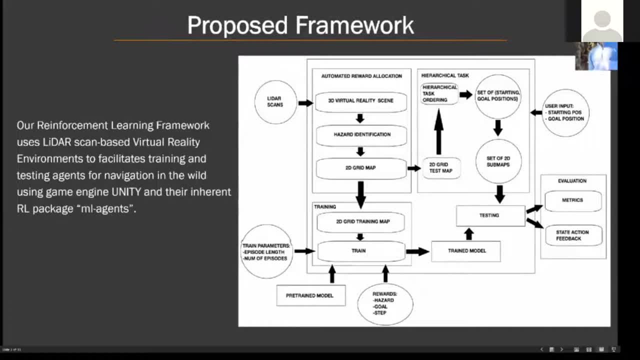 Motivated by our performance results on tasks constrained over a shorter distance and the intuition that learning to navigate around a city block is easier than navigating around a city. with the same rule set, we use hierarchical task setup for testing by breaking down a top-level task into subtasks. 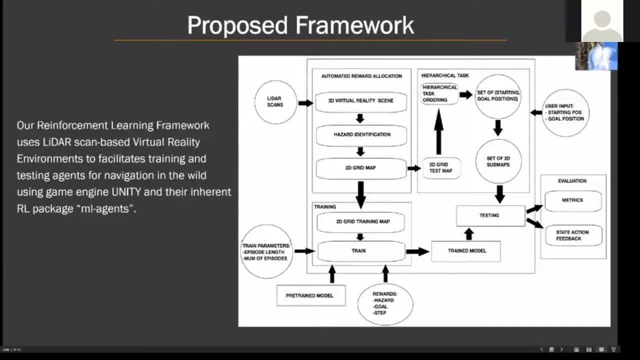 This boosts the accuracy by a lot on difficult cases, as we will see later in this presentation. We will explain easy and hard categorization of tasks in the next few slides. Our framework also provides feedback in form of state-action pairs allowing any end user or teleoperator. 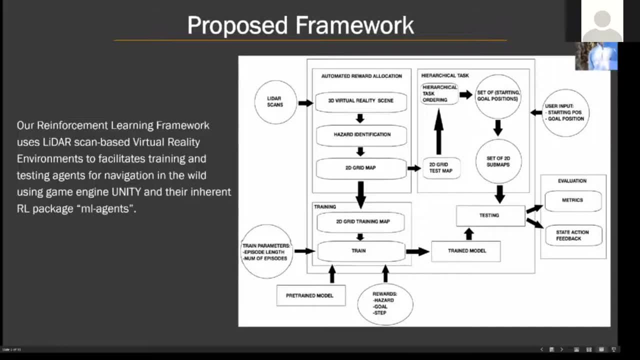 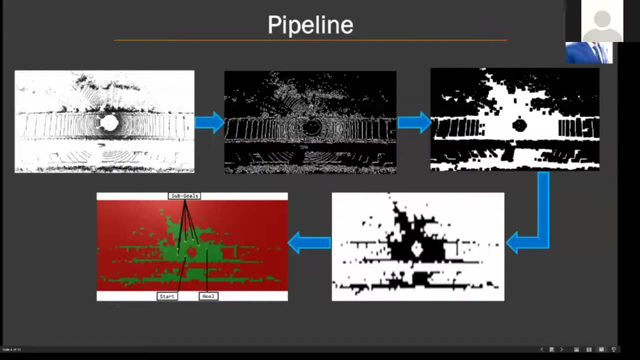 to monitor the autonomous agent. This also allows understanding of scenarios where the agent fails, for improvement of the reward structure and overall better training of agents. Here we are going to discuss the steps involved in generating a 2D reward map from a LiDAR scan. 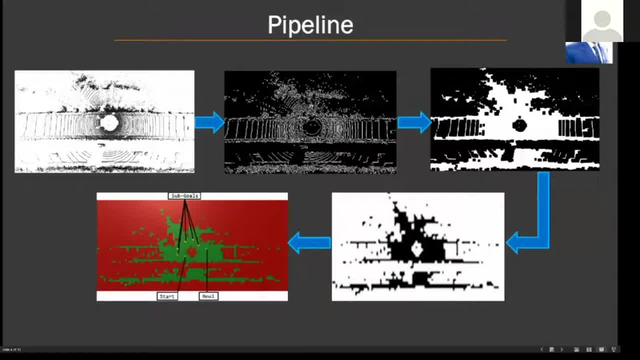 To generate a 2D reward map, we first create a depth map using the depth information from the LiDAR point cloud. The depth map is inverted to facilitate the next step, which is applying a canny edge detector on the depth map to detect significant differences in depth values. 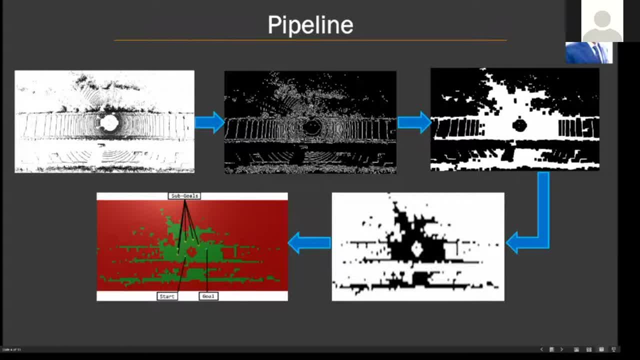 This helps us detect traversable paths in the map without the need of manually setting a height threshold for the ground level. After this, we apply a closing morphological operation with a dynamic kernel size dependent on the resolution of the depth map and the final output grid- world size. 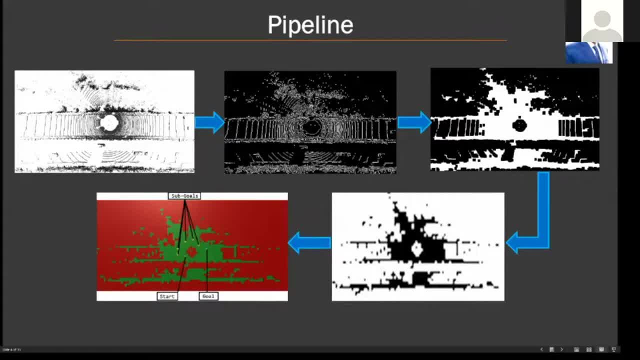 which in this case is 100x100.. The dynamic kernel size allows us to close up the small gaps between the LiDAR waves close to the source, without closing up the gaps produced by the objects, Since the source itself doesn't have any waves going through it. 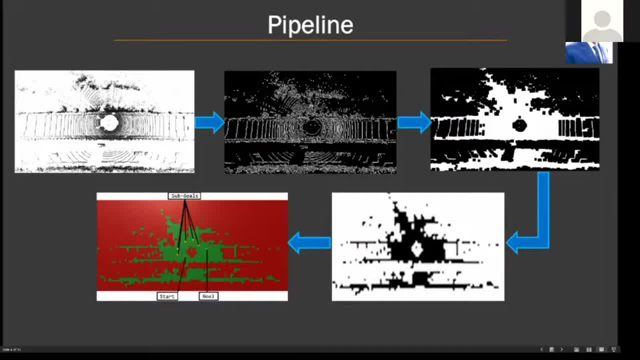 it is represented as a hazard in the final reward map. The image resulting from the closing operation is inverted and downscaled to the required grid size, which is then used by the Unity application as an input. The Unity application goes through the image and creates a map of normal and hazard tiles. 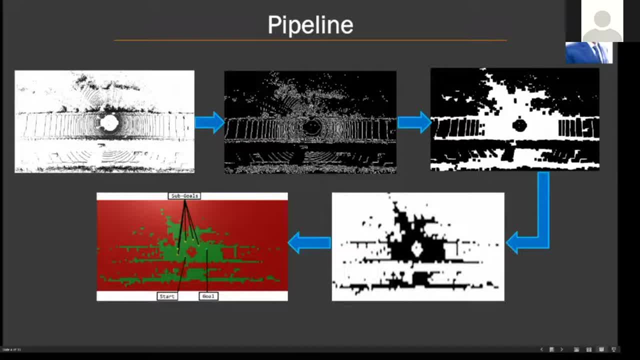 based on the pixel values. The goal, sub-goal and start positions are selected randomly from the list of normal tiles, which in this case are indicated by tiles in green. The tiles in red are the hazard tiles. A DFS algorithm ensures that the goal is reachable. 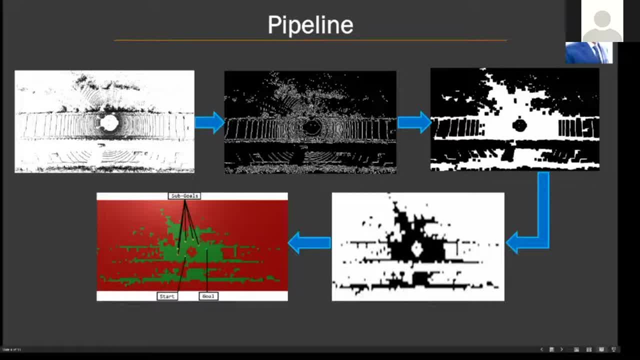 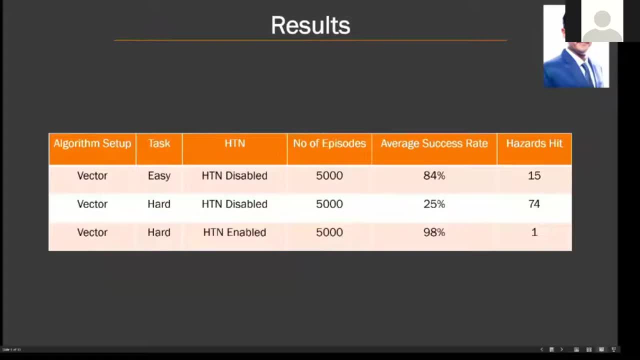 from the start position by checking if they are connected by normal tiles For testing. we break down the tasks into easy and hard categories. The difference between these categories is the distance between the start and goal positions. The distance is 4-6 tiles for easy tasks. 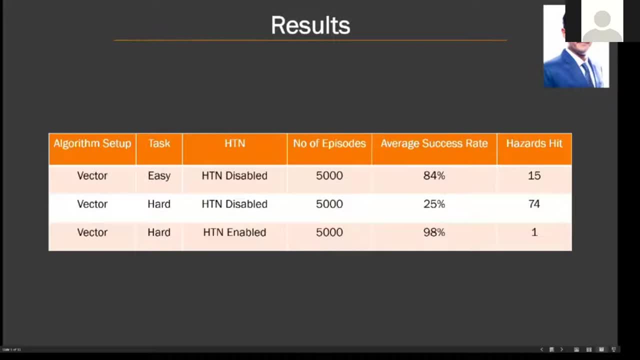 and 12-15 tiles for hard tasks. The exact distance between the start and goal positions in each episode is randomly selected between these ranges. Since the hazards between the start and goal positions are not accounted for in this heuristic, there are some cases where an easy task 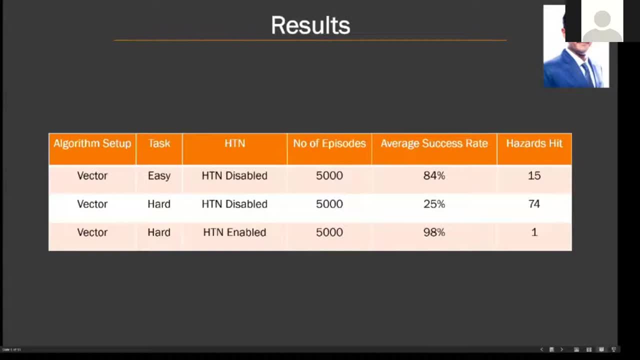 can actually be hard to navigate to due to hazards blocking the path. There can also be cases where a hard task can actually be easy to navigate to due to a direct, hazard-free path being present between the start and goal positions. The algorithm setup decides the input or feedback. 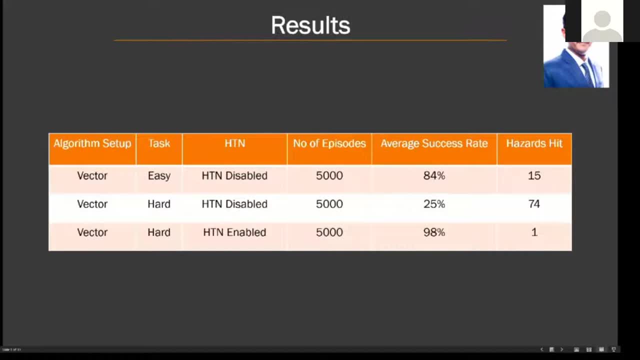 the agent is provided to make decisions for each step. For this test, we use vector inputs, which includes the difference between the goal and current position of the agent, as well as the types of adjacent tiles surrounding the agent. We measure the performance of the agent. 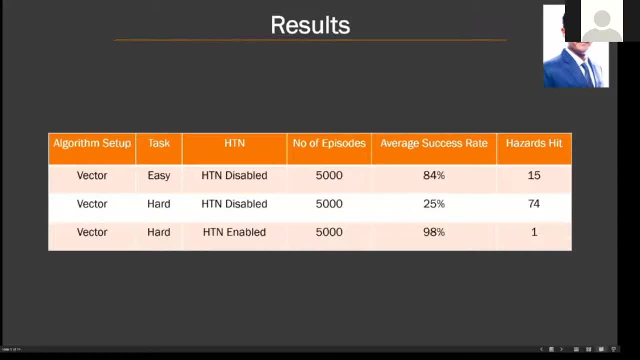 in terms of average success rate, which is the percentage of episodes in which the agent was able to reach the goal, and hazards hit, which is the number of episodes that ended due to the agent hitting a hazard. A low hazards hit number indicates the agent has learned to avoid hazards. 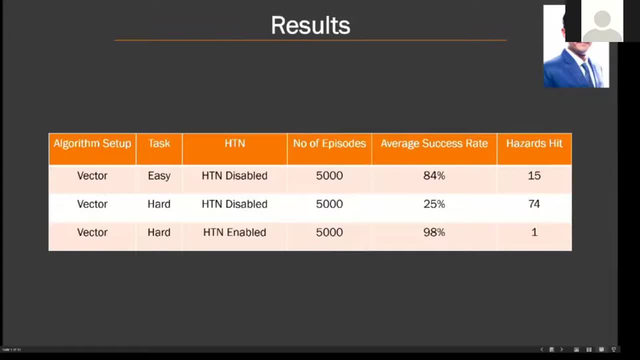 while a higher success rate indicates the agent has learned to navigate towards the goal While avoiding any possible hazards in the path. As you can see from this table, with HTN disabled we are able to achieve 84% success rate, with 15 hazards hit for easy tasks. 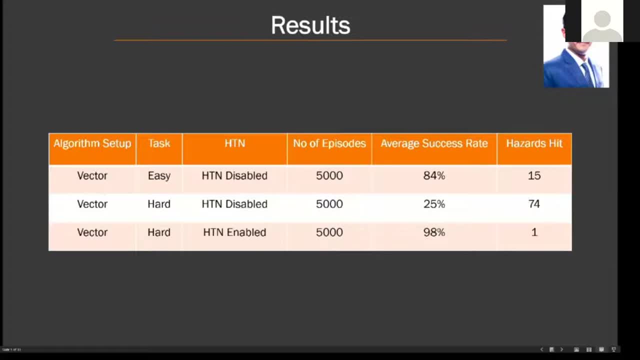 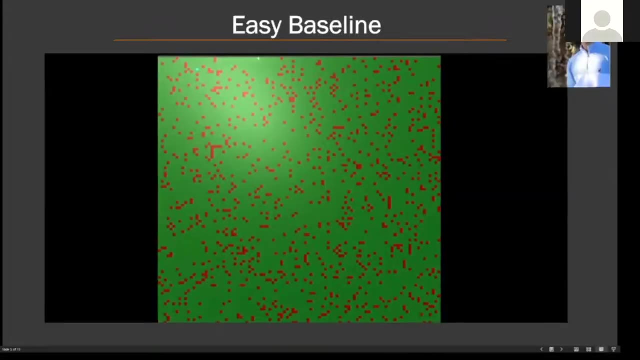 and 25% success rate with 74 hazards hit for hard tasks. With HTN enabled, however, we are able to achieve 98% accuracy with just one hazard hit for hard tasks. For comparison purposes, we generate synthetic maps with randomized hazards. 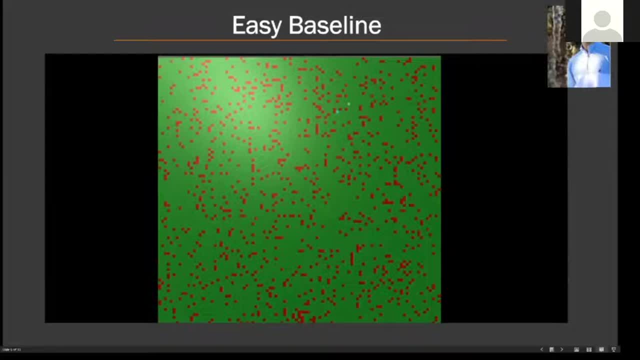 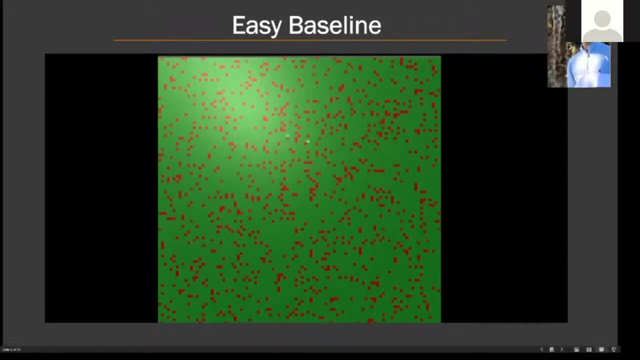 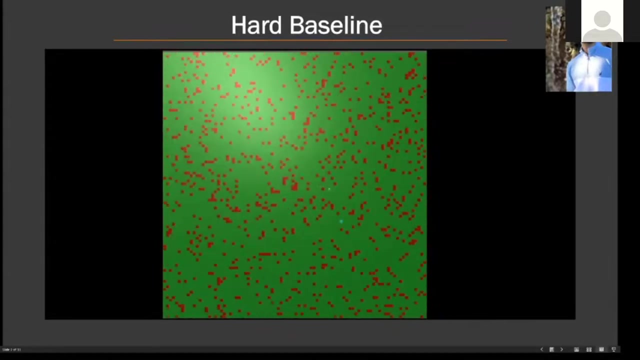 goals and starting position of grid size 100x100.. In this slide we present results for easy category. In this slide we present the comparative results for the hard category. As we can see, the agent never manages to navigate to the goal. 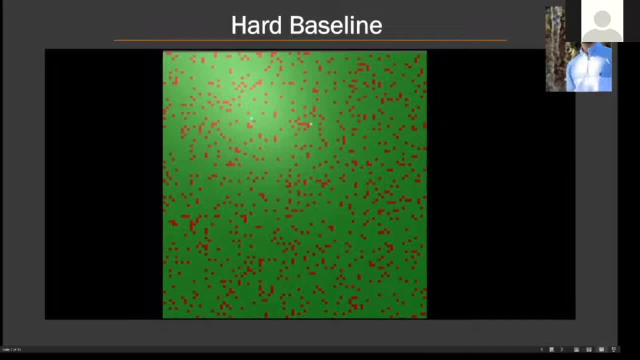 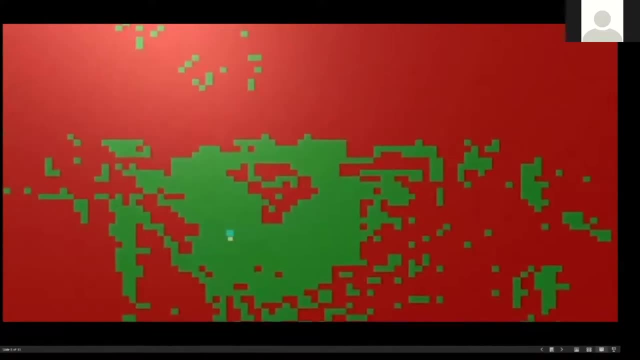 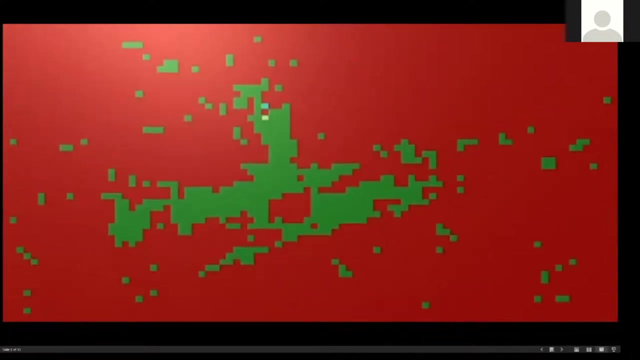 In this slide we present our testing results on the KITI dataset. for easy category, The blue grid represents the goal and the white moving grid represents the agent trying to reach the goal. In this slide we present results for easy category: The blue grid represents the goal. 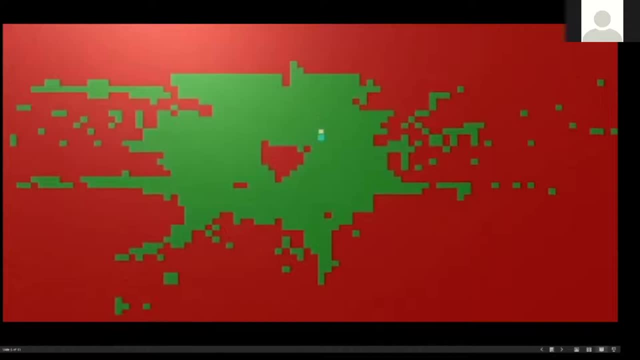 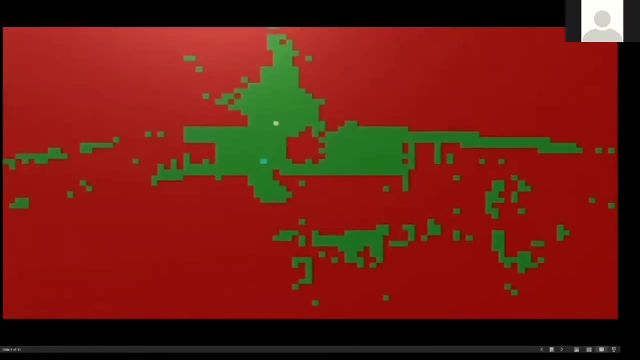 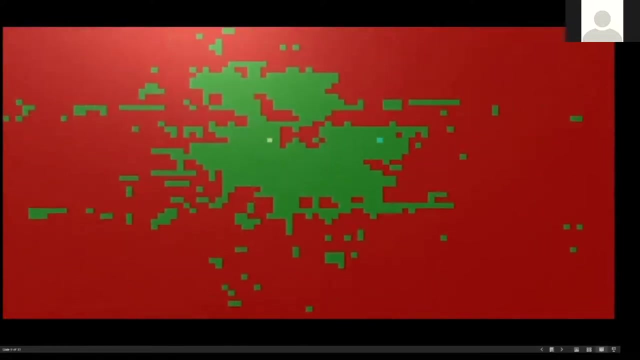 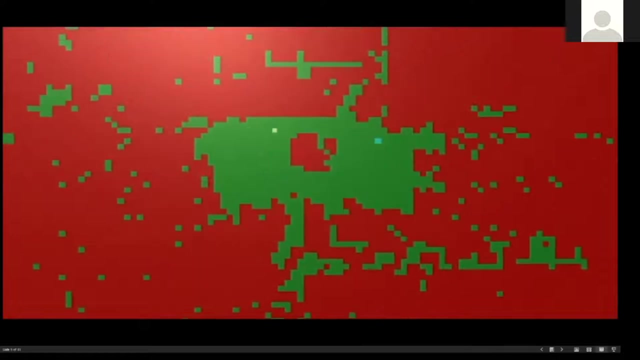 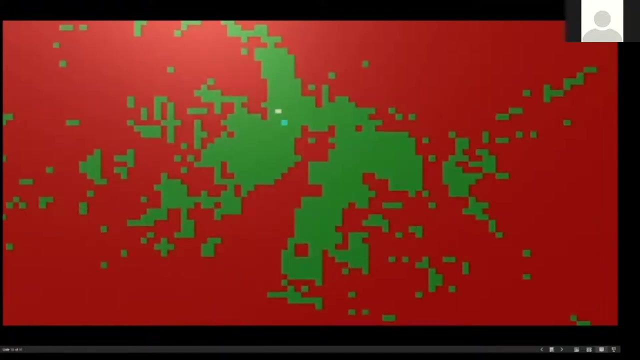 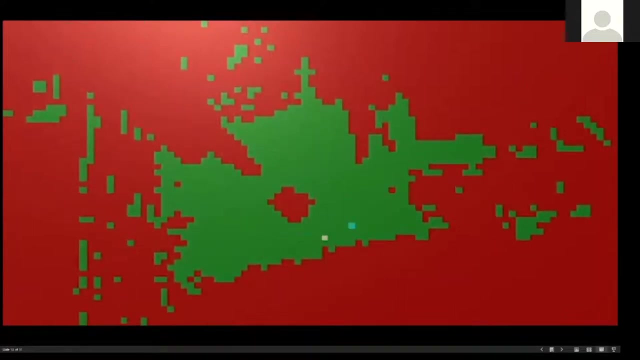 and the white moving grid represents the agent. in this slide, we present our results on the hard category without hierarchical testing setup. we present our results on the hard category with hierarchical tasks enabled. as we can see from the video, the agent almost always reaches the goal through this hierarchical setup. 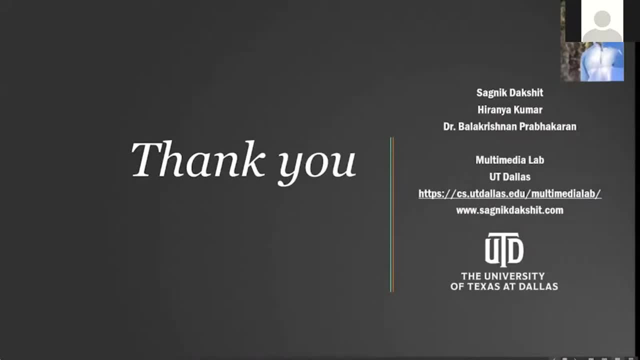 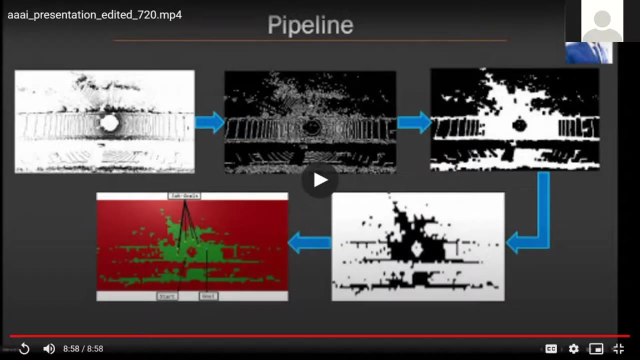 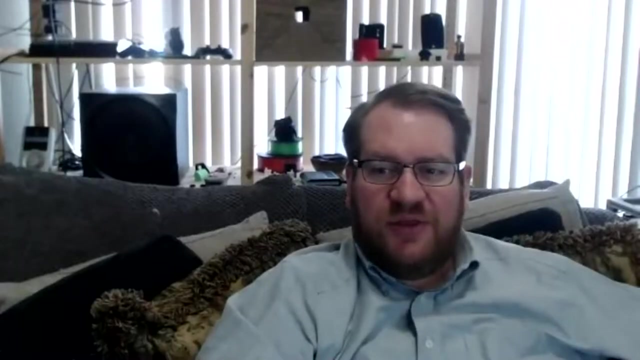 as future work, we plan to extend the framework to accommodate frontal view navigation as seen in autonomous vehicles, and implement strategies to make reinforcement learning, training, more data efficient. thank you, and now we will move on to the next slide. all right, well, let's uh, thank our speakers and open the floor to questions. 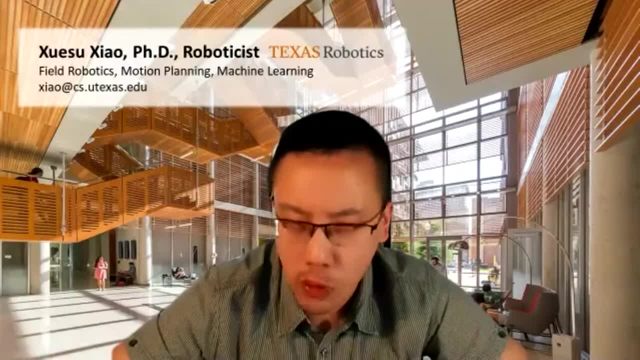 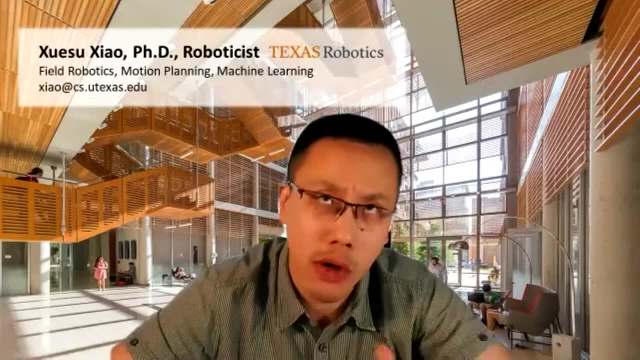 do we have any questions for our speakers? i have a minor question, uh, regarding one figure in slide four. so the you are trying to find the next slide to generate this grid word using lidar scans, right, so why is the center of the robot? i know it's not. 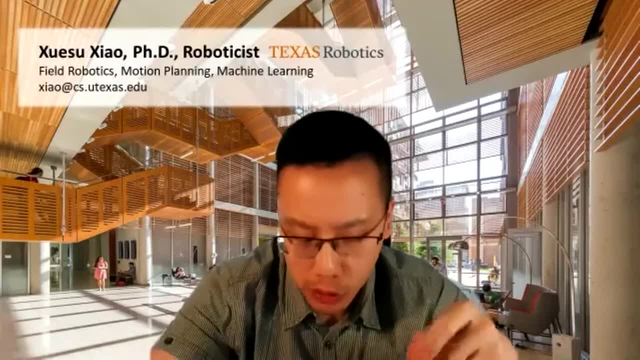 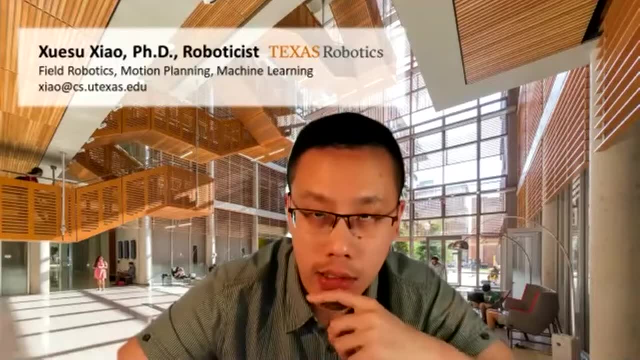 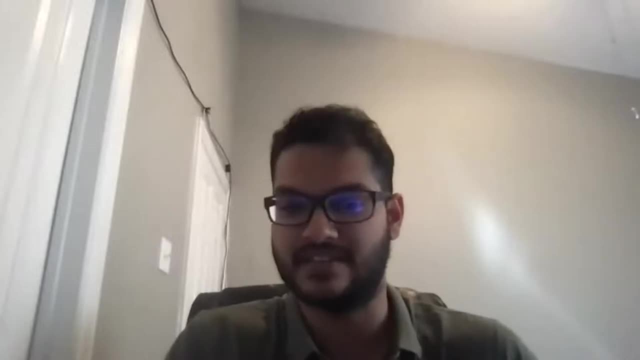 perceived by the lidar, because that's where the lidar is. you also have the center of the- the lidar- as red. that's kind of like the dangerous spot. can you explain why that so? since with the lidar data did not have any data in this 360 degree camera setup, we just gave it as a dangerous. 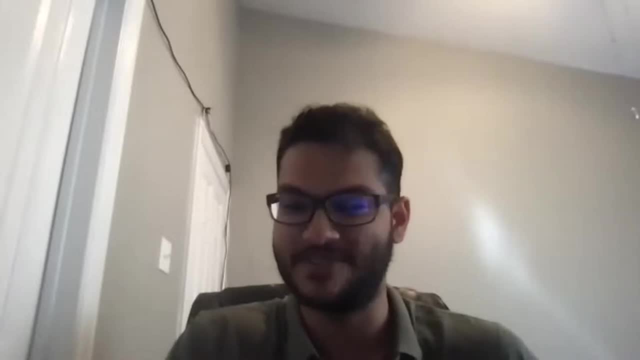 path. i mean, there is no particular reason to making that red. we can make it green as well. you can just easily make it green because you know that's where the ladder is at. that's yes, but the lidar is again on top of a car, right. 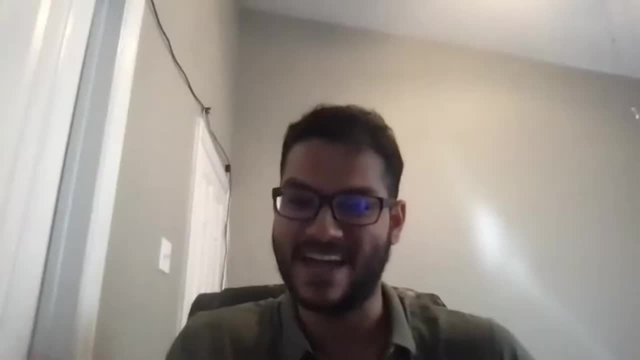 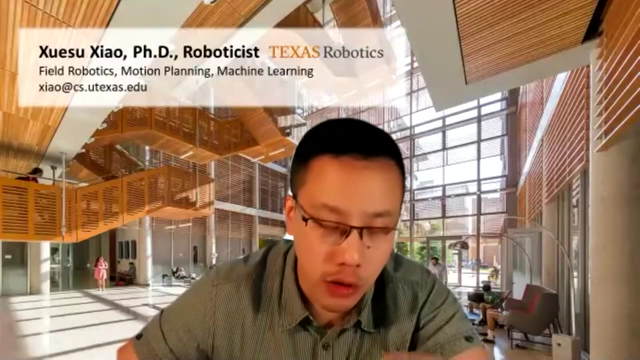 assuming. so the car itself will have some distance front and back, so we didn't want to bump into the car also, so we thought it's safer to give a barrier there, okay, okay. now all these other so you showed in the video print like video demonstration or the the robot moving. those are 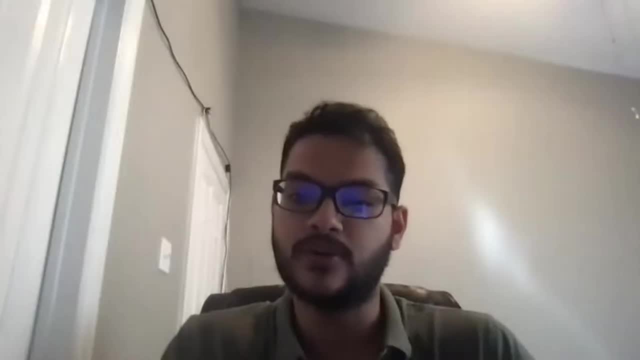 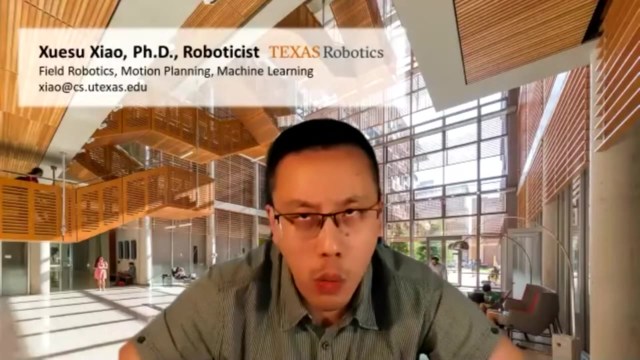 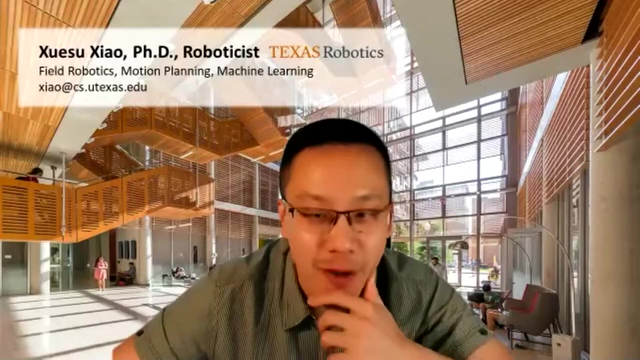 from kids data set. yes, the first two were for baseline in in the baseline we randomly generated hazards and the others were from the kitty data set. okay, okay, so what is the training algorithm you're trying to use? we use the approximate policy optimization, thank you. yeah, thank you. 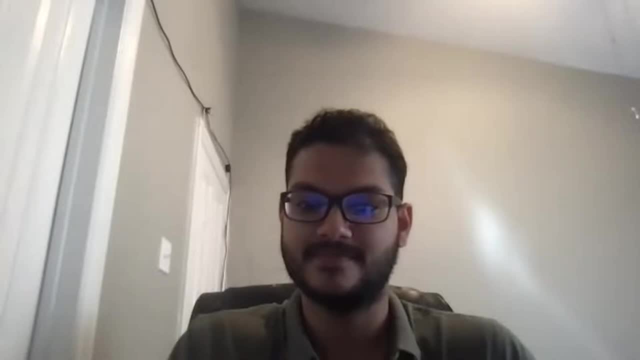 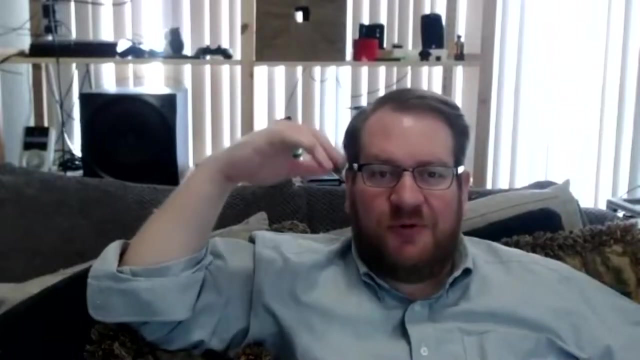 do we have any other questions? so you kind of have this like hand generated way of pre-processing your map, right? is there the possibility of plugging in any of the other existing tools out there that output, like you know, a slam map or um, you know, um, maybe even? 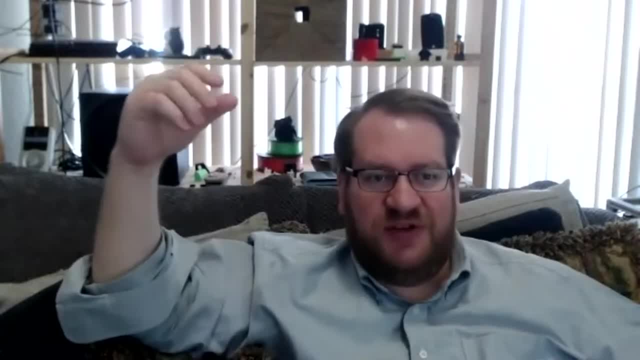 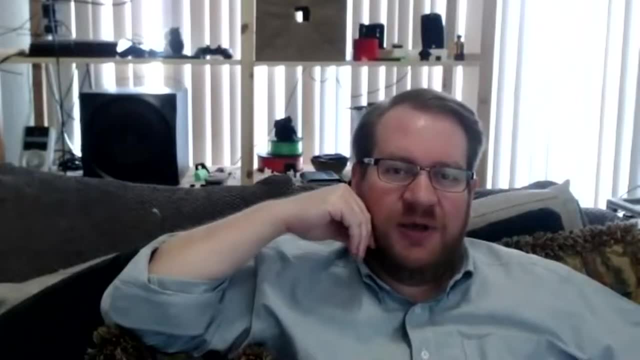 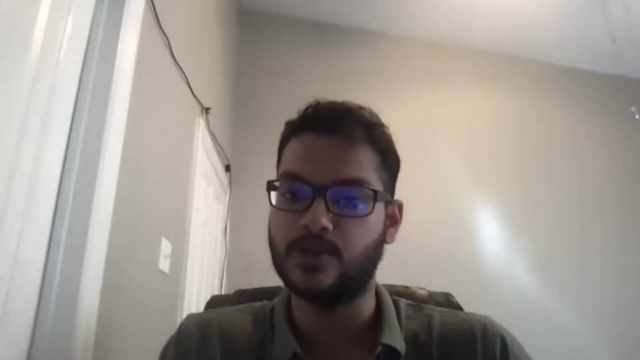 point cloud stitching and you know watertight surface, fitting type things uh to as your pre-process rather than your sort of hand-engineered one. so we tried some automated tools. but since we are doing the, we are taking the point cloud's depth value to create the hazard map. 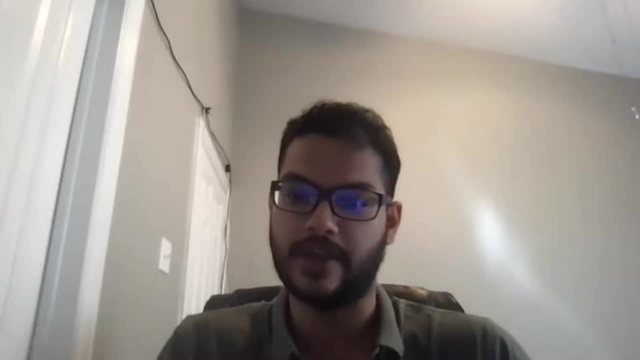 the pre-processing steps need to be there to get that depth value accurately. otherwise if you use existing software, some of them are giving me weird depth values. so in future we'll try to automate it, but for now we have to use this processing steps exactly. well, that makes. 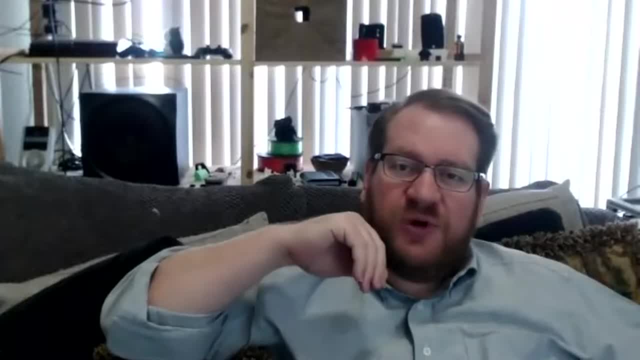 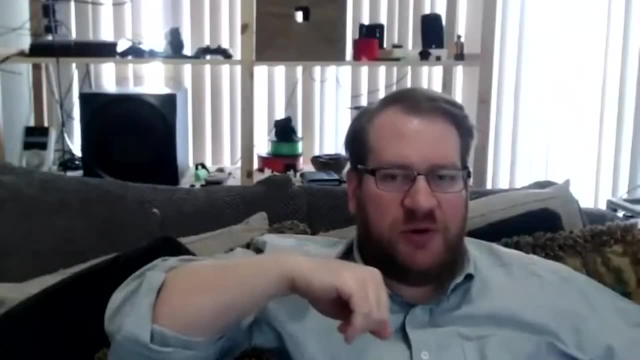 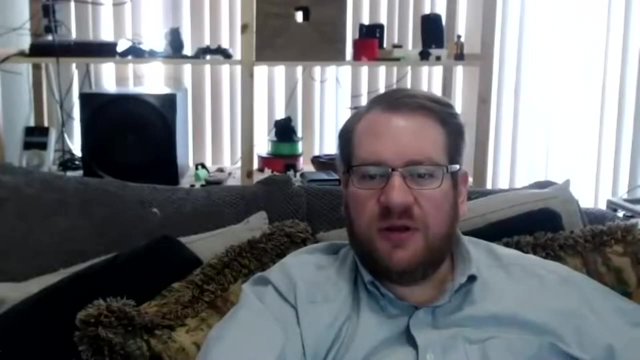 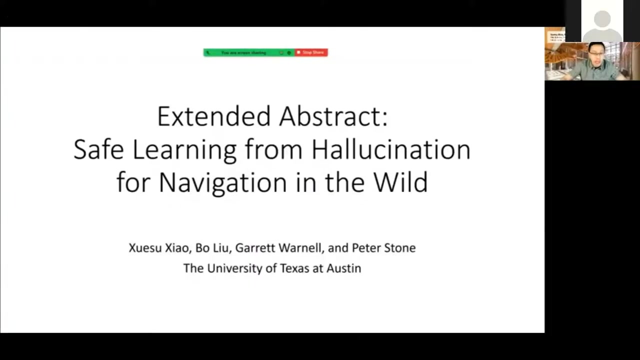 a lot of sense. all right, do we have any other questions for our speakers? well, uh, our next one is. our next speaker is we tribe, who i think everyone knows at this point. uh, i'm going to go ahead and view up his presentation. so, hi everyone. this is our estimated abstract. safe learning from hallucination, or lfh for navigation in the wild. 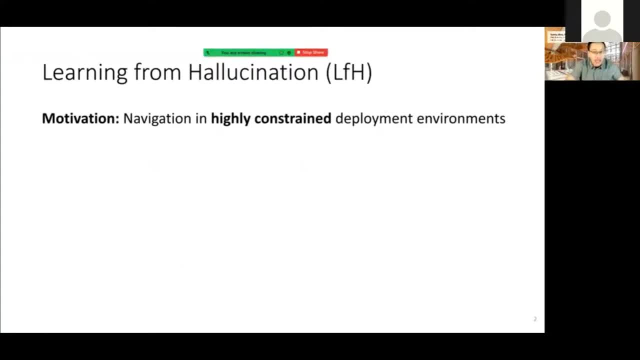 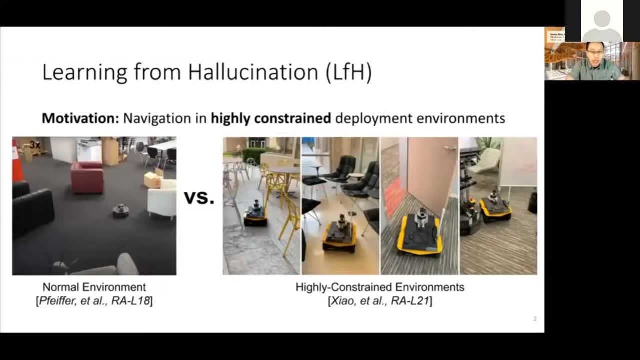 the motivation for lfh is highly constrained environments, when the robot needs to engage in agile maneuvers to squeeze out a fantastic variable- bredилиvenent nie de thou- between obstacles. a contrast between a representative, normal cluttered environments existing mobile navigation approaches have addressed, versus the highly constrained. 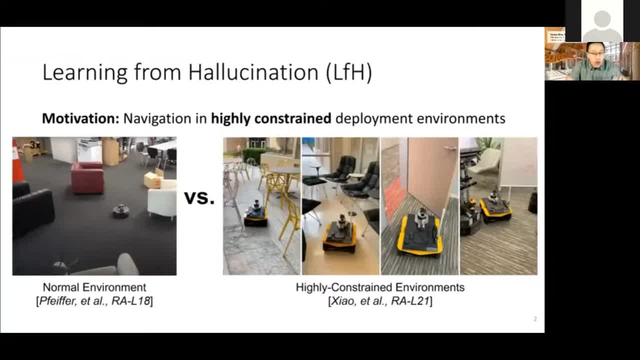 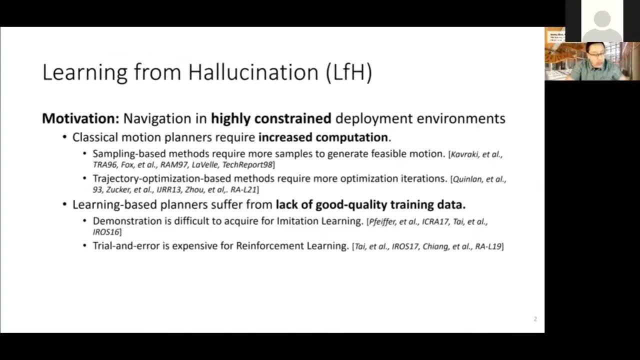 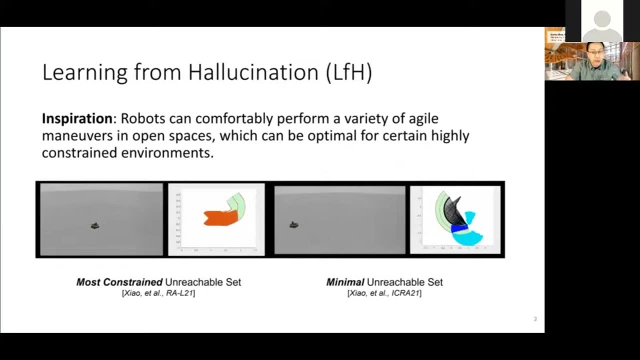 environment lfh is designed for those places will cause trouble for classical motion planners because they will require increased computation. however, learning-based methods do not make things easier either, due to the lack of good quality training data. lfh's inspiration is that robots can comfortably perform a variety of agile maneuvers in open spaces. those maneuvers 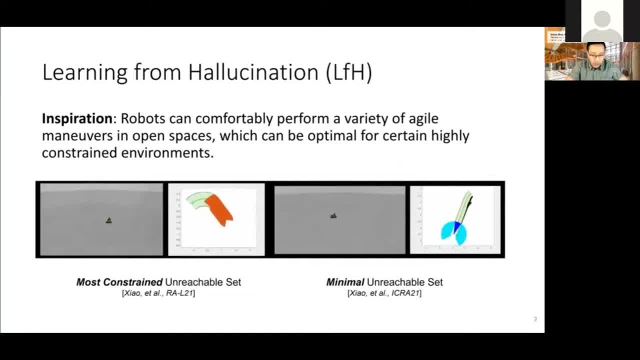 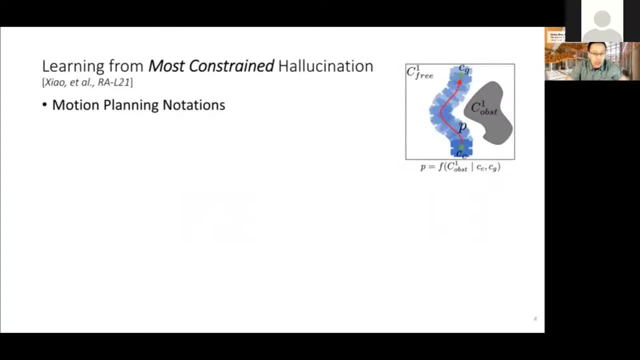 owned by spaces can be optimal for certain highly constrained environments by generating- or we call it hallucinating- those spaces. we have quite many training data. today i'm going to talk about two hallucination methods. the first method is to hallucinate the most constrained, unreachable set some notations in motion planning. we are dealing with the configuration, space c. 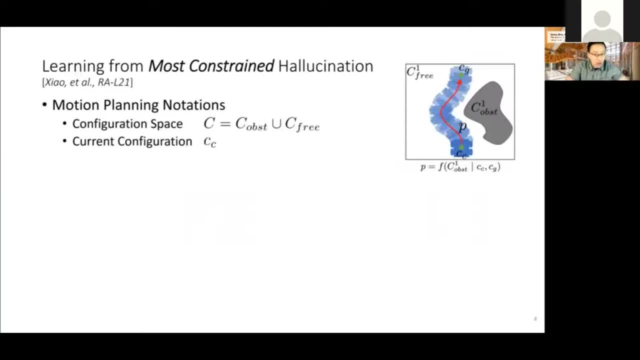 composed of obstacles: c obstacle and free spaces- c3. the robot locates at the current configuration cc and wants to go to the goal. configuration cg. the robot can take action u at each time step, such as linear, angular velocities. a sequence of actions comprises a motion plan, p, a motion. 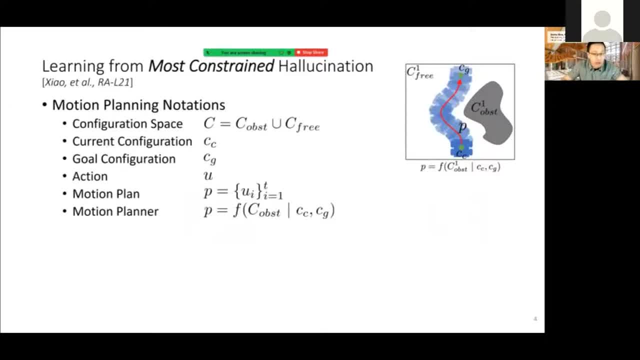 planner is basically a function f that maps from obstacle configuration to an optimum motion plan, given current and goal configuration. the motion planning problem is to find out function f. in this lfh we propose to investigate the inverse function of f. so, given an optimal plan p, what is the? 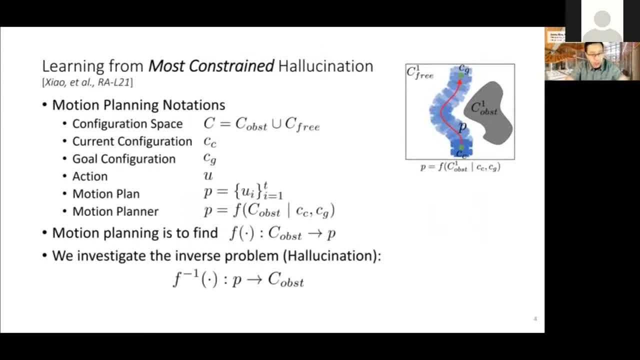 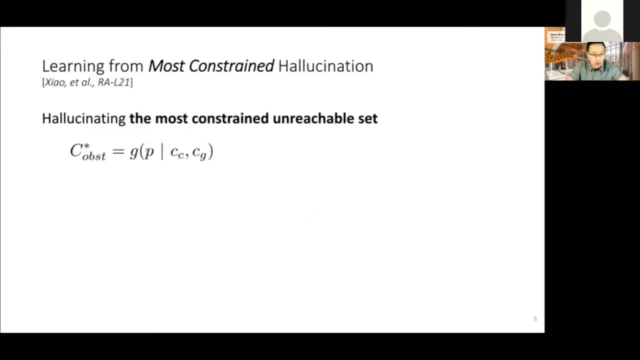 obstacle configuration- c obstacle, which is an easier problem. unfortunately, this inverse function is defined because multiple obstacle sets can map to the same optimal motion plan. as you can see on the right to address this issue, we introduce the idea of the most constrained and reachable set- c obstacle star, in order for an unreachable set to be the most constrained, unreachable set for any. 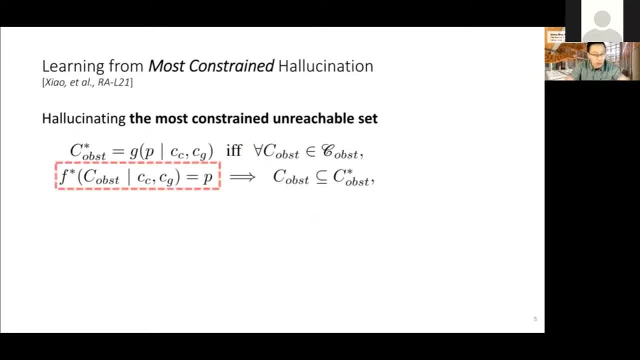 unreachable set that will cause the optimal motion plan p. this unreachable set will belong to the most constrained unreachable set. so, basically, the most constrained unreachable set is the obstacle set that contains all other obstacle sets that make the plan optimal. for example, c obstacle one and c obstacle two. both lead to optimal plan p. the union of all these obstacle sets with optimal plan. 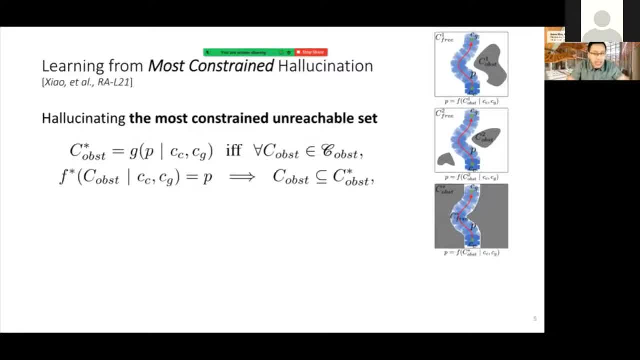 p is c obstacle star. so it is not possible to add even one more single obstacle in the most constrained obstacle set without invalidating the optimal plan p. there we can train a function approximator, for example using a neural network to map from the most constrained, unreachable set. 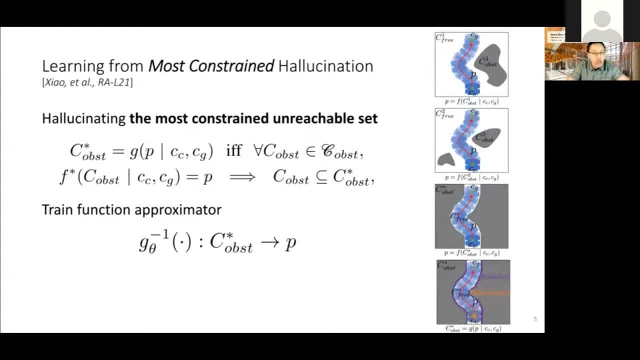 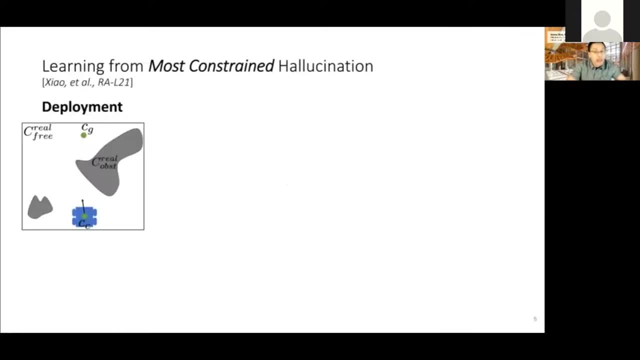 to the optimal plan. the specific instantiation of the most constrained, unreachable set can take the form of, for example, light out scans or depth images. during deployment, the robot faces the real obstacle configuration. but the robot has only learned how to react to the most constrained spaces during training. 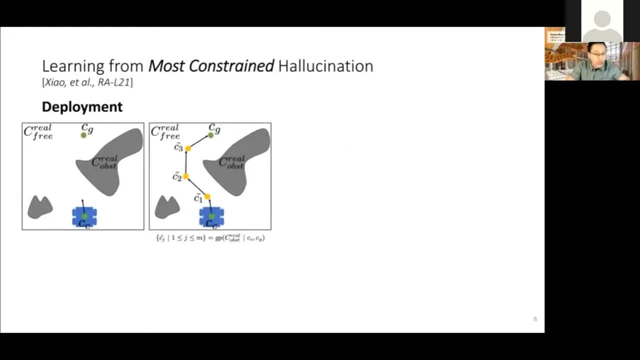 this is where we actually utilize the global planner gp. in a classical navigation system, the global plane is usually a few rough waypoints the robot should reach in the future, mostly in a lower dimensional workspace, for example, ignoring orientation. we utilize these rough waypoints on the global path to generate the most constrained, unreachable set and also to 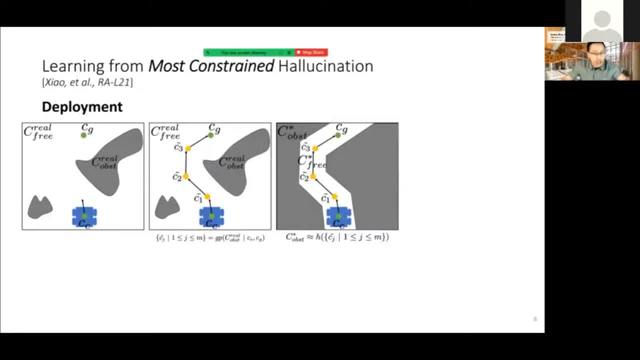 generate runtime hallucination and then query our trained g-1 function to produce motion plans during runtime. to deal with uncertainties during deployment, we add gaussian noise to the produced motion plan and use a forward prediction model to predict where the robot would be after executing the motion. we compute what percentage of the perturb. the motion plans were called inflation. 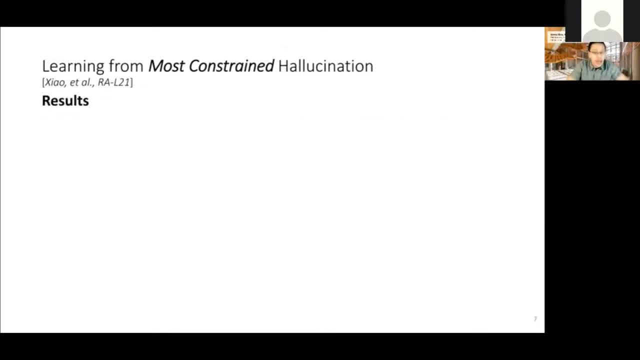 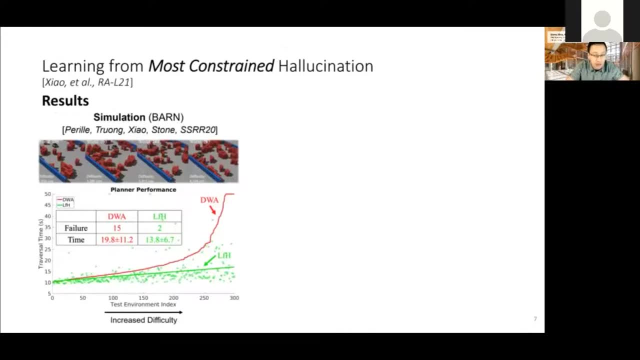 and then adjust the speed correspondingly. we implement the alfh idea on a jackal ground robot in the simulated barn dataset with 300 environments randomly generated by cellular automata. As you can see, DWA's traversal time significantly increases, with increased difficulty since it 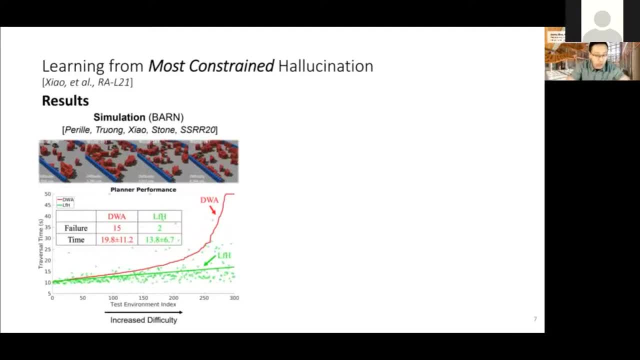 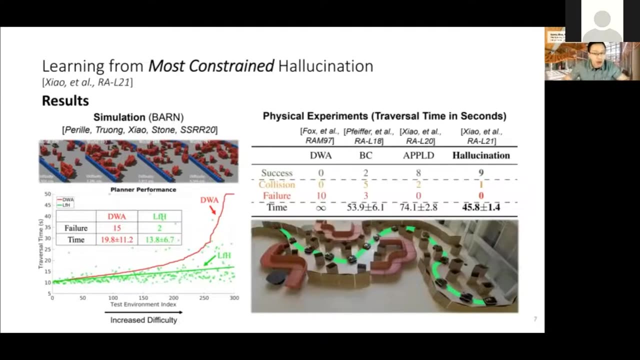 fails to sample feasible motions in the highly constrained workspaces and gets stuck. very often, LFH computation is simply creating the runtime hallucination with the global path and then querying a pre-trained neural net which is not dependent on how confined the real environment is. We also implemented LFH on a physical Giacomo robot. 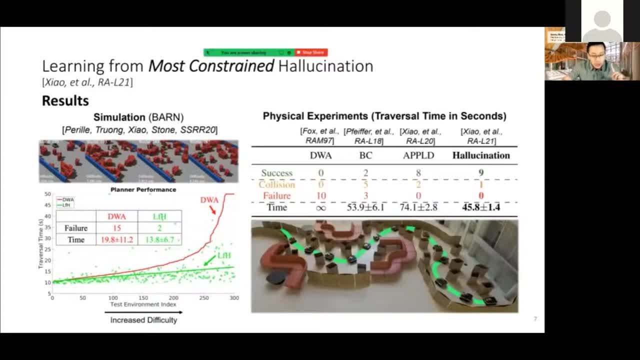 In addition to DWA, we also compared to a state-of-the-art and BC behavior cloning approach and our previous L4D approach. As you can see, hallucination achieves the shortest average traversal time and the smallest variance. These videos show the LFH performance in natural. 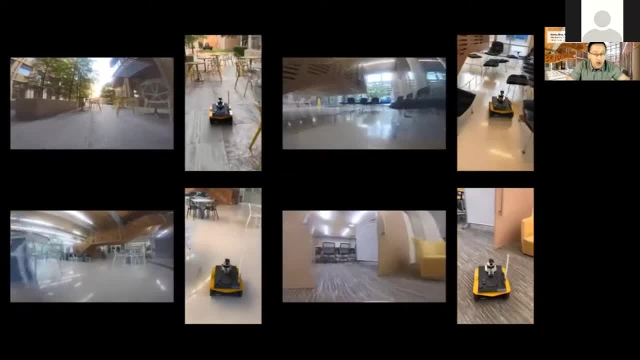 cluttered environments. Remember that the robot does not require any human demonstration for the learning and it has never even seen a real obstacle during training. But during the training, the LFH performance in natural cluttered environments is very high. During the training, the LFH performance in natural cluttered environments is very high. 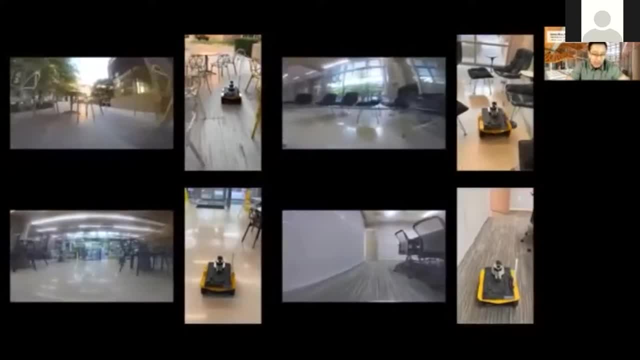 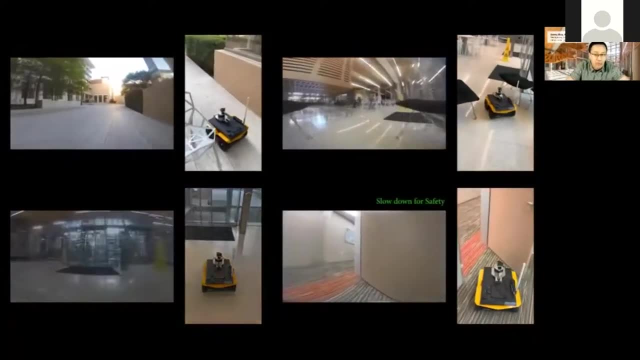 During the training, the LFH performance in natural cluttered environments is very high. During deployment it can negotiate through those highly constrained spaces. Note how close the robot is to the obstacles in some frames. These places will require classical sampling-based and optimization-based methods, a lot of samples and optimization integrations. 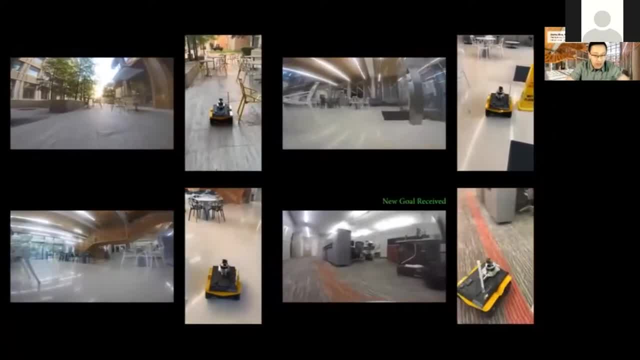 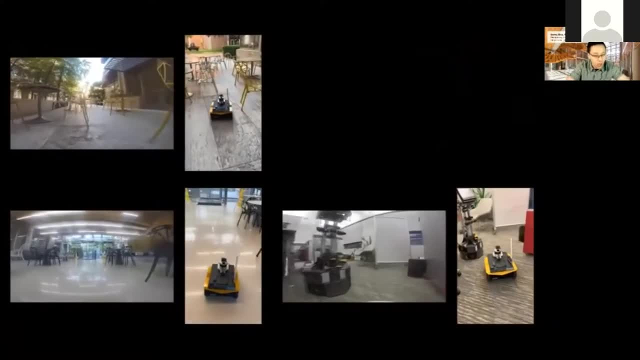 until it can find a feasible motion plan. But for LFH the computation is simply constant and it can maneuver through those challenging spaces without any problem. For LFH, the computation is simply constant and it can maneuver through those challenging spaces without any problem. 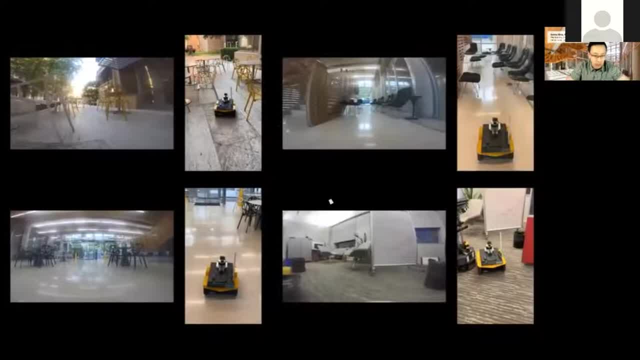 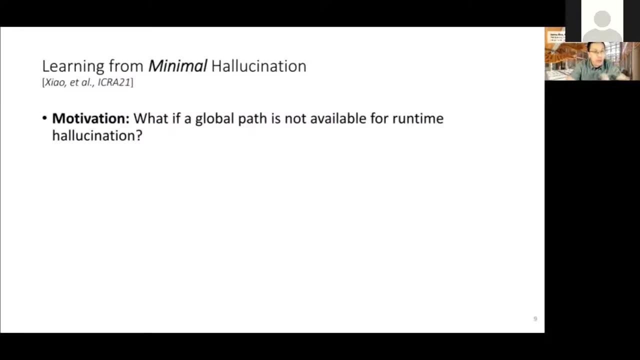 For LFH, the computation is simply constant and it can maneuver through those challenging spaces without any problem. Sorry about that, folks. let me uh, oh, there we go. our second approach is to address the problem that sometimes a global path is not available to generate the mental hallucination. 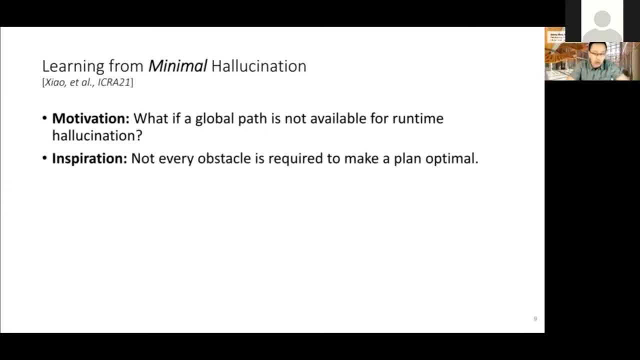 this is the version of our second. learning from minimal hallucination approach is that in the most constrained obstacle set, not every obstacle is required to make a plan optimal. therefore, we can identify a minimal and reachable set randomly sample obstacles. in addition to this, this minimal set during training to generalize for many real-world obstacle configurations. 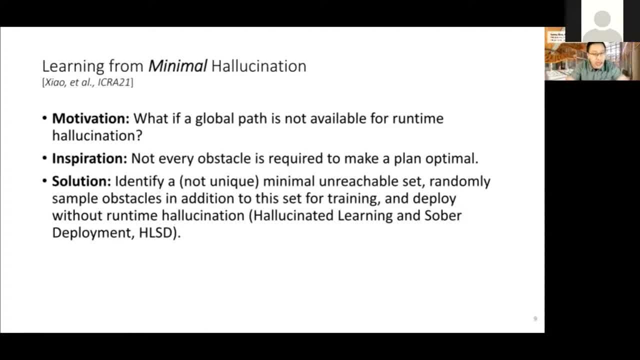 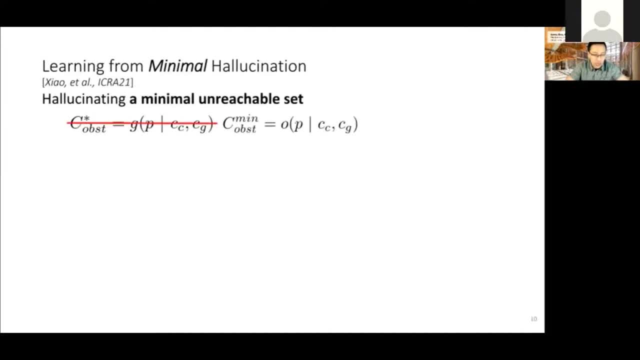 and then deploy without runtime hallucination. We call it conditional learning and stupid deployment, or HRSD. So instead of the most constrained unreachable set, we define a minimal unreachable set For minimal unreachable set. C- obstacle min for any single obstacle. configuration C in C: 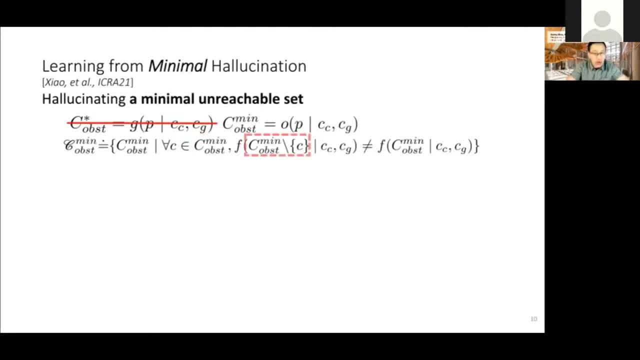 obstacle min. removing it from this set will cause a different optimal plan. I will use the point mass holonomic robot, which follows the Charlotte's path principle, as an example. Let's look at this graphical illustration: Assuming the robot locates at CC and wants to go to CG Instead of a straight. 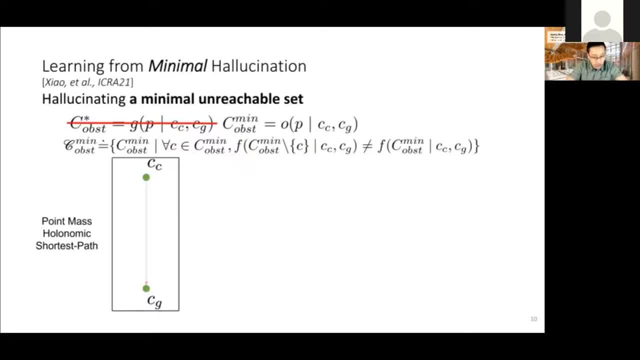 line, which is obvious in Charlotte's path it actually takes a D to work through CM. Why is CCCM-CG the optimal path instead of the straight line CCCG? It is because of some obstacles. One example: obstacle set is shown as the black line. It starts from CM and ends at some point: CE. 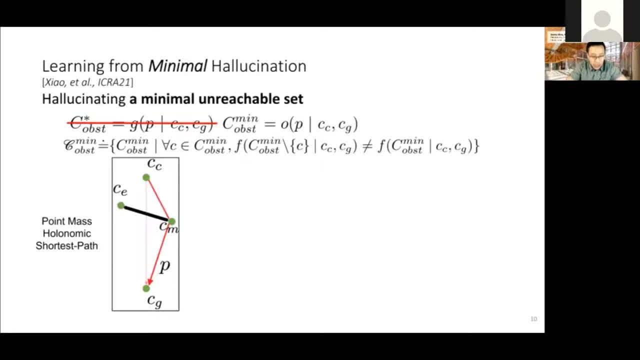 Apparently it blocks the Charlotte's straight line path, CCCG. But you also need to make sure there's no other Charlotte paths than CCCM-CG. So on the other side you will need CE to locate on the ellipse where the focal points are CCC and CG, So CCCCG. 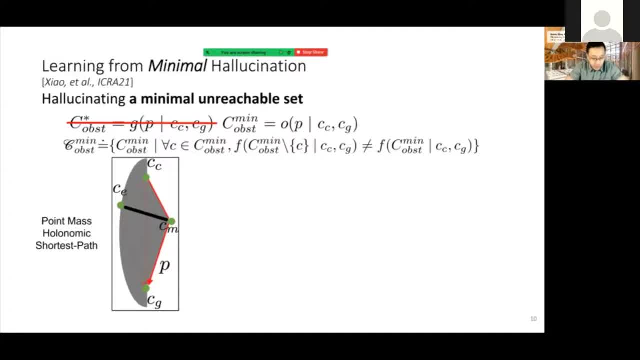 has the same length as CCCM-CG per definition of ellipse. As you can see, if you drop any of the obstacles on the black line, such as this arbitrary chosen C, CCCM-CG are not an optimal path to go from CCC to C anymore. You can actually go through that, drop to obstacle C and have a. 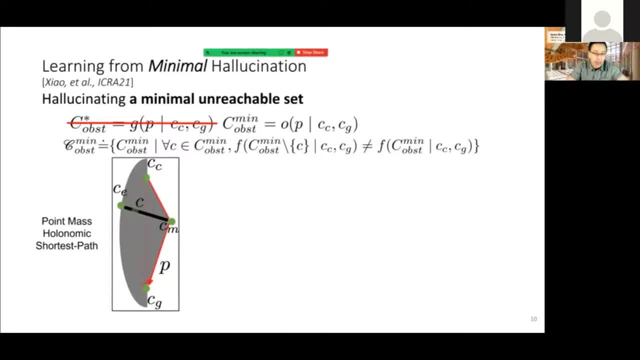 Charlotte path So you cannot drop any obstacles on this ellipse. So you can actually go through that, drop to obstacle C and have a Charlotte path. so you cannot drop any obstacles on this ellipse black line and therefore it is a minimal original set, although there are many other minimal. 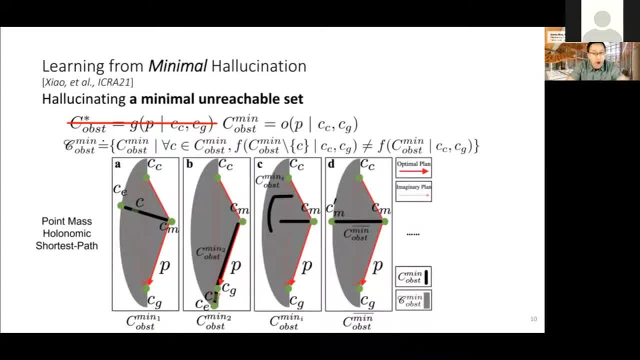 unusual sets as well. we can prove in the paper that the set of all minimal initial set is the gray area composed of a half ellipse and a triangle. so if the gray area is small enough, we can probably just use one representative minimal obstacle set to represent all of them. 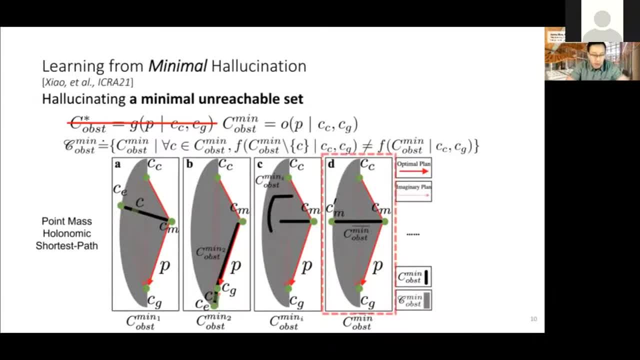 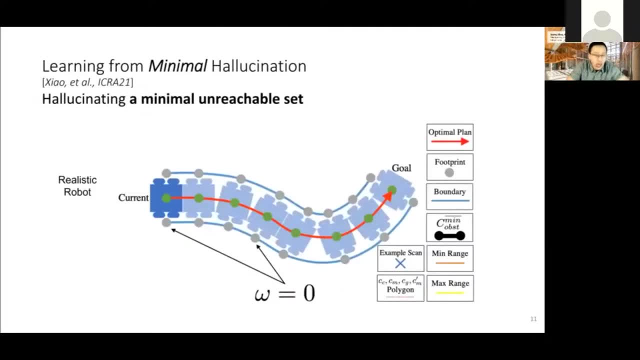 so let's use the straight line cmcm prime, showing figure d to represent all of them. cm prime is the symmetrical point of cm with respect to cccg to deal with a realistic non-harmonic robot. we apply a similar reasoning from the last slide to consecutive configurations collected in urban. 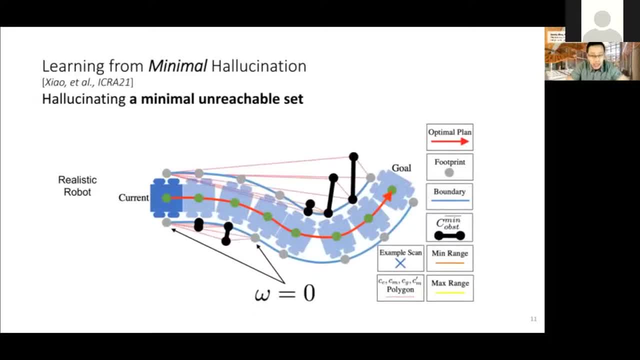 space. the red dotted lines represent the cccmcg cm prime polygon in the last slide and we use the black straight lines cmcm prime to approximate this minimal obstacle set. we call them c, min, c obstacle, min bar. so these black lines are the configurations which must be obstacles for. 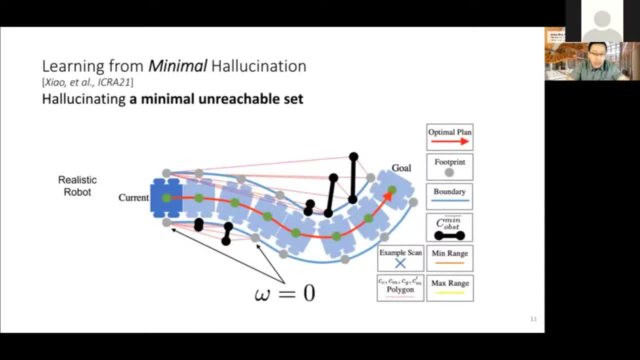 other configurations. they can be obstacle or they can be free, as long as they are not within the area where the robot's footprints are through defined by the blue boundary. to instantiate the obstacle, we use ray casting for laser range readings. the blue boundary and the black minimal initial set give us a minimal and a maximum reading. 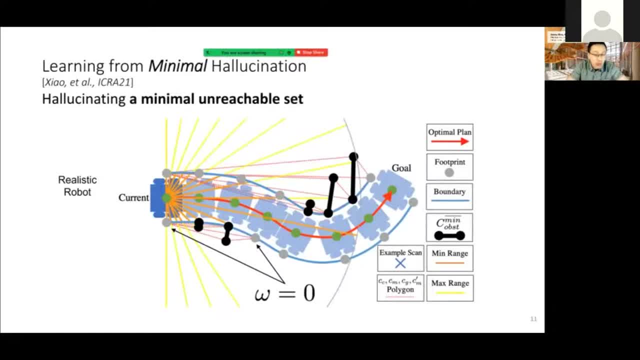 of each beam showing orange and yellow and every value between these min and max still makes the red motion plan optimal. therefore, we can simply sample many times between the min and max values to generate the many c obstacle as training data. these blue crosses are only one example of a sample. 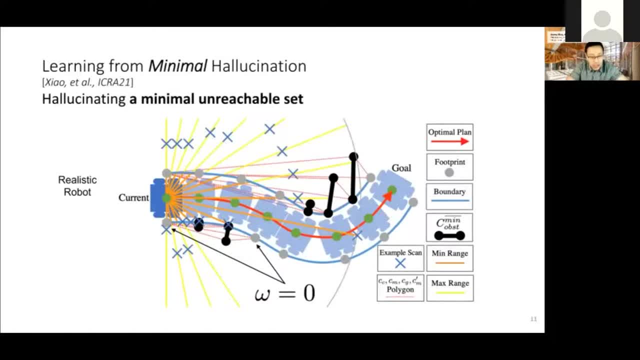 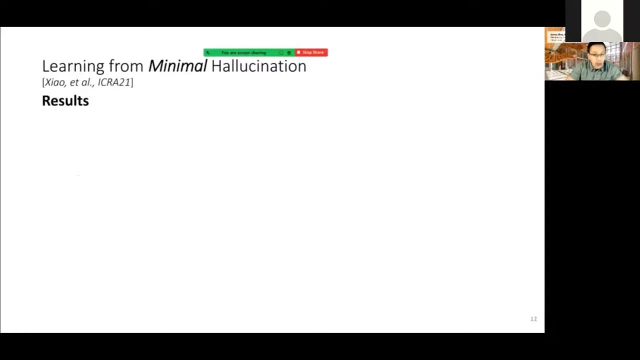 we can also bias the sampling based on uncertainty, for example, fast emotions with higher uncertainty, the sampling can be biased towards the maximum value. while for slower, more accurate motion we expect the robot to be moving in very confined space and the biased the sampling towards the minimal value. we also implemented hrsd on the jaguar robot. you can find more experiment. 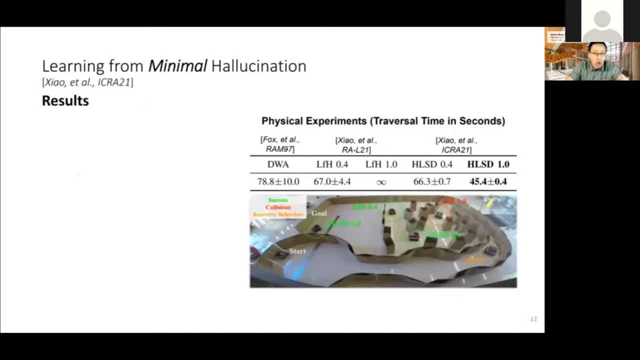 details in the paper but the main idea is hrsd can deal with very linear velocities in the training set, such as as a 1.0 meter per second data set, but the lfn is confident that the lfh data set can deal with many linear velocities in the training set, such as the 1.0 meter per second data set, but the lfh is confi. 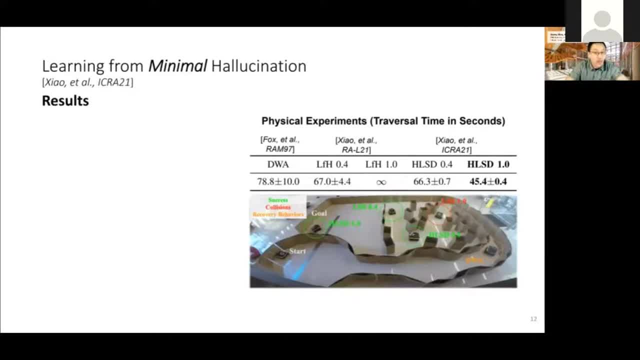 in the training set, such as the one point only two seconds data set, but the lfh is confi due to the ambiguity caused by the most confirmed unreachable set. Therefore, HLSD does not require runtime hallucination and can also generate fastest navigation performance. 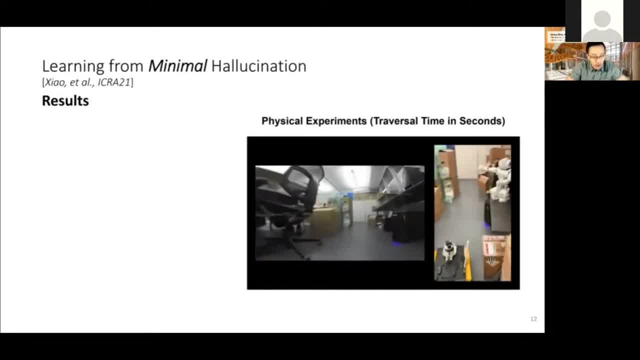 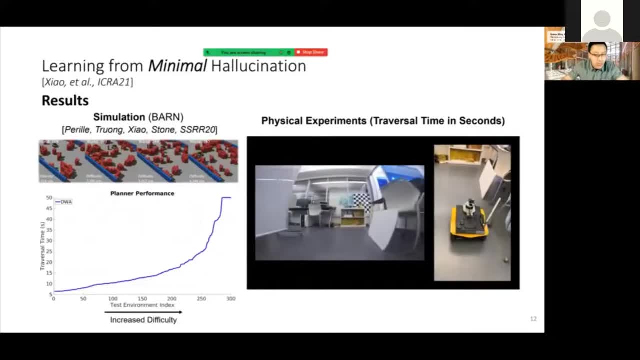 A video of HLSD being deployed in a natural environment. We tested HLSD in the BARM dataset as well. Again, we ordered 300 navigation environments in BARM based on DWA traversal time. HLSD achieved the best traversal time and the performance is not very sensitive. 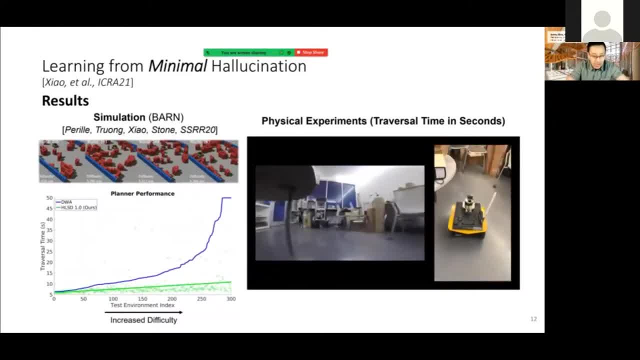 to the environmental difficulty as shown by the flagged green line. LFH 0.4, shown in magenta, and HLSD 0.4, shown in cyan, perform similarly, while LFH 1.0 gets confused due to ambiguity. 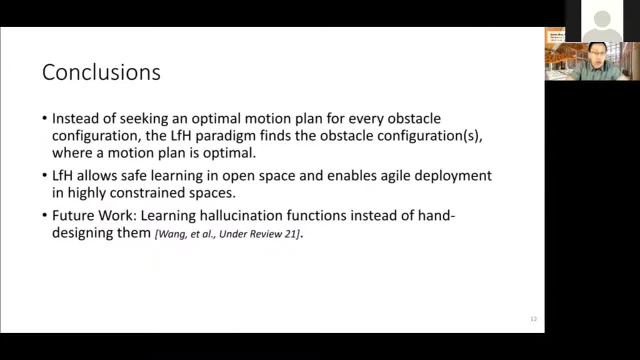 so the red dots are scattered all over the graph. In conclusion, the LFH paradigm investigates the inverse problem of classical motion planning by hallucinating appropriate obstacle configurations to make motion plans optimal. It can generate a lot of safe training data in open space and enables agile deployment in highly constrained ones. 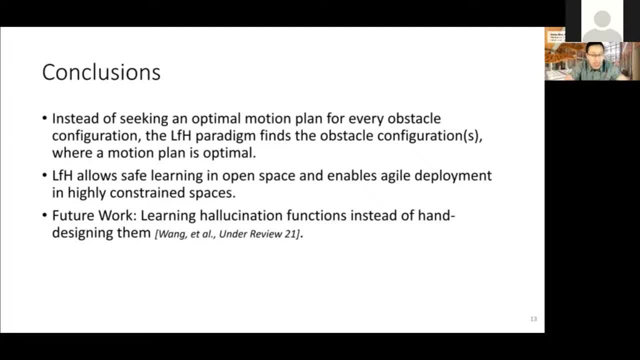 One of our main challenges is that we don't have a lot of information on how to solve these problems. Our future work is to learn hallucination functions instead of handcrafted ones, to generalize to different types of robots with higher degree of freedom, such as fast maneuvering drones. 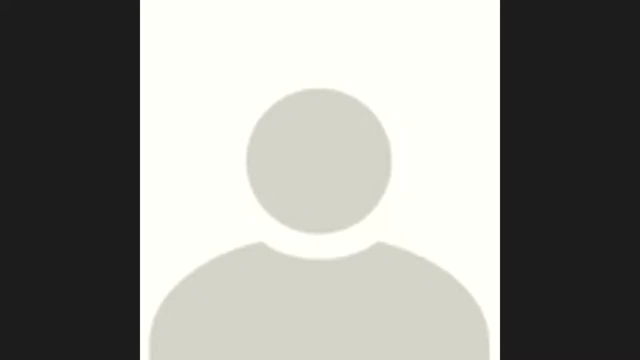 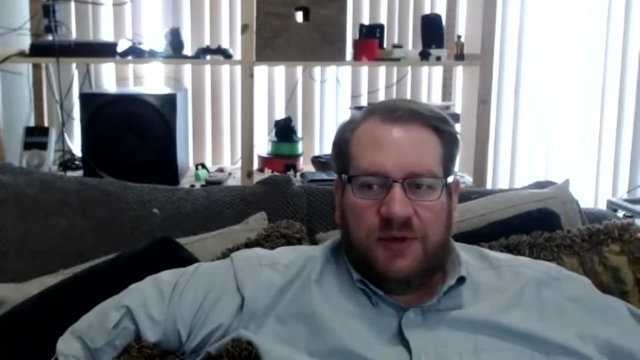 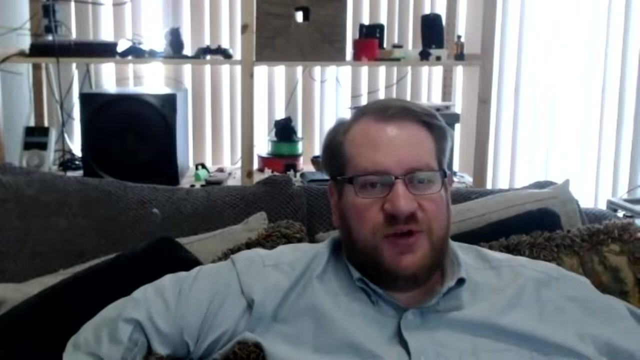 or even manipulator arms. Thank you for your attention and I'm open to take any questions. All right, Let's thank our speaker and open the floor to questions. All right, I've got a question, So I see you have this paper under review. 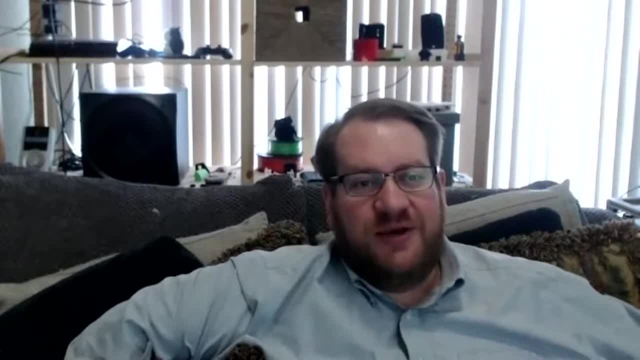 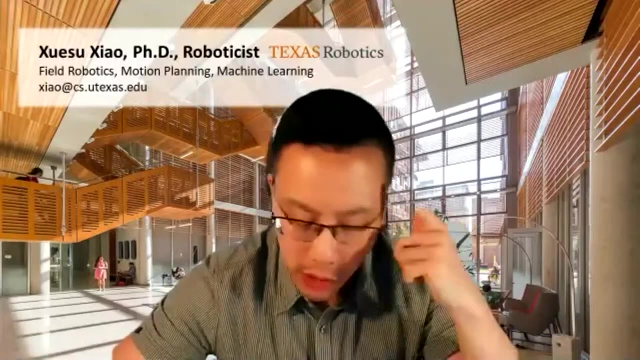 where you're learning about the obstacles, right? So what does that look like? What's the algorithm look like to learn the hallucinated obstacles? Yeah, So the methods we talked about in this presentation is about manually designing those obstacles. In this learning paper, we try to learn it. 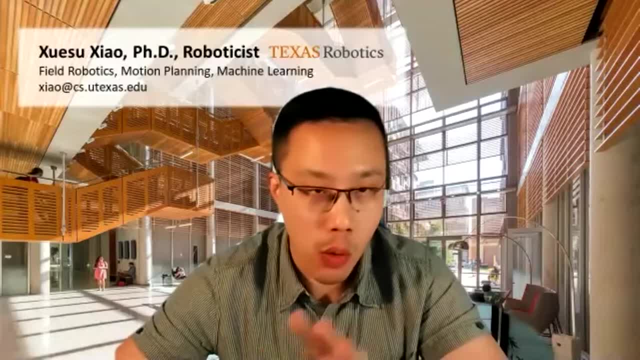 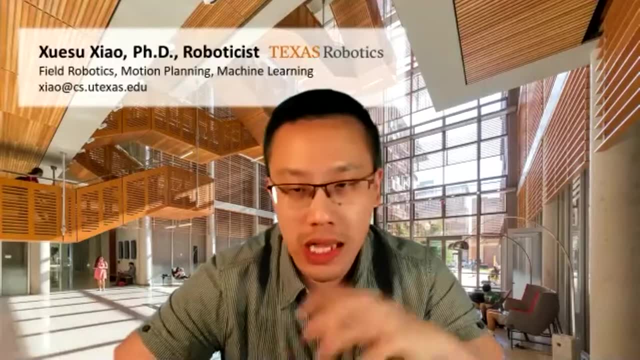 The basic idea is we use an encoder-decoder architecture where the decoder is fixed. It is kind of like a differentiable motion planner, like classical motion planner. So we collect lots of training data in the open space and then we feed that into the encoder. 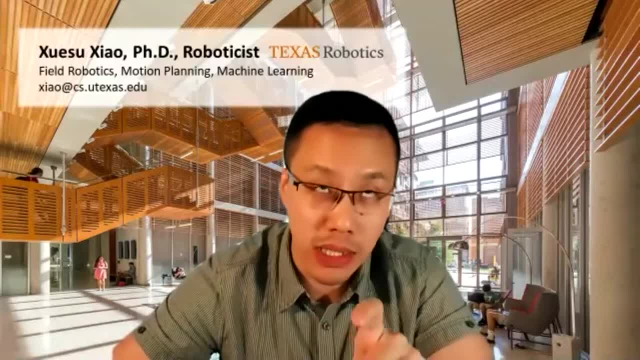 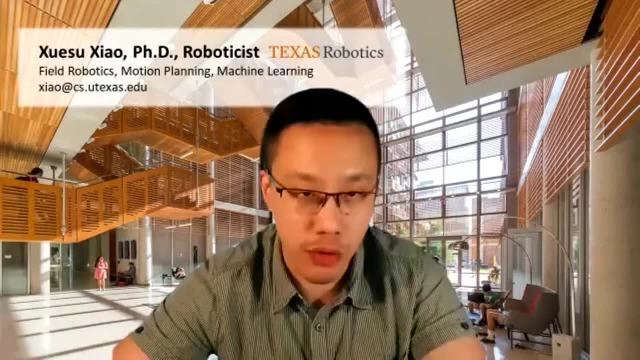 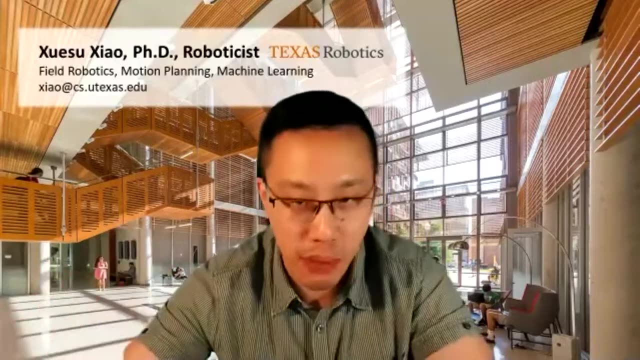 The encoded latent space is basically a distribution of obstacles we can sample from, And then we sample from this obstacle distribution. We use this differentiable decoder like a classical motion planner and try to reconstruct the same motion plans that we collected in open space. 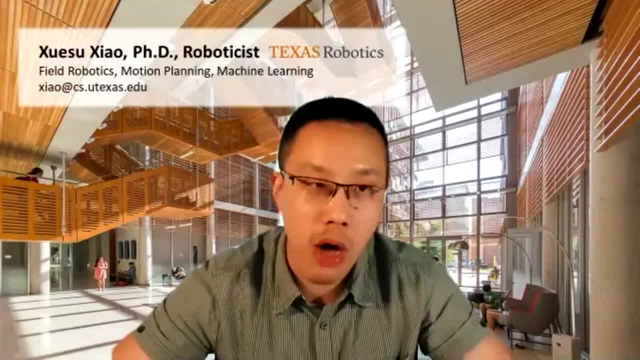 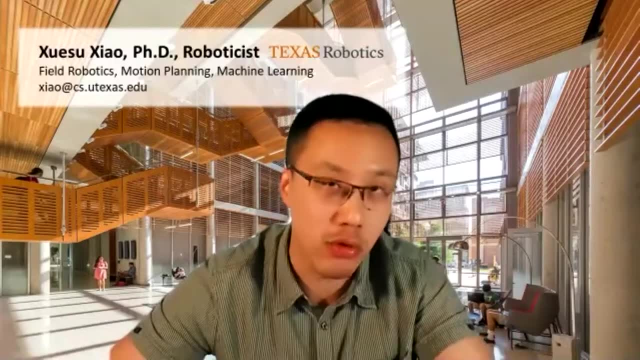 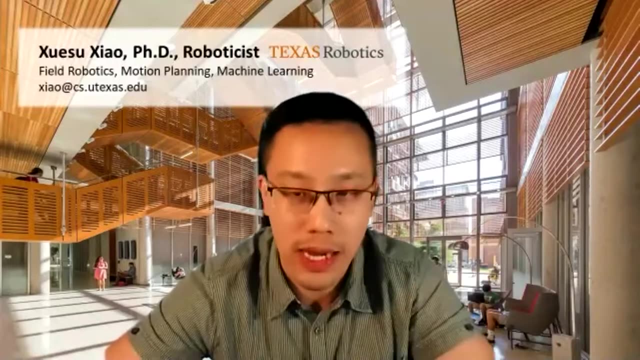 In this way the latent space is constrained to be the reasonable obstacle configurations that make the plan optimal. Then we can sample many, many times from this latent space to reconstruct many different obstacle configurations and then train and mapping from obstacle to motion plans this way. 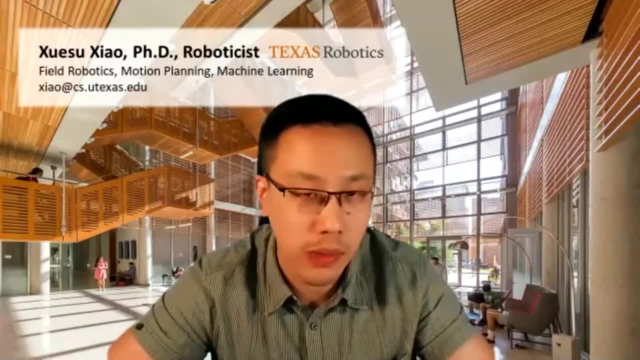 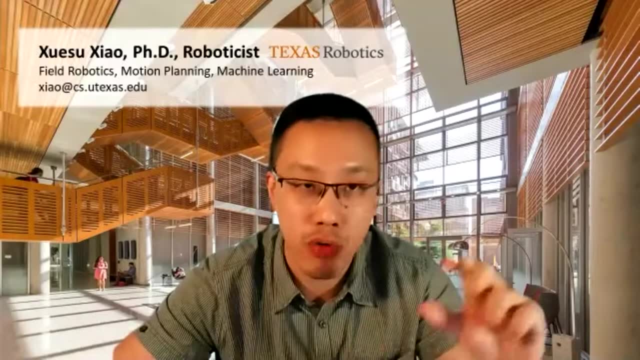 Yeah, The idea of this is because we want to extend to higher dimensional workspaces or even like longer planning horizon. We actually show that this method works very well, even for 3D flying drone, because that's very difficult for us to design. 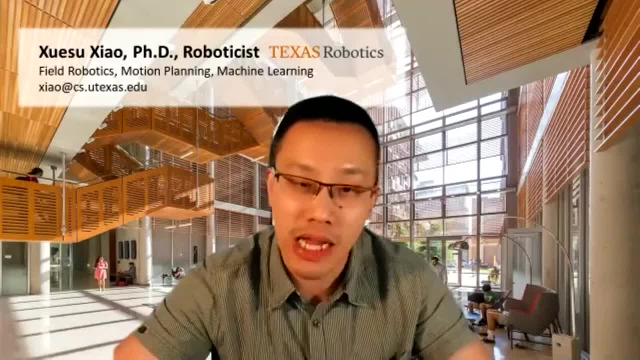 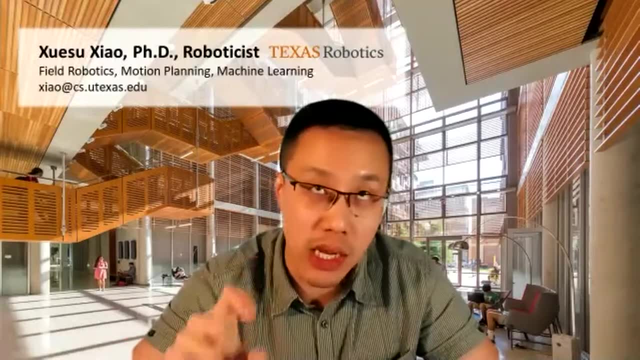 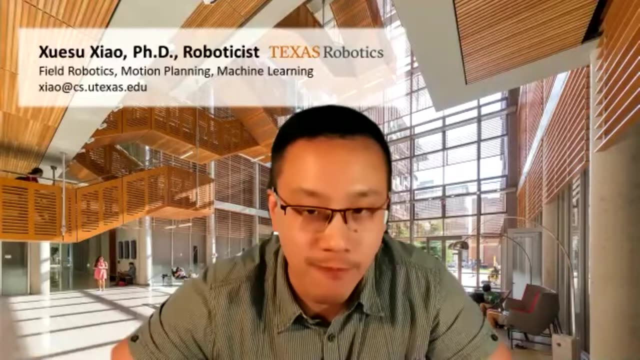 to manually design a hallucination function to make like a very complicated 3D trajectory from a drone optimal. So through this way we can learn this embedding space and then try to sample from them, come up with lots of training data without manually designing hallucination function. 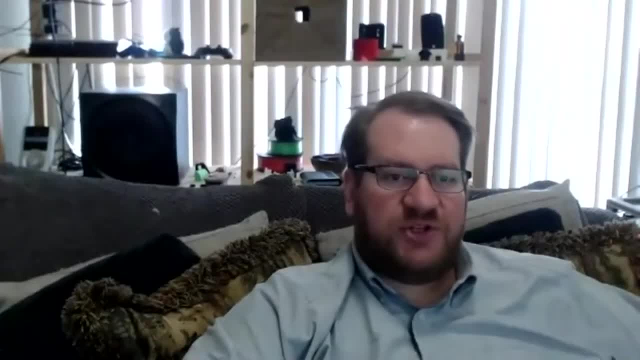 That makes sense. Do we have any more questions? Well, if we have no more questions, let's go ahead and proceed to our next presentation. Our presenter will be Suram Siva, and I'll go ahead and cue that up. So let's see now. 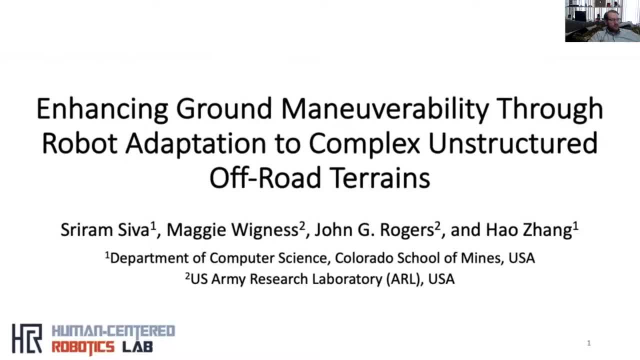 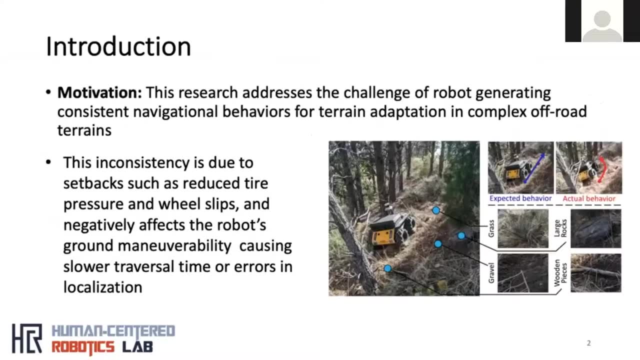 Hello, Welcome to our presentation on enhancing ground maneuverability through robot adaptation to complex unstructured off-road terrains. This project was conducted at the Colorado School of Mines in partnership with the United States Army Research Lab. In this research, we addressed the problem of generating 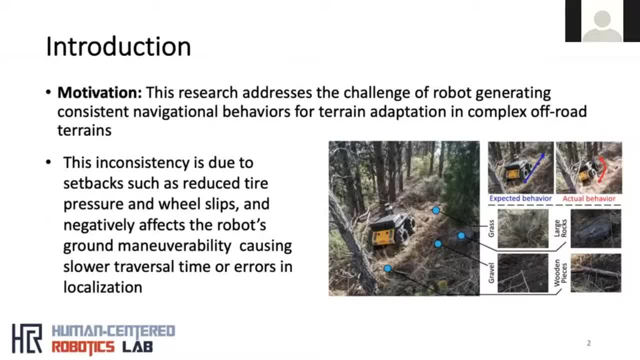 consistent robot navigational behaviors for robot terrain adaptation in complex unstructured terrains. The inconsistency in navigational behaviors arises due to the presence of setbacks in robot navigation. The setbacks include reduced tire pressure and wheel slips. This inconsistency negatively affects a robot's ground maneuverability. 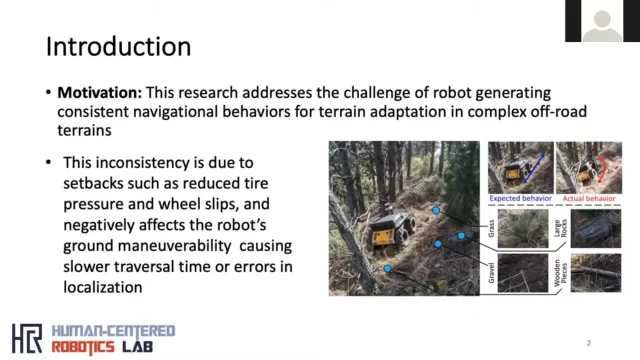 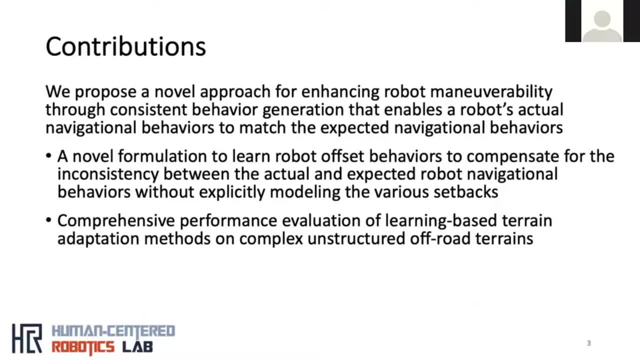 and can cause slower traversal times or even errors in robot localization. To address this challenge, we propose ANOVA formulation for enhancing robot's maneuverability through consistent behavior generation that enables a robot's actual behaviors to match its expected navigational behaviors. Our approach then learns to. 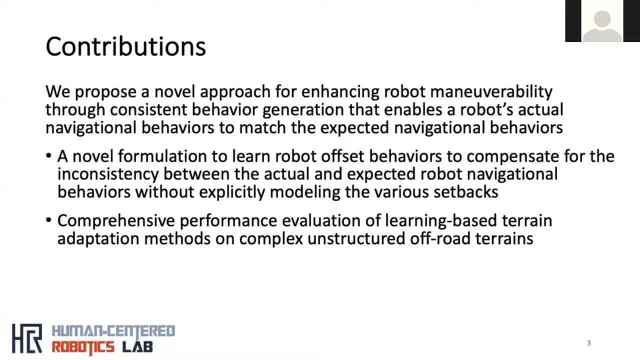 generate consistent navigational behaviors through learning an offset according to the terrain the robot is traversing on. This offset is then used to compensate for the inconsistency between the robot's actual navigational behaviors and its expected navigational behaviors. Our approach also doesn't require 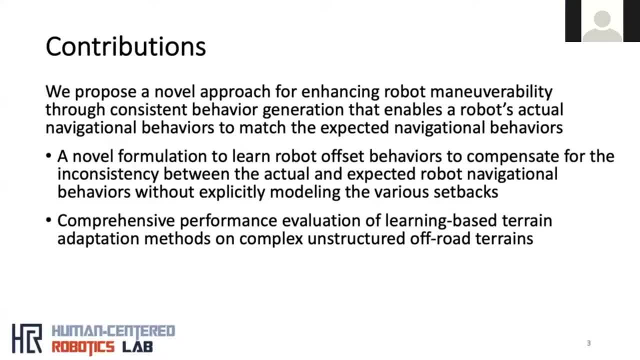 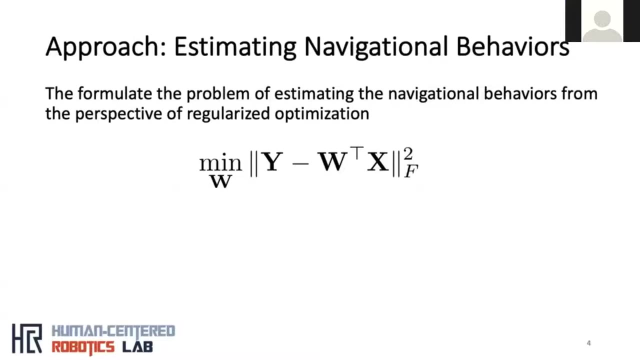 the need to model the various setbacks. implicitly. As an experimental contribution, we provide a comprehensive performance evaluation of learning-based terrain adaptation methods by designing a set of live robot navigation scenarios over complex unstructured off-road terrains. Coming to our approach, we first formulate the problem. 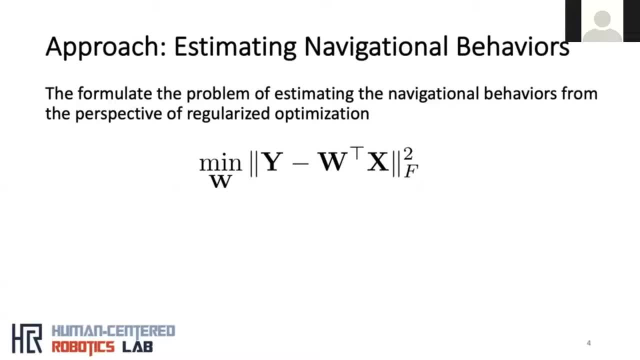 of estimating the robot's expected navigational behaviors using the framework of regularized optimization. Here, the matrix X is used to denote the terrain features and the matrix Y is the corresponding expected behaviors. The Frobenius loss function is used to encode the error of using a linear model. 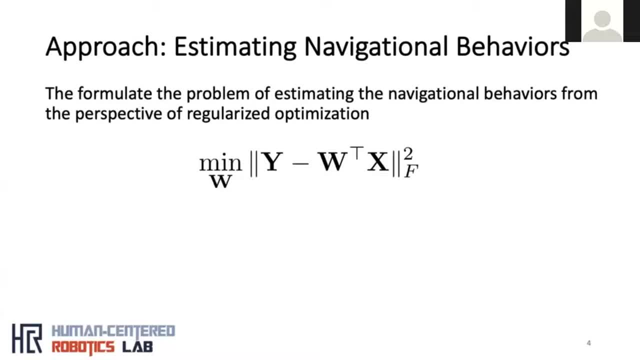 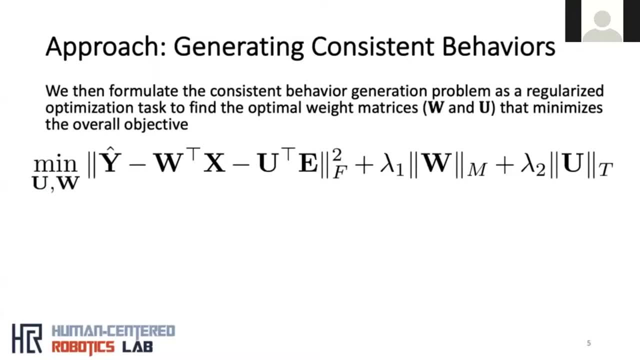 parametrized by matrix W to project the terrain features onto the estimated robot behaviors. Then the problem of generating consistent navigational behaviors is formulated as a regularized optimization task with the aim of finding optimal matrices W and U that minimizes the objective function. 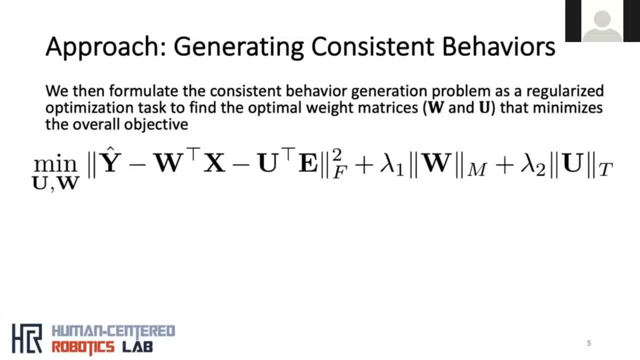 in the given equation. Here, the variables Y-hat represent the actual robot behaviors estimated using a post-estimation technique such as SLAM. The matrix E is a behavior difference matrix consisting of the difference between the robot's actual navigational behaviors and the robot's expected navigational behaviors. 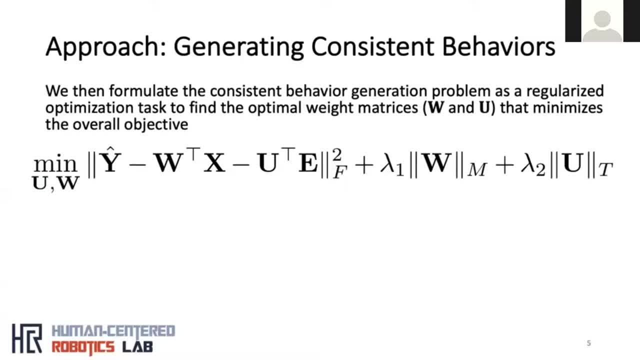 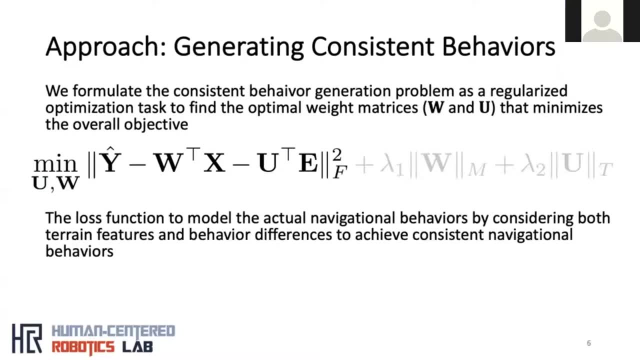 The expected navigational behaviors are provided by an expert human demonstrator while operating on the robot. The first term of our objective function is a Frobenius loss function to model the actual navigational behaviors by considering both terrain features and the behavior differences to achieve consistent navigational behaviors. 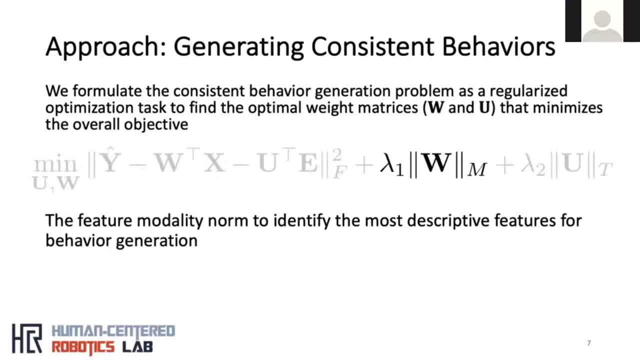 The second term in our objective is a regularization term named as the feature modality norm. This regularization term enforces sparsity among different feature modalities to identify the most descriptive features for behavior generation. Finally, the last term in our objective is also a regularization term. 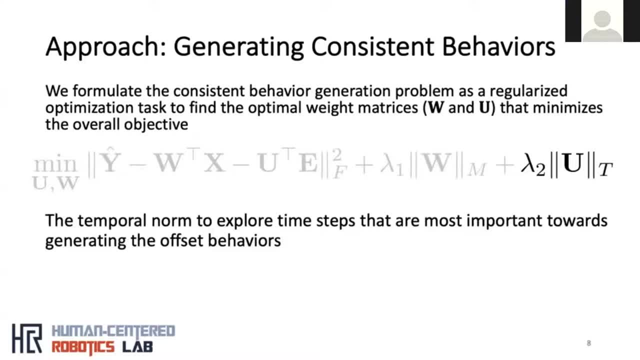 This regularization term is called the temporal norm and is designed to explore the time steps in historical data that are more important for generating offset behaviors. In our objective function, lambda1 and lambda2 are trade-off hyperparameters to balance the loss function and the regularization term. 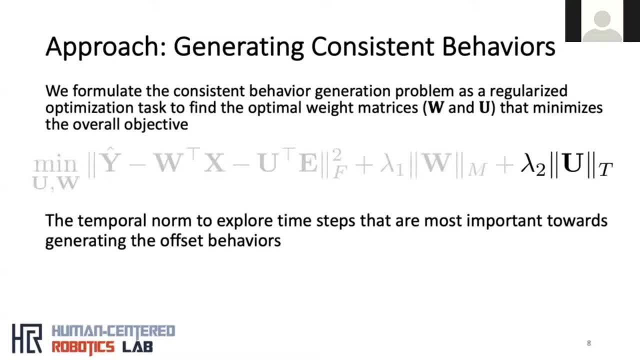 It's to be noted that the value of lambda1 and lambda2 are always greater than or equal to 0. Our objective function is then able to generate consistent navigational behaviors. while identifying the most important feature modalities and also historical time steps, We evaluate and test our approach. 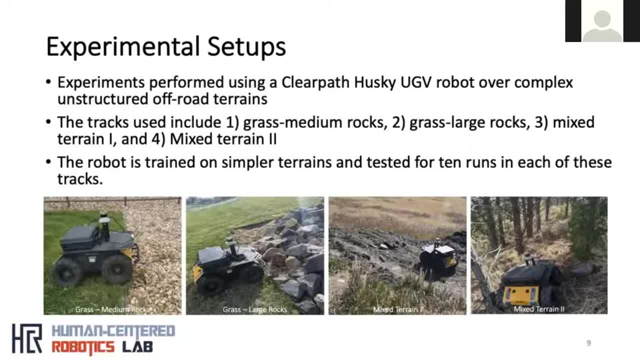 on a ClearPath Husky UGV robot over complex unstructured off-road terrains. The robot is equipped with an Intel RealSense D435 camera, an AllStar OS164 LiDAR and internal sensors, including wheel odometers. inertial measurement units. 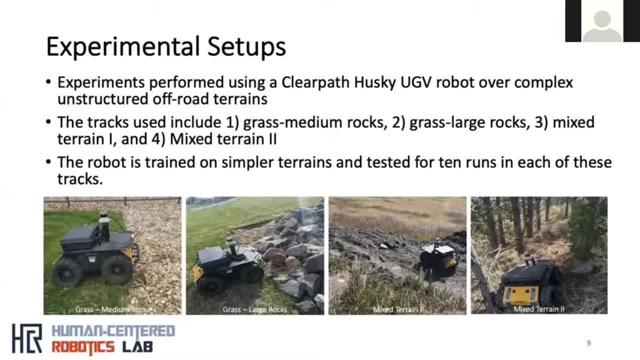 to measure the robot's internal states. The tracks used in our experimentation either show transition between different types of terrain, such as grass to large rocks and grass to medium rocks, or a mix of terrain types in real off-road environments, such as the mixed terrain type 1. 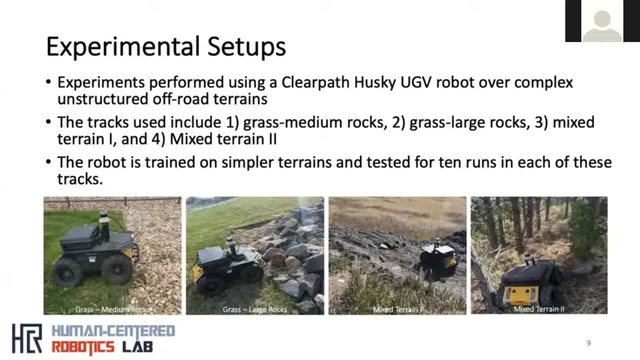 and mixed terrain type 2.. The mixed terrain type 2 is a forest environment. Our approach is trained on data obtained on simple individual terrains, such as grass only, mud only or rock only terrains. The training data is obtained as a human operator controls. 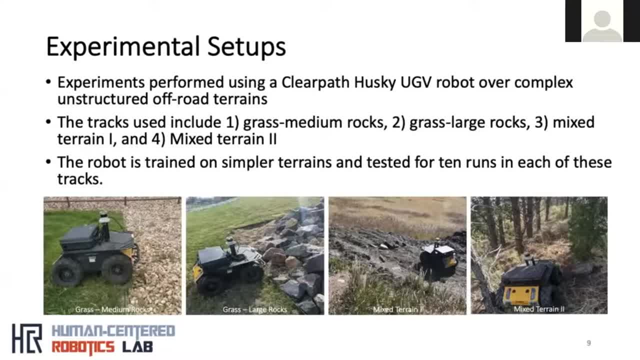 the robot to traverse over these terrains as fast as possible while also maintaining safety that is, not flipping or crashing the robot. For testing, we execute our approach on each track for 10 runs and record an average for the results. We also test our method against. 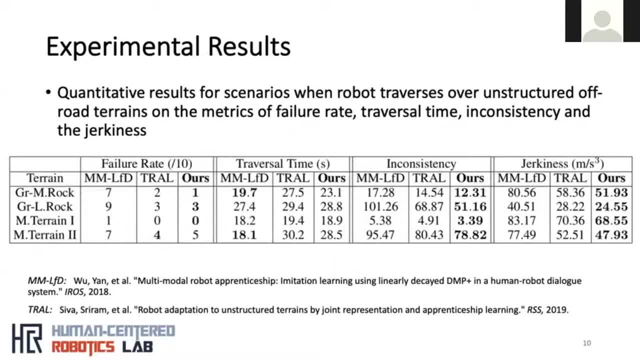 previous learning-based approaches, including learning from demonstration and the state-of-the-art TRAL approach. We compare these approaches over four evaluation metrics, including failure rate, traversal time, inconsistency and jerkiness. Failure rate is taken as the number of times the robot failed to reach its navigational goals. 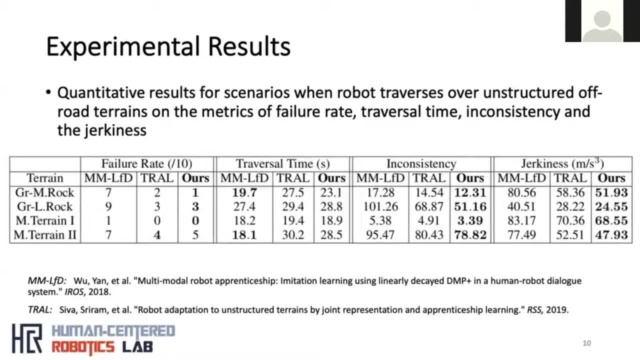 from a total of 10 different runs. In the successful runs, the time taken for completing this navigation task is taken as the traversal time, And inconsistency is defined as the measure of difference between robot's expected navigational behaviors and the robot's actual navigational behaviors. 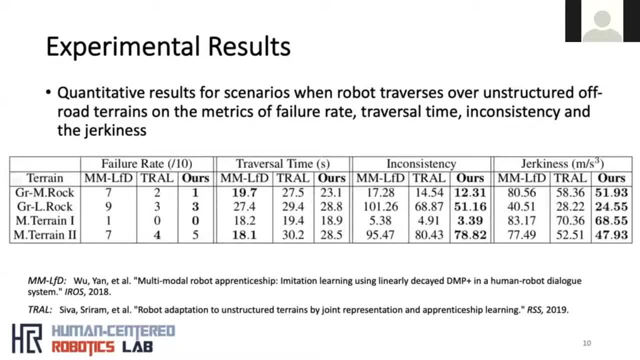 Jerkiness is then taken as the average sum of acceleration derivatives along all of the robot's accesses. The quantitative experimental results from the table shows that our approach obtains the least failure rate. in most of the terrains Our approach also significantly outperforms. 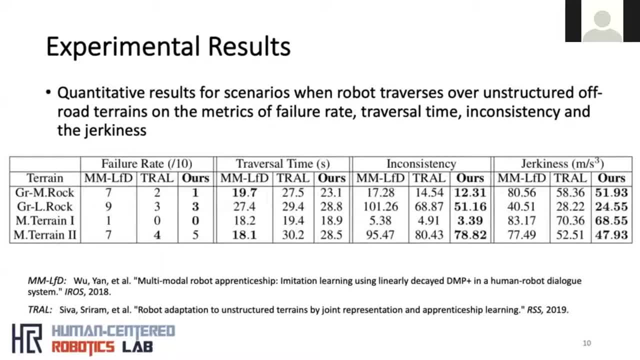 the learning from demonstration approach in terms of failure rate. We observe that learning from demonstration method has a lesser traversal time for successful runs, but has a significantly higher failure rate. Moreover, learning from demonstration approach is outperformed by our approach with respect to inconsistency. 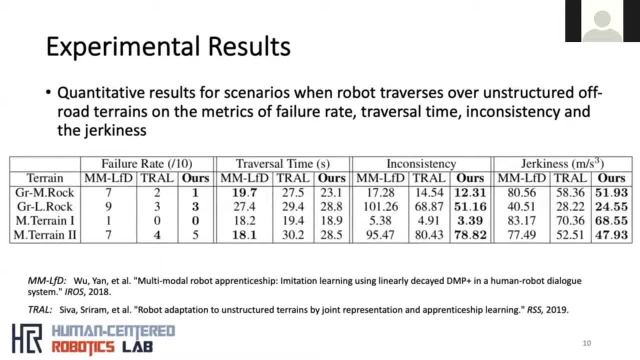 and jerkiness metric. Especially, the difference is much more observed in the jerkiness metric When comparing our approach with the TRL method. both approaches obtained comparatively smaller values of failure rate over all the terrains. However, when comparing both approaches using performance metrics of 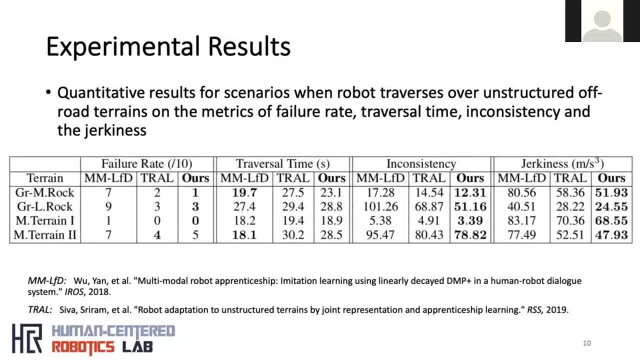 traversal time, inconsistency and jerkiness. the difference between these two approaches is much more visible. We observe that our approach completes the navigation task with lesser traversal time as compared to the TRL method. Furthermore, our approach also obtains lesser jerkiness measure. 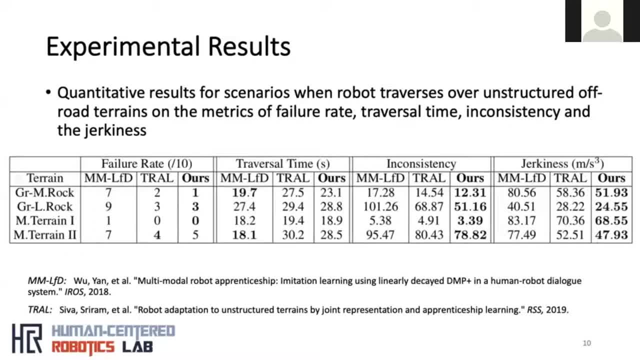 compared to the TRL approach. In terms of inconsistency, our approach significantly outperforms the TRL approach. The clear performance improvement obtained by our performance metric is in view of the fact that our approach is designed to be a closed-loop controller which considers not only terrain characteristics. 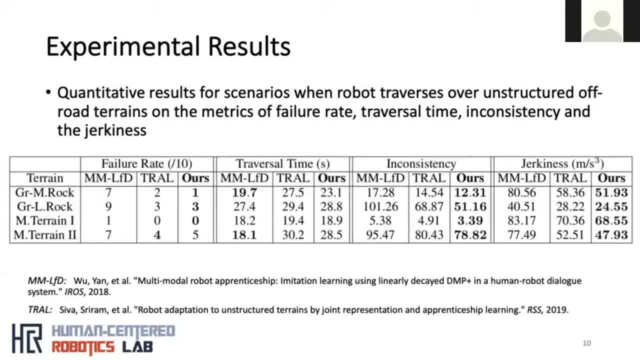 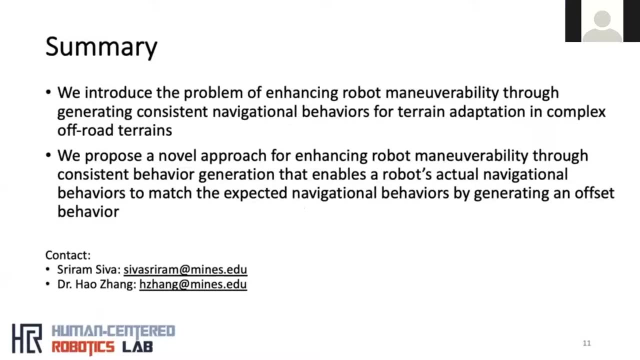 but also robot states when adapting to our work's ground maneuvering behaviors over complex, unstructured off-road terrains. In summary, we introduce the problem of enhancing robot maneuverability through generating consistent navigational behaviors for terrain adaptation in complex off-road terrains. 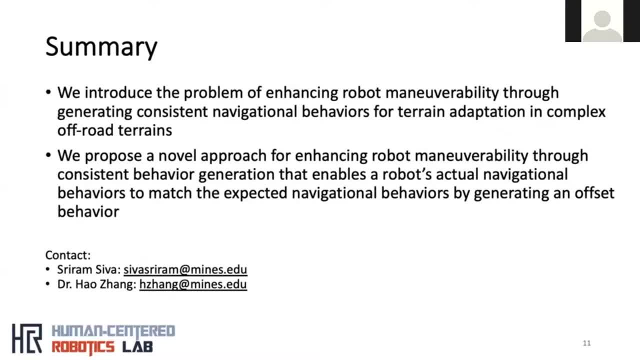 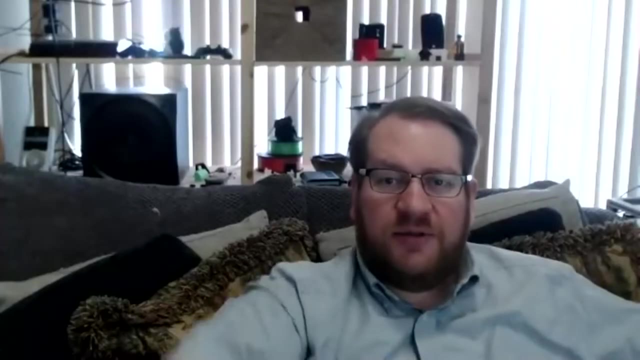 We then propose a novel approach for enhancing robot's maneuverability through consistent behavior generation by generating an offset behavior. These offset behaviors enable a robot's actual navigational behavior to match its expected navigational behaviors. Thank you, Alright, let's thank our speaker. 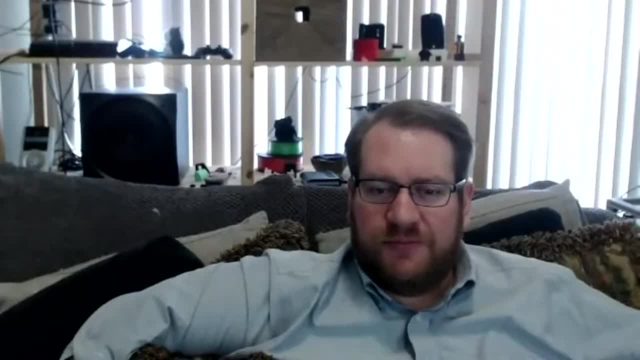 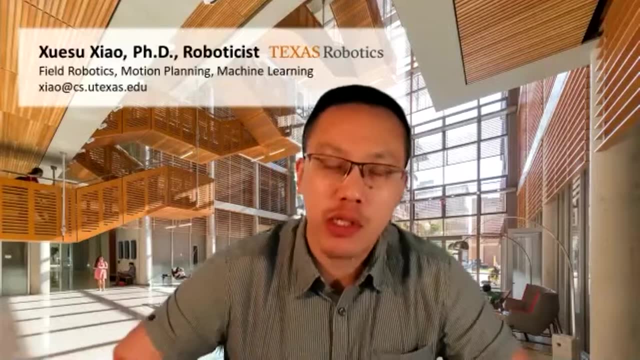 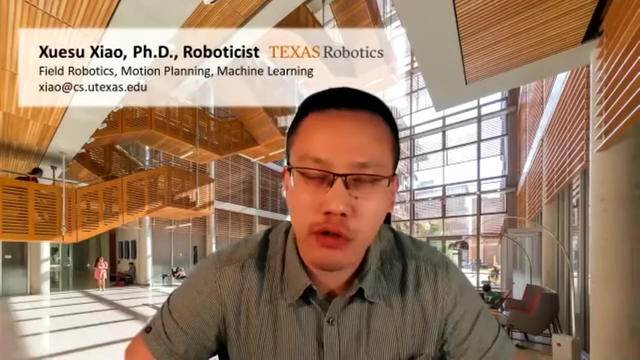 and open the floor to questions. Hey Shuyuan, Very nice presentation. So I'm actually very familiar with this line of work, also your previous TRL work. So I'm really curious like I haven't seen a video demonstration of the final result. 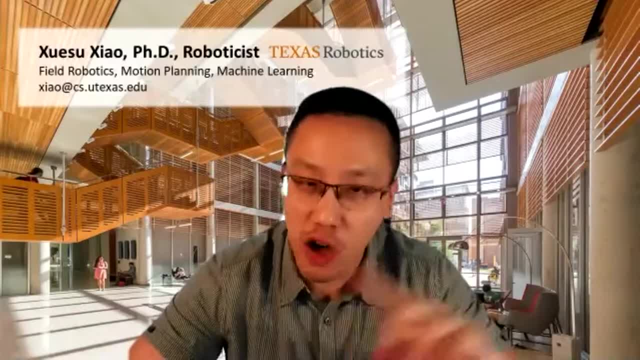 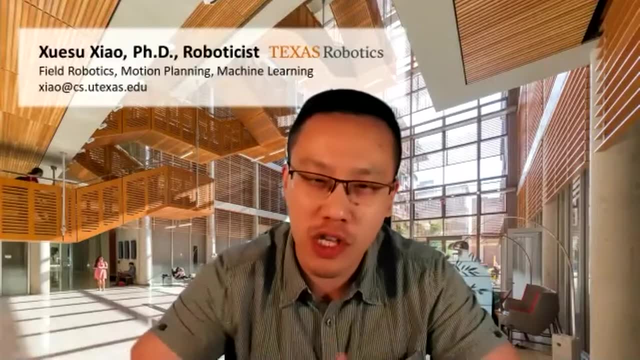 I'm very curious to see what is the qualitative difference of all these methods. right, All the numbers are very convincing, show the advantage of the proposed method. But I'm just curious: what are the qualitative difference like, maybe from a video demonstration point of view? 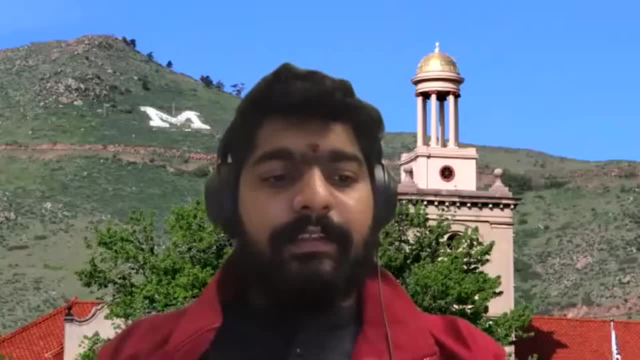 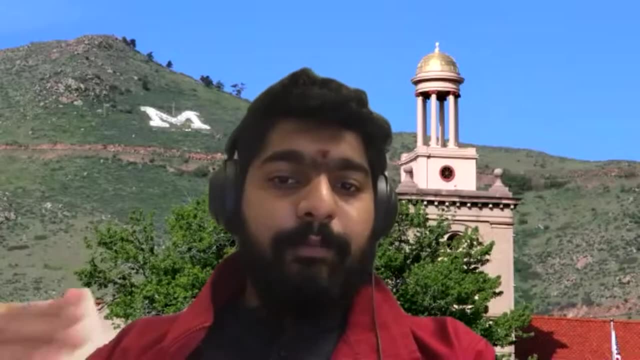 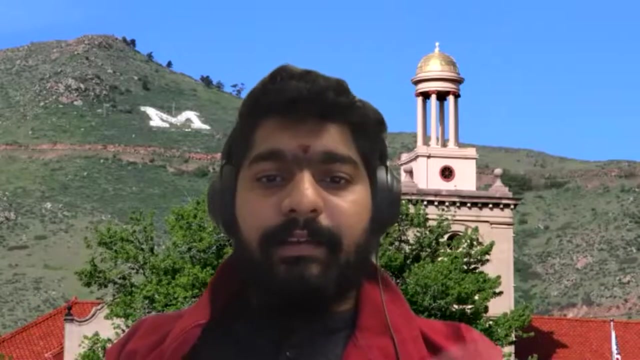 So the qualitative difference, the main reason, like the TRL approach, was just based on data. It was not like on a video demonstration. However, this approach has a video demonstration as it was an extended abstract only for a paper that we have submitted to RSS right now. 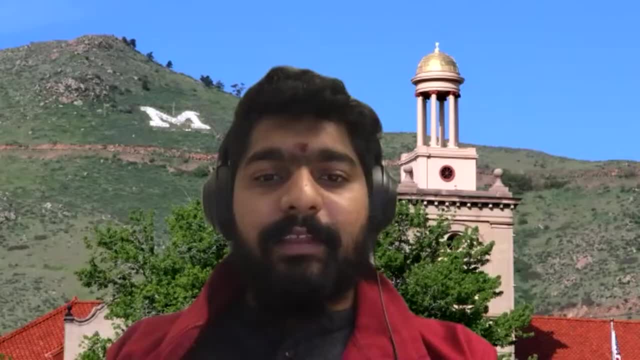 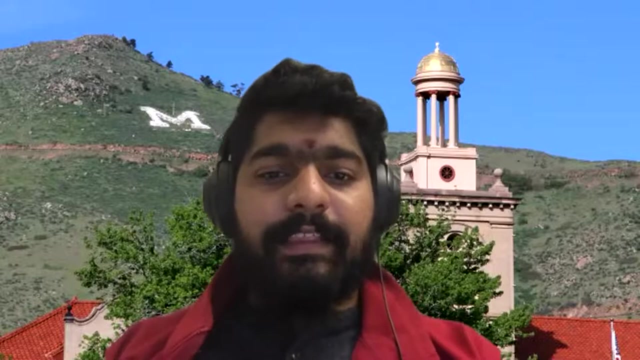 So the plan was to submit like the video to RSS like instead of like, providing the video demonstration. And also the reason is that many of the experiments have also been conducted in like the army research lab facility, And because of that, so we had to build a whole test track. 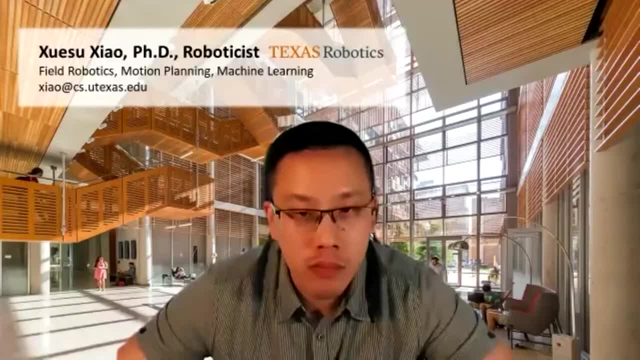 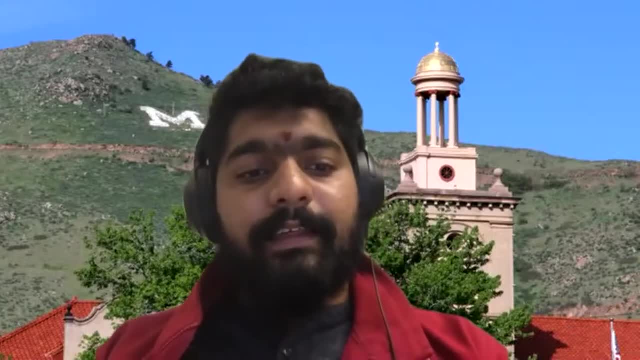 which was like 20 meters by 20 meters long. So many of the experimental videos are like shot in there as well. So once the paper is accepted, we plan to release the video demo And I'll specifically make sure that I have it in my website. 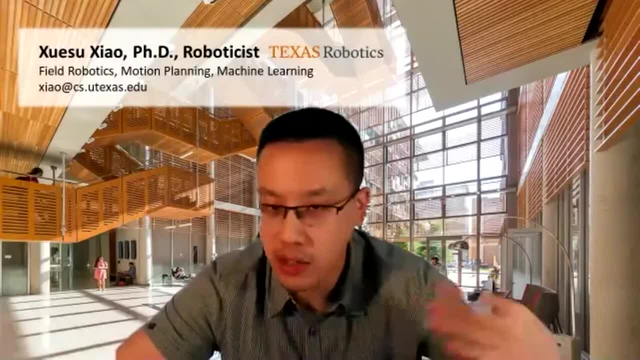 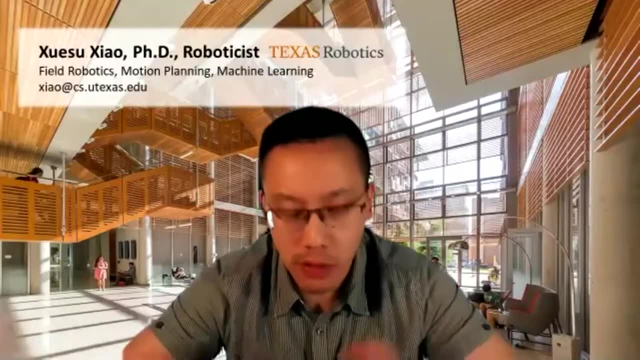 Definitely. Yeah, I'm very curious to see the like qualitative difference between right, Yes, Maybe. Yes, Go ahead please. No, go ahead please. So I'm just maybe you can like. I saw there's. 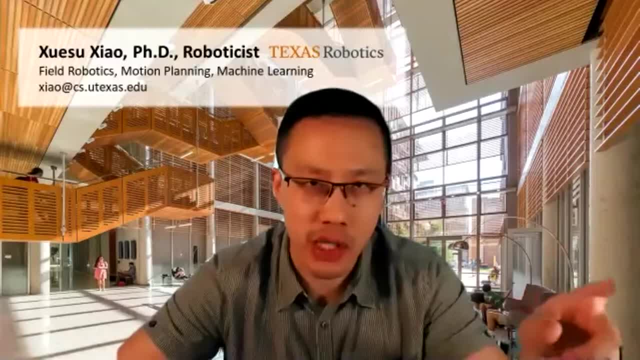 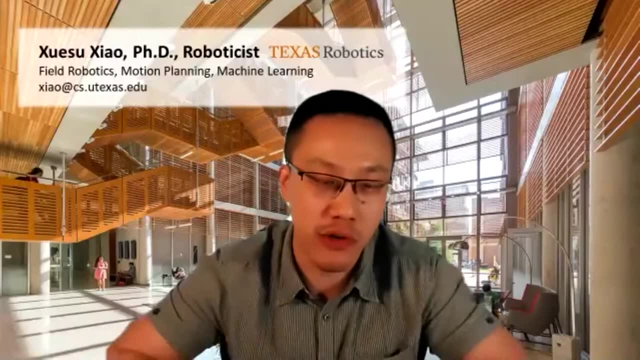 for example, for the behavior cloning method, there's nine failures out of 10 trials. right, So usually the failure is like tipping over or getting stuck on some rocks. Can you like briefly give So? so the main failure happens whenever you have a large rock environment. 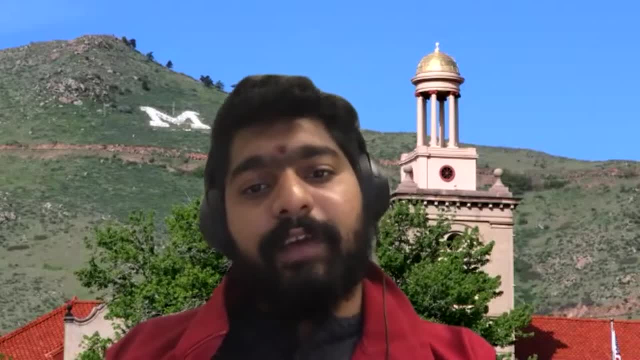 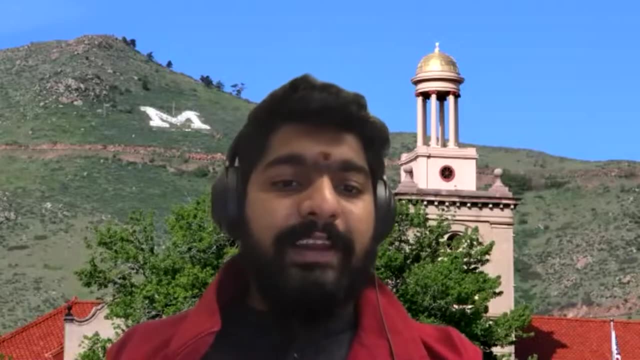 as well as like when you're going through a highly forest environment. In these kinds of environments, as there is not much slope, the main failure is just because it gets stuck, Or you know when it navigates just from grass to large rock. 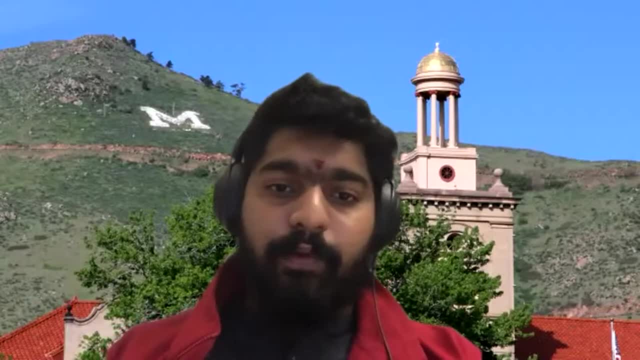 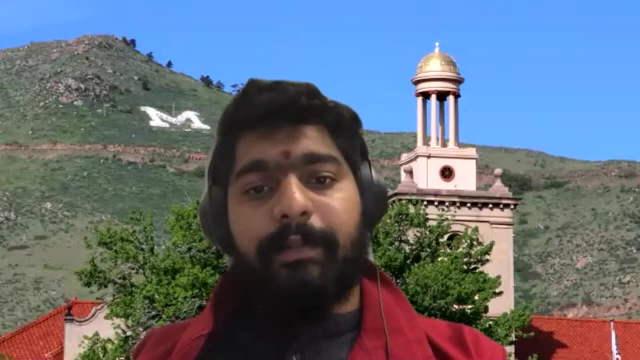 during the transition itself, it gets stuck. So that's one of the main concerns. So like we use like features which are like global features obtained from like the robot's front camera, as well as LIDAR sensors to like form representations of the terrain, 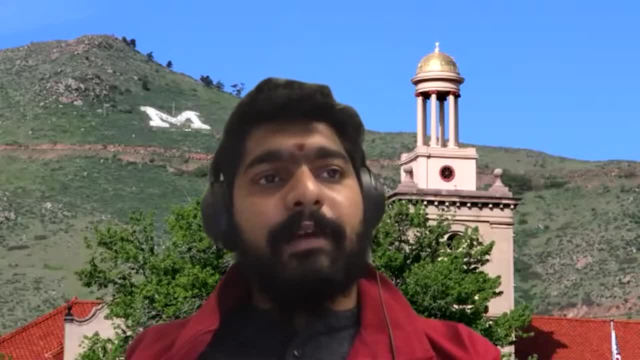 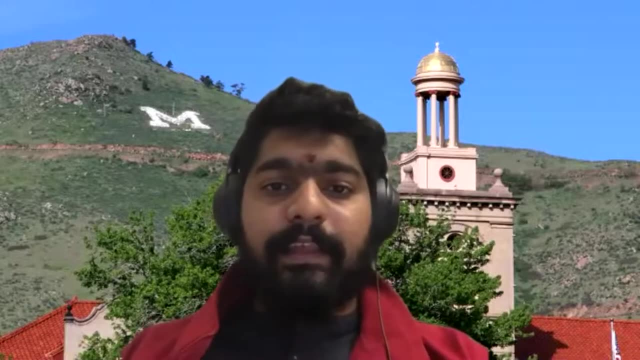 and try to navigate. But the main problem comes whenever you have a transition between, like, one terrain to another terrain. So the robot has to like proactively, that is like before itself, adjust its navigational behaviors. So what happens with learning like behavior, cloning method? 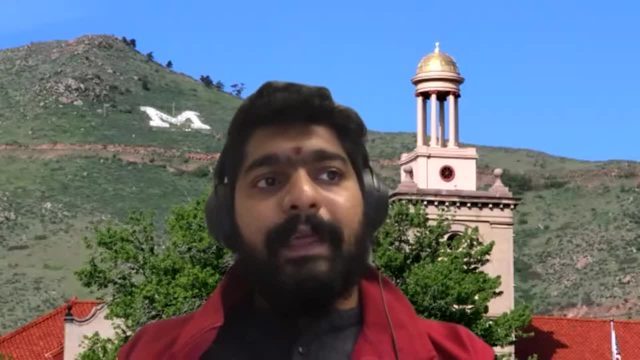 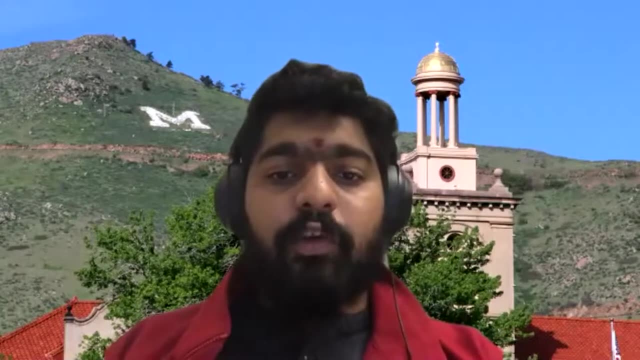 is, it directly goes into the terrain until a switch comes right. So when the switch starts to come, the robot then adapts, but by then it's too late, And you see that when there's a transition it like gets stuck. 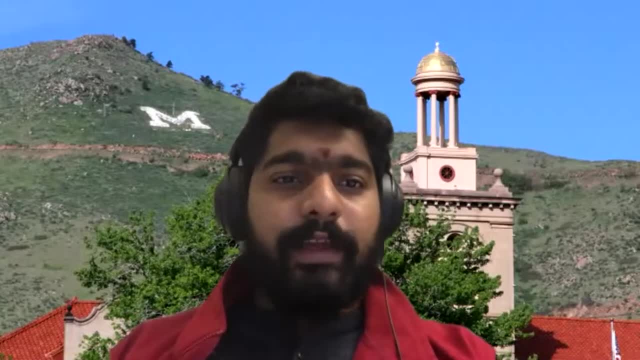 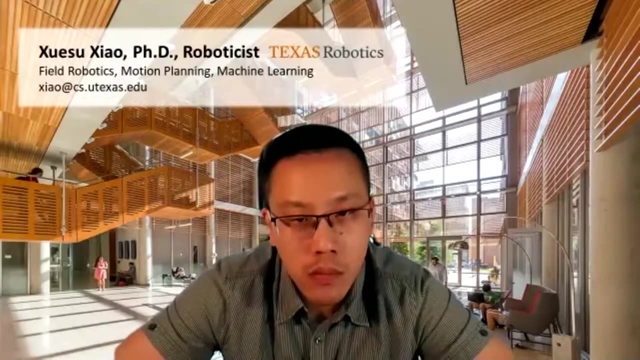 Flipping over is seen only in one or two cases like that I've seen, like when the rocks are too big and the robot is trying to navigate uphill. that's when we see flipping, but it's mostly getting stuck. Okay, So getting stuck. 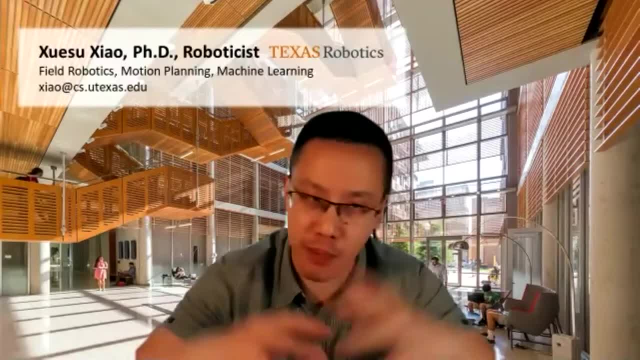 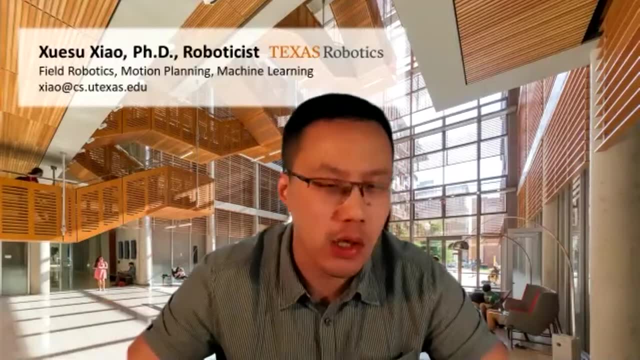 you mean the robot is taking probably like a wrong pass over like a big rock, instead of taking a more like smoother pass. Is that the reason of the getting stuck? Or even lower level, like motor commands how you turn the wheels, getting stuck? 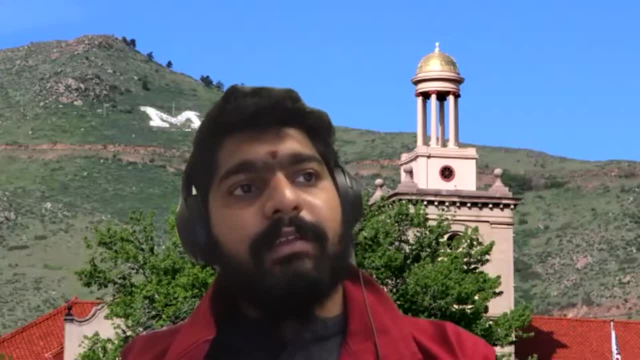 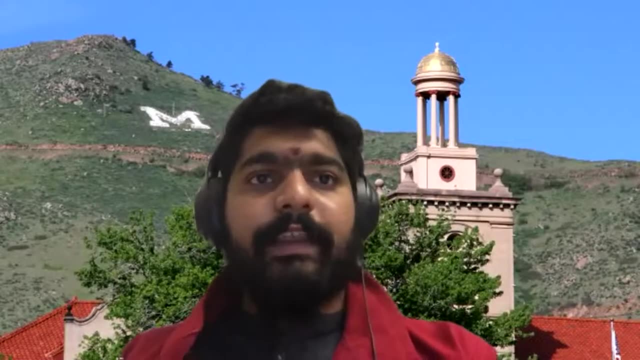 So the robot? so like the behavior cloning method, it's not like a feedback based method, So what it does is it's just like feed forward. So you see the terrain and you try to generate navigational commands. But the problem is: 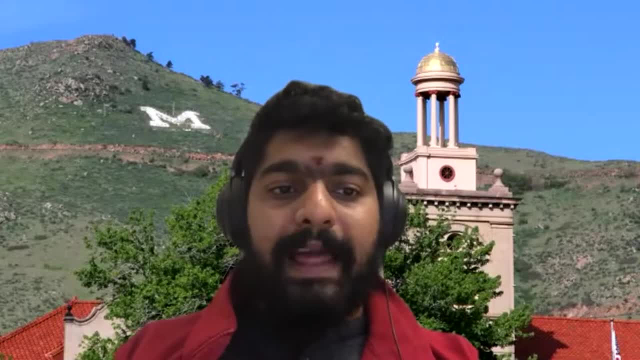 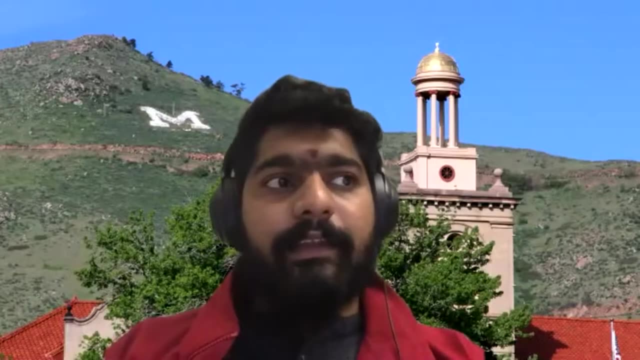 I would say it falls under the domain of not planning the path adequately, because it gets stuck in places where the robot, like the size of the terrain, is much higher than the robot's, like wheel base. So right, So it gets stuck in rocks. 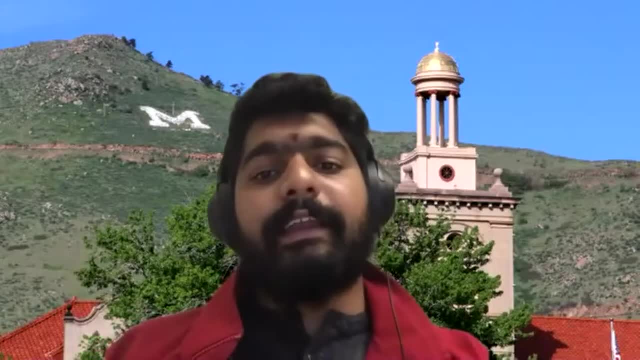 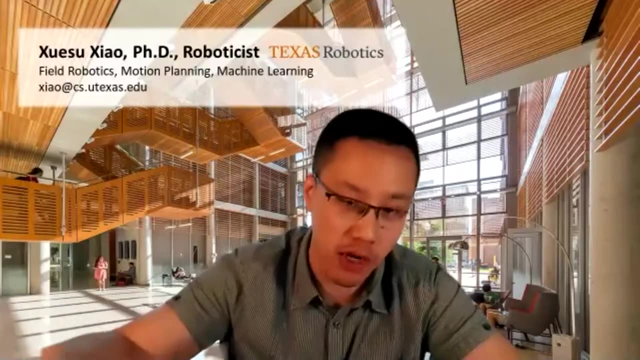 and try to get the wheels rotating, but it doesn't get any traction. Okay, So it's more kind of like a pass level mistake. I would say: right, You shouldn't go through that big rock, It should be taking a pass beside it. 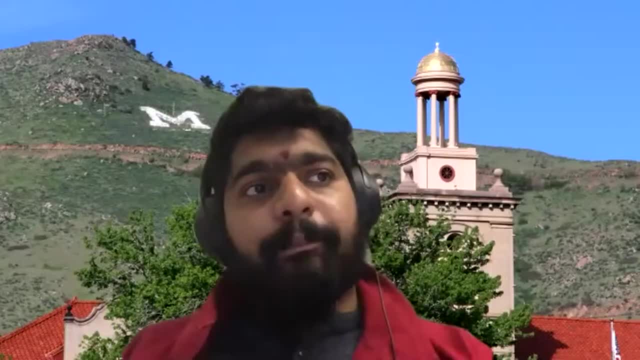 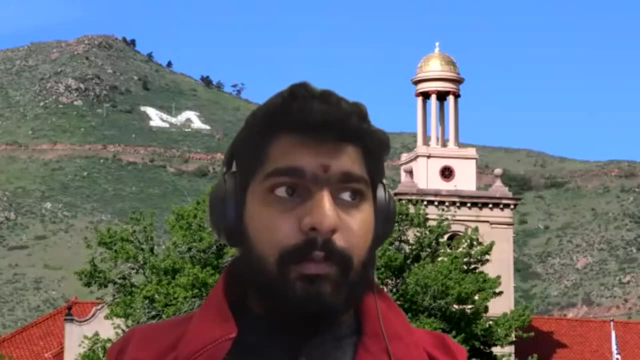 like with smaller rocks, it does. Oh no, The thing is with the same rock itself. if you are able to adjust your speed properly, you would not see the robot getting stuck in that rock right? So what it does is: 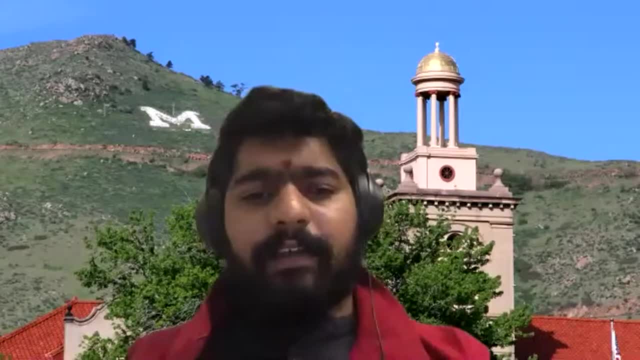 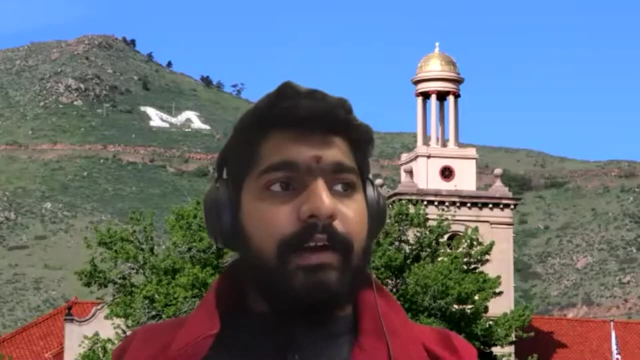 so if you are just trying to go fast, as fast as possible, on these rocks as well, the robot gets stuck. But if you slowly maneuver your speed, like we, know that we do not want to damage the robot and we teach the robot in such a way- 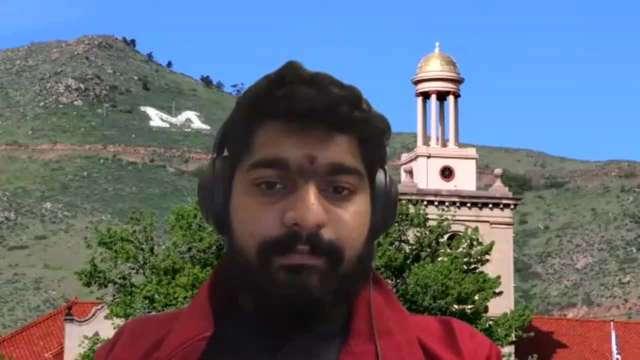 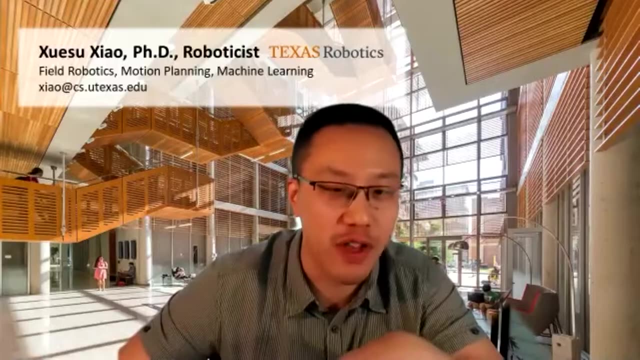 So when you do that, you would see that the robot is like not getting stuck. Okay, Yeah, That'll make a lot of sense. Yeah, That's also why I'm very looking forward to see the video. Yes, So just to add on your question. 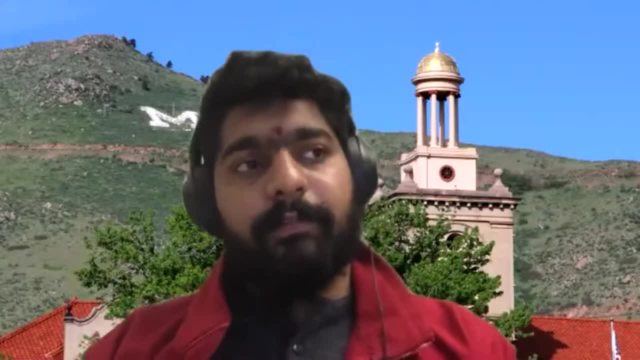 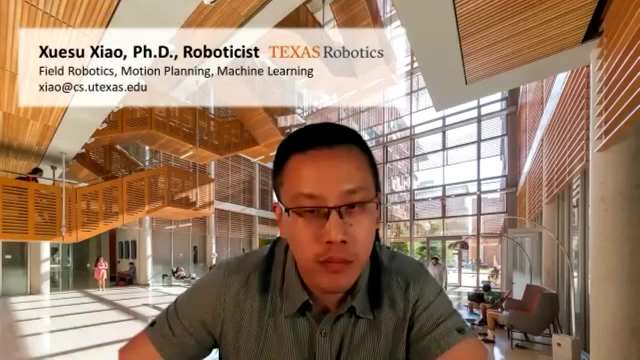 I know that in the abstract paper we cannot provide all the information, but if you consider, like the fourth scenario, which was the mixed terrain too, it was like a forest environment, The robot often- because we have like an obstacle avoidance- also running in the background. 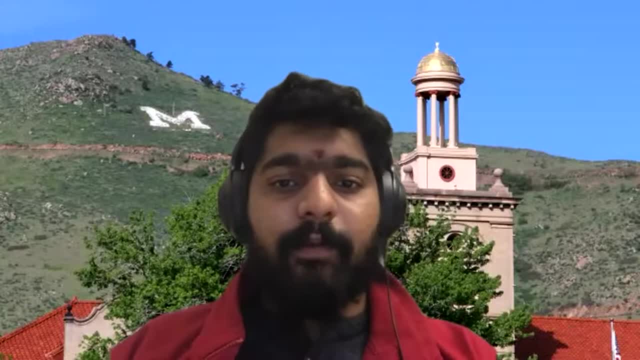 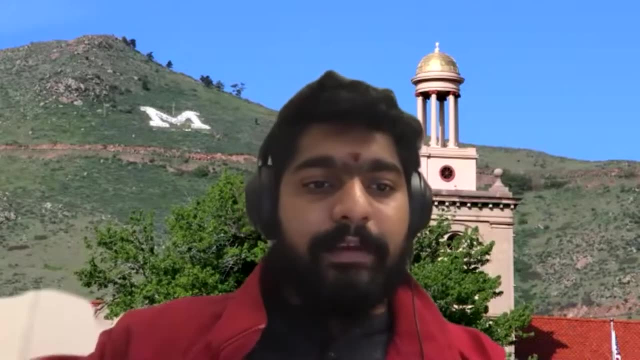 So it always considers like tree barks and things like an obstacle. So we do not give like point A to point B. Instead, we do like a waypoint navigation within, like for like, within each meter, we provide like waypoints for which the robot has to traverse upon. 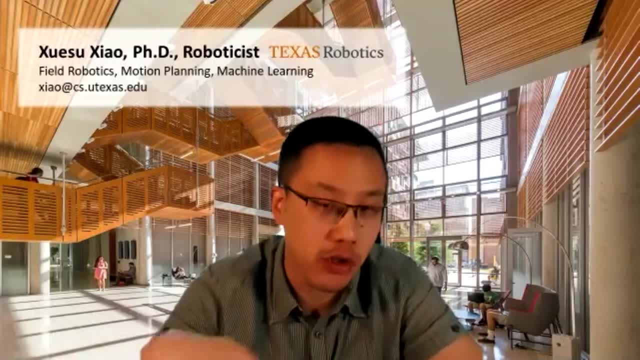 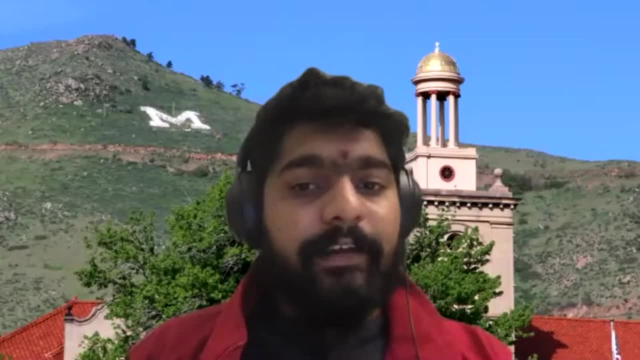 Okay, So there is a waypoint like a goal in front of the robot. you need to go to right. Yes. Yes, The robot is going. I remember in the TRAL work you do not have a waypoint. Yes, 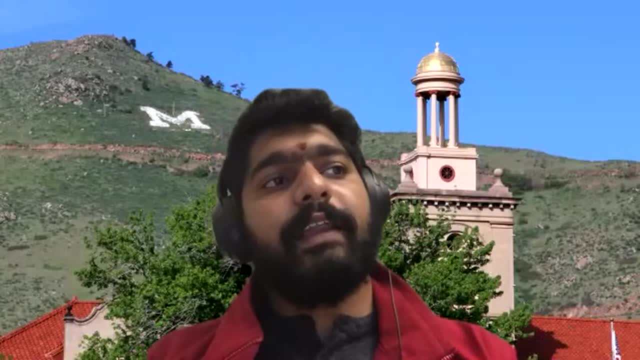 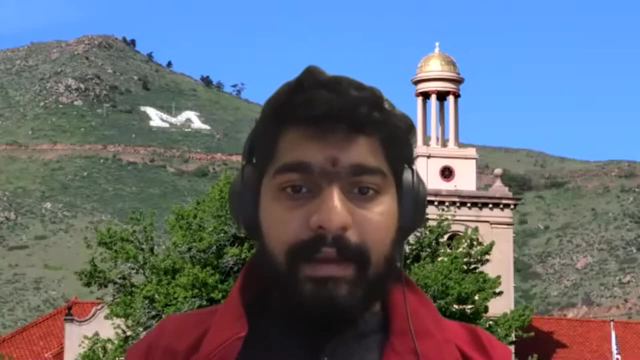 Yes, Yes, And right now what we do is we basically have like an external planner which has like point A to point B, and the TRAL approach just acts as a local controller inside of the planner, Right? So so it's used to just adjust its navigational. 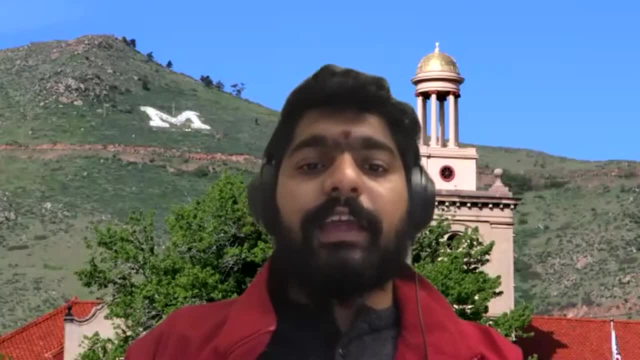 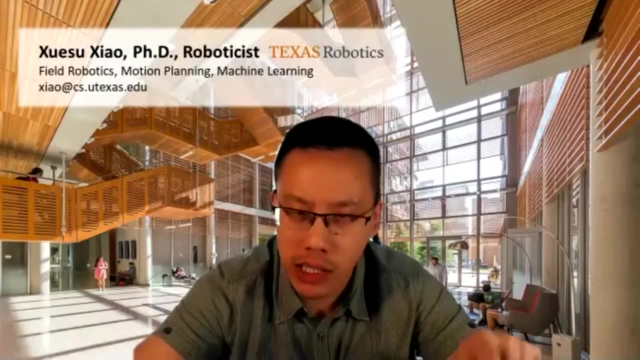 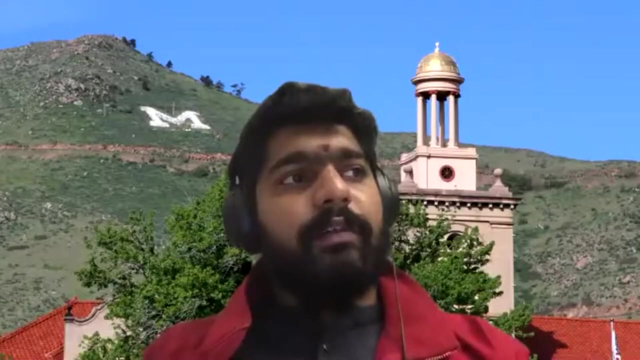 like velocity, like the, the linear velocity, as well as the steering angle of the robot Right. So how? how did you actually like inject the information regarding the waypoint? Is that part of your state representation, or Like? so what we use is the army stack. 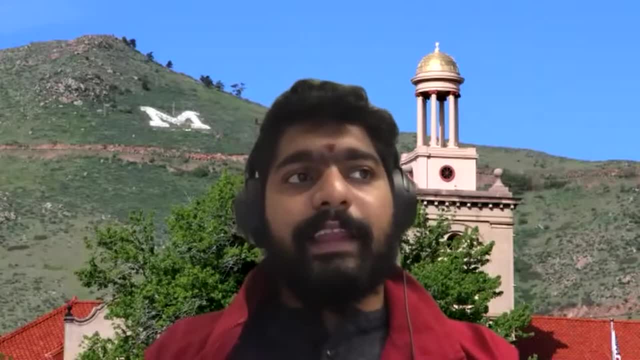 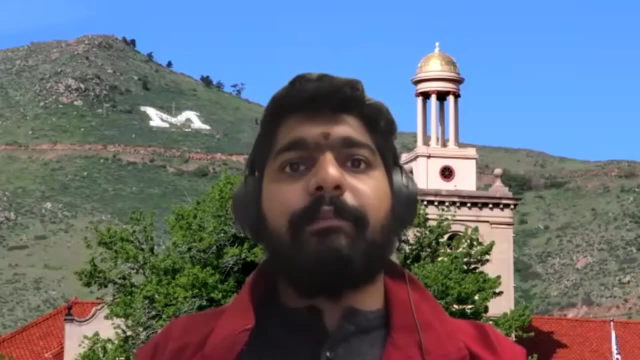 We already have like the ARL stack. So in that we use like an MPPI planner, like MPPI controller, So it generates like a local planner, like for navigating, But what we do is we override the commands which the MPPI planner has given. 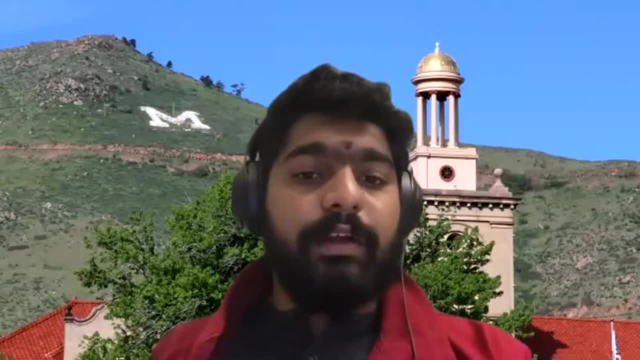 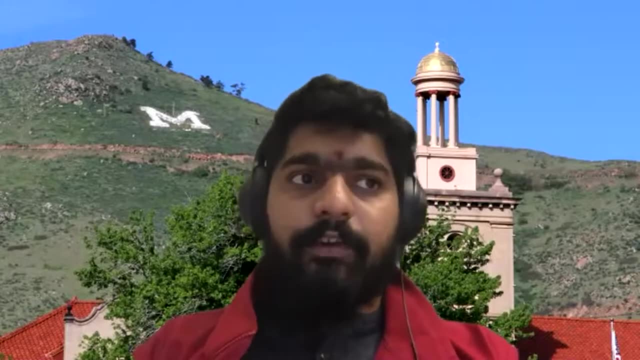 in terms of its linear velocity, And we override it with our local controller. So that's that's what we are doing. And in terms of states, I don't know if I'm answering this like if it answer your questions, but the states we use are like just the robots. 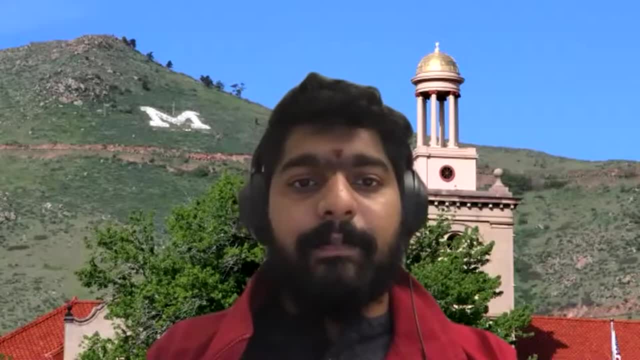 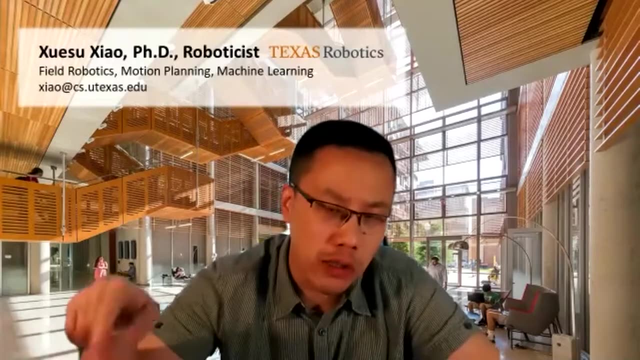 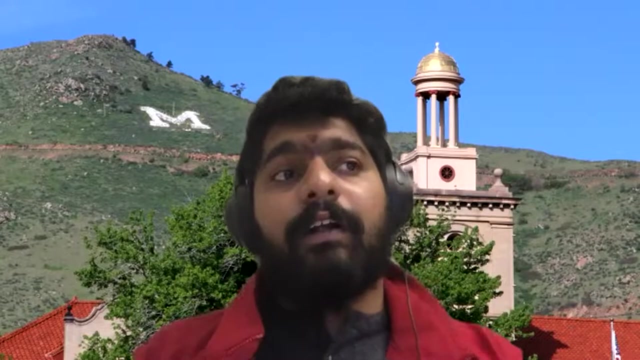 like, like the twist angles, like the linear and angular velocities, That's, that's the state angles, So that's the newer work, right? So basically, you're trying to correct the MPPI, local planners, linear velocity and the local navigational velocities. 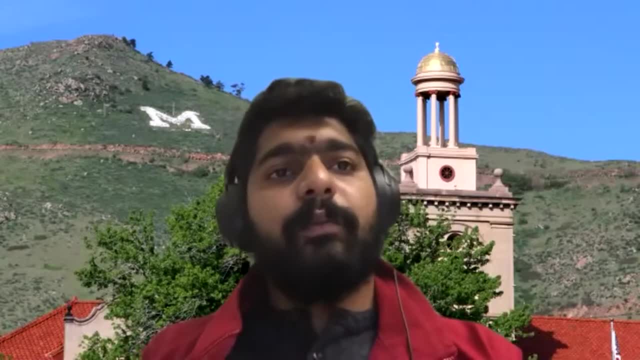 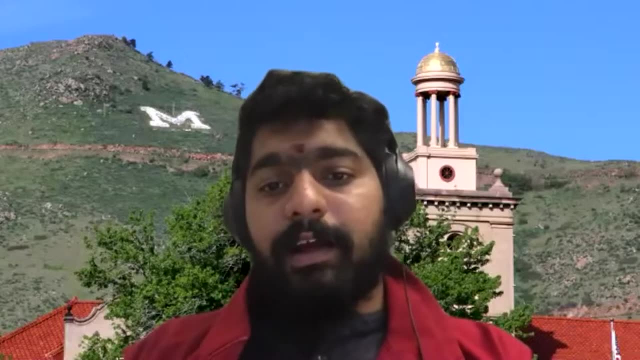 So you're trying to correct the MPPI- local planners, linear velocity and the local navigational velocities. So that's the learning method, Not essentially correct, but override it. So we didn't write it. Yeah, But so just for heading. 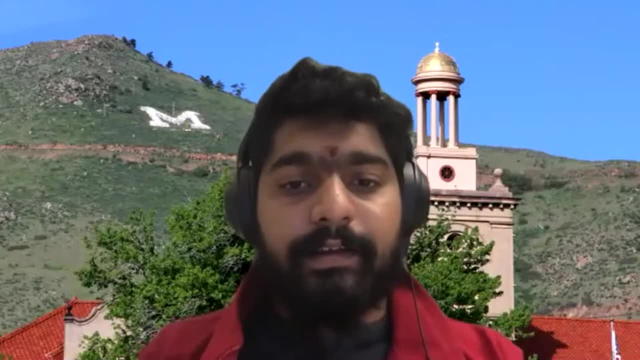 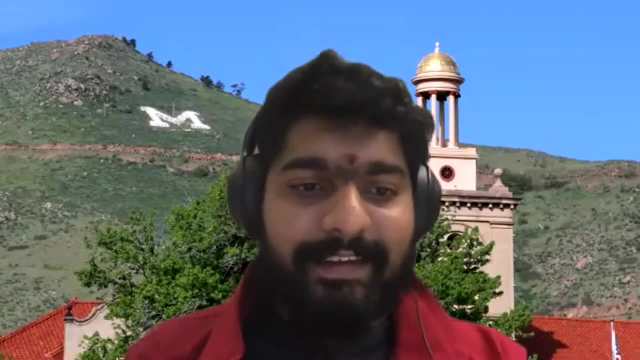 we use the MPPI as heading, but the local, like just the navigational velocities. I'm using our like TRL approach, Like that's. that's how I override it. Okay, Okay, Yes, But the video is just because. 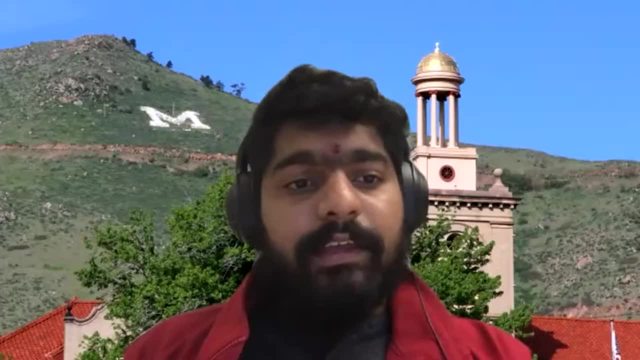 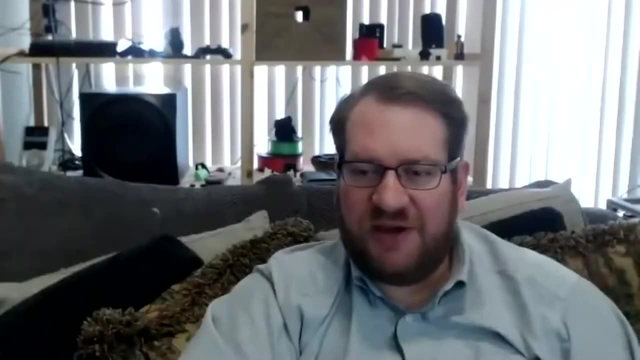 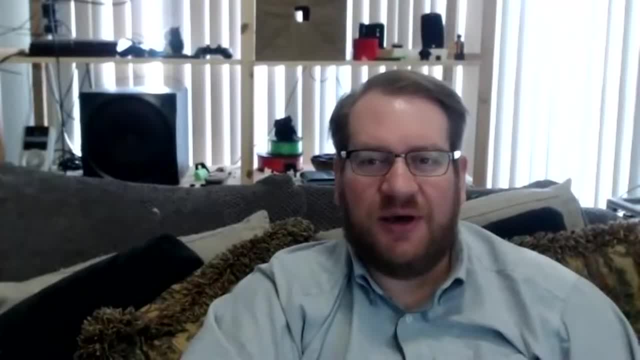 Do we have another question? Okay, So I I have one that is probably pretty quick: What, what if you, what if you train this on you know open flat terrain and had that in your data set, would that change things? 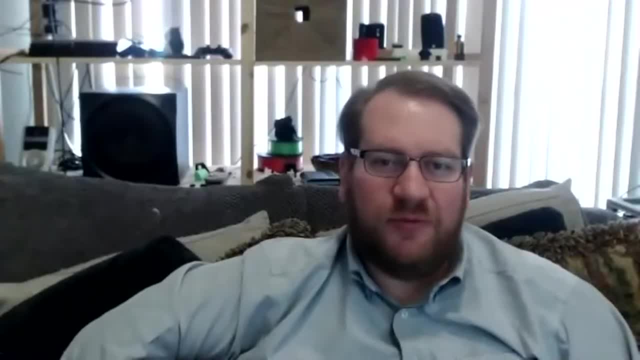 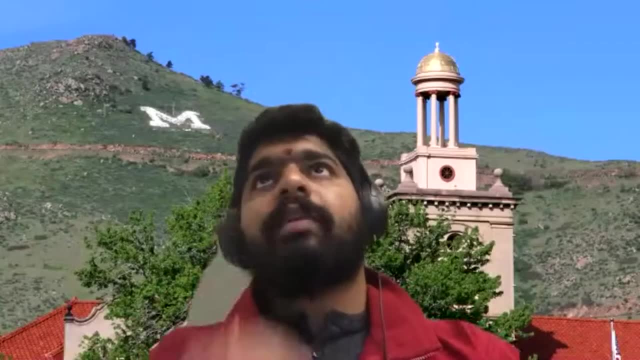 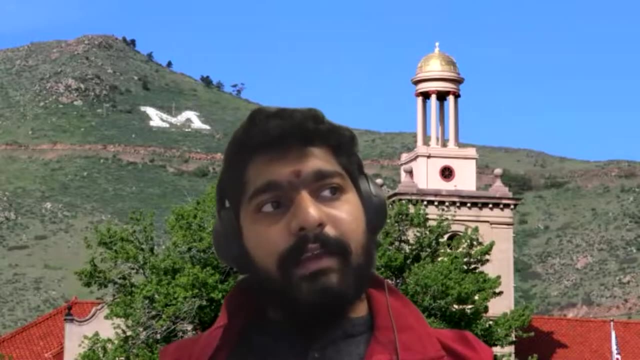 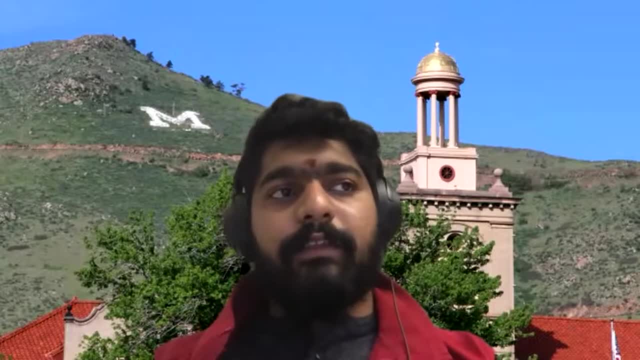 like if you have gravels in structure and as well you know you need to adjust your robot's velocity when you're training it right. So we provide like training data from human demonstrators are the ones who teach them about in this right. 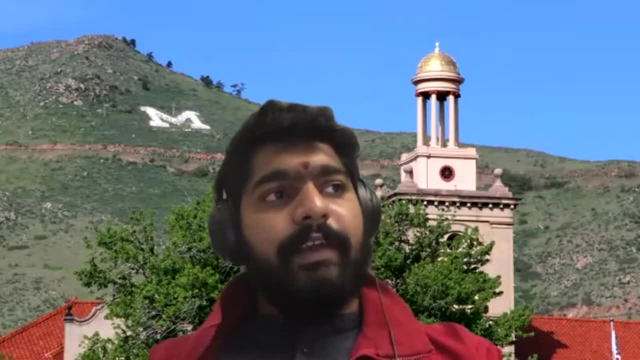 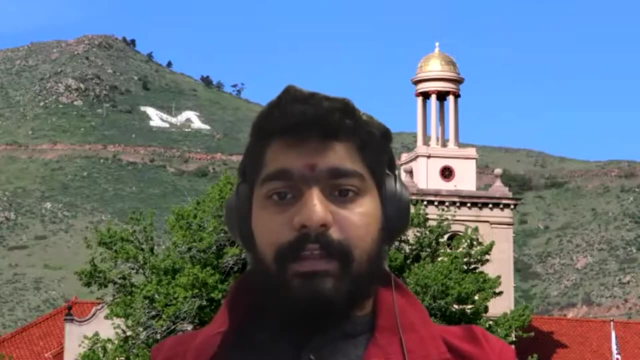 So if you are directly driving it on concrete and drugs, it's going to change a lot. But if you try to include like gravels as one of the trainings as well, and like medium-size droids, something like that And like, 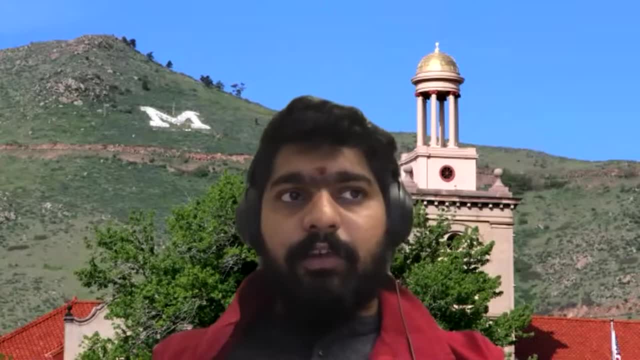 I know, tell you something. not like really large sized rocks. you can essentially see the difference, But as you include more and more types of terrains, it's really good, just because all the complex environments we see are a combination of all these different types of. 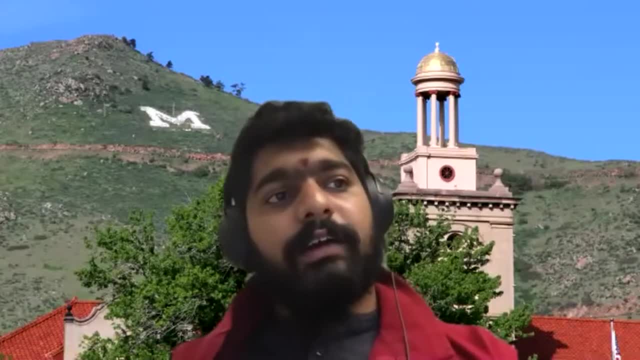 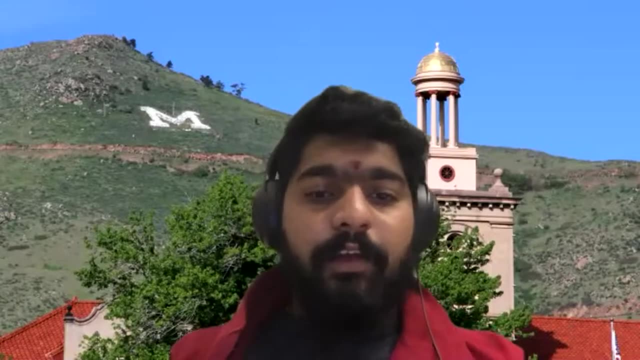 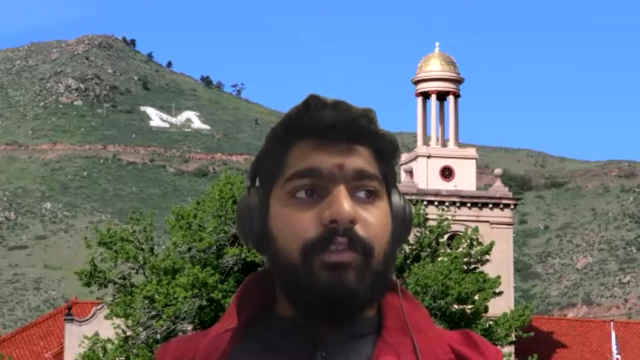 terrains. So just based on that. so I mean it is an adaptive approach which, based on feedback from how it is performing during the past few time steps, it tries to generate navigational behaviors in future time steps. But like to answer your questions? just flat terrains would limit your. 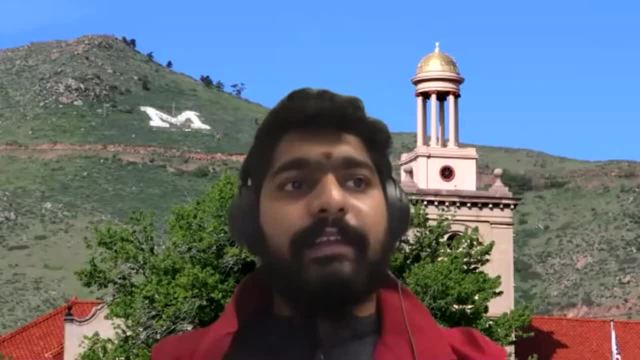 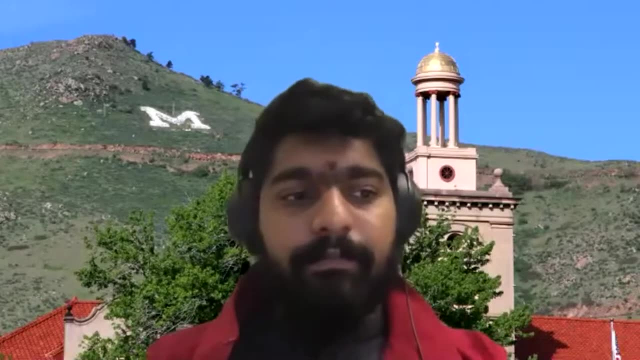 capabilities. But like I'm assuming this flatness is just in grass and concrete kind of terrains, But if you include like gravels and like medium sized rocks, that performance you would see in testing as well. Much appreciated, All right, well, I guess. 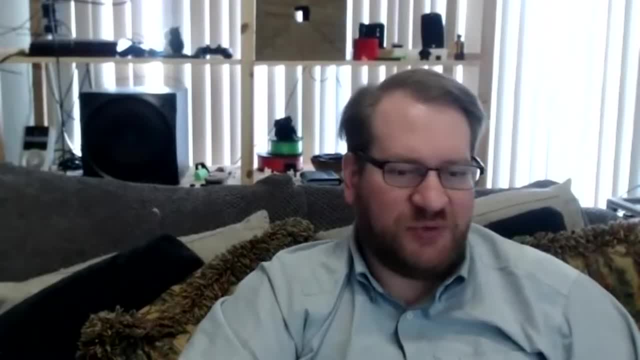 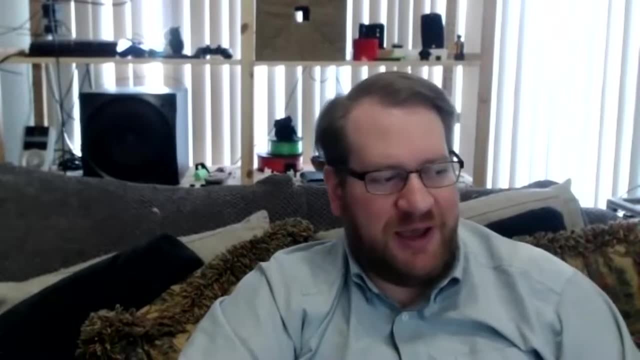 we're coming to the end of our last talk session. Of course we'll have a discussion and closing remarks after, But this is the last talk of the symposium And our presenter is Bo Liu from UT Austin. I'm going to go ahead and run that video. 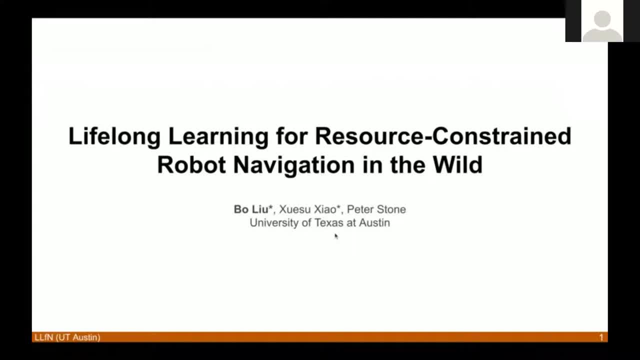 Hello everyone. Today I'm going to introduce our work: Lifelong Learning for Resource Constraints: Over the Navigation in the Wild. My name is Bo Liu, and this is a joint work with Xue Su Xiao and Peter Stone at the University of Texas at Austin. I'm going to introduce our work Lifelong Learning for Resource Constraints- Over the Navigation in the Wild. My name is Bo Liu, and this is a joint work with Xue Su Xiao and Peter Stone at the University of Texas at Austin. I'm going to introduce our work Lifelong Learning for Resource Constraints: Over the Navigation in the Wild. My name is Bo Liu, and this is a joint work with Xue Su Xiao and Peter Stone at the University of Texas at Austin. 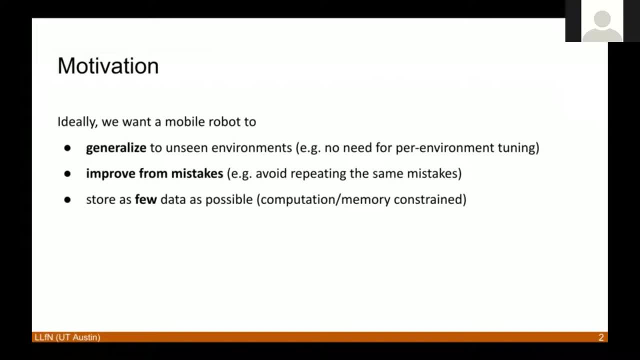 Speaking of the motivation, ideally we want to design a mobile robot to generalize to on-scene environments, So there is no need for per environment tuning, And also we wanted to improve from mistakes so that it won't repeat the same mistakes multiple times. And also we wanted to store as few data as 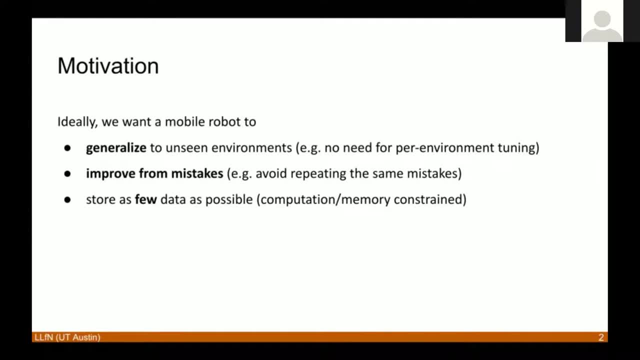 possible due to the computation and memory constraints. So if we take a look at classical planners and learnable planners, we will see that classical planners are very good at generalization, So a single algorithm can apply to most of the environment. However, whenever a classical 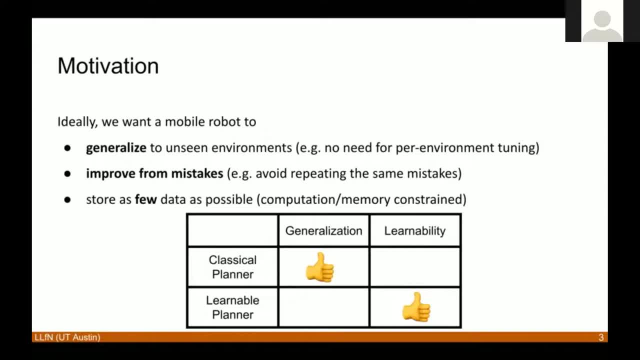 planner makes a mistake, it's very hard to improve from that mistake. On the other hand, learnable planners are designed to learn from those mistakes within a single environment, But usually they are very bad. they generalize badly to on-scene environments. 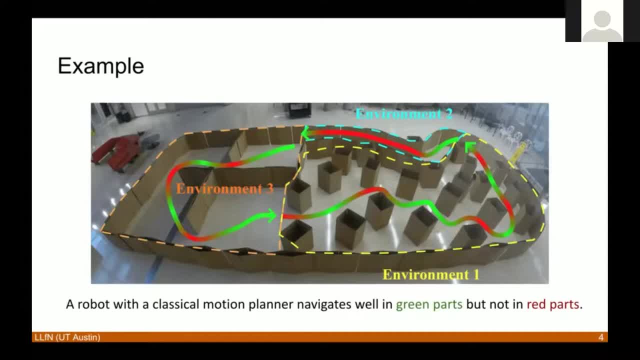 So, for example, here there is a robot with the classical motion planner navigating in three consecutive environments And we label those parts where the robot navigates less smoothly in red. The robot basically cannot learn from those mistakes, even if we apply it in the three environments multiple times. 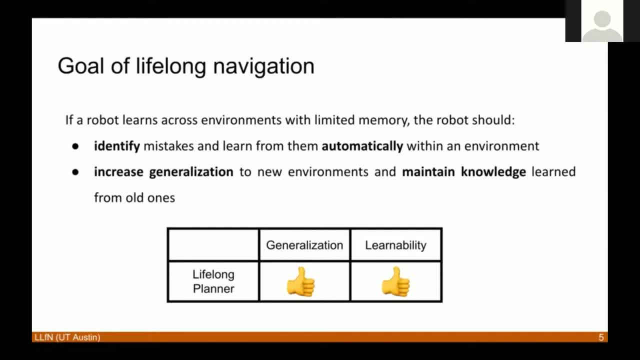 The goal of Lifelong Learning for Resource Constraints Over the Wild is to improve on the knowledge-to-learn ability of one or more of the three environments the robot uses to learn. So the lifelong navigation is to make a robot that learns across environments with limited memory. 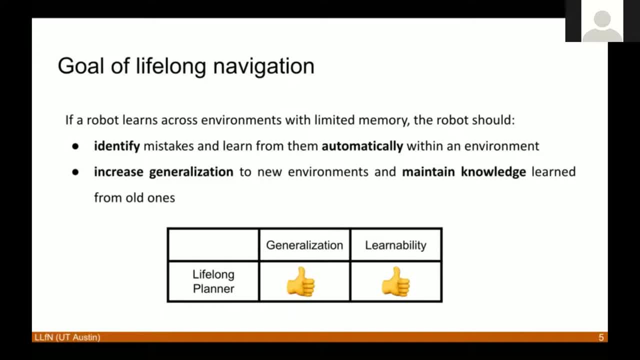 And the robot should identify mistakes and learn from them automatically within the environment and also increase the generalization to new environments while maintaining the knowledge learned from the old ones. In short, a lifelong planner should be good at both generalization and learnability. In short, a lifelong planner should be good at both generalization and learnability. To this end, we propose the Lifelong Life Plan. A lifelong plan should enhance your life style and enhance your ability to learn about both new and old. To this end, we propose the Lifelong Life Plan, which will place your life in a more flexible environment and will make you more creative in what you are doing. 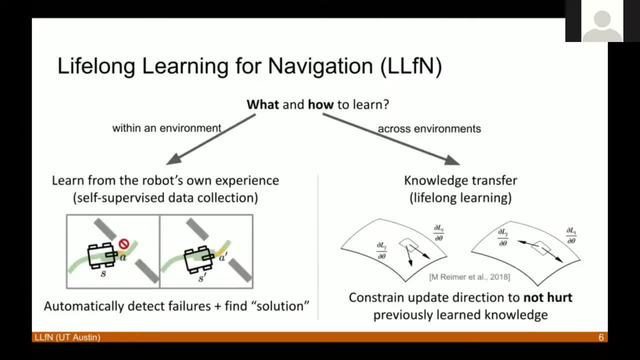 To the end of this chapter, we propose the Lifelong großer, which will also help you to increase your learning, and the Lifelong Learning for Navigation, the LLFN framework. Basically, it answers what and how to learn Within a single environment. 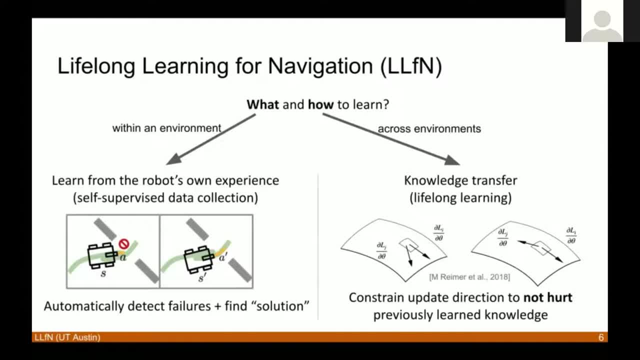 we want the robot to learn from its own experience. This step we call the self-supervised data collection. Basically, the robot should automatically detect the failures and find the solution Across environments. we want the robot to do knowledge transfer and, essentially, the lifelong learning. 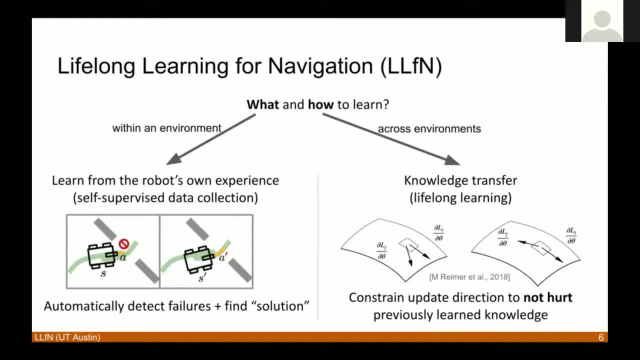 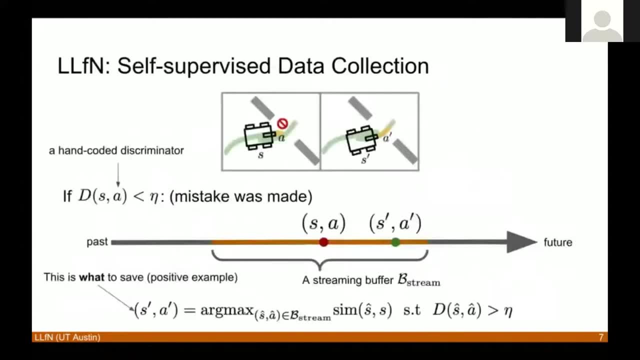 Here we adopt the method to constrain the outdated direction to at least not hurt the previously learned knowledge. We will explain in more details later. For the self-supervised data collection part, we design a hand-coded discriminator D that takes in a state S and an action A and outputs a score. 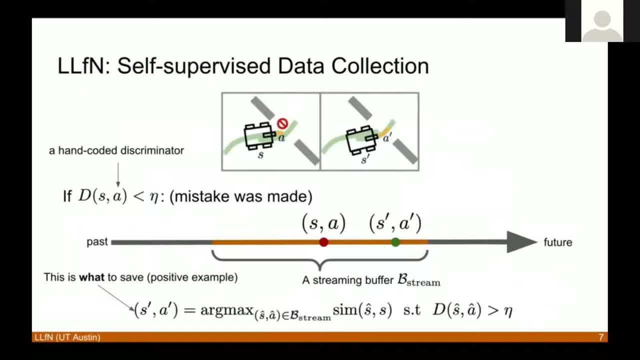 The score is higher the better. So whenever the D of SA is below some threshold, eta we say a mistake occurs. We use the streaming buffer B-stream to keep track of the robot's path trajectory And if we take a look at a state-action pair SA in the B-stream, 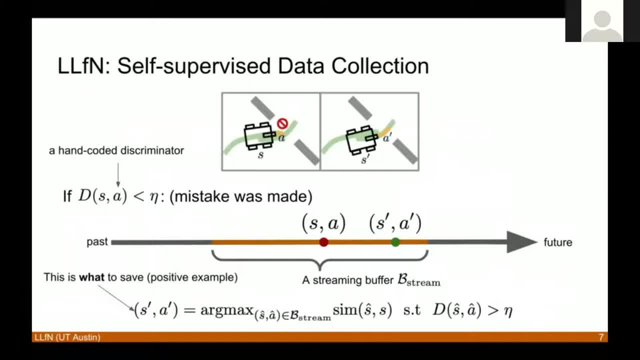 such that D of SA is below the threshold. then we look for the most similar state S' to the state S, such that the action A' at the state S' has a higher score above the threshold from the discriminator D. And this S' and A' is what we want to save. 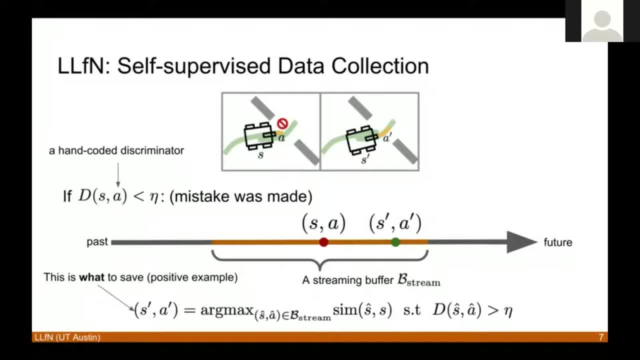 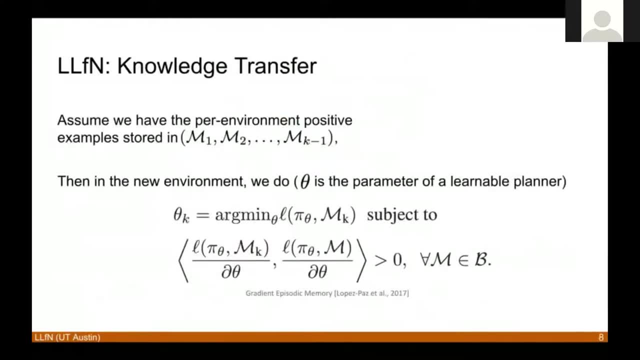 and what we want to learn from. We call these positive examples. After we save those positive examples from all of these previous environments in a separate buffer: M1,, M2, up to Mk-1, and now we are learning in environment K. 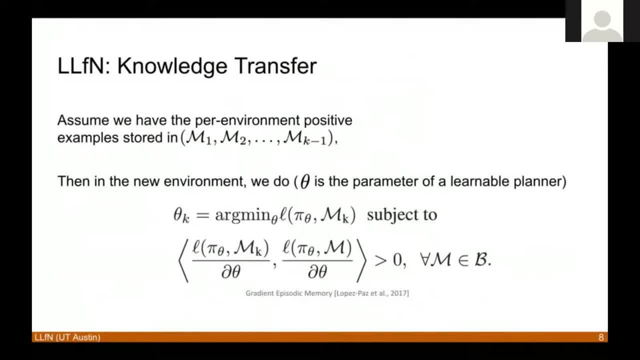 In this new environment we do the following update: Basically, we minimize the loss on the K-th environment. subject to that, the gradient on the K-th environment shares a positive angle with the gradient from the previous environments evaluated at those positive examples. 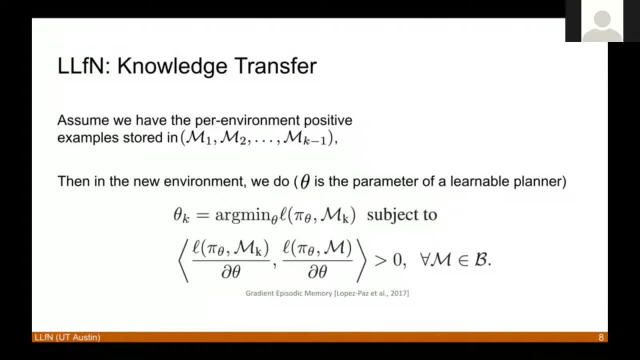 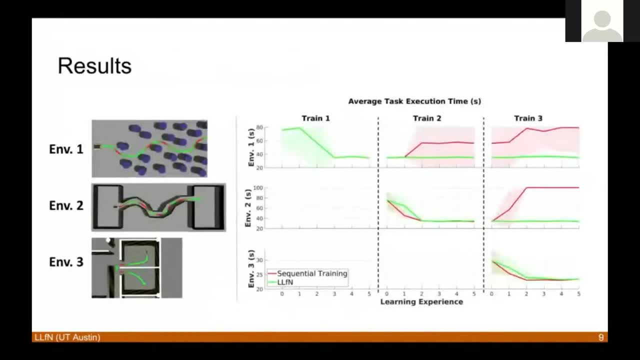 This is a standard trick called a gradient episodic memory from the Continued Learning Community. Next we see some results from the three simulated environments. We provide the overview of those environments on the left And we label those parts where the robot navigates less smoothly in red. 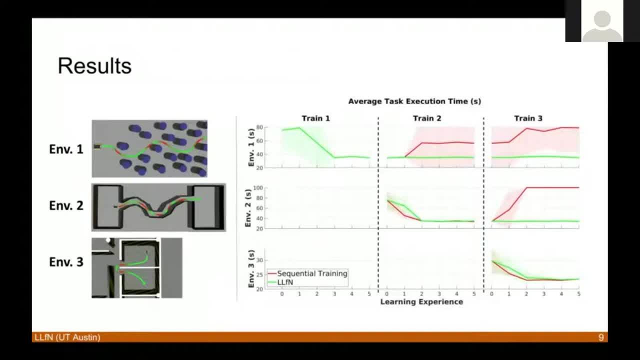 On the right we provide the average task execution time of the robot, evaluated in one environment after training on another. So if we take a look at the second plot on the first row, it evaluates the robot performance in the first environment after training on the second. 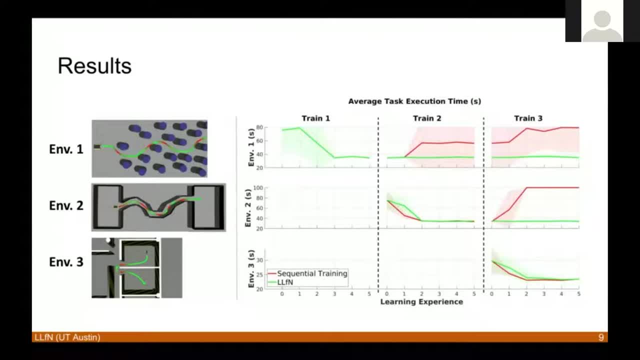 Here we compare sequential training with LLFN. Sequential training refers to the method that simply sequentially trains over those environments without any further consideration. So after training on the first environment we see that because the robot can learn from its own mistakes. so both sequential training and LLFN achieve the same result. 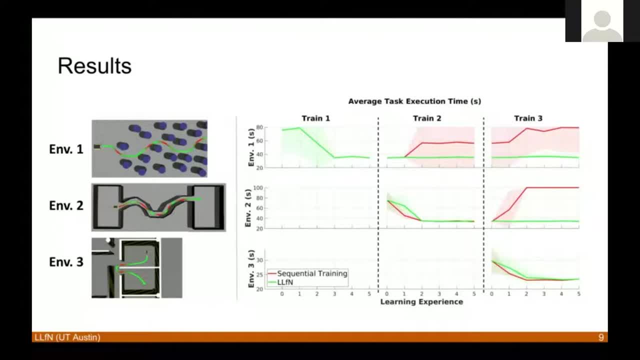 That's the top left plot. However, after learning on the second environment, if we take a look at the second plot on the first row, we see that LLFN is able to keep the performance in the first environment, but sequential training forgets. 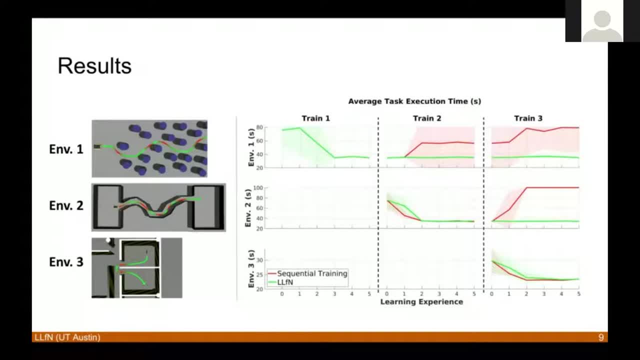 about what it has already learned and the performance drops drastically. The same pattern continues to the third environment. So here we see that LLFN is able to generalize and also maintain the knowledge from the old environment. Just to summarize in this work: 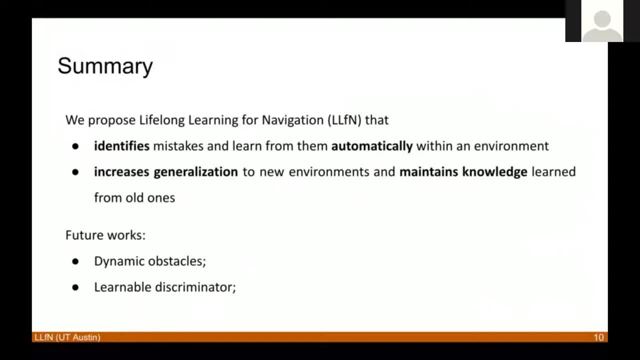 we propose lifelong learning for navigation that identifies mistakes and learns from them automatically within a single environment, and also increases generalization to new environments and maintains knowledge learned from the old ones. Future works include incorporating dynamic obstacles to the LLFN framework, and also it's possible to design a learnable discriminator. 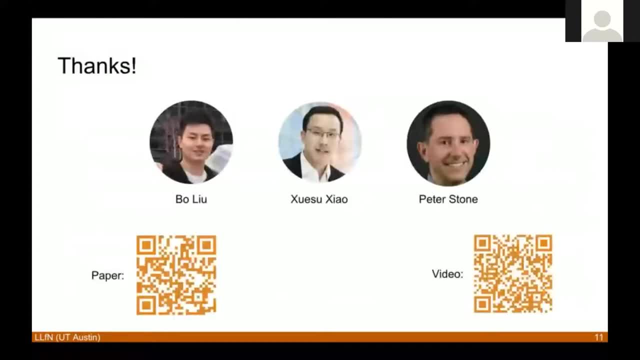 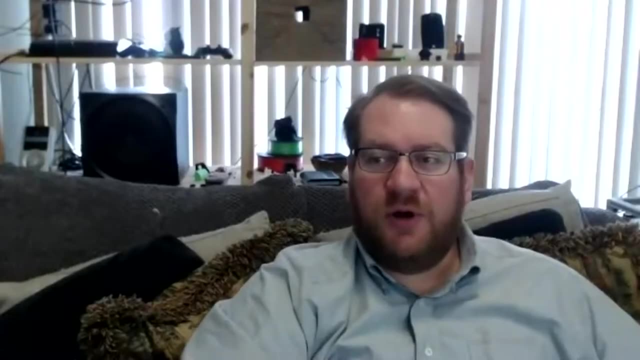 instead of a hand-coded one. Thank you very much for listening, and we'll provide the QR codes for our full paper and video of a physical experiment. Thank you Well, thank you, Bo. Let's all thank our speaker and open the floor to questions. 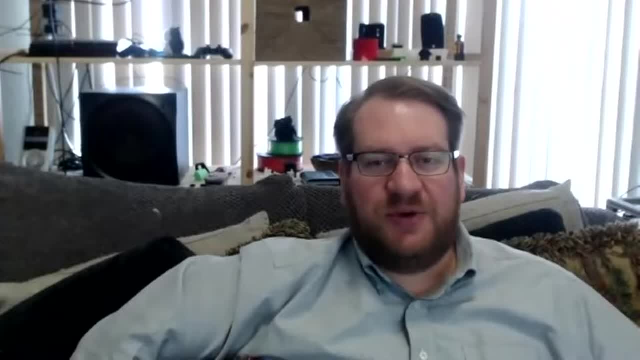 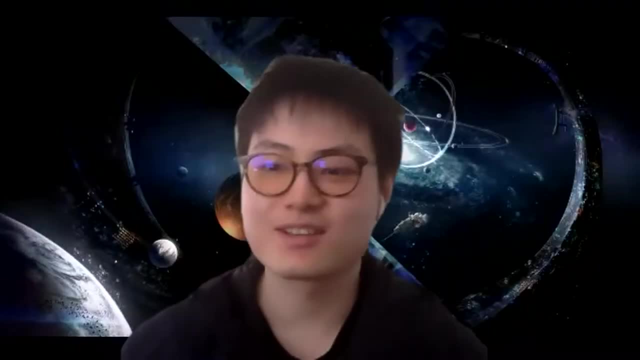 Can you tell us a little bit about your plans as it relates to dynamic obstacles, And are you looking at this in the multi-robot case as well? Yeah, so yeah, because that's also the one review we received from the REL submission. 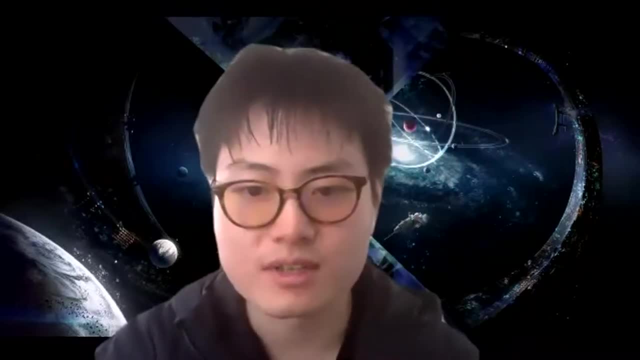 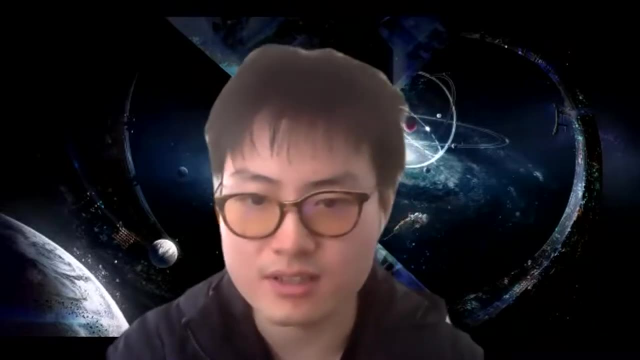 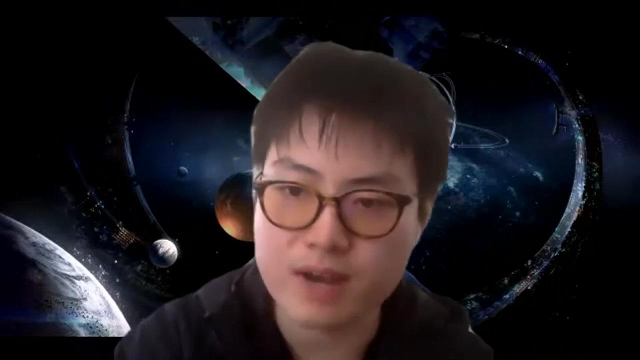 So people are more interested in dynamic obstacles. So in principle our method could apply to dynamic obstacles directly, but I can foresee that there are many difficulties. So, for example, how do you collect, like? because in our present work 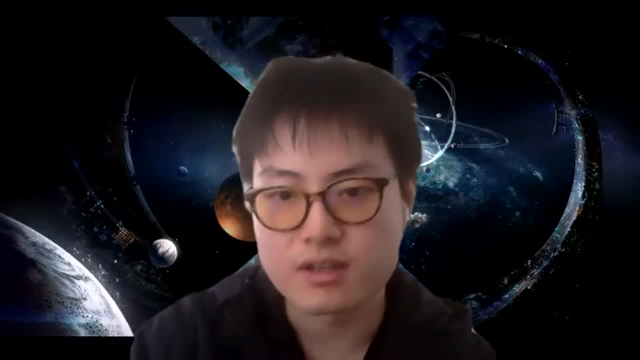 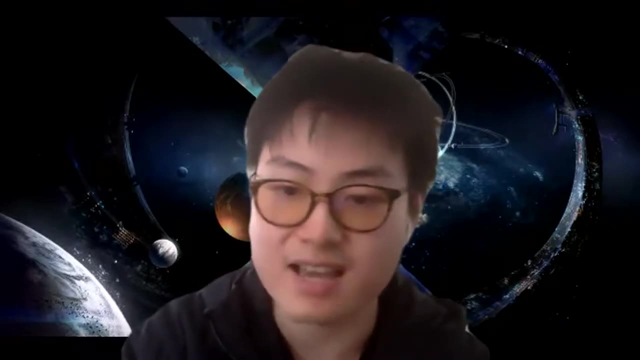 we are relying on the robot itself to find a solution automatically, but in a more dynamic environment it might be harder to define what a success move would be, And also from a long-term perspective, for example, if we want to generalize this. to multiple robots? then yeah, because it depends on what system we are using. It's either like centralized or like a decentralized system. For decentralized systems, it can be very hard, because you have to know what the others are doing. 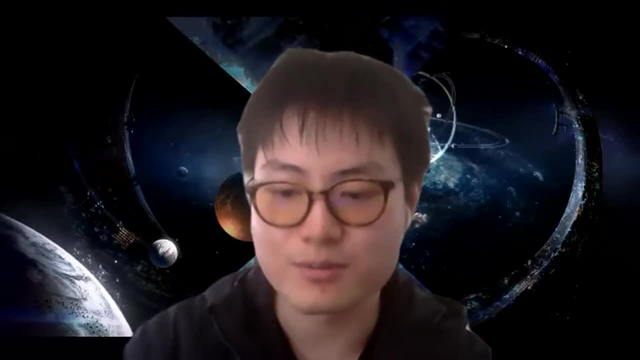 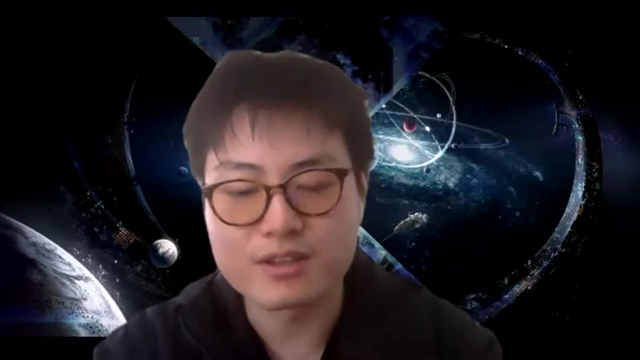 because the gradients, for example, can be very difficult for the others And basically you need to know what's the improvement of the other strategies in order to improve yourself. So I think that that could be very, very difficult. So maybe our close plan: 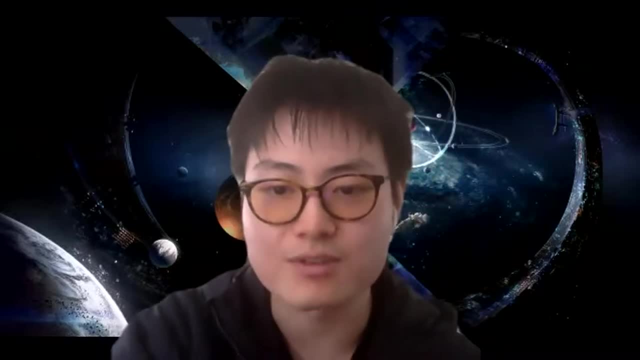 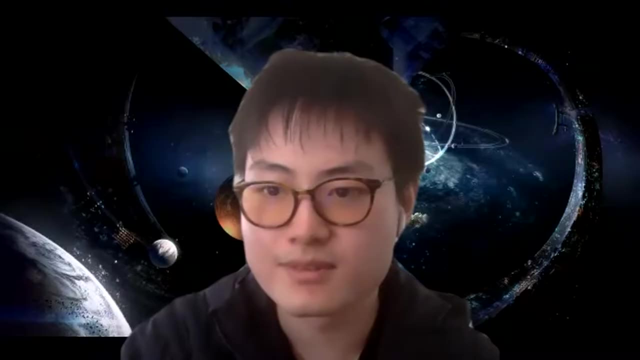 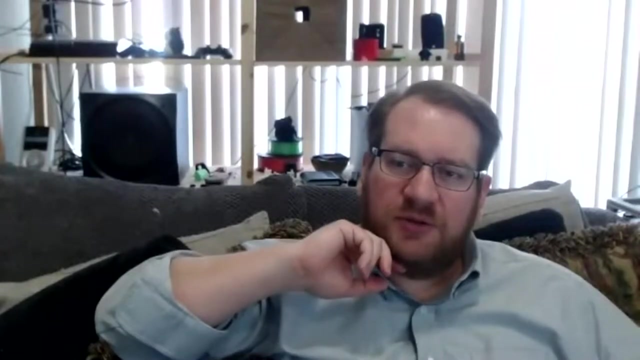 like most recent plan will be like: just generalize this to a more dynamic obstacle setting and see if that works at all. Yeah, Yeah, that makes sense. Do we have any more questions for our speaker? Well, I think we had a fantastic set. 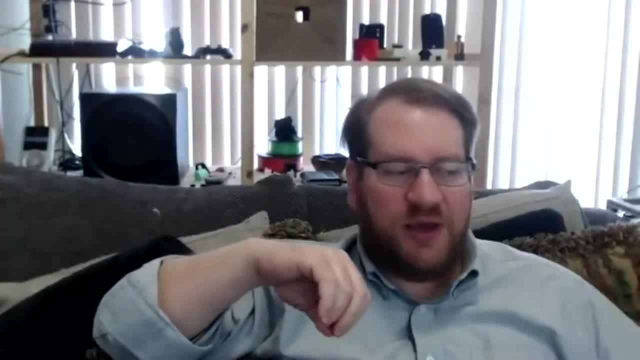 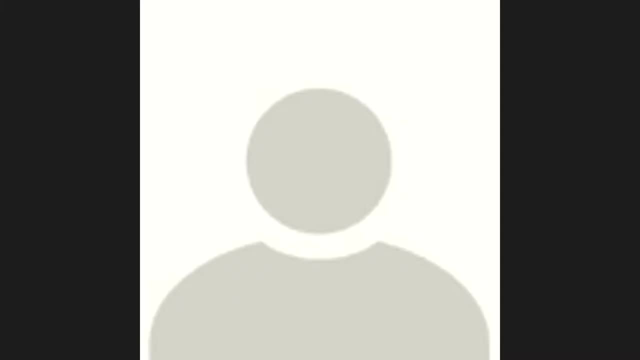 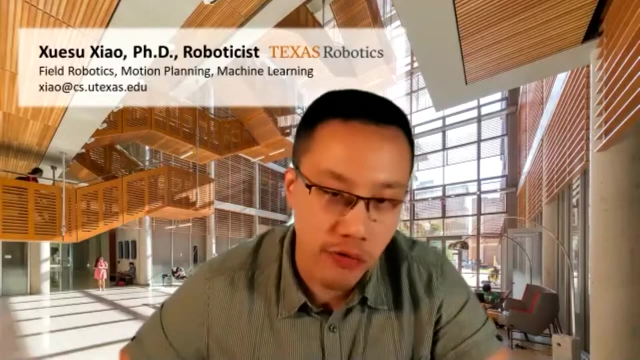 of talks this morning, I'm going to go ahead and turn it over to Zui Xu to lead our kind of closing discussions. Sure, yeah, Thanks Justin. Yeah, I think we have a very nice set of talks this morning. So I guess now is the last free discussion session. 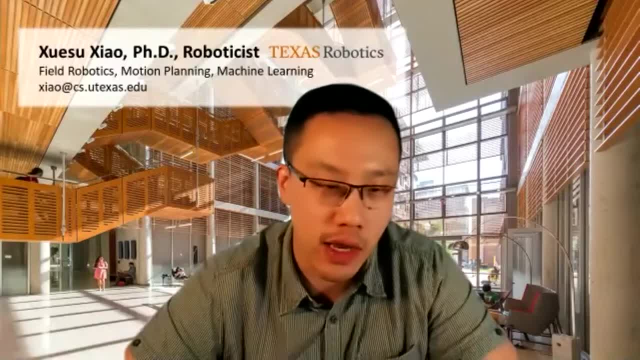 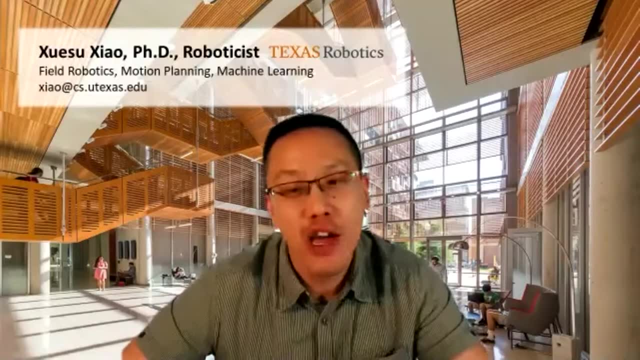 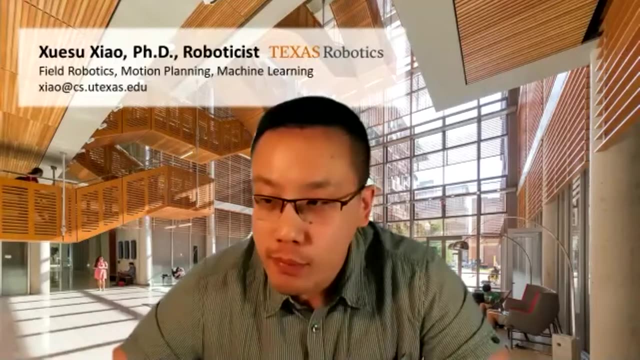 So feel free to unmute yourself And if you have any like ideas, suggestions, comments on- I don't know- the whole general case, general idea of applying machine learning for mobile robot navigation in the wild, please feel free to chime in. 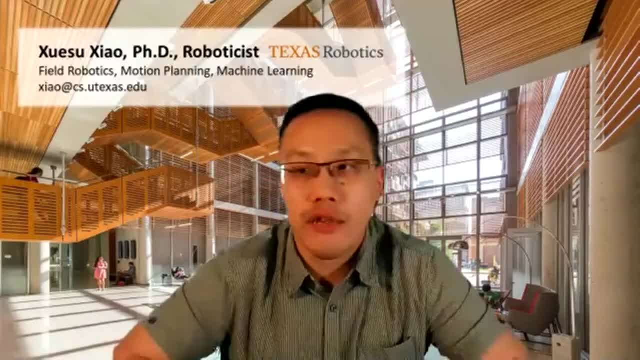 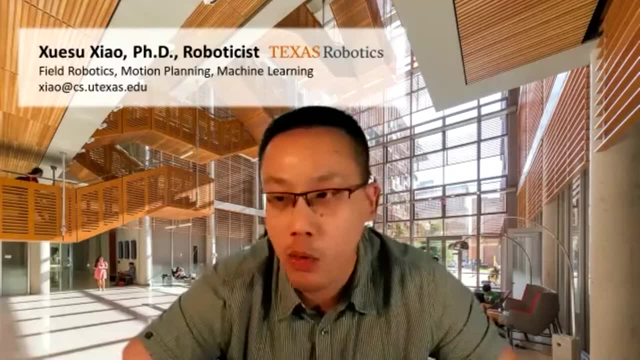 Yeah, we have covered a lot of different things in these two and a half days. First day is mostly about navigation in unstructured environments, with a focus on outdoor environments, aquatic environments, lots of nice talks and also two invited speakers in the first day. 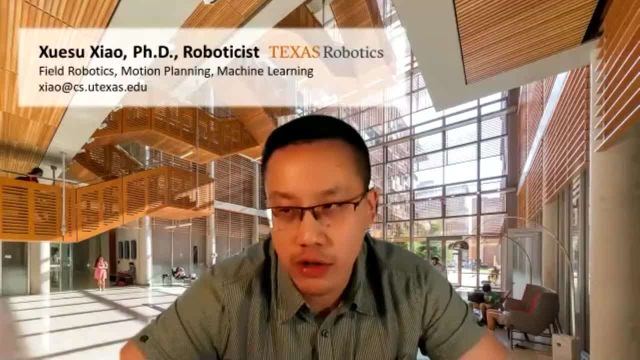 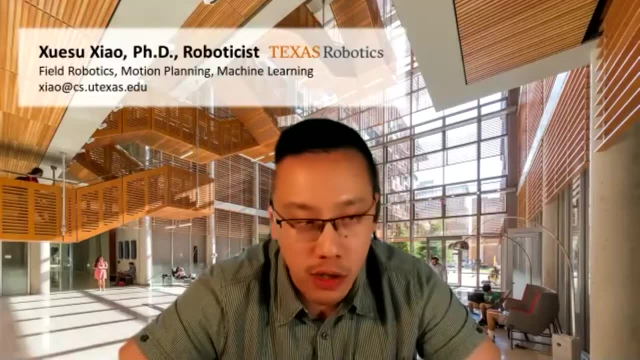 Second day is mostly a focus on social navigation with other robotic or even human agents. I think, yeah, also lots of interest on that. So today is the full day of extended abstracts, So lots of short papers presented in a shorter period of time. 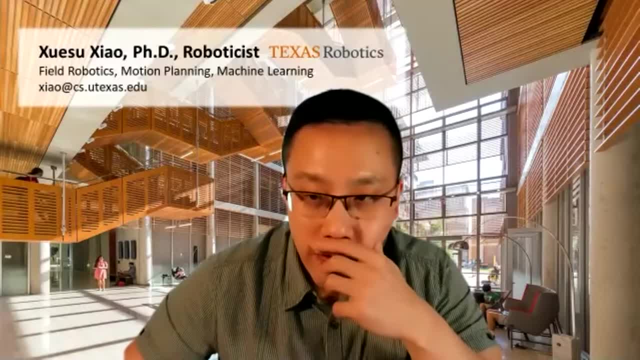 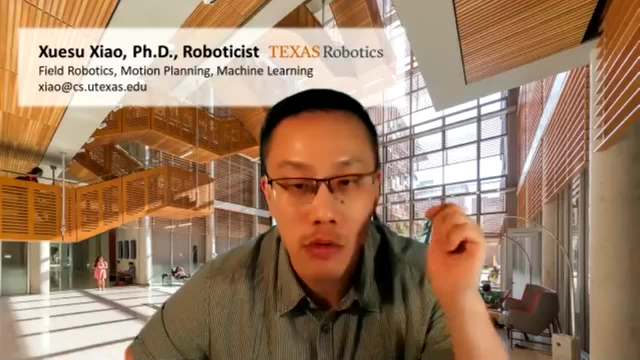 like lots of interesting ideas as well. Yeah, Feel free to like any suggestions, any comments like: where should we use machine learning for mobile robot navigation in the wild and how should we use it? Why should we use it? Yeah, 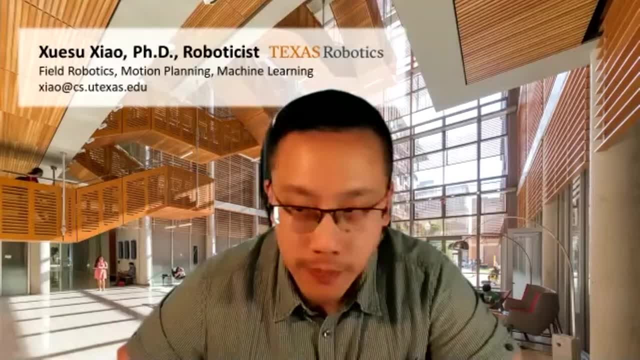 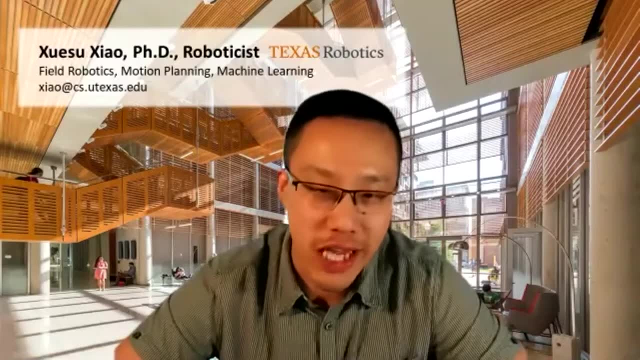 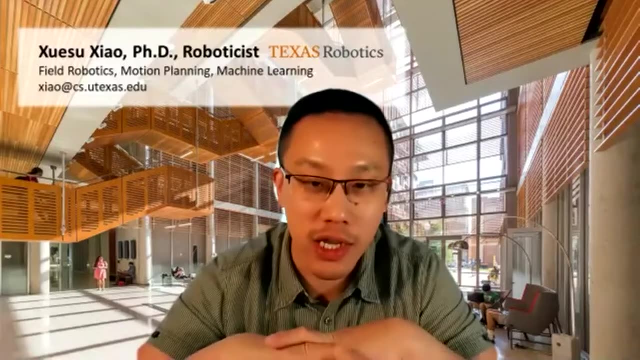 Anything if you have any thoughts. By the way, thank you for sticking around. I know it's a virtual conference. It's kind of difficult to keep people staying till the end. People have other commitments, but that's okay. Like we still have a pretty decent attendance right now. 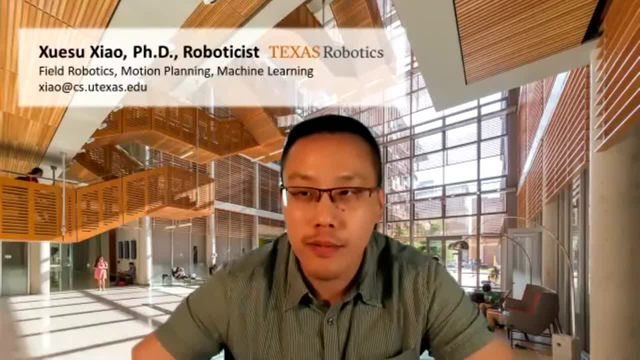 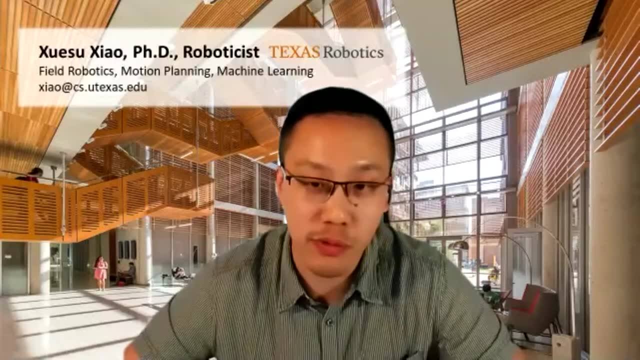 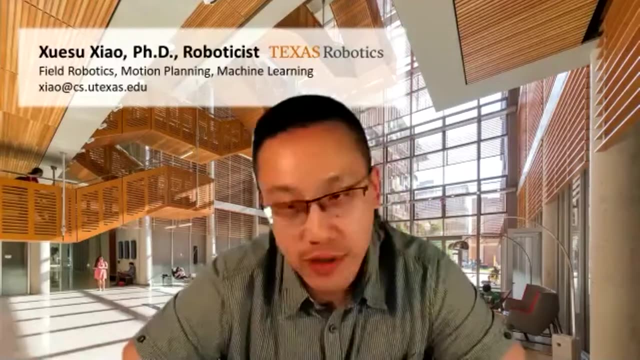 Yeah, Yeah, hopefully we can. next time we can meet in person. Yeah, this symposium is supposed to happen in Stanford, which is not possible due to the current pandemic. Yeah, If it's a better like situation, we can meet in person. 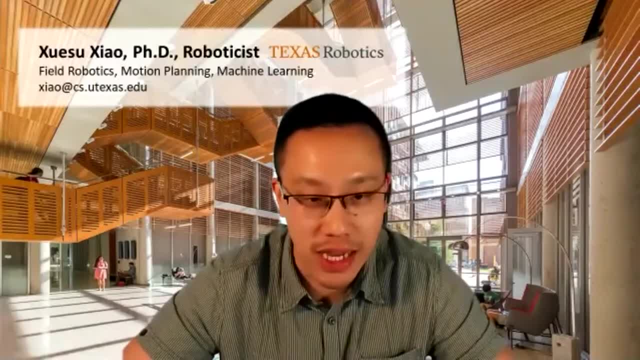 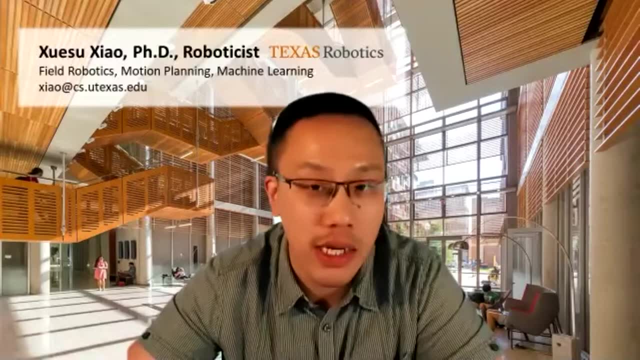 I bet it's going to be a much better attendance. People can stay till the end, physically stay till the end, Yeah, But I think it's still quite a successful symposium, like lots of interesting ideas. By the way, everything can be found on the website. 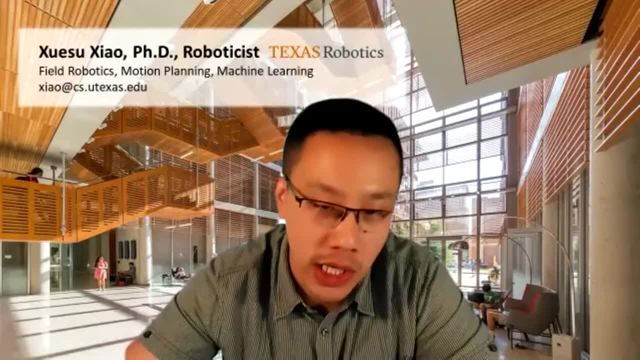 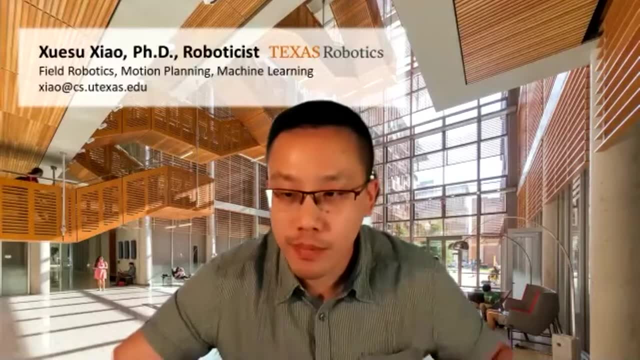 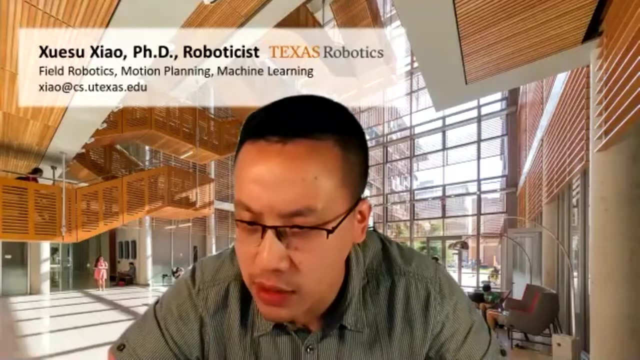 The paper presentation, the paper manuscript and all the industrial partners intro videos and some of the slides of the industrial spotlight. Yeah, I think Greg mentioned in the chat that he will be back. I don't know. Yeah, He left for a few seconds. 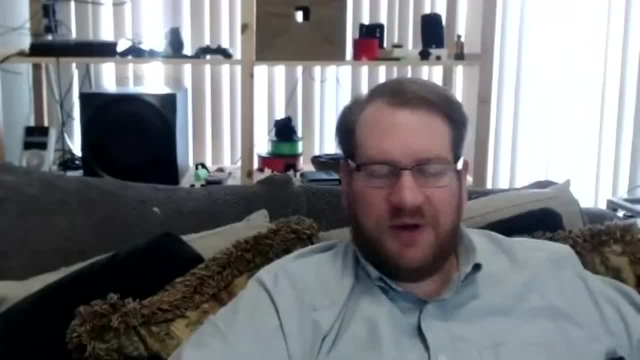 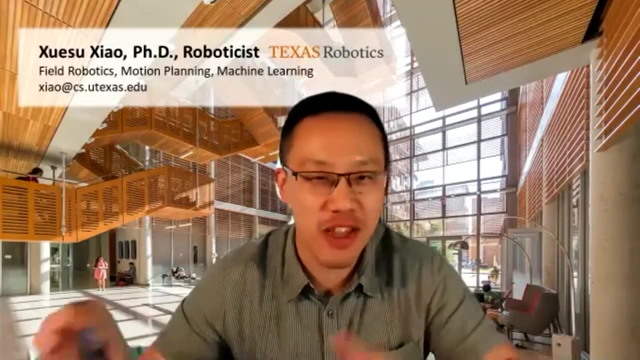 I think, Yeah, Yeah, He probably had some sort of commitment at noon. Yeah, Yeah, That's kind of the problem with those virtual conferences, right. People don't really focus on this one thing. They have other commitments at the same time. 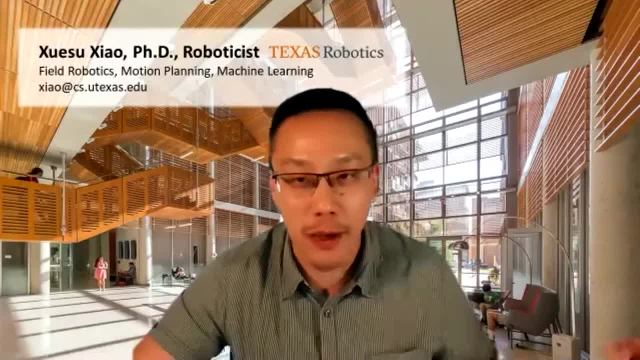 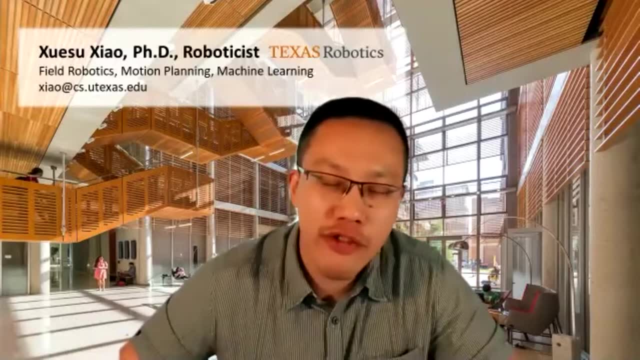 and they just, you know they need to take care of different things. Yeah, Yeah, Michael, I actually have a question for you. So you have done lots of like DRL approach for social navigation. Do you have any other? 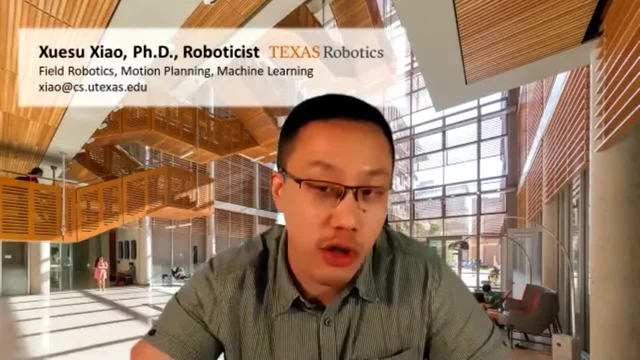 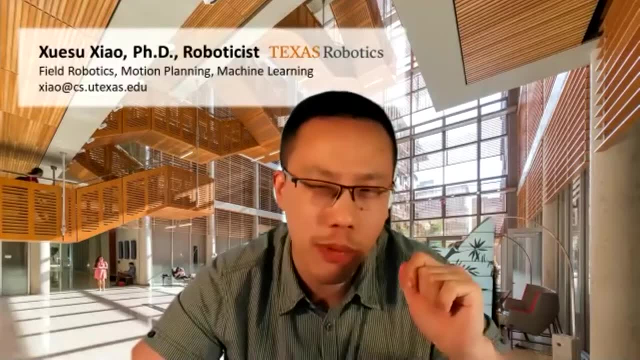 like future plans on this line. So because Harrell and I are trying to look into this problem using the hallucination or the deception idea we talked about. I talked about like during this morning session. So do you have any other? 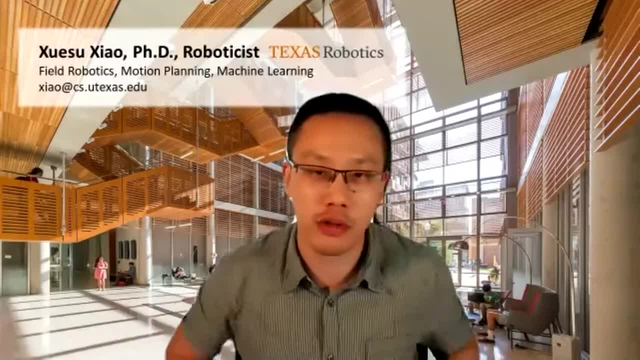 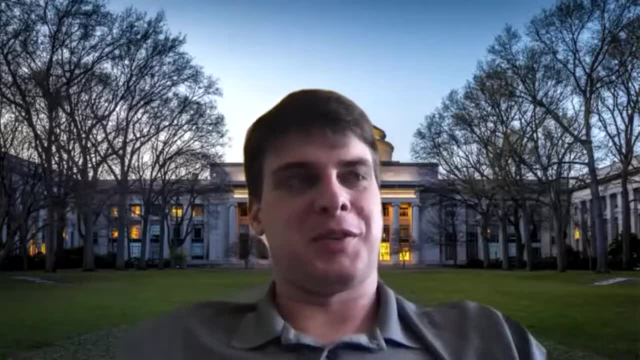 like future directions that you are trying to pursue on the social navigation end. Yeah, I was going to ask you about that. You know what do you? how do you hallucinate in a dynamic world? Yeah, Yeah, So yeah. 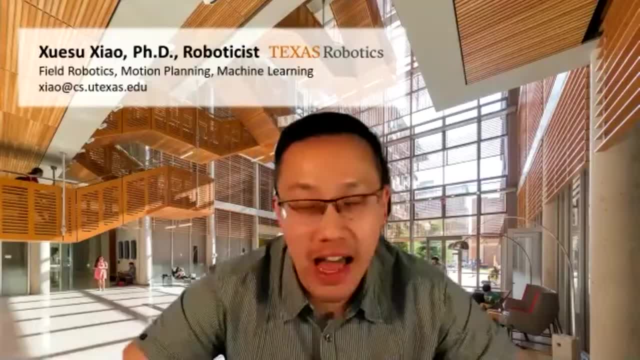 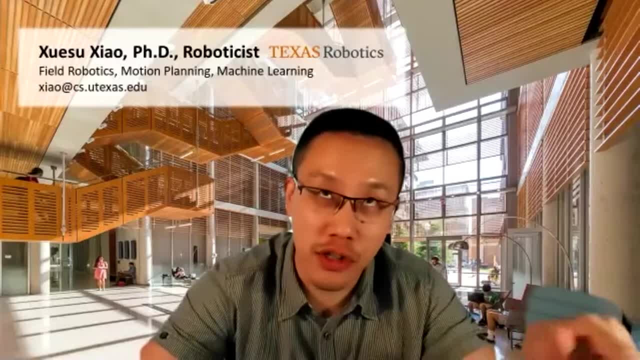 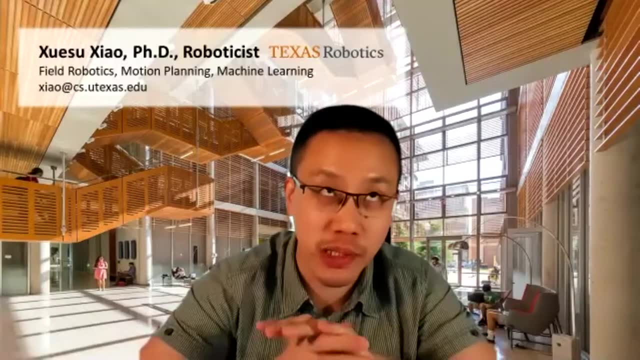 I don't know. So we are kind of like- I won't say- opposed, like the hallucination planner is also into our local planner. But we are still trying to basically leverage as much as possible from the classical work the classical motion planners. 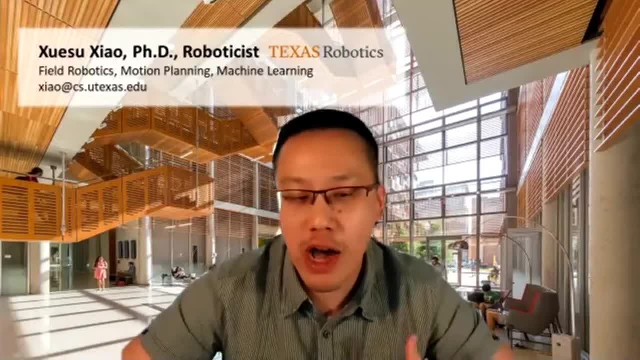 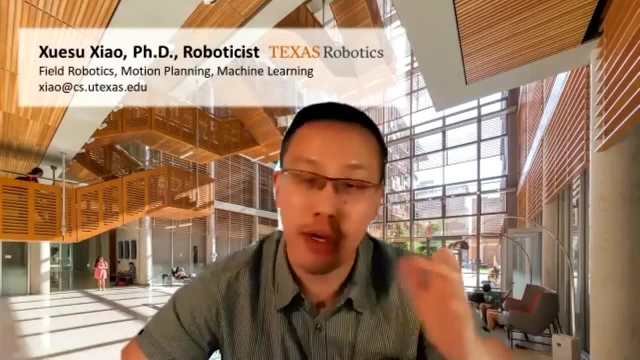 the classical robotics approaches. So hopefully, like our idea is, if we can avoid learning a local planner to do dynamic obstacle avoidance, that would be great. So, because we still like when you deploy around I don't know how, how the the Cato line of work you did. 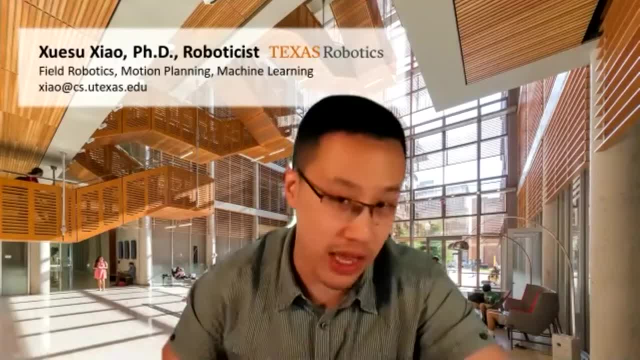 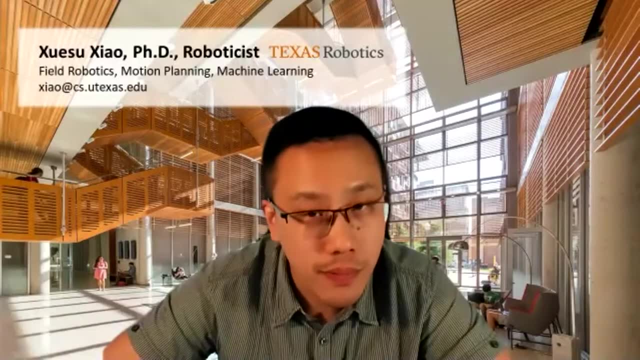 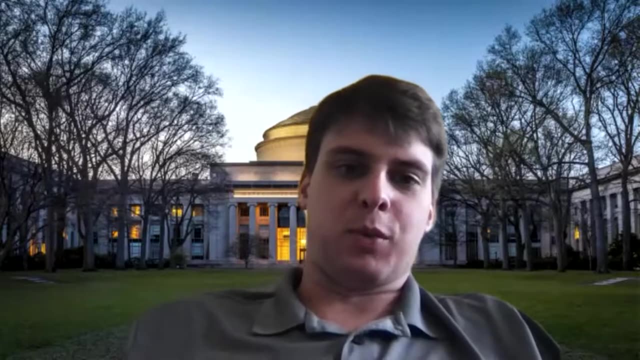 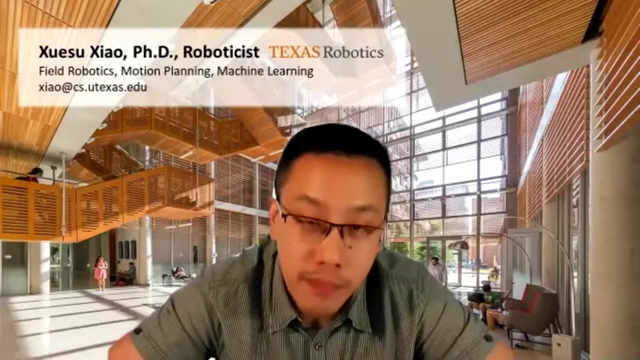 Like for is safety? you have like a safety check, like, if you are about to collide to a person, would you stop the robot? is there anything on that end? yeah, uh, we definitely, when we were doing like tests among people, we definitely had safety code in there that was to get within some radius of somebody, okay, or do something else, and i think 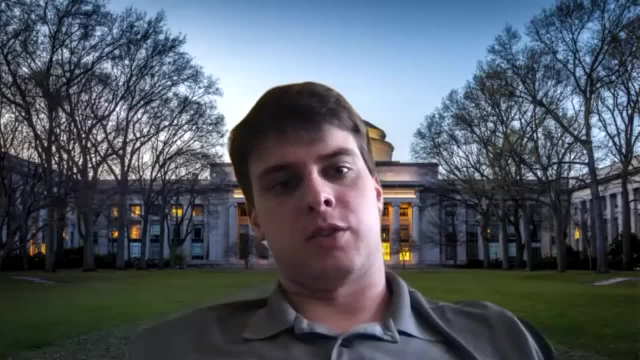 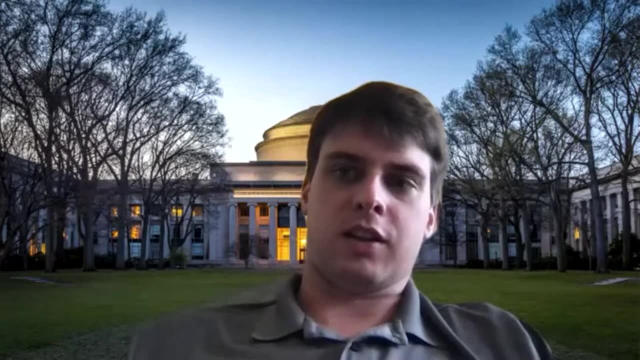 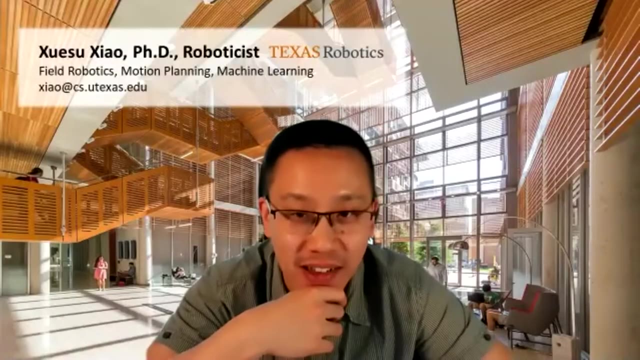 like. i think that gives you a lot of freedom then to have your robot kind of do whatever it wants when it's not in one of those kind of dangerous states. so i think that sort of um state machine infrastructure, oh, that's the same thing as the lfa, which is naturally safer. yeah, yeah, so for the 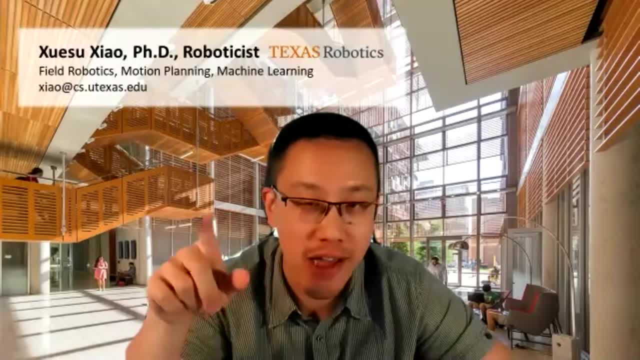 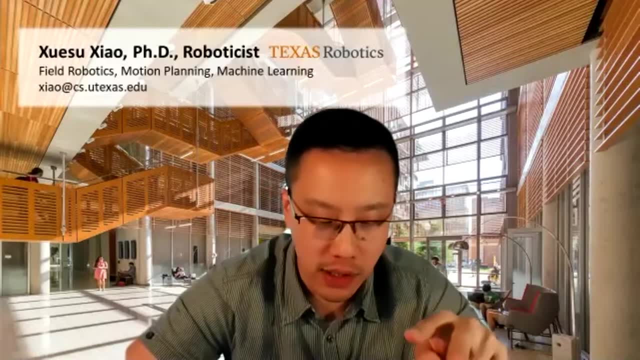 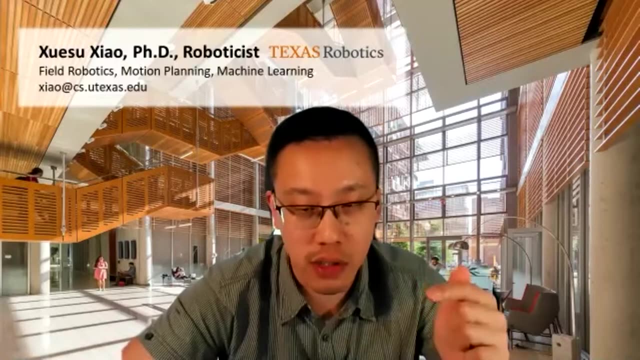 lfh worker. we also did a stage transition machine like like, whenever you don't feel safe, do some classical stuff, don't use the learn your net. so we have two uh uh plans to kind of extend this lfh for dynamic obstacles. one is to design like hallucination. 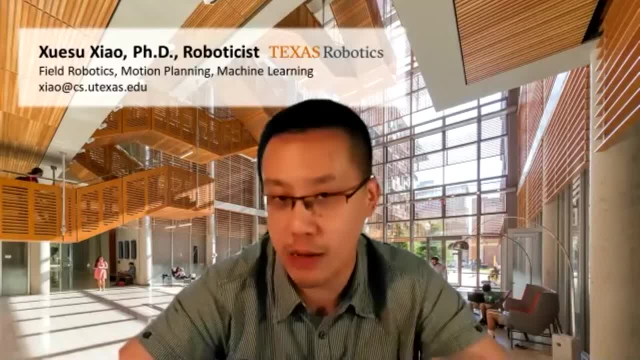 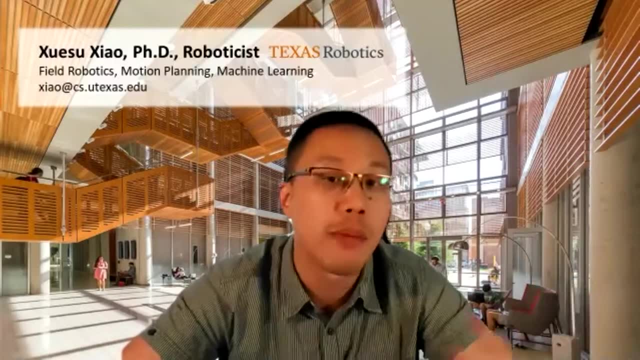 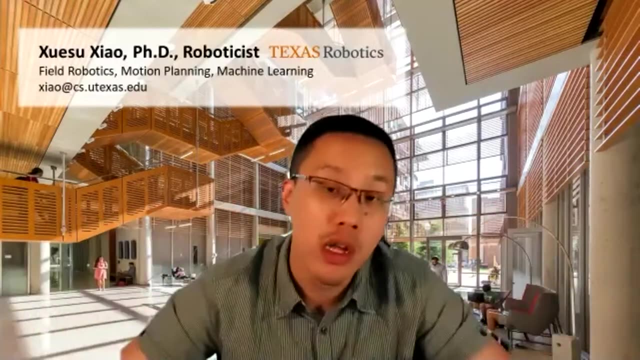 hallucinating obstacles in a high dimensional space, including time, because what you currently? we are only hallucinating the geometrical location of the obstacles to make the plan optimal. right, the other thing we can do is add the time dimension, so you are actually hallucinating the trajectory of the dynamic obstacles to make your plan optimal. that could be very difficult. 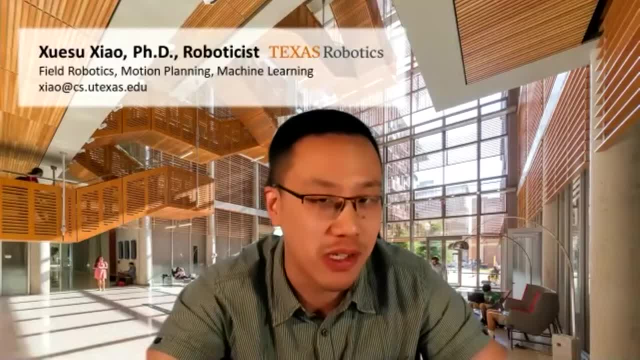 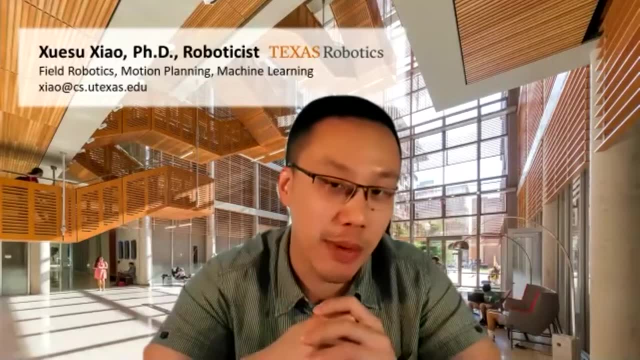 because i i still don't know how to do it. you need to think about how do you come up with. so it's actually very related with chris's talk yesterday. like the his b, like the the braid, right, it's kind of the same idea. right you have a like x, y, coordinates of the trajectory plus a time. 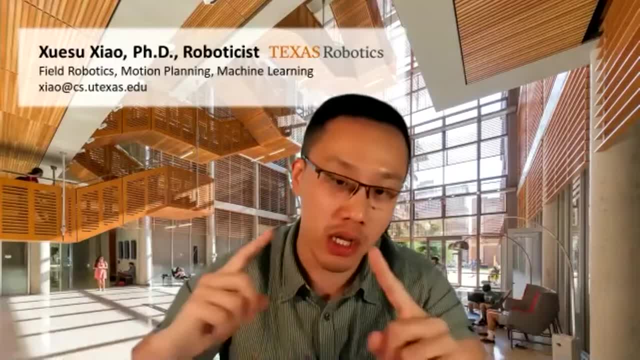 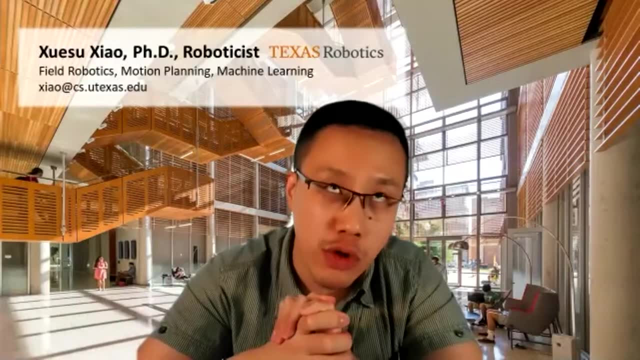 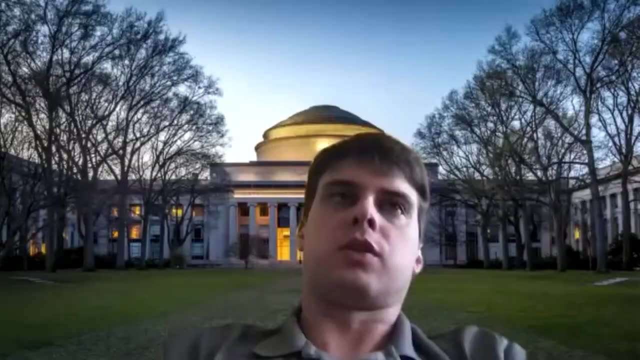 dimension. so you want to come up with all these spray to inter, leave each other, but not collide, right? that's chris's take on this. i think there could be a hallucination strategy that on like from the same idea: right, adding this one, right, so you're. you're hallucinating right now in position space. yeah, but i'd say a lot of the work in. 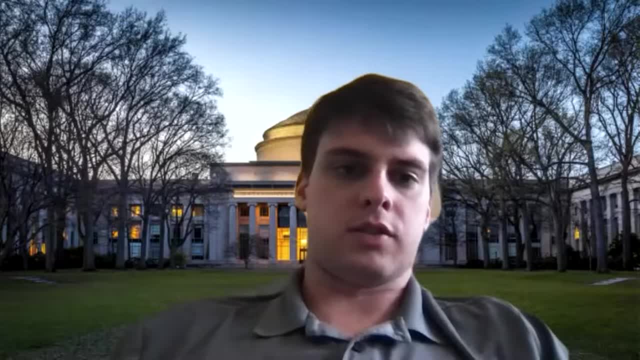 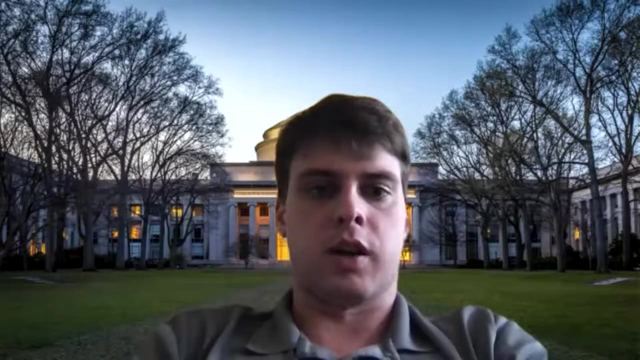 in dynamic obstacle navigation is planning in velocity space. yeah, yeah, something rather agents velocities, and then you figure out what velocity you can choose that you don't such that you don't collide with them. so there's all the velocity obstacle. reciprocal velocity obstacle: no, not those approaches from maybe 10 years ago, definitely yeah. 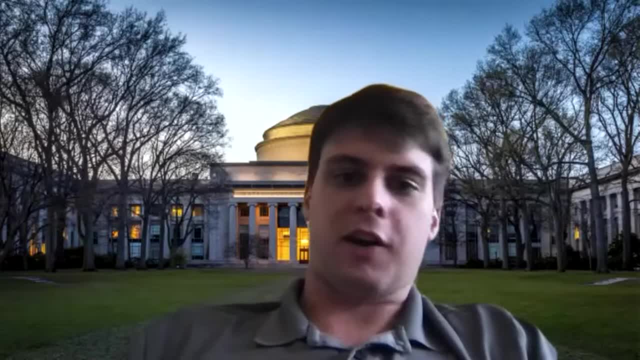 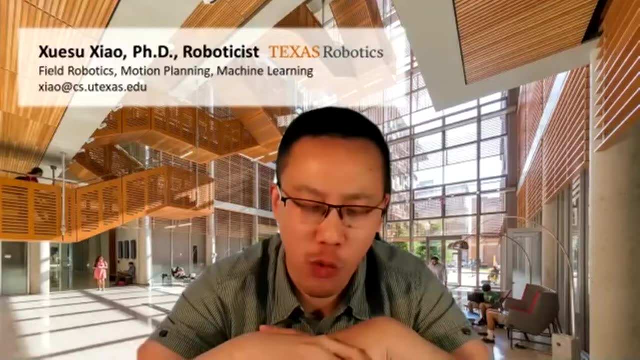 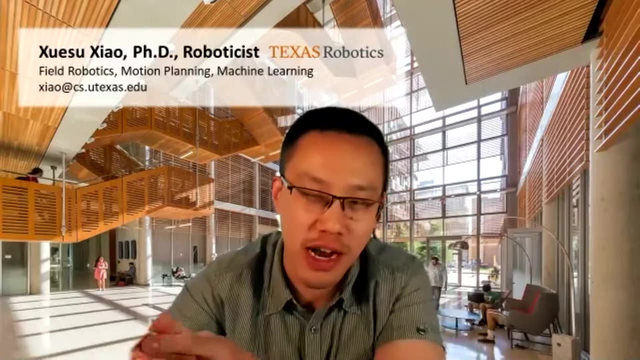 a small adjustment you could make. i don't know how small it is, but maybe like one, one way to attack that problem. yeah, the other thing is, again like i mentioned yesterday to chris, like what would be the best um cost function, like what do we really care? like, chris, is entropy and progress right and you are. 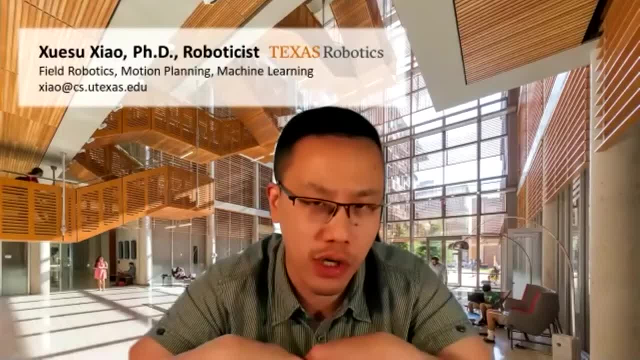 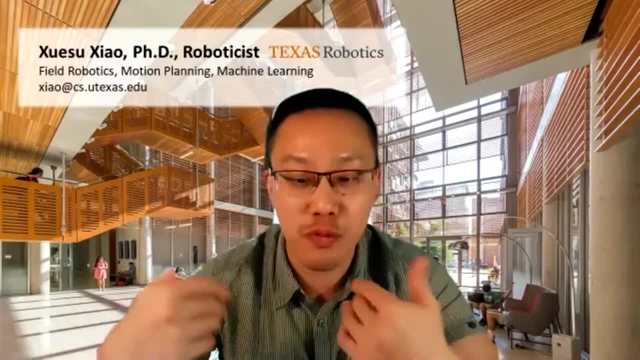 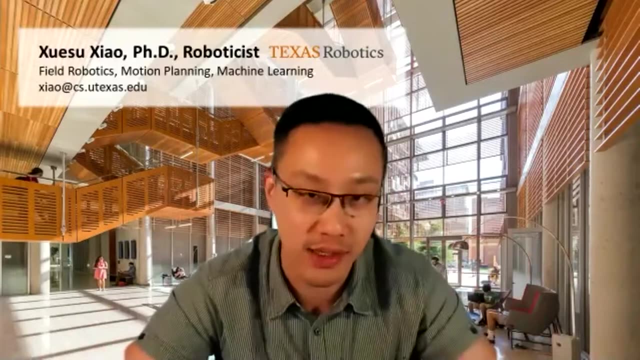 probably more about like social norm, how do we add those kind of information in there? that's also difficult, but for the hallucination is kind of difficult how the, the notion of optimality is much, much more different, because for us, for the, the hallucination work, we, the current work is mostly about shortage paths like shortest. 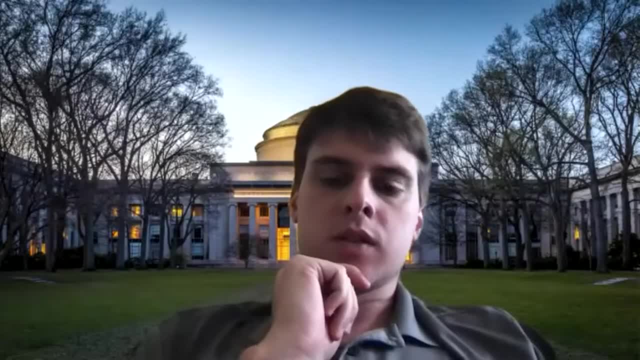 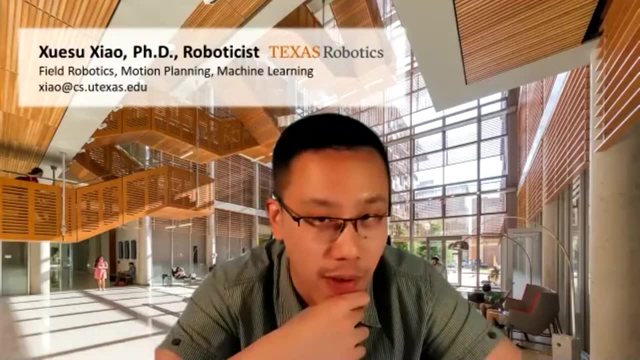 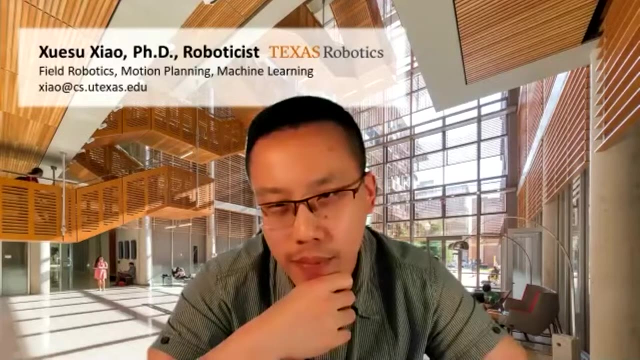 traversal time. that's it. but for for social navigation, that's different. well, i'm not sure. i think it may still be shortest path. okay, i think that's. it's just really hard to quantify what the shortest path in time in a dynamic world, because of the interaction between 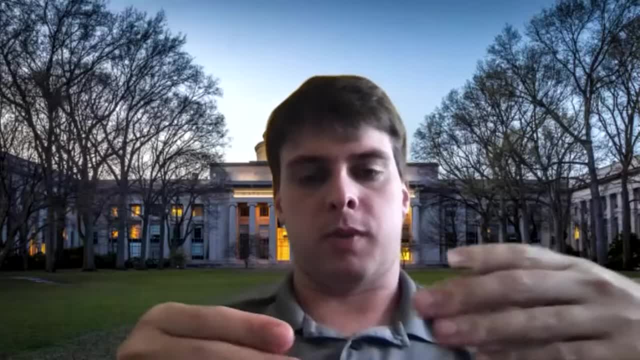 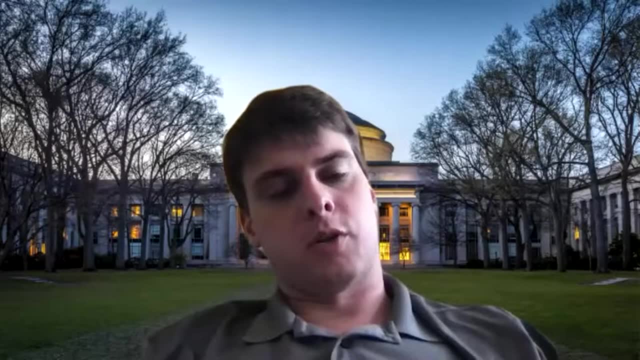 agents, like if you take a certain path and the other person responds in a certain way, that can influence the amount of time that path is going to take you quite a bit, yeah, yeah. so what you're saying is i'm hoping to talk with chris a little bit more about. i'm going to try and follow. 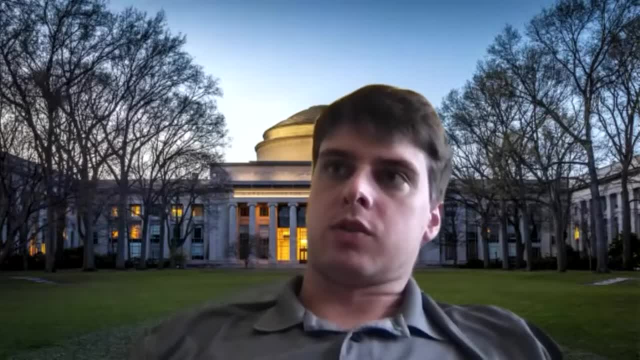 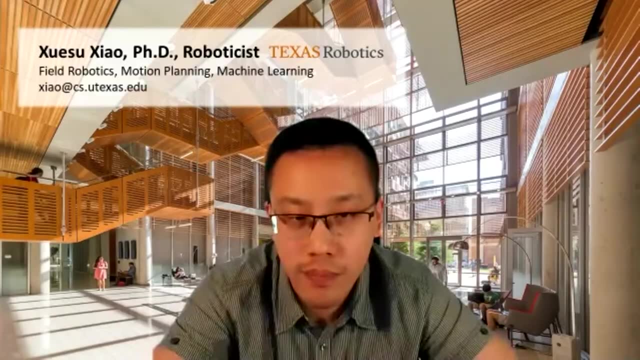 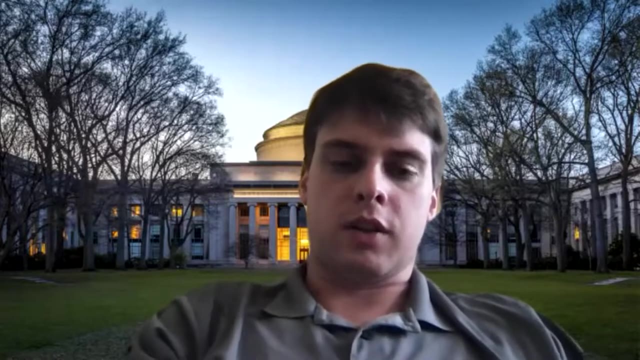 up with them. but yeah, like understanding, so sure there's that there's an entropy cost of you want to help, you want your robot to choose the actions that help people understand what the robot's going to do next, so that it like kind of implicitly communicates a topology that you want to pass. 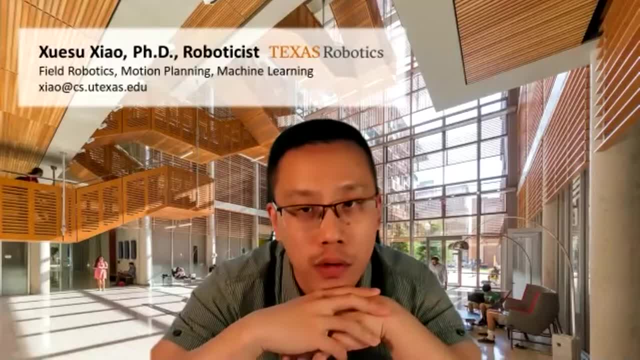 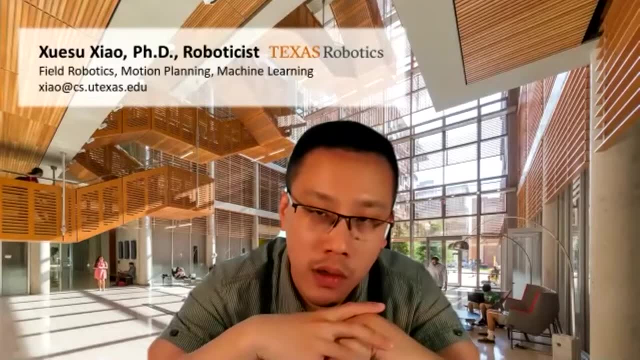 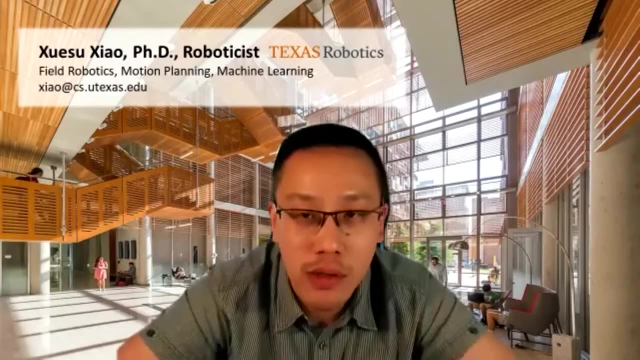 somebody with somehow. i think there's probably a link between that idea of the topological representation and the amount of time that it's going to take to execute that topology. uh, that would be interesting to explore. yeah, yeah, that should be interesting. yeah, okay, yeah, i do think, like most, you know most motion. 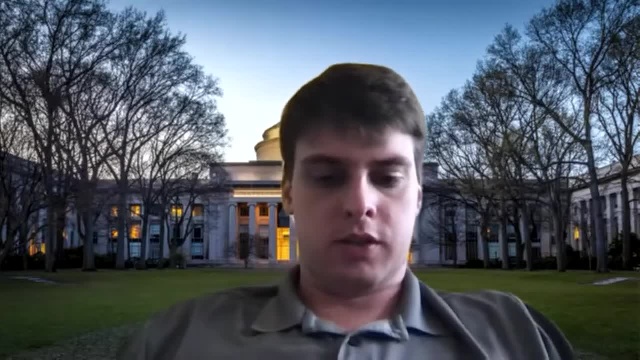 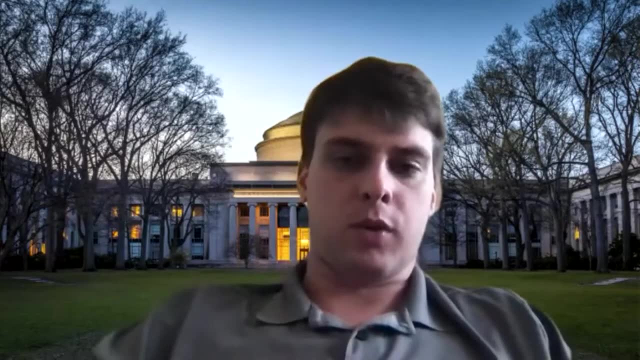 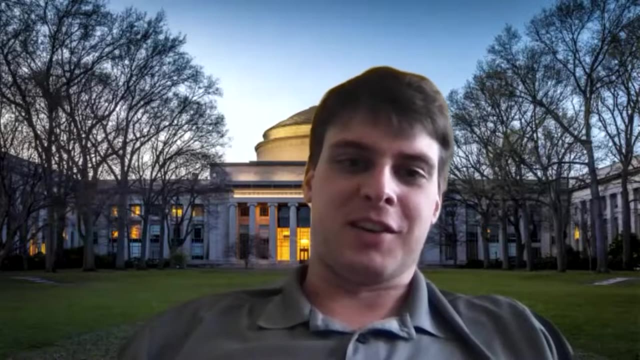 planning problems historically is there's some cost function like some minimum time, there's something in your eyes and there's something you have to estimate about what you can't predict, and having all of those terms have the same units- if it's all on time, uh, makes life way easier. it's really hard to get different objectives. 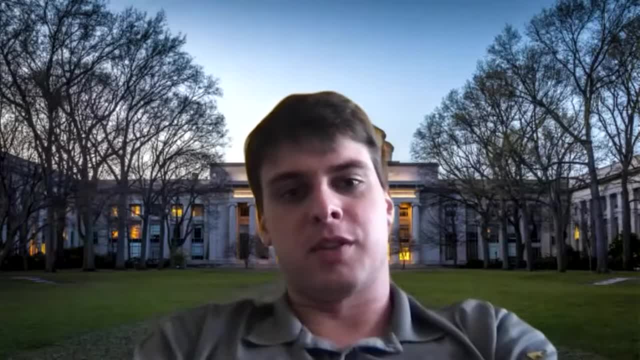 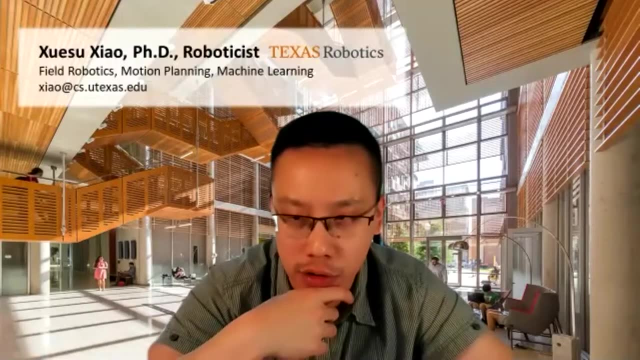 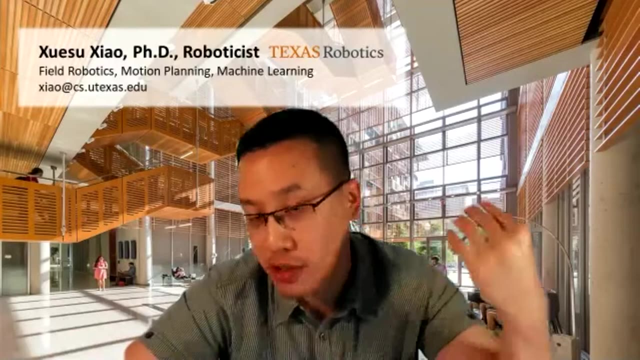 that are that come from totally different units and dimensions? definitely, definitely, yeah. so, in parallel to this idea, the other thing heri and i trying to pursue here is: can we come up with a runtime hallucination policy that try to mess around with the perception, so that we can still? use a classical motion planner through a enough et cetera approach and actually fix andsnaze a classical motion planner toма a startup for squatwork or somewhat abstraction, so that we can still use a classical motion planner to do that in the other way è. 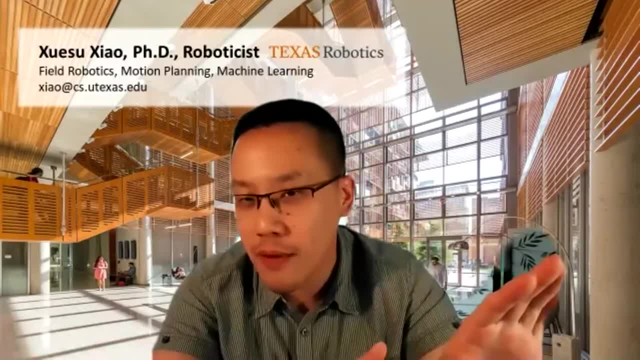 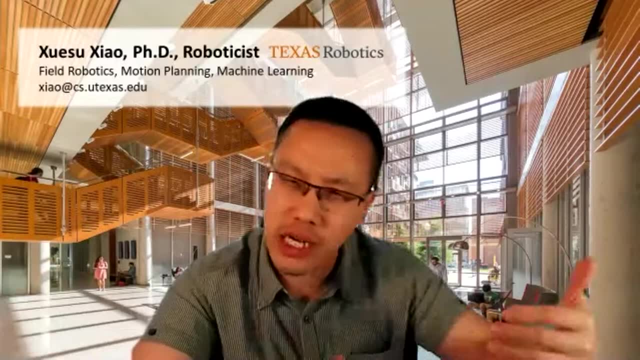 social navigation. so example could be: if you see a person there, somehow you can hallucinate like maybe a bigger region of the person. it's kind of like trying to predict their future trajectory, kind of deal. but you are trying to have this rl agent to come up with it, like we also call. 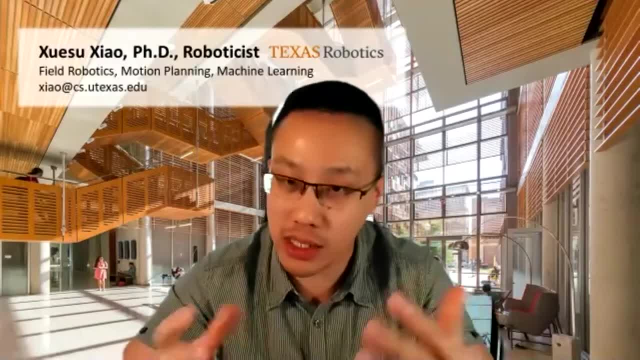 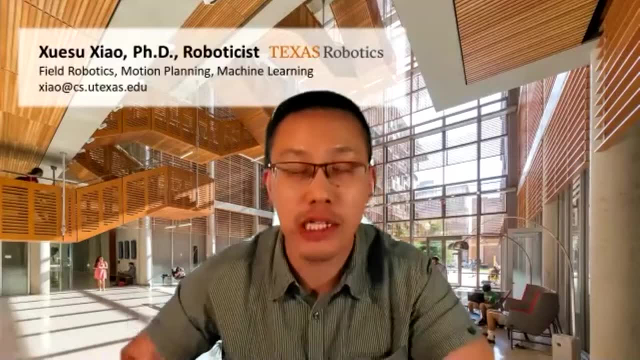 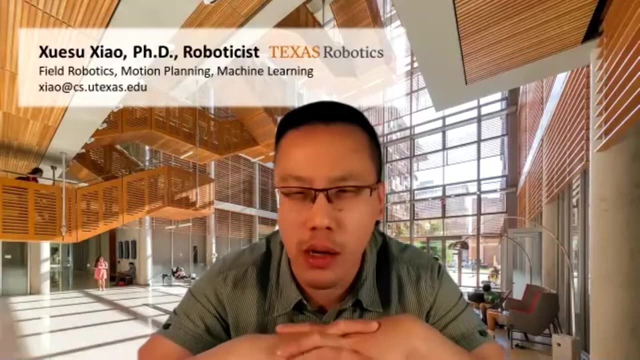 deception right to deceive the lidar input so that the end end result of this deception- the deceived lidar can- can cause a cost map which is utilized by a classical motion planner to enable various smooth transition between different agents. that's one thing we are kind of like currently exploring. 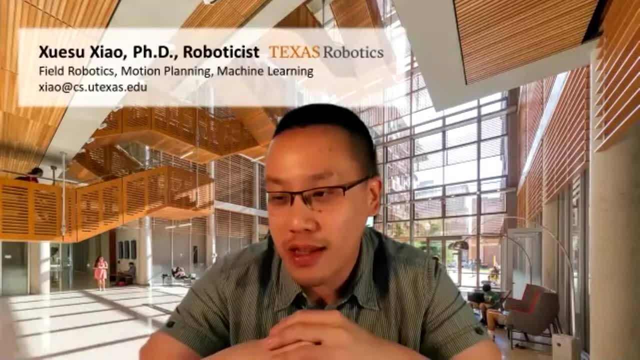 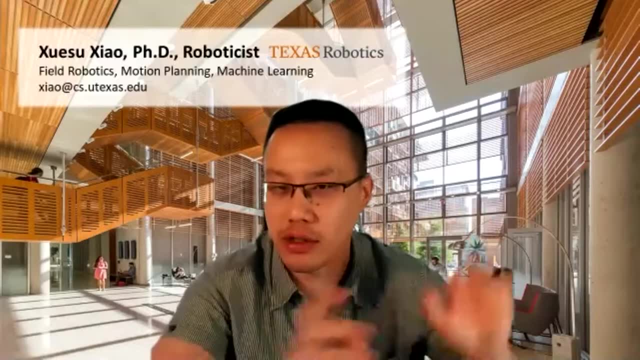 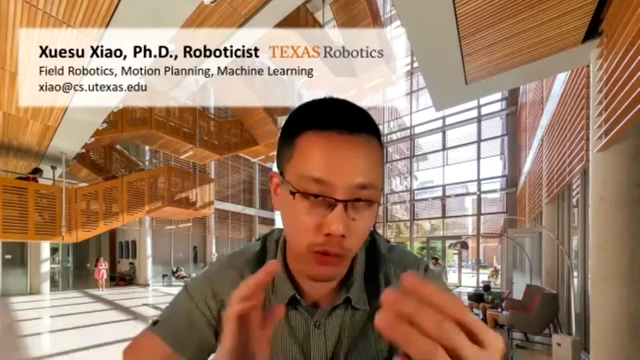 maybe it will work, maybe not, yeah, but i guess the, the action space of the, our agent, will be simply like where to add some some- i don't know- blockage of the, the moving agent. on the other side, and we are particularly interested in in the narrow hallways, a person passing each other in a narrow 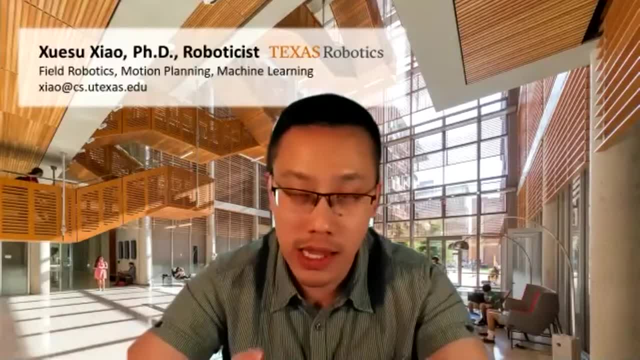 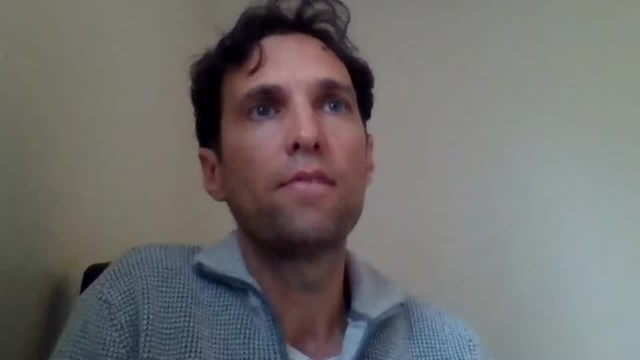 hallway one, maybe two robots, maybe one person, one robot. and then how can you? we have this bw robot in our lab which, uh, navigate around this hallway like holding extended amount of time, from 9 am to 5 pm every day. the thing is, if it sees another robot. 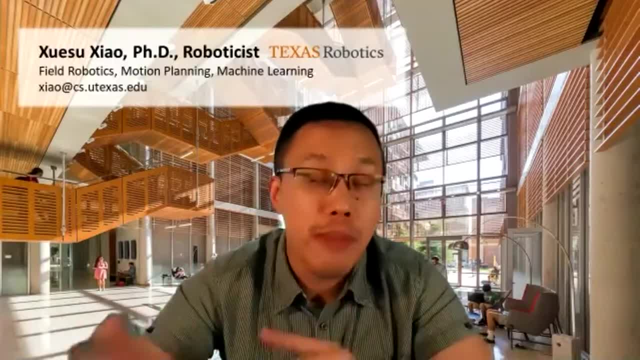 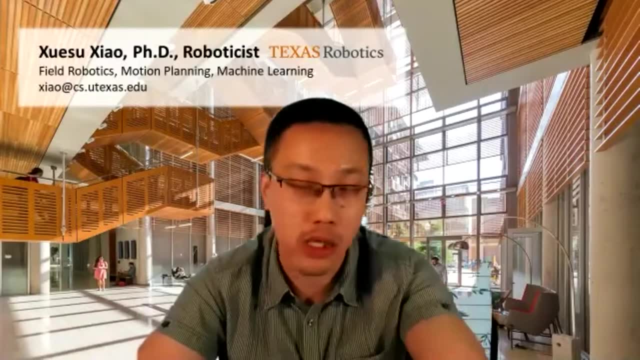 or it sees another human using the- i think we are using ebay planner. using ebay planner, it is very, very likely that the robot will turn around because it thinks, okay, there's an obstacle there, i'm not gonna go this way. it just turns around. so we are trying to come up with the methods that. 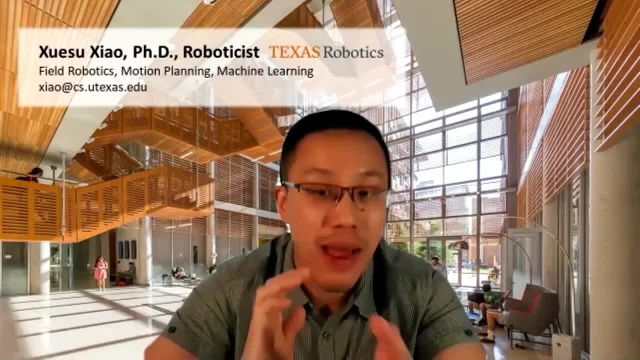 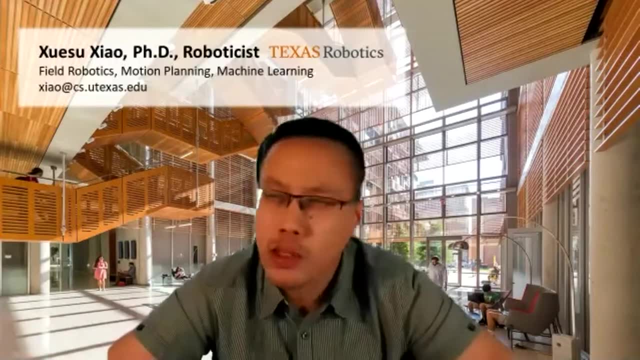 we're going to use to make sure that we're not going to lose navigation efficiency. so most of the time it will smoothly pass each other if it's possible, but try not to turn around or get stuck somewhere. that's one thing we are trying to explore right now. yeah, yeah, yeah, you have anything? 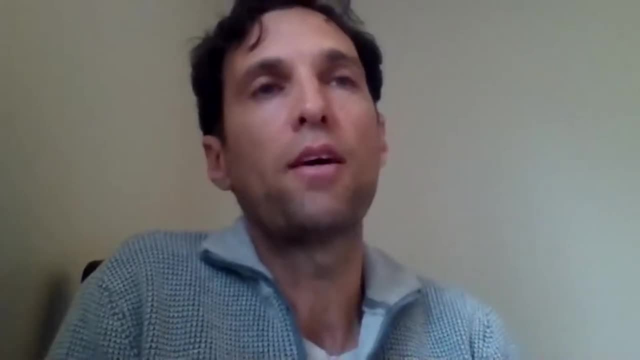 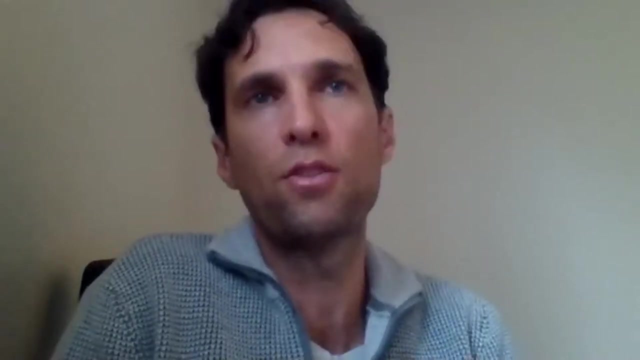 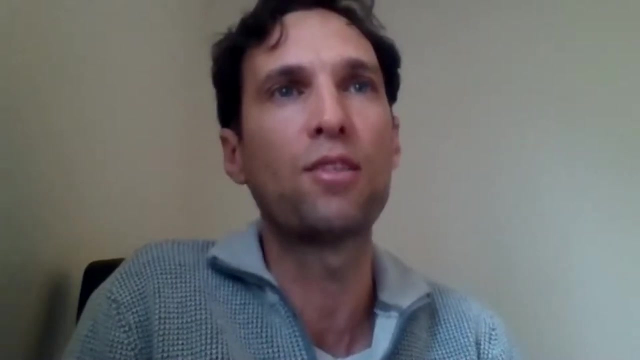 to add. it's both about hallucinating the location of the object and also the shape of the object. so there's two like these parameters need to be learned. i mean we can hand code something, but it's we might find some function. that's general enough, but we're trying to do this by learning um. 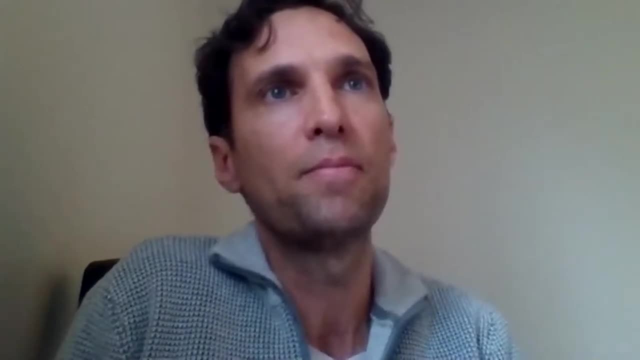 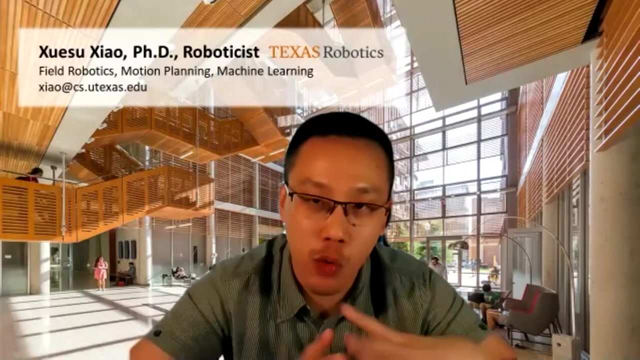 the hallucination aspect. yeah, yeah, so harrell had some previous work on like come up with a strategy like a, like a polite strategy: one robot go to some place and park and the other just goes through. so it's very efficient for the other one, but the the first. 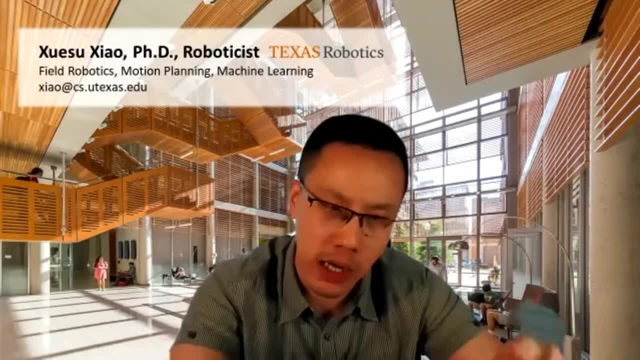 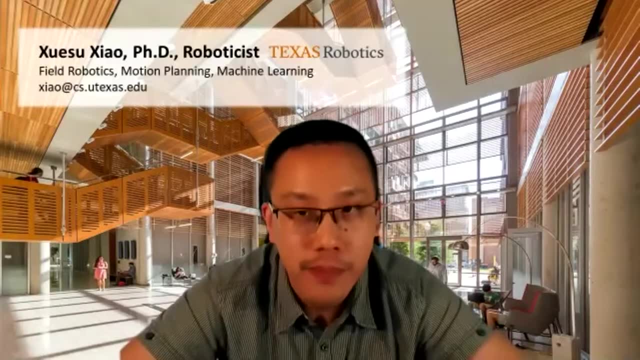 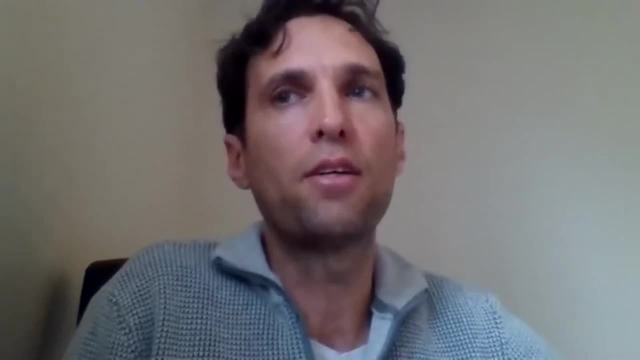 one, the polite robot, need to stay somewhere and we try to. i think harrell's previous work is trying to learn where to park so that the transition would be very smooth. yeah, and i'll just say about the hallucination that it's not a standalone policy, because in some cases- so sometimes- the 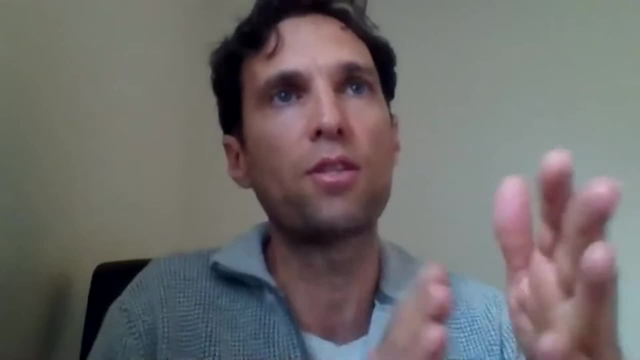 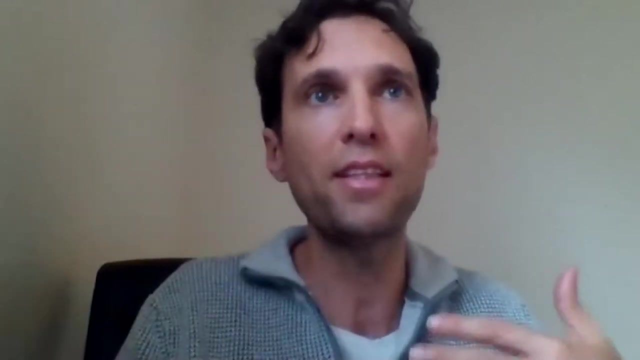 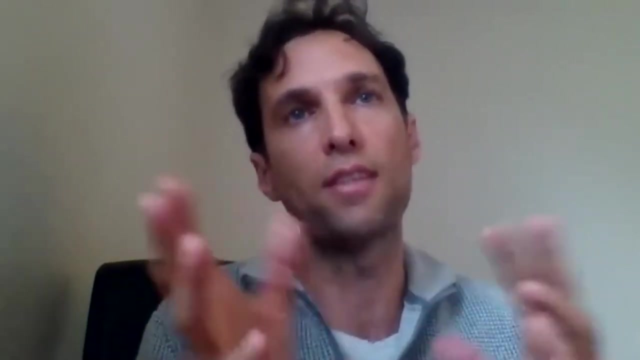 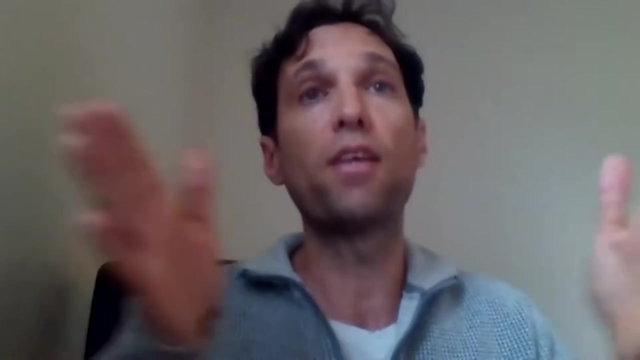 hallway is wide enough to enable two robots to pass, and it's just. they occupy the center of the hallway. so if they- they see each other and one in front of the other- they just see an obstacle and turn around. so if they hallucinate, um, uh, some trajectory of the other robot, they might go through. um, but the thing is, if the 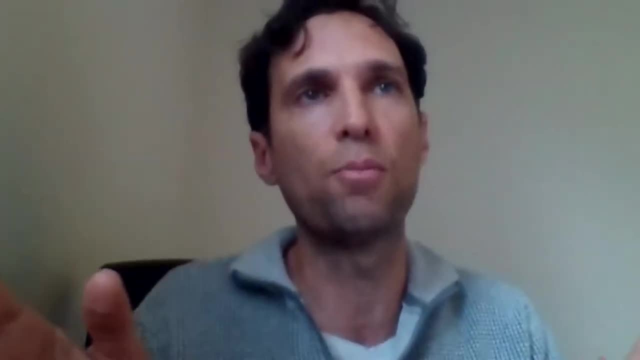 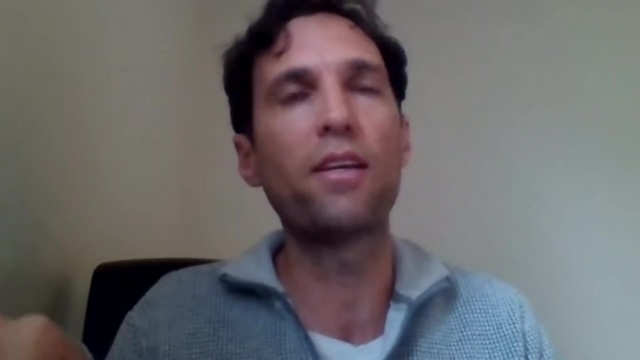 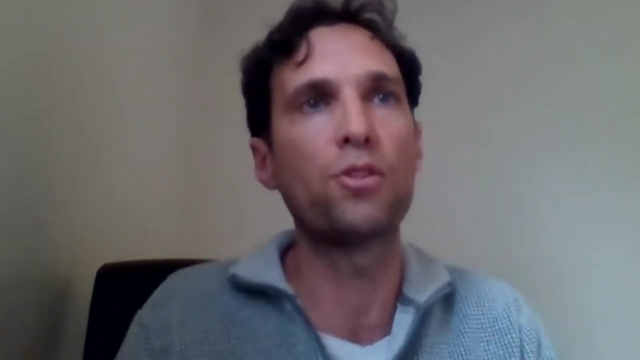 hallway is too narrow, with which doesn't allow two robots to pass, then one of them will have to stop somewhere and wait. and that we cannot achieve through hallucination, because if we hallucinate a blockage on the whole entire hallway, the robot would simply turn around. 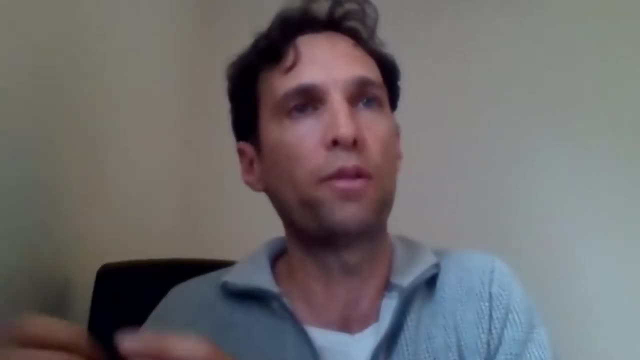 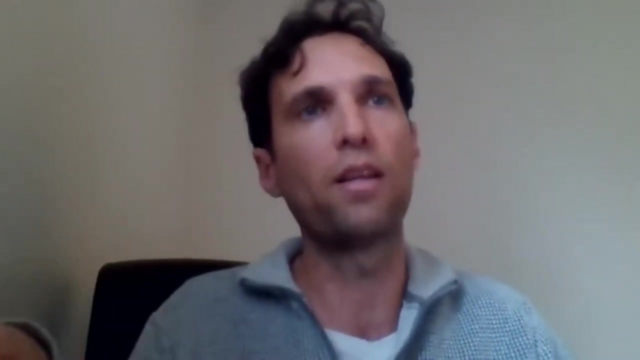 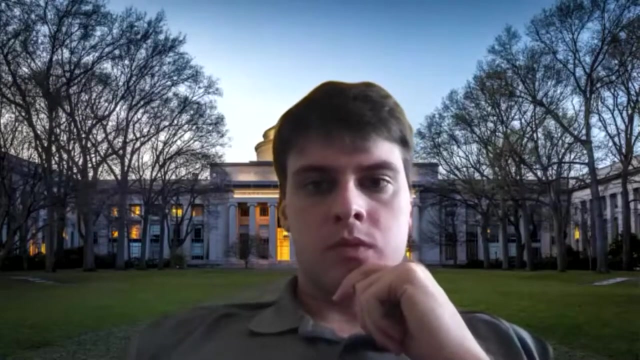 so we still need to use that, the waypoint method. so if the hallway is wide enough, we'll hallucinate. if it's not wide enough, um, we'll have to use to to learn where to park in order to let the other robot pass. yeah, because it's physically infeasible to for them to pass in a narrow hallway, right, yeah? 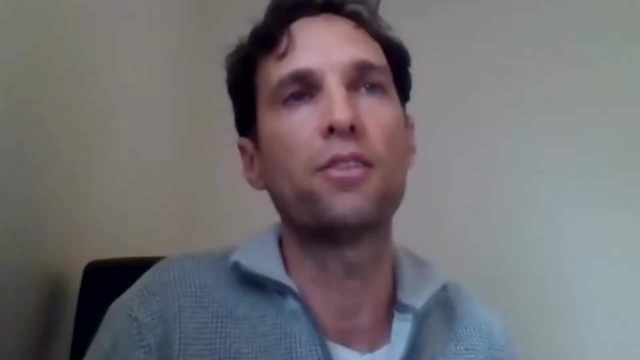 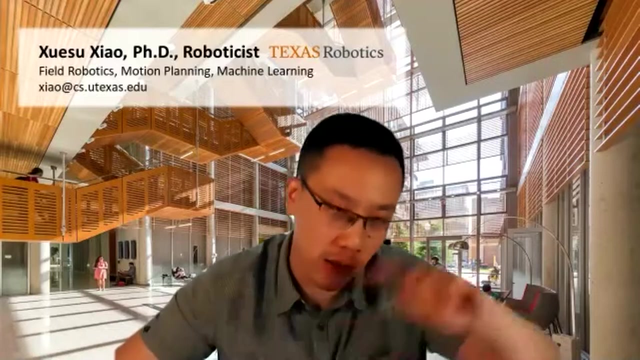 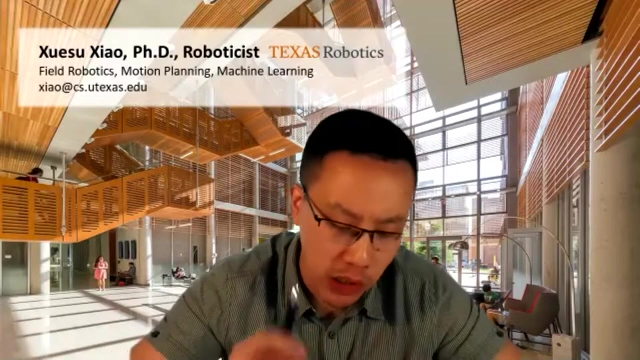 right, yeah, we can't achieve the weight action through hallucination, that's. that's kind of- uh, some limitation of it probably could be a state machine, right, whenever it's not possible to pass, go to the waypoint assignment module. so you, you park somewhere to let the other one go. yeah, i also want to point out that maybe the social norm 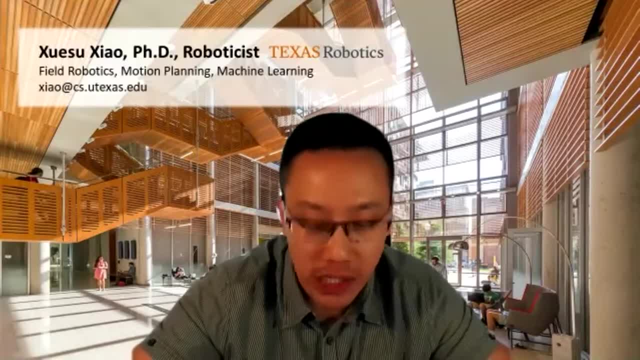 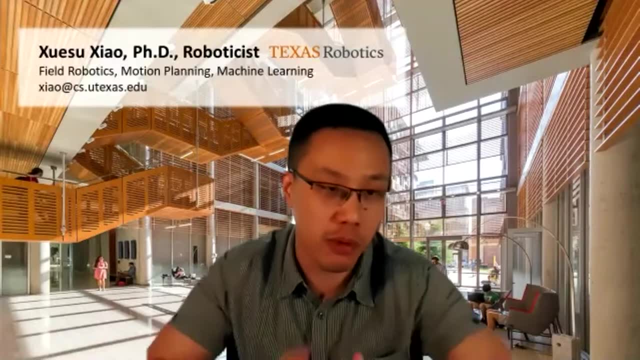 aspect can be encoded in this hallucination because, for example, in a wide hallway, two robots are trying to pass, but if in the middle there's no, no, not sufficient clearance for them to pass, and then the hallucination could be always hallucinating on the left, because that's what the 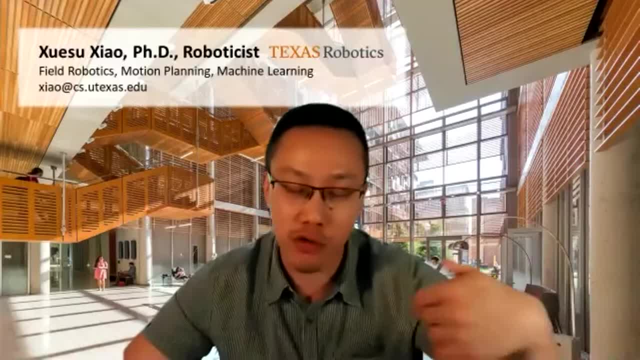 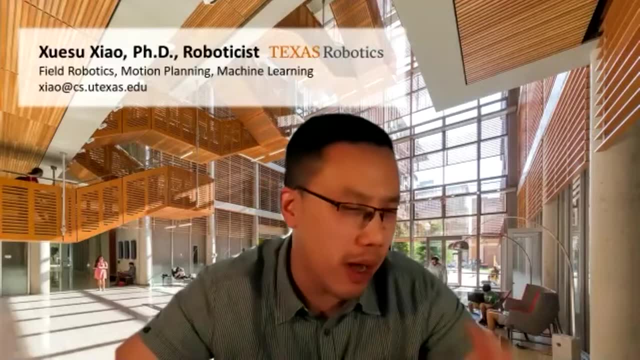 social norm indicates right. so that's what the social norm indicates right. that's the waypoint people usually go, like for the other direction, like we always move on the right so we hallucinate the other, the opposing robots on the left that could be somehow encode social norm in this. 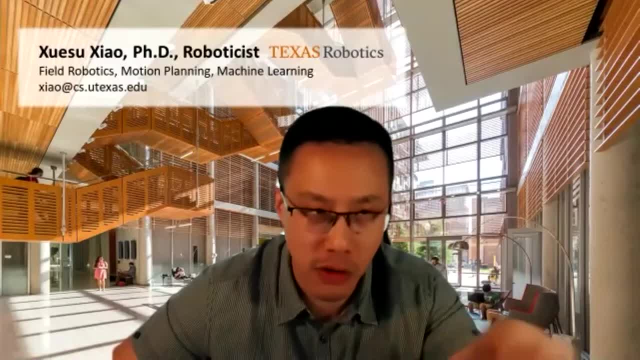 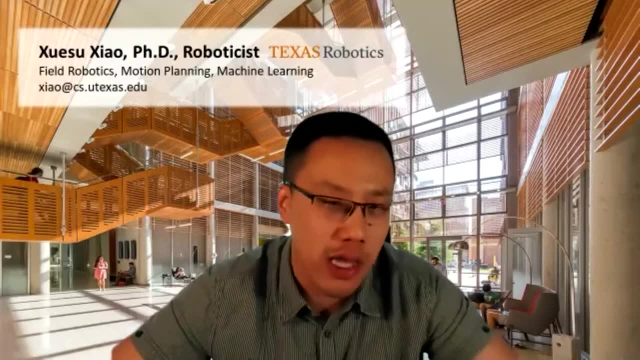 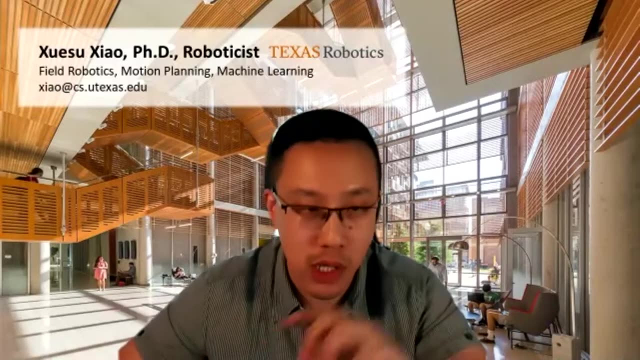 through, for example, like michael's work on on on the kato line, we can say, okay, if the passing is the other way around, that's, that's a penalty, that's not good. and then we can probably try to encourage uh, behaviors that is like in correspondence to social norms, using this. 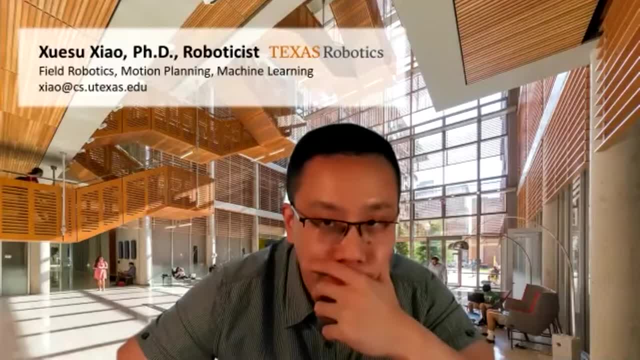 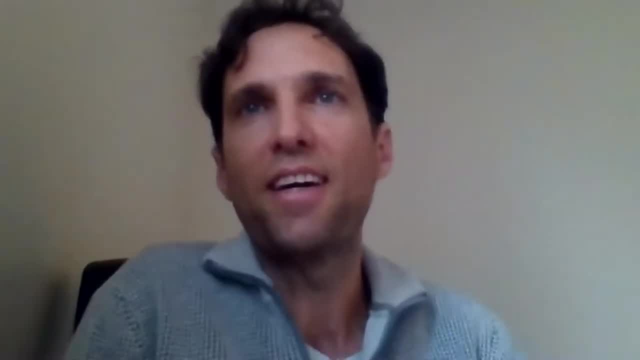 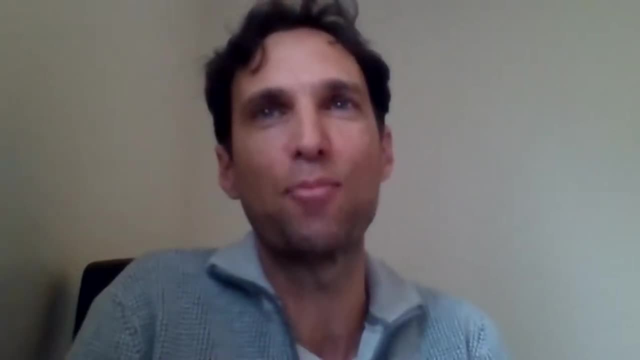 hallucination agent. you know, i find it interesting that the i robot in the presentation she said that they don't use use any machine learning at this point, like on their deployed products. yeah, yeah, i guess that that's amazing about it, but everything is classical planning right now. 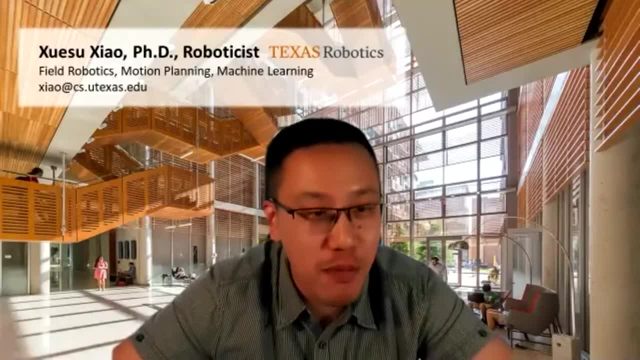 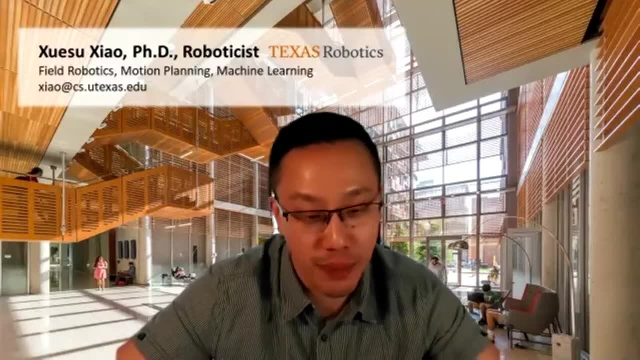 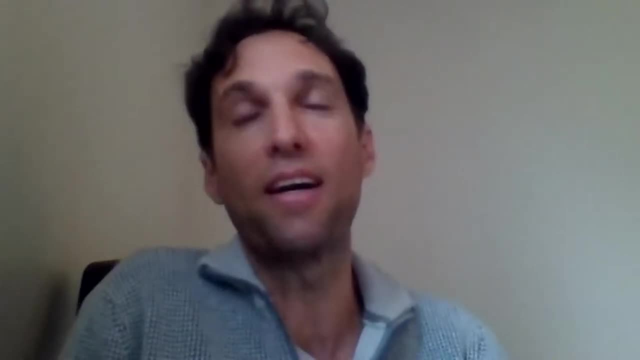 yeah, yeah, that's the thing. so, yeah, there's lots of papers on machine learning for more, like for for navigation, but there's not many products actually being deployed using those learning methods, right? so so what does it mean that that you know either that classical methods work good enough? 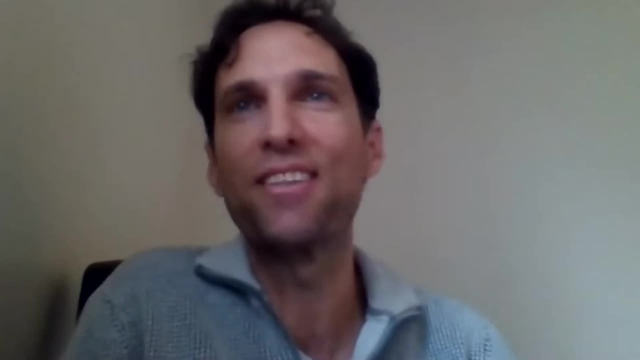 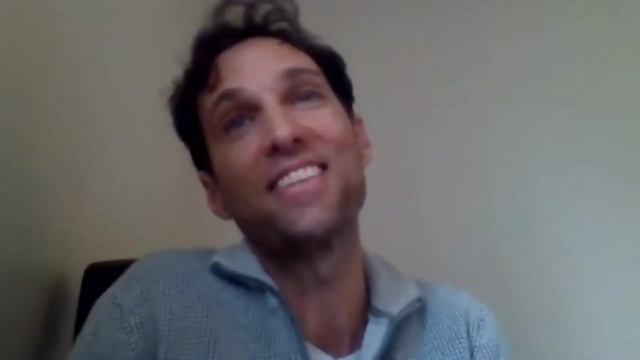 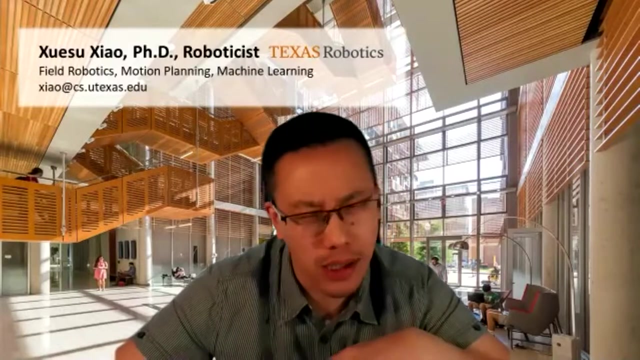 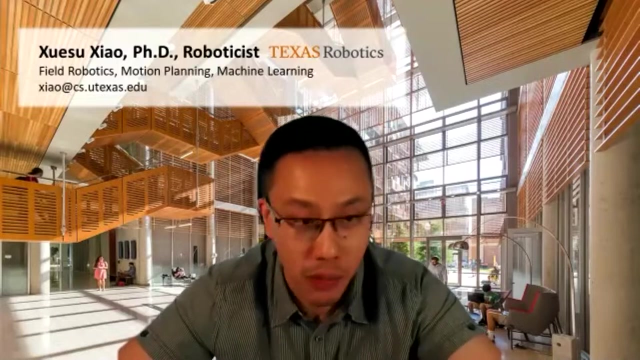 yeah, or that the machine learning approaches are not reliable, or many resources for their computer, i guess. i guess that's the main thing, right. so so people don't trust machine learning to be deployed in the wild. that's the main thing, right. they trust classical methods. they are verifiable, they have safety guaranteeing. they also explain, explainable. 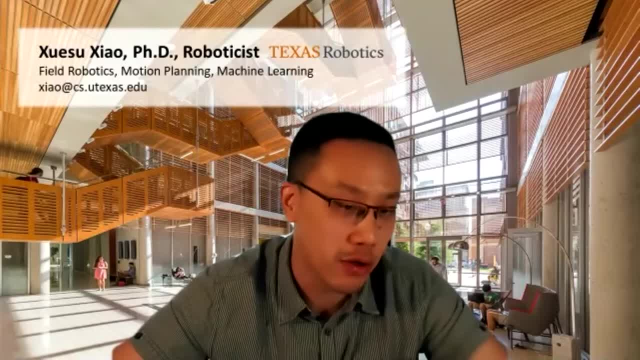 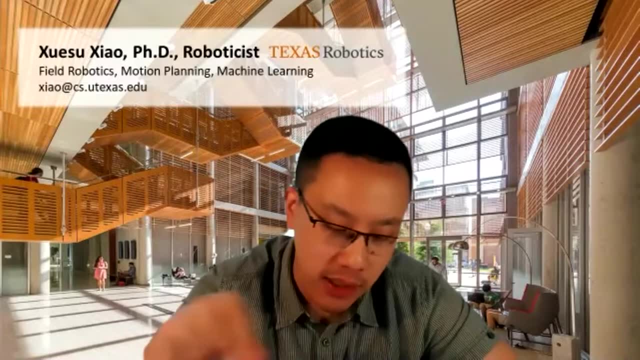 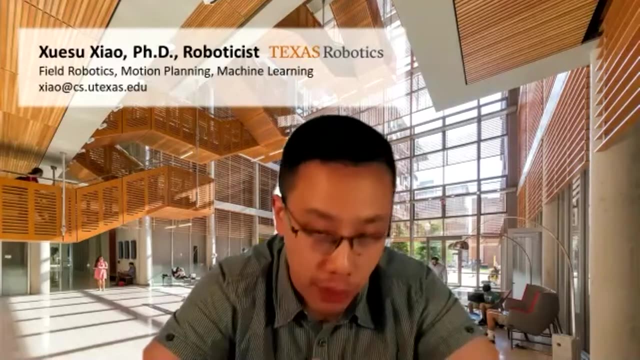 they can debug everything bad happens, they go in there and fix that issue. but for learning- and that's usually not the case- yeah, one one thing we, like bo and i, are trying to look at this lifelong navigation is just to trying to identify the weak spot of classical approaches, for example, i robot. 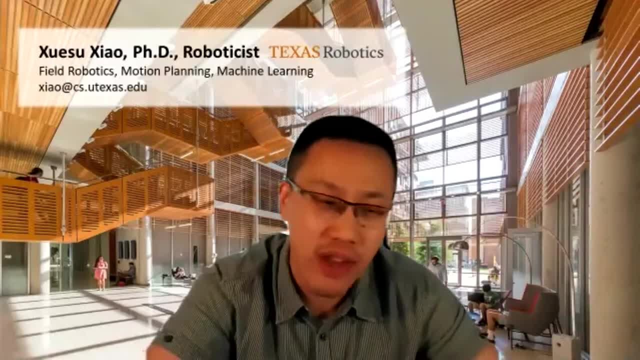 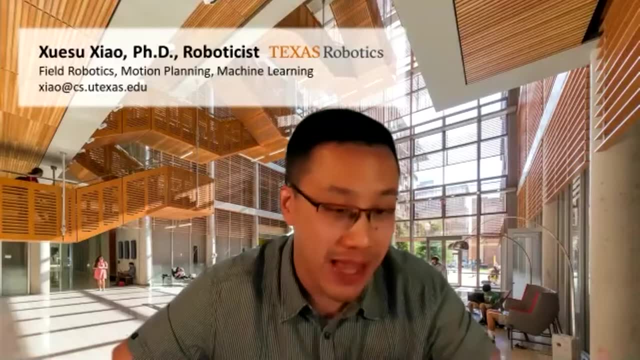 like get stuck in lots of places in your homes all the time, right? even if it's the same floor plan. it gets stopped the first time, the next, the next time it's come back to this place, it may get stuck again. but this shouldn't be happening, because this mistake can be learned, so we can. 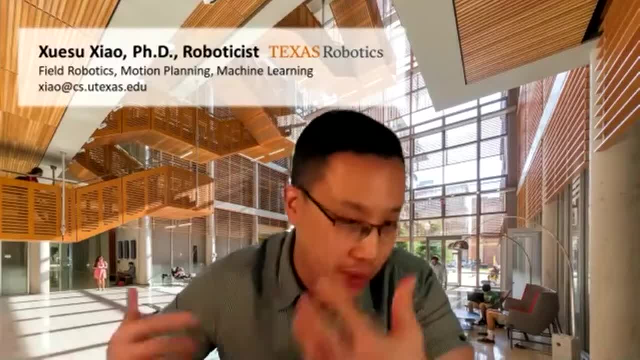 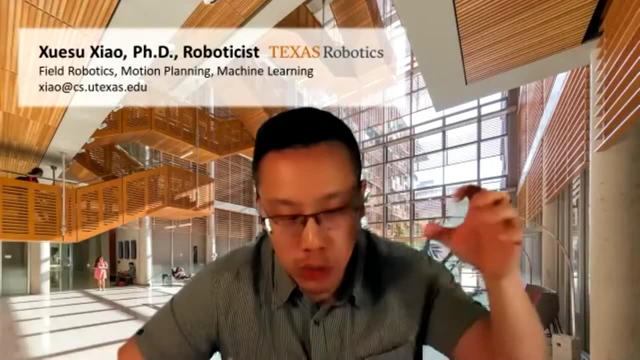 learn from those mistakes and then in the future we shouldn't repeat this mistake. i think that's a place where machine learning can really help, and so the boss approach is what we try: to identify those places. we try to learn an end-to-end local planner to address those. 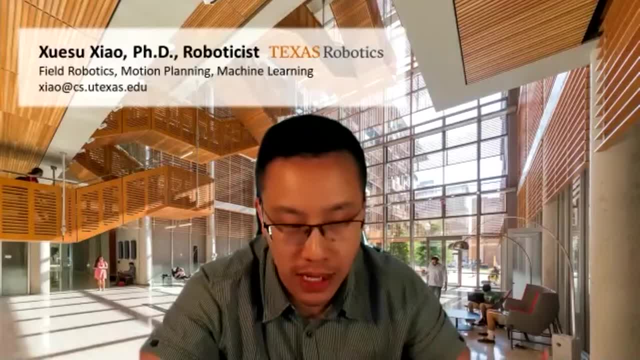 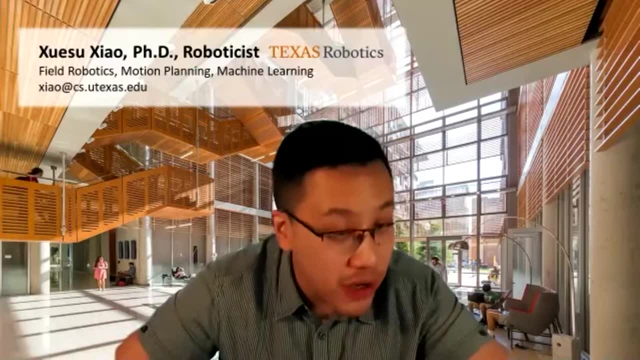 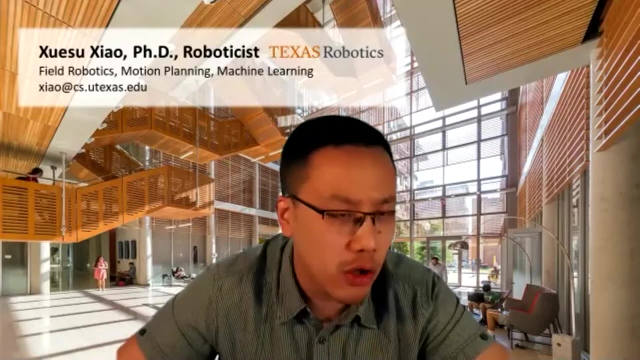 so the next time a similar situation happens, when the classical motion planner gets stuck again, now we switch to the learned local planner. so the benefits of this is is super efficient because we- i think we only use i don't know how many like like maybe a few thousand data point to learn this. 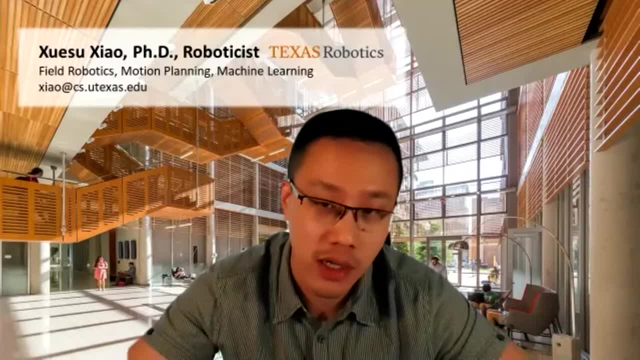 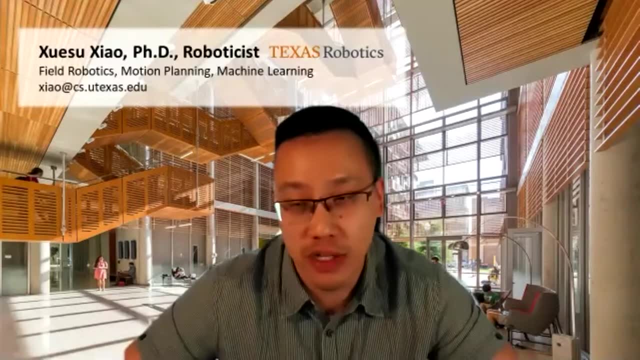 complementary right, so i don't remember his name, but it's super fast, a super small amount of data and also very, very fast to learn. everything is on board. we don't even need a gpu for this. you know everything could be on cpu. it's a very small neural net like three uh 32 neural, 32 neural two. 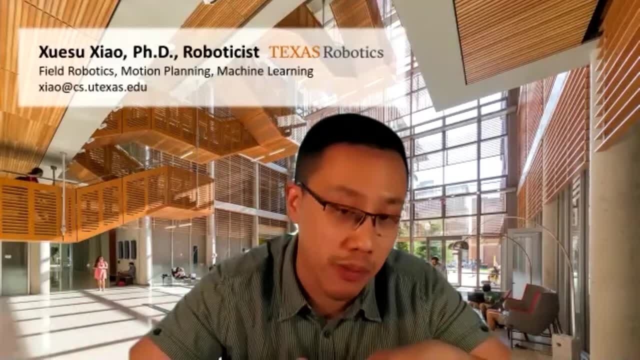 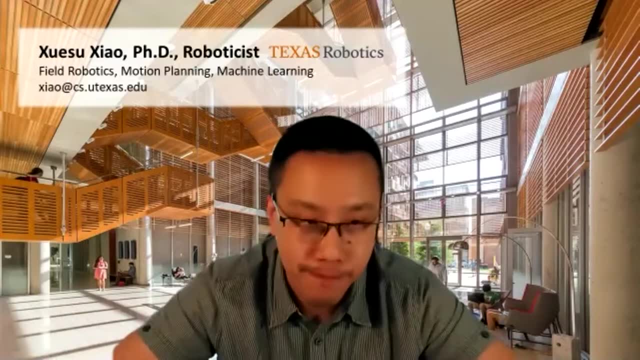 or three layers, that's it. you know, even use a gradient, uh, episodic memory, like it's kind of increased computation time, but everything is learnable online on border robot. yeah, that's something like we are really thinking. so machine learning- end-to-end learning- is probably not. 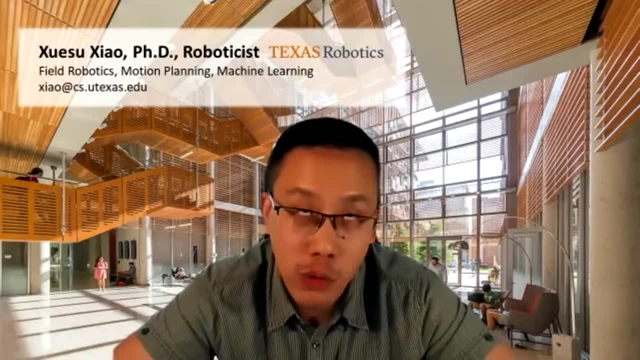 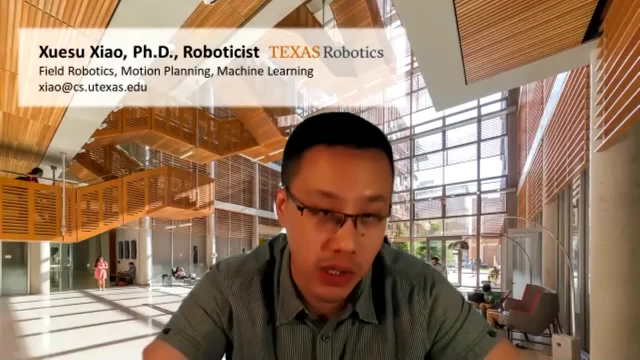 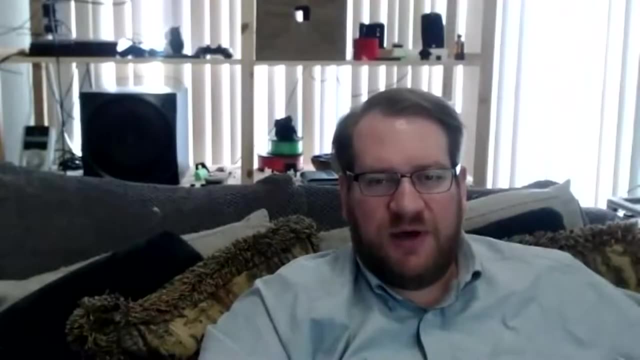 like people don't trust it to be deployed in the wild. but really what we can do is find the piece classical navigation to improve with respect to different experiences, because that's classical methods usually do not do that right. i think that, uh, in the wild, at least for consumer applications. 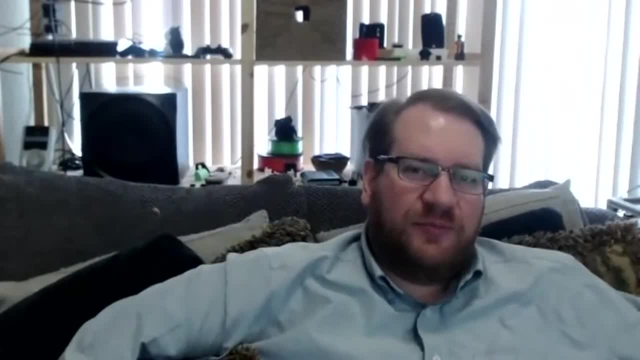 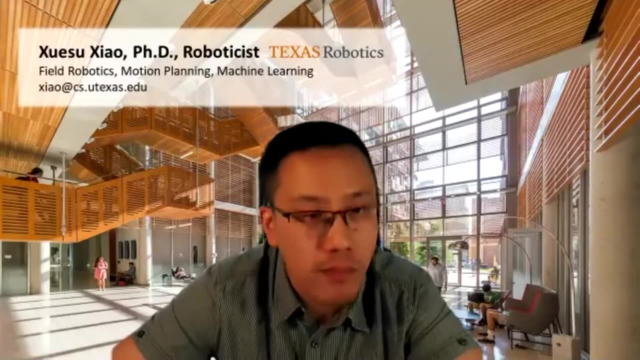 you're also, even though you're not, you know, putting this on some big gpu. i think you're still a little bit cost constrained. you're still a little bit instrumentation constrained, like um they're. they're, like you know, especially from the perspective of a company like irobot. 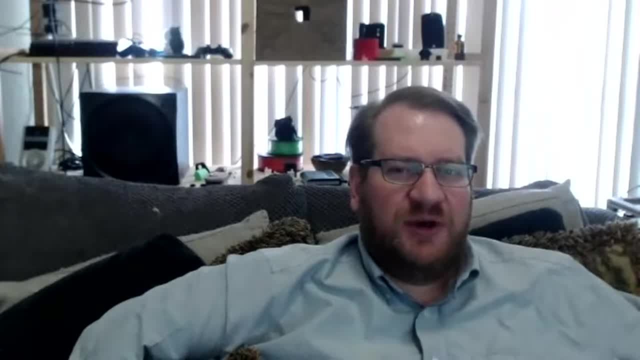 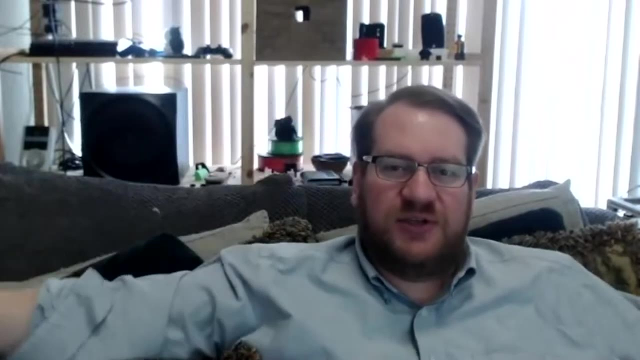 you're looking at the total fabrication cost of a consumer product. if i understand the guideline, it's about a third of the msrp right. and then you have a company like irobot that has a bunch of research scientists working there and people with phds and and that only drives your personnel cost. 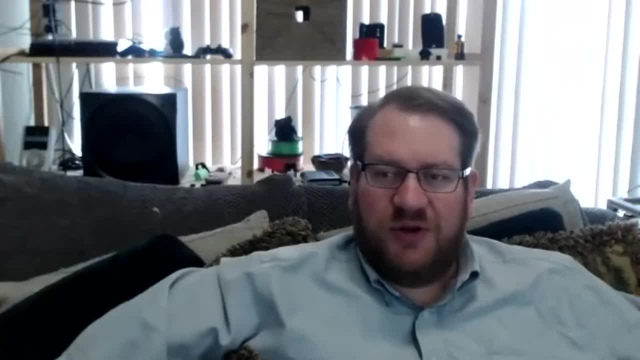 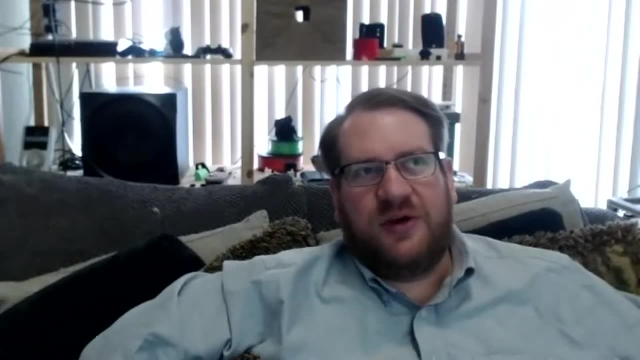 up, you know. so the margin per unit needs to be pretty high, right? which means that, um, which means that you know. you know, if you think of a roomba going for like maybe 300 bucks and there's like a hundred dollars worth of hardware on there, you know you're now talking about a route- i don't know what type of- 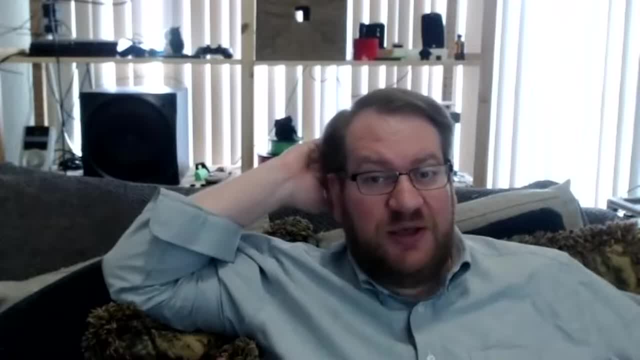 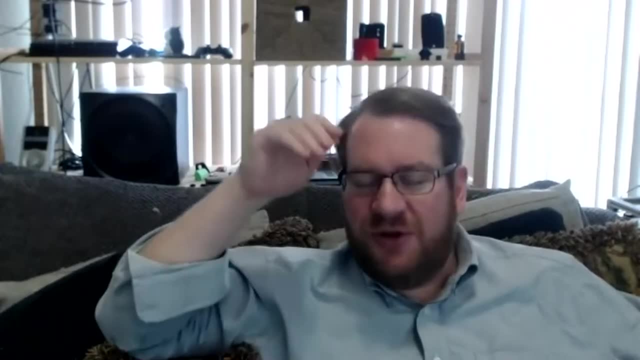 microcontroller is in there, but it's, it's going to be a teeny tiny thing, you know. and and then you know, i guess the current versions have a camera of some sort on them. um, so you know, like, like, i think that i can kind of sympathize with under that regime it's pretty difficult to. 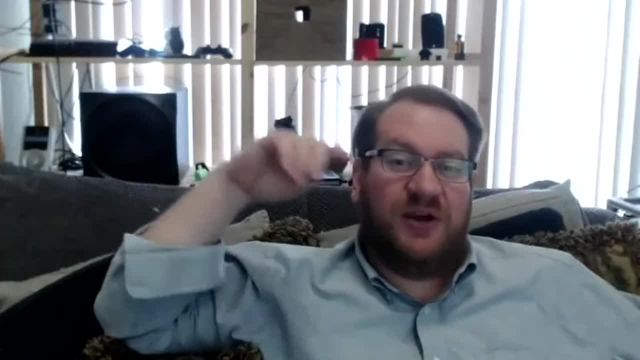 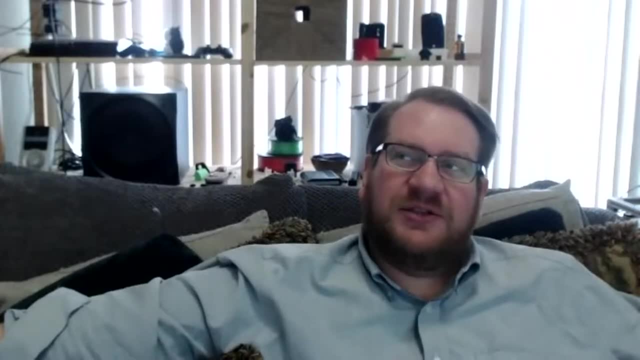 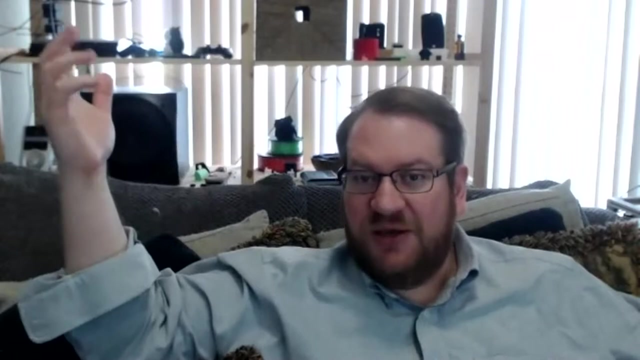 to put in. you know meaningful machine learning algorithm. plus, they're also usually fielding. you know when you're feeling a consumer product. you're probably general. you know like not to, not to say that they don't innovate, but they're probably fielding the. you know best known best practices right and applying machine learning to this domain. you. 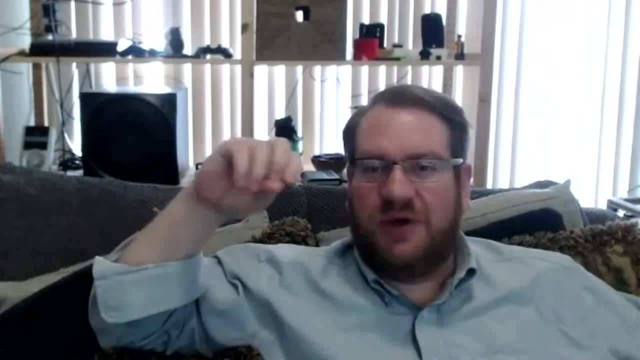 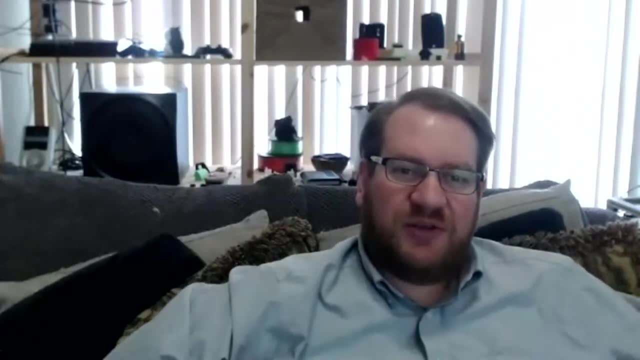 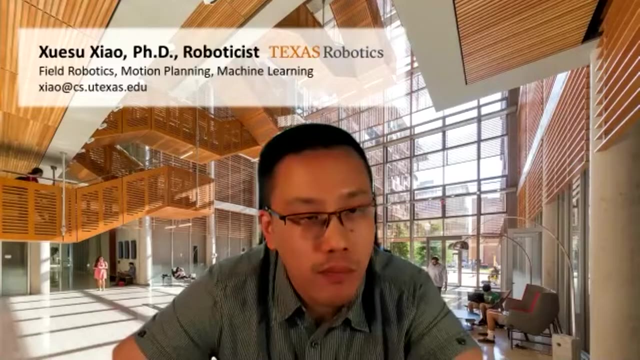 know is something that has been done for a long time, but, like the more recent stuff, you're never going to see uh, or rarely we'll see uh put directly to consumer products, right, unless, unless they feel really like this is the proven thing. this is going to last. yeah, i guess this. 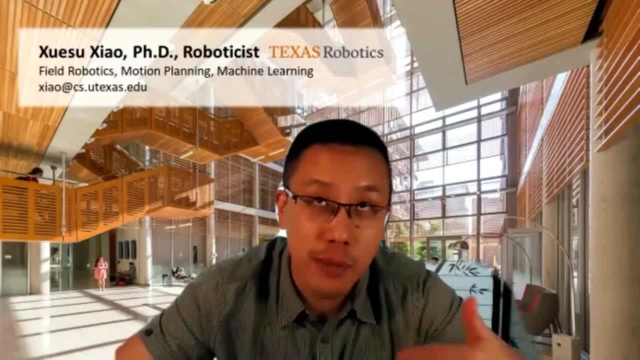 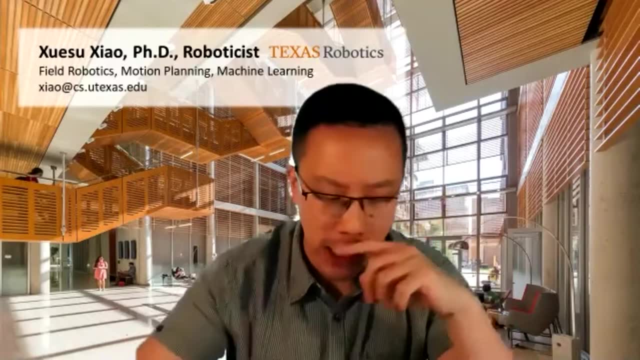 dude didn't like it's not. still, the benefits brought in by machine learning cannot justify the extra cost. obviously, yeah, but there's also the other thing i i want to point out. is this kind of like cloud computing, edge computing, right? so the rhombus in the field at everybody's homes. 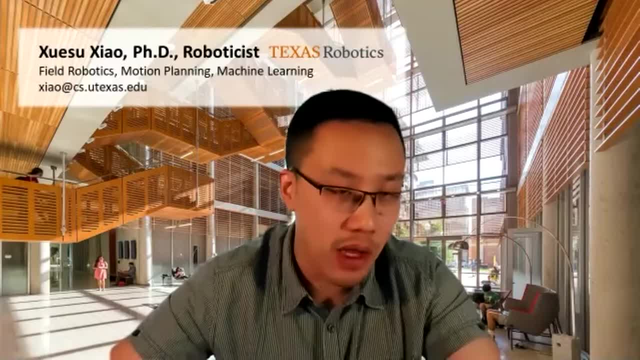 does not need to have all these resources for the training. if they're collecting data and they are connected to wi-fi, they can probably just dream and go. you know, get theThank you for that. yeah, that's really my thank you for that, Eli. it's been a pleasure to be here. Have a great day. 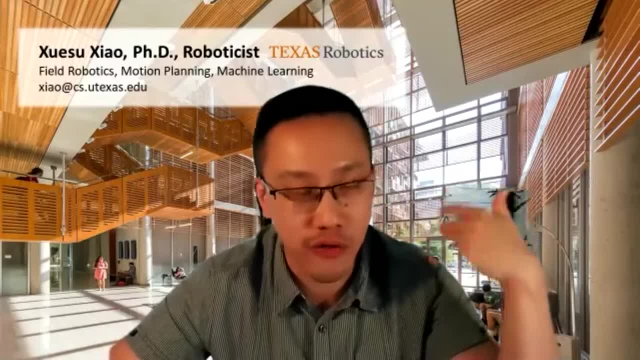 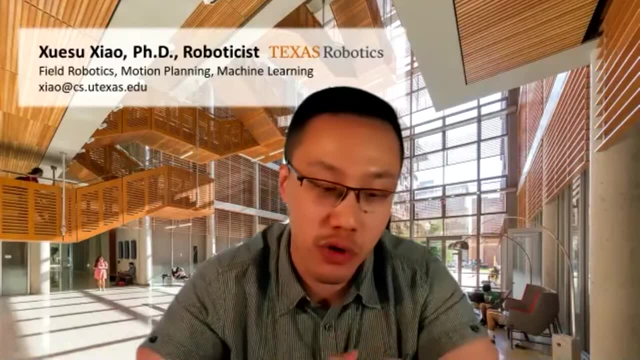 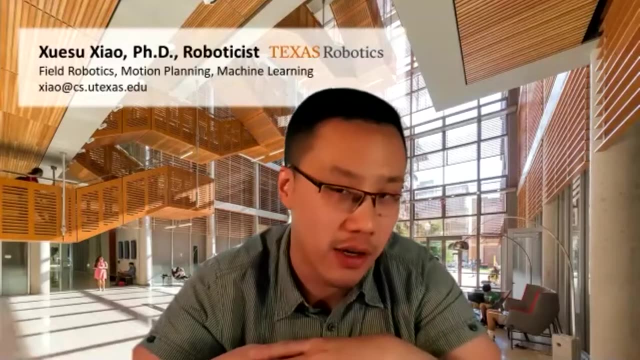 the data online and then they can do this in their server and then just downlink all these new learned policies, very small neural networks- to the, the robot at our home, and then they can just deploy them without many overhead. i think that's what. so i think i asked laura that question. 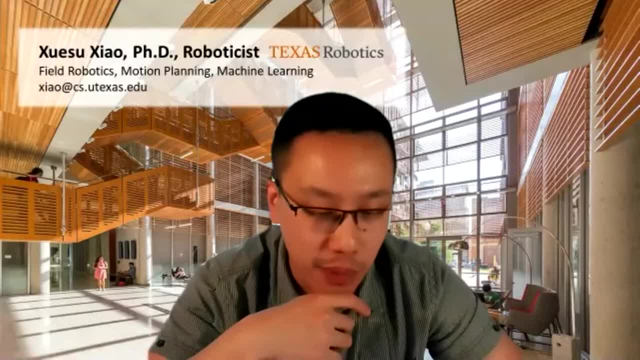 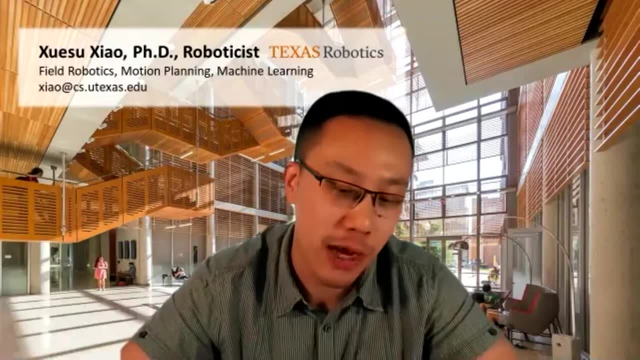 uh, yesterday. so she was saying, yeah, they are collecting data, but they are currently not doing that, if i i understand her correctly. but lots of things are not public, it's confidential. i understand that, but i would say is learning can definitely be be done only on in the cloud. you 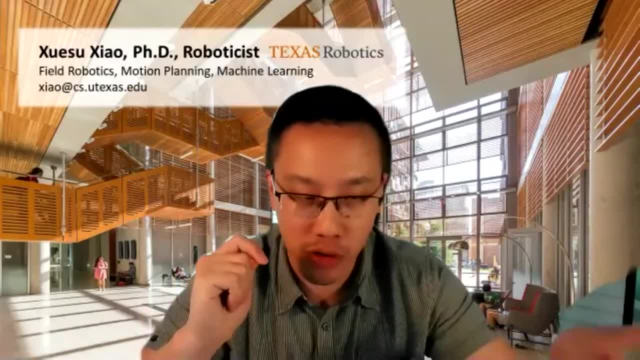 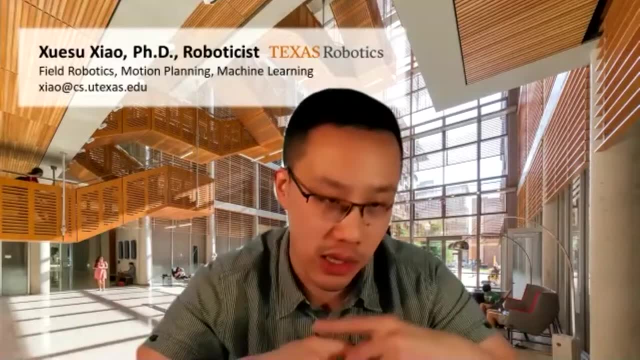 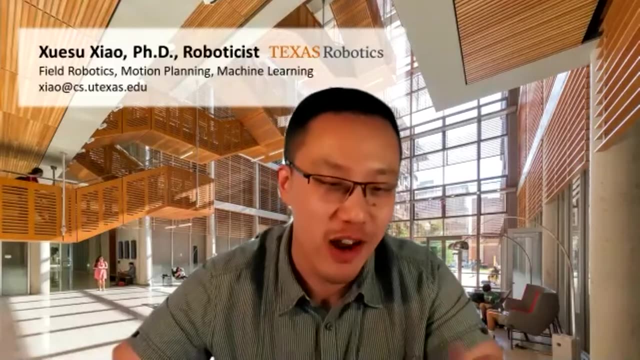 know, and whatever the the like front end, the edge computers, the edge robots is doing is only the learned product. the policy is like: just download it from your server and then try to improve their performance because i and laura is not here- i hope she's here because i i don't want to badmouth. 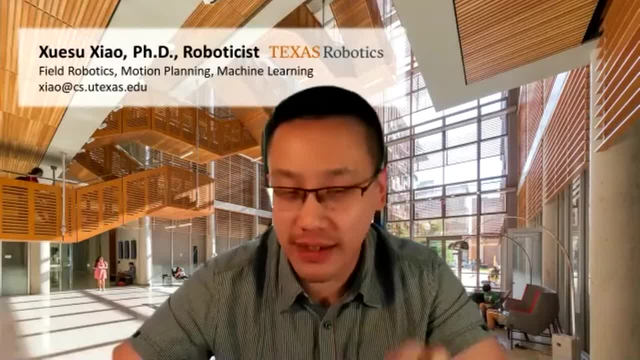 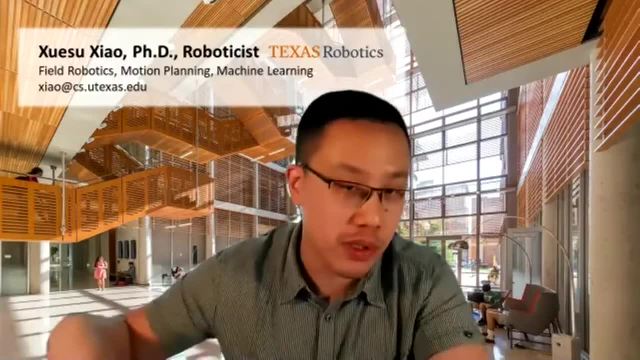 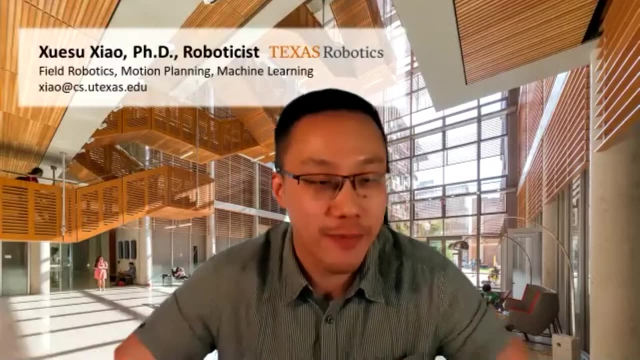 i robot, right, but? but the case is sometimes it gets stuck in our homes, quite often, right. usually you need to like pick it up, put it somewhere open and then it resumes. that that's okay if it gets stuck, but eventually we want to get rid of these sub optimal behavior, right? 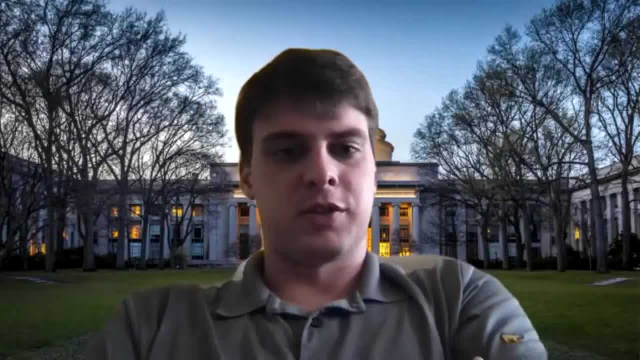 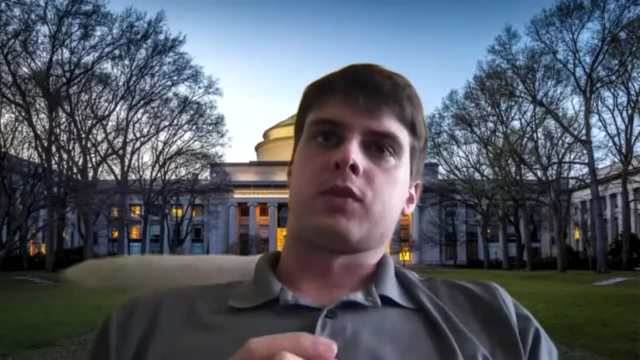 yeah, i wanted to chime in a little bit about something that was. i forget who said it, but a couple minutes ago, uh, i think interpretability and whether these things can be verified came up, so that's been something i've been looking at a lot in the past year or so is. 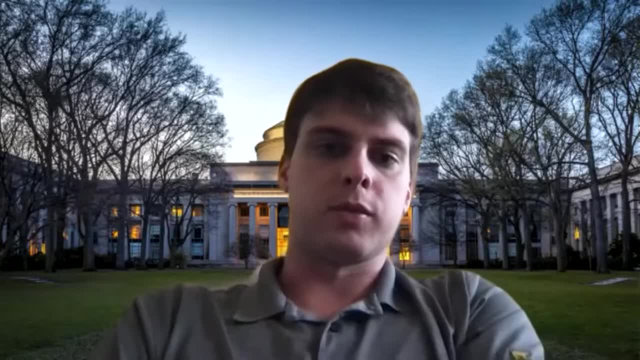 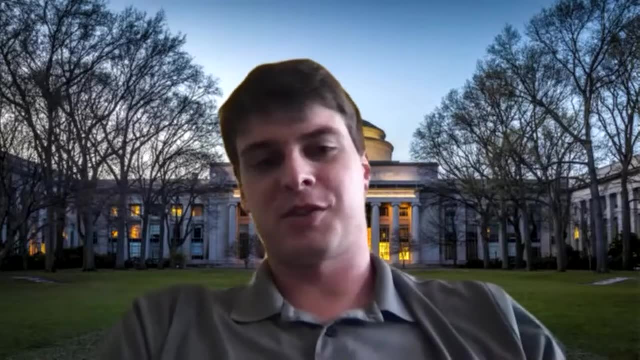 like: what sort of performance guarantees can we provide for machine learning systems? because i think it it has been the crutch and the easy answer for a long time of we're going to use classical things because we don't know how to verify machine learning. i feel like there just 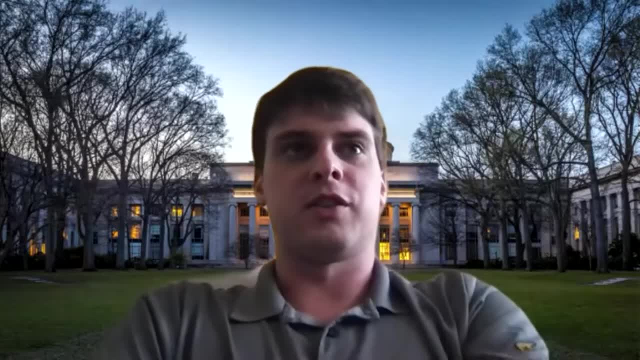 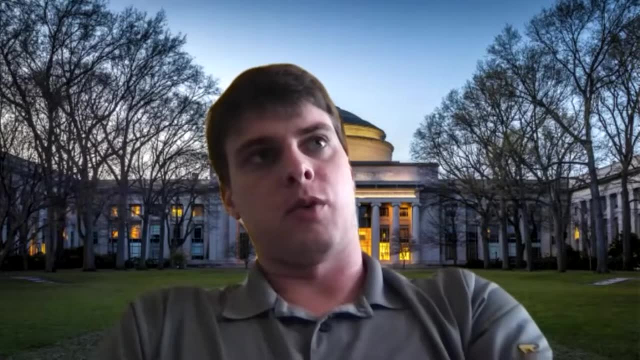 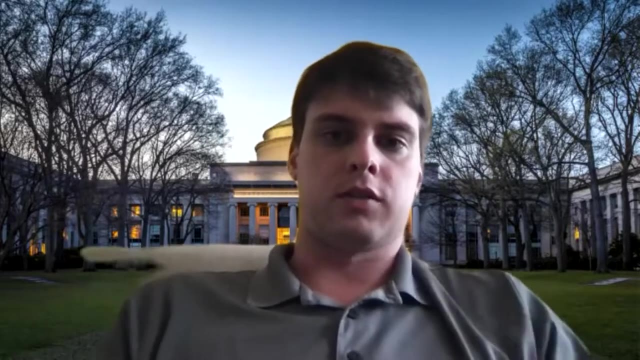 needs to be more effort in coming up with the tools, rather than just saying it's never going to work. so the question comes up. they're like: what, what properties do you even want to verify, and what sorts of guarantees that exist in classical systems actually represent the real? 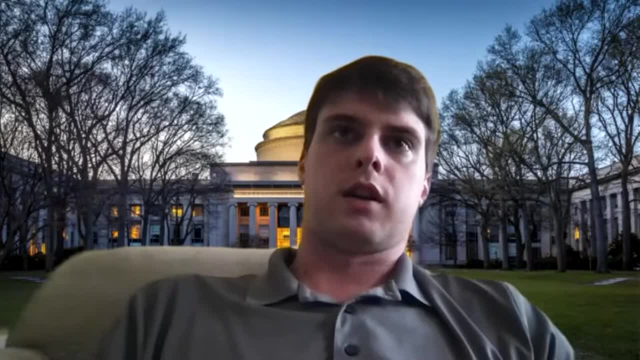 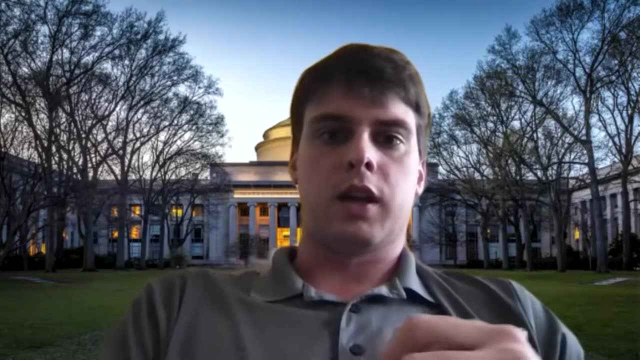 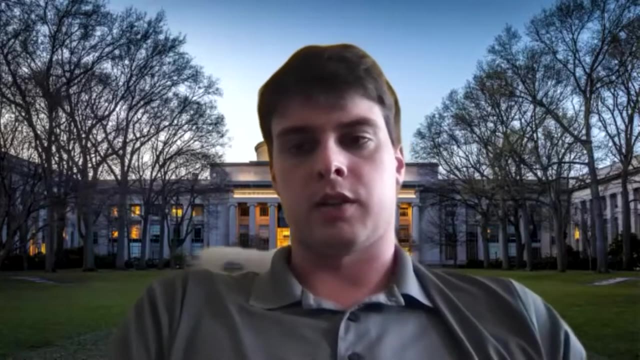 world because you know i could, you could take like a, you know, a dynamic obstacle avoidance algorithm, say from like 10 years ago. it has some like hard guarantees that if you assume something about other agents in the world it will avoid them, and sure you can come up with those guarantees. but 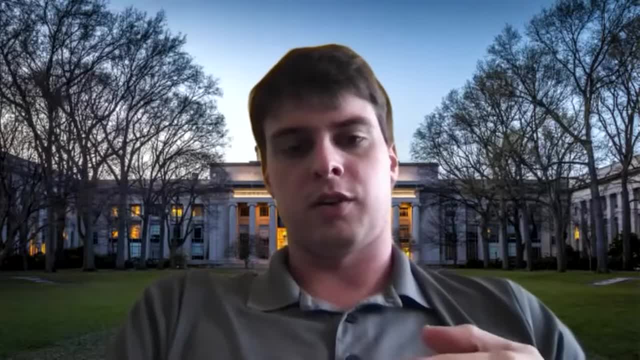 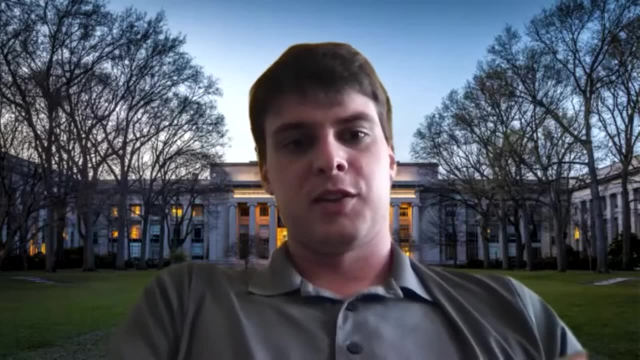 the real world. those assumptions about what other agents are going to do in the world aren't, probably aren't going to hold. uh, so then you're back in the same boat of now. you have one algorithm that you can maybe explain it well, but the guarantees don't really mean that much in the real world. and then you've got a 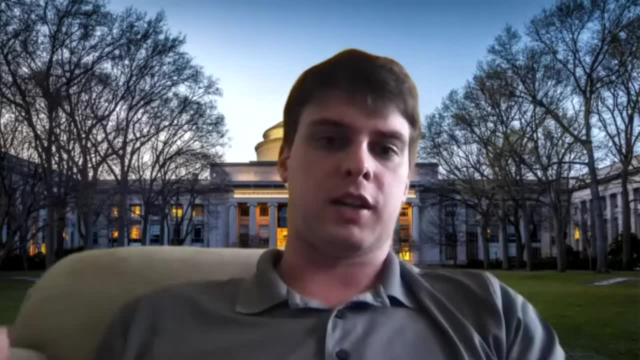 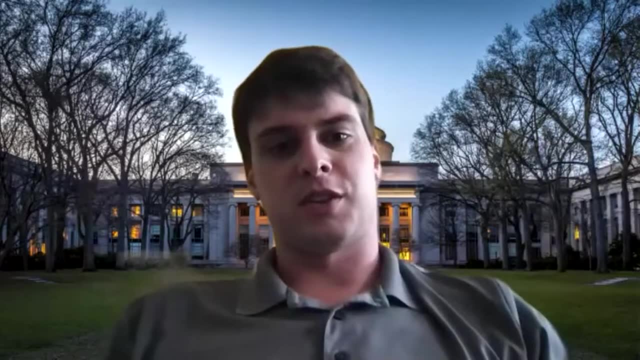 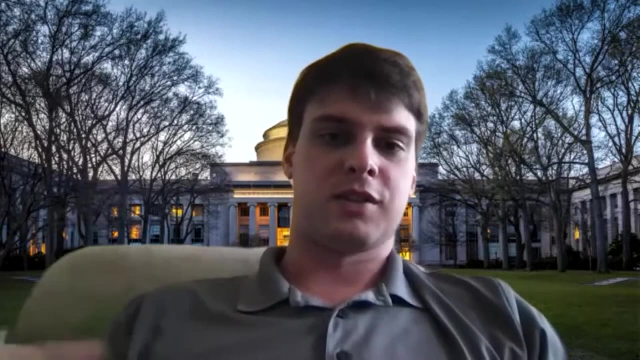 neural network that maybe performs even better. you can't explain it, but you also can't guarantee anything about it, so i don't know. there's this like question of which of these things are the most important here- explainability, verifiability, performance- and at some point do we just give up on 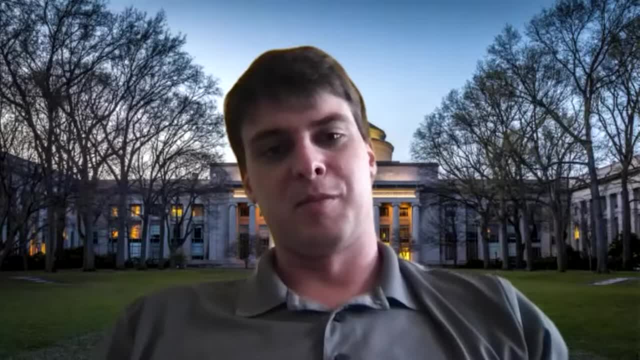 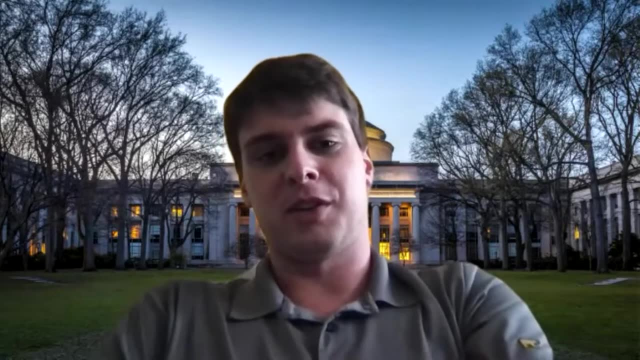 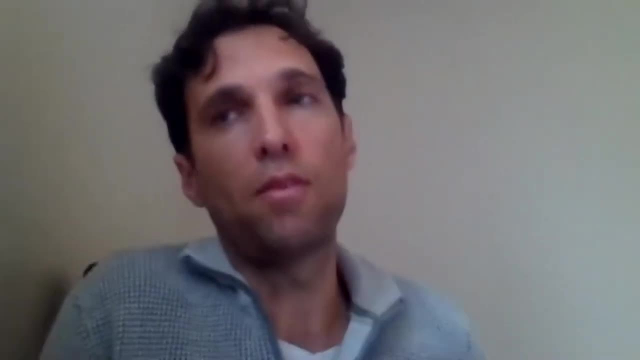 explainability and say: if it works, it works. uh, i'm i'm trending in that direction nowadays, um, and i can also talk a little bit more about the verifiability stuff that we've been doing, if that's interesting to people. yeah, i think. i mean, i think that the way forward would be to um learn within. 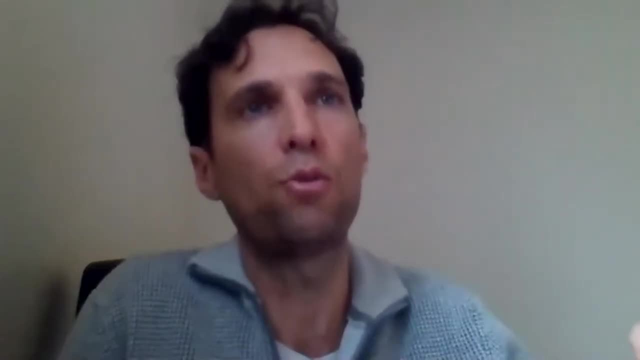 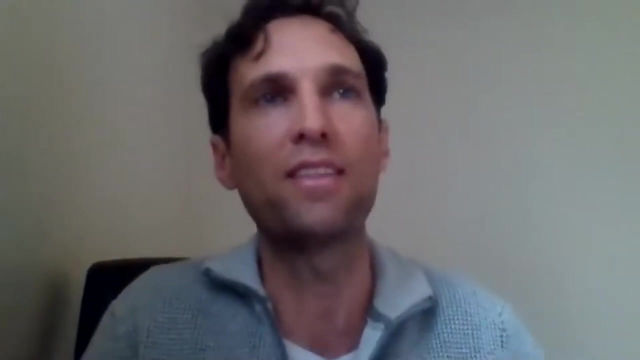 safety guarantees. like what you said, your robot used to move, but it had some, some guarantees that it's going to run into people. um, the same goes with, you know, autonomous vehicles. we're learning driving policies but, uh, we still have these uh hard-coded rules of don't go too close to the 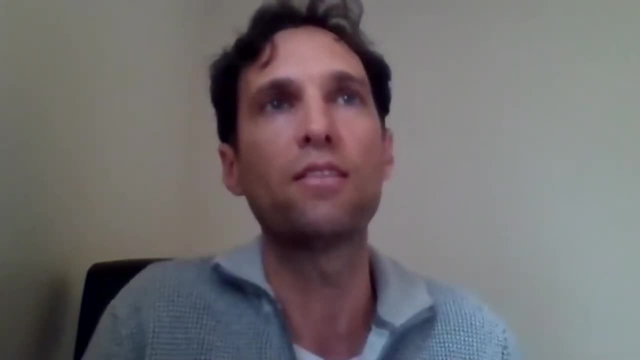 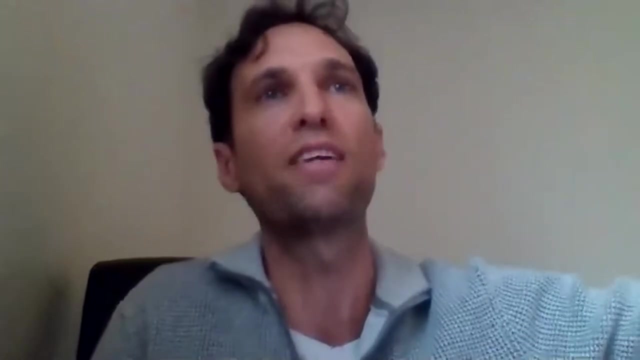 follow to car, you're following and everything, so you're learning within those guarantees, um, and i don't think that at any time we're going to be able to say, okay, we're putting these aside and we're leaving it out of the machine learning algorithm to figure out, even though we're not sure. 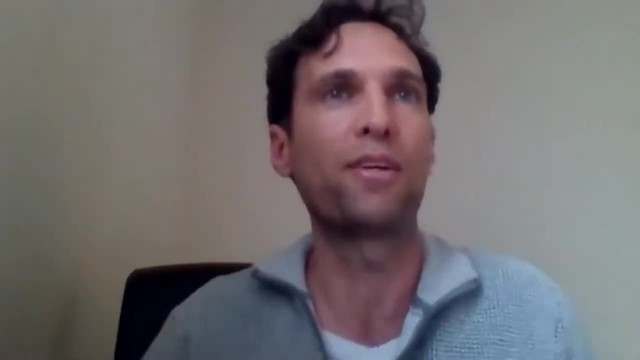 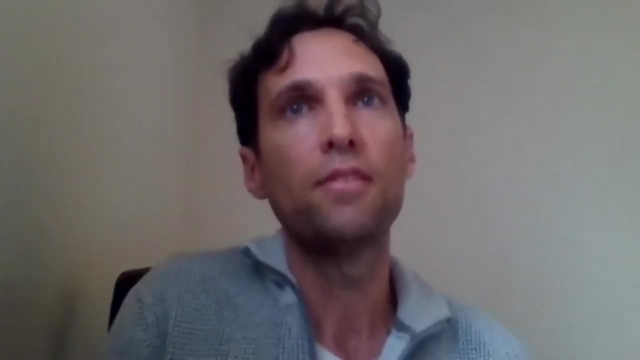 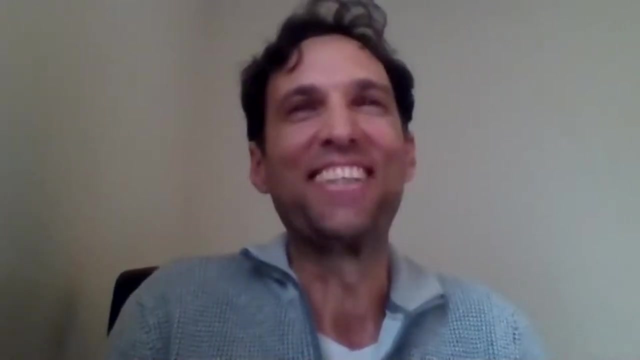 that it's going to handle it. um, empirically it it seems to be better, but we're not sure. i don't think anyone's going to drive a car that doesn't guarantee them well plenty of people driving their test list. that's a good point, um. 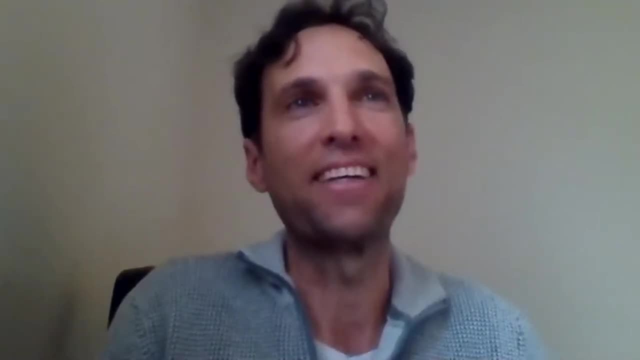 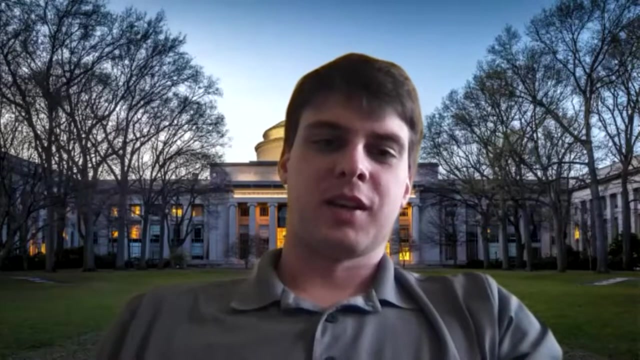 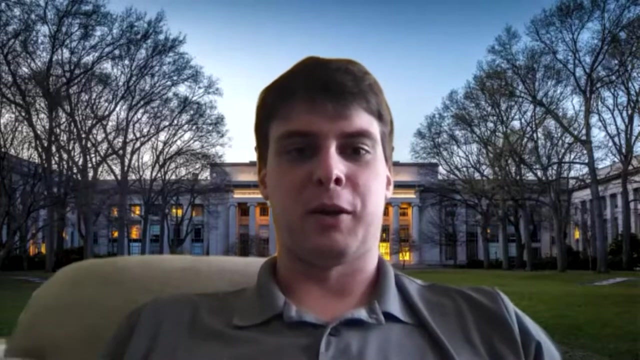 yeah, but again, i'm not sure that they didn't hard code something, um right to override these dangerous situations, right, yeah. and then another question is: i mean, so i get in- maybe not during covid, but i'll get an airplane, and i don't know that much about who. who signed off on it? who guaranteed that it's going to work? 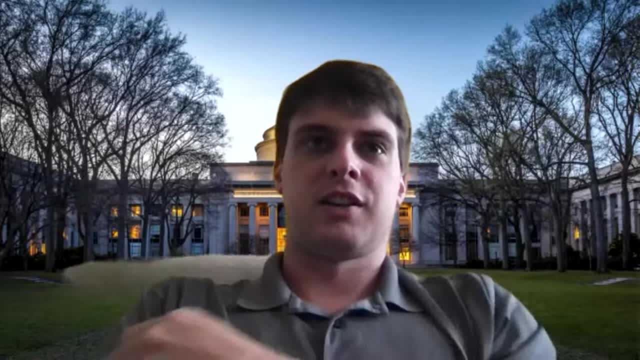 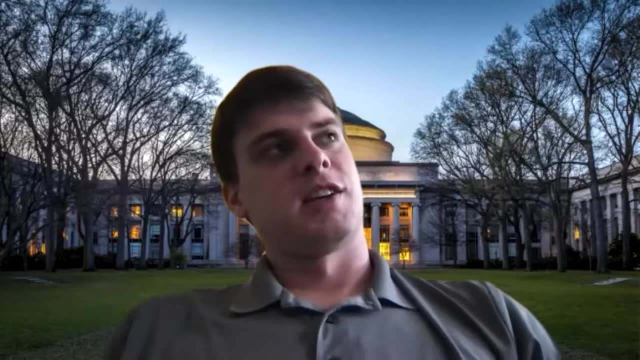 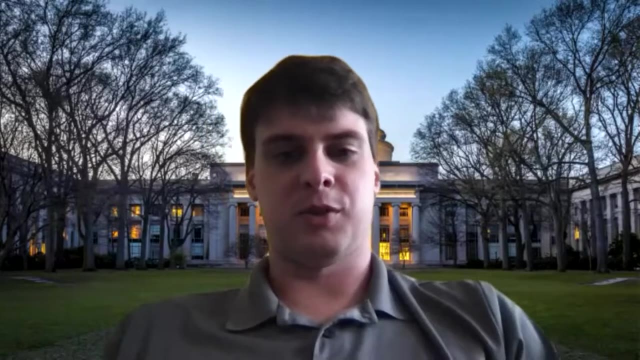 but i somehow have some inherent trust in, you know, a person that's going to be a pilot for me, that's going to get me to where i want to get to. uh, i think that that gets uh forgotten about a lot, that people are willing to give up some amount of like uncertainty in whether the system is going to work very well. 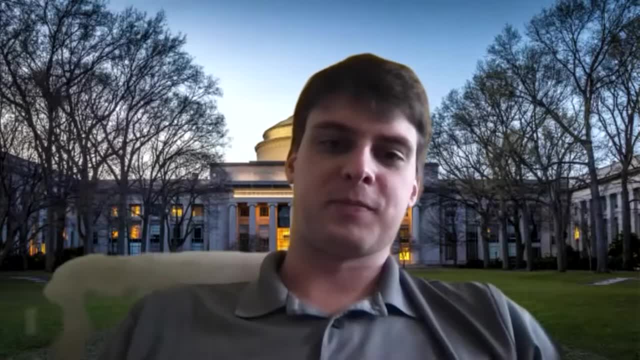 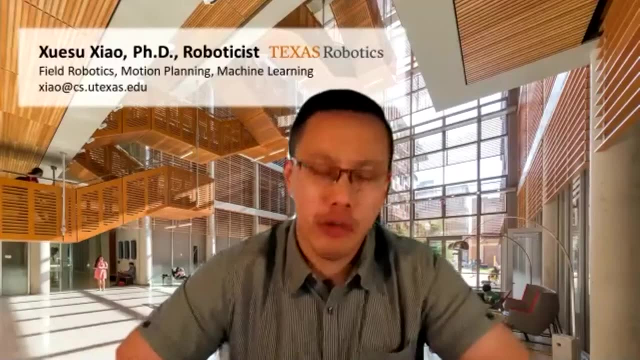 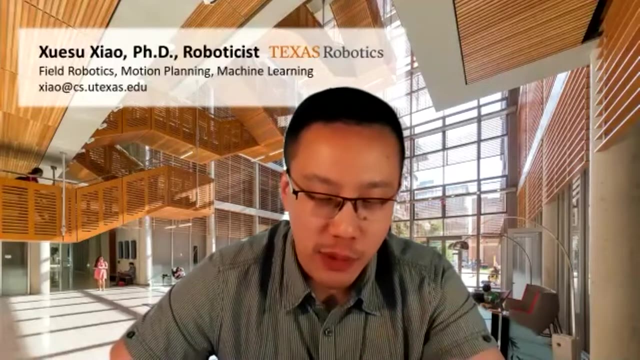 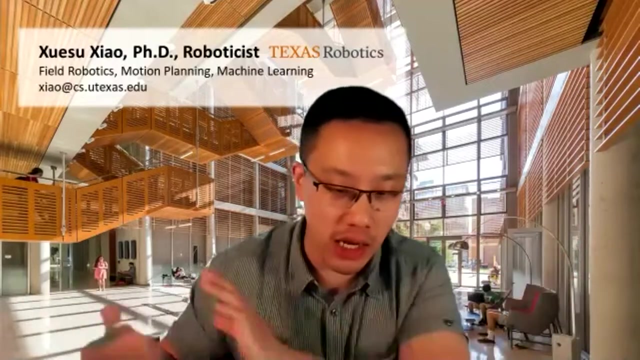 if it provides them a really meaningful service. i don't know. yeah, the other, the other thing regarding safety i have in mind is because i had this conversation with the ball a lot, so because for local planning we think it is pretty good for for learning to do, because, like when we navigate in a highly constrained space, when we navigate in a 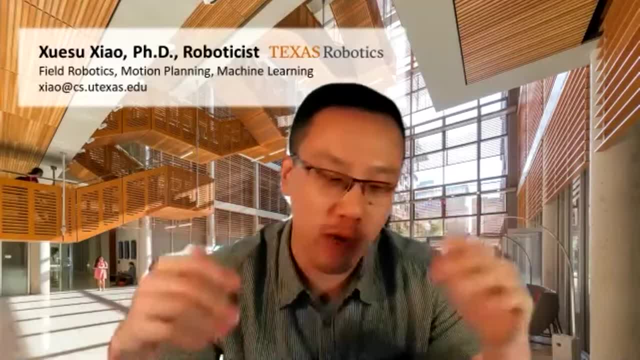 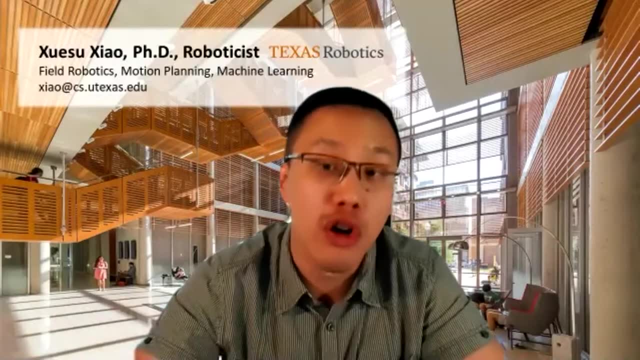 like tight spaces. we don't actually reason a lot like. we don't do sampling, we don't do optimization, right, we just react. that's somewhere. it is very suitable for learning because it's reactive. right, we can train a very small neural network to do those local planning for us. so it's very reactive. 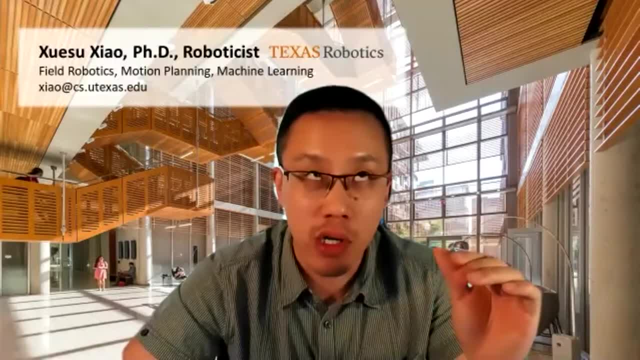 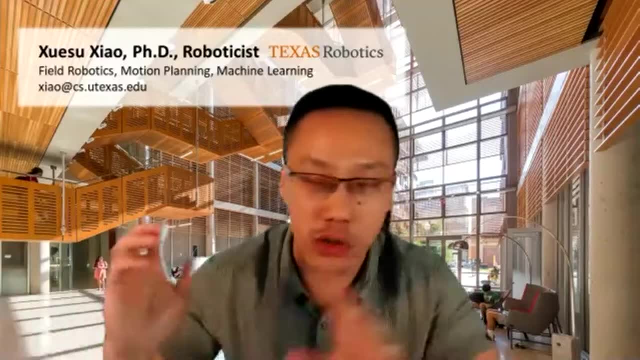 but on a global level, it's better for very sophisticated reasoning, right? so if you want to go to the airport, which highway you take? which actually you take? how do you? which turn do you want to take? all these things can be done by public transportation, right? so it's very good for. 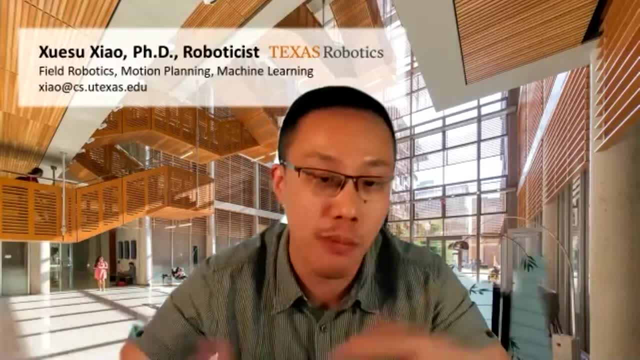 learning. but if you are planned by the local plan or you're planning your own plan, you have to take a lot of time to do it and you have to learn which ways to do it which are the most difficult. so it's very difficult to do. so it's a lot of work and it will be done by planning, by search. 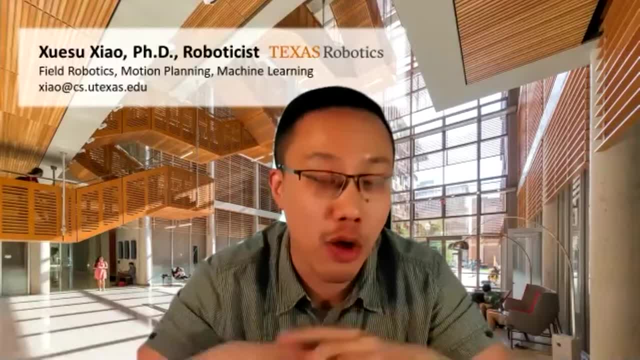 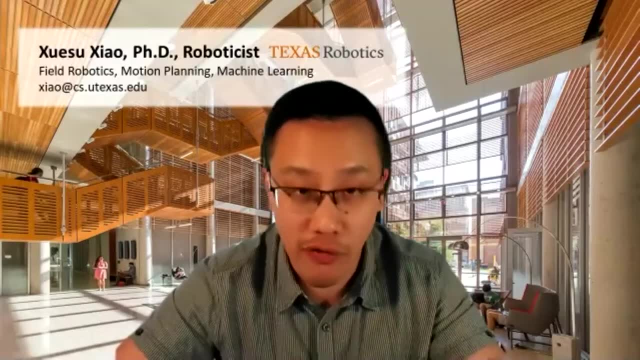 by those like various of its model based approach. so that's our take on this. so, and then i talked to an another professor. we have this argument: um, he's actually a verification person, he hears about all these, but he was telling me: hey, if you do everything you, if you learn the local planners. 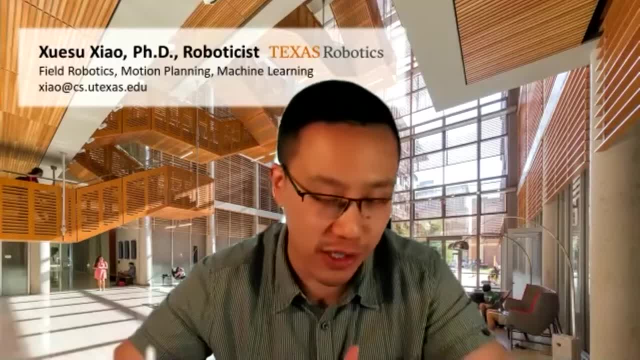 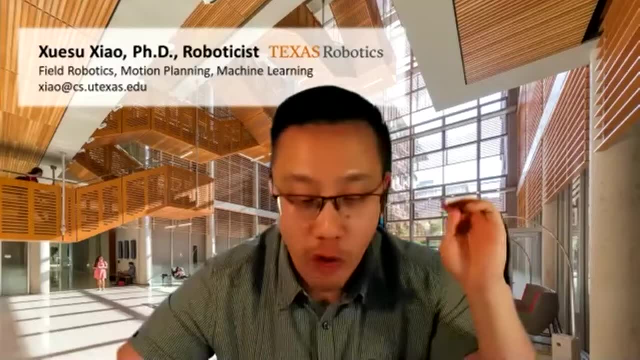 it's kind of difficult to verify because it's learning based. we don't trust it. it may collide with obstacles, it may have very like serious consequences because you are learning the raw. So his idea is we should actually learn the decision-making modules on the high level. 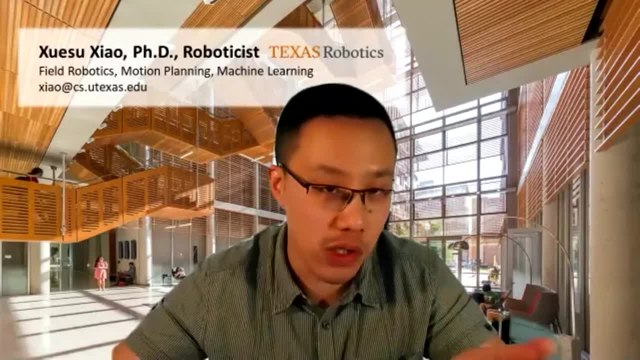 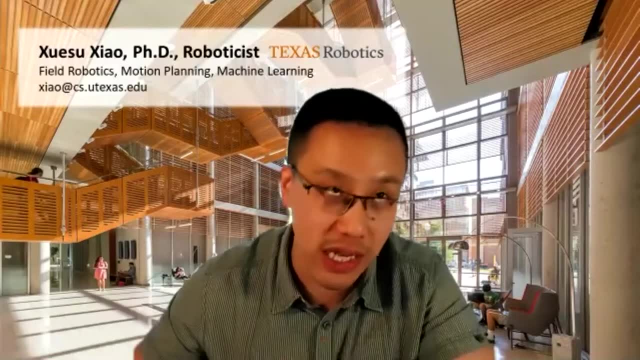 If all these decision modules are learned, it won't interfere with the low-level safety, because the low-level safety are still the classical methods, but they can be verified, as safety is explainable. all these benefits from the classical words, And that's actually his point. 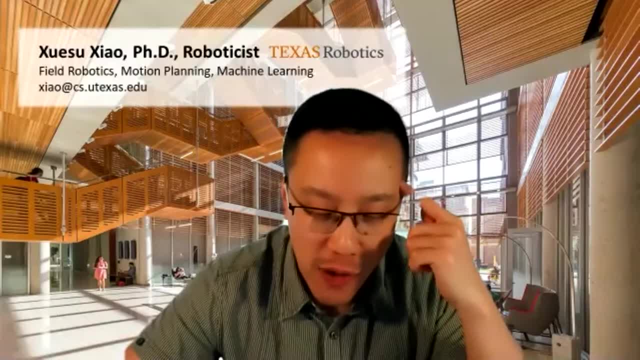 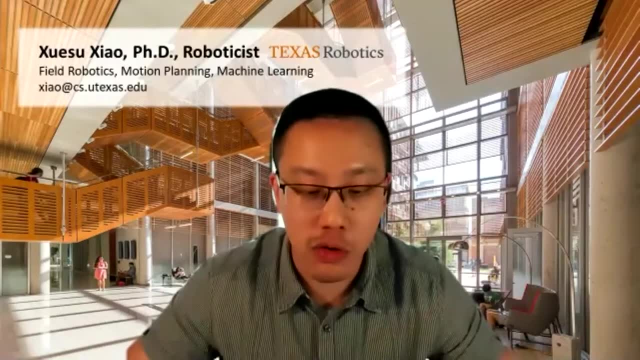 So I saw genius here, So I had this survey paper on just classical navigation using. so basically how people use machine learning for classical navigation problems. There's only one work- I think it's from Jean's group- that's a social navigator is trying. 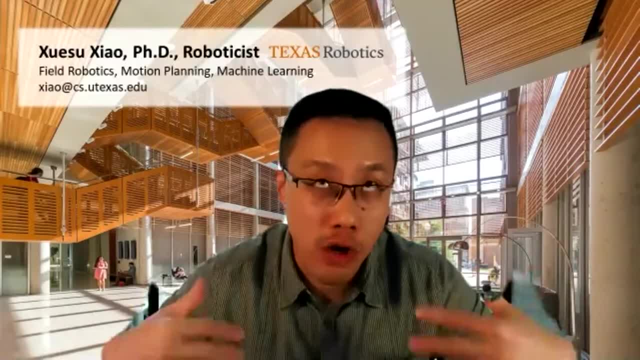 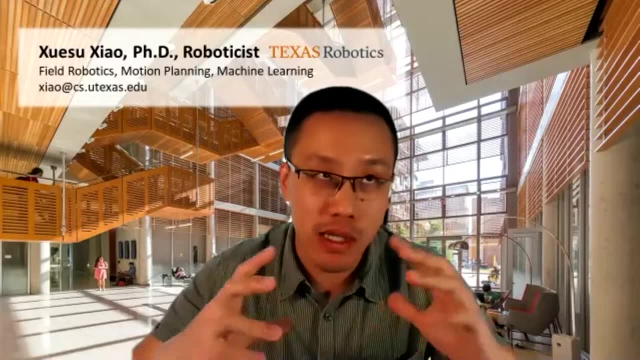 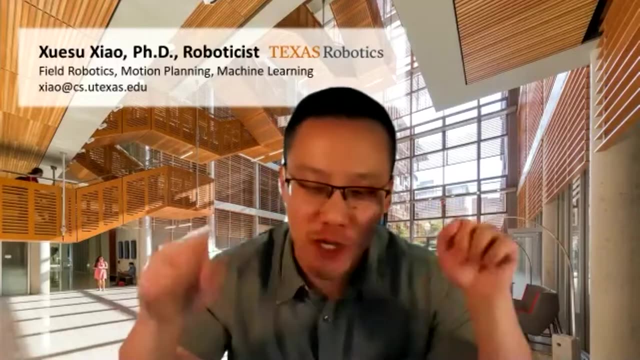 to learn this high-level global planner or global representation. Not many work are doing those, So you are still using the classical motion planners on the low level, but the high-level decision-making, the global planner, is based on a learned social navigator. So I think there's two different ideas on this. 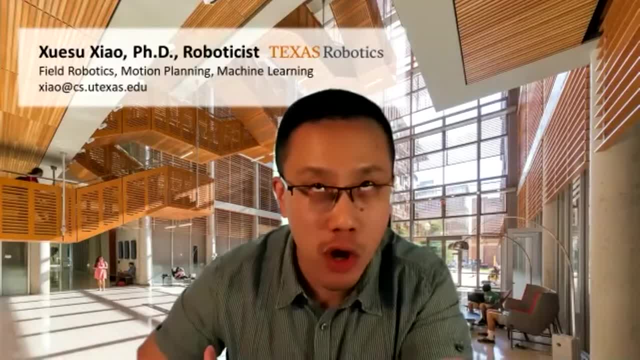 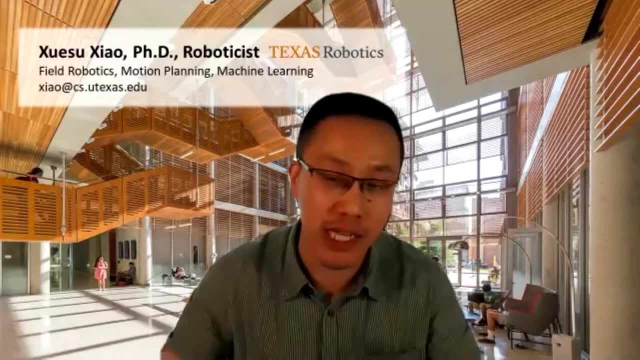 Where should we actually learn? Should we learn the more reactive local planners or should we learn the more sophisticated high-level reasoning modules, decision-making modules? And where does the safety or the guarantees or verification aspects come in? Maybe you have some ideas on this, Jean. 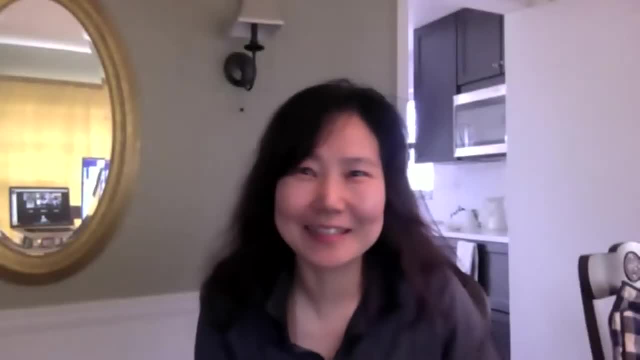 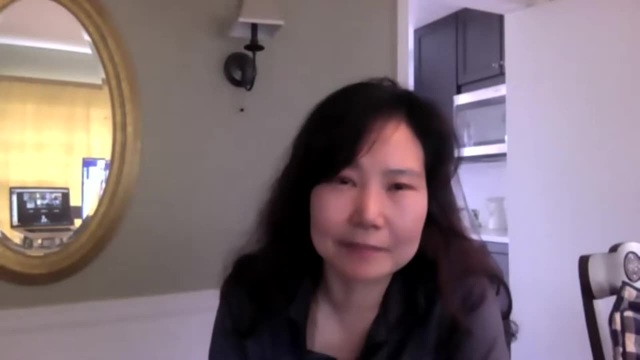 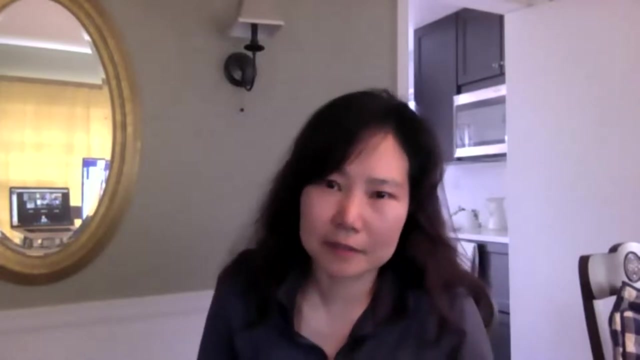 Yeah, so I'm not sure if I kind of understand the context of the conversation that was going on. But for the safety I think that It really depends on the problem domain. So we need to consider this risk part. So in the navigation in pedestrian space, even if there is a collision, the risk is 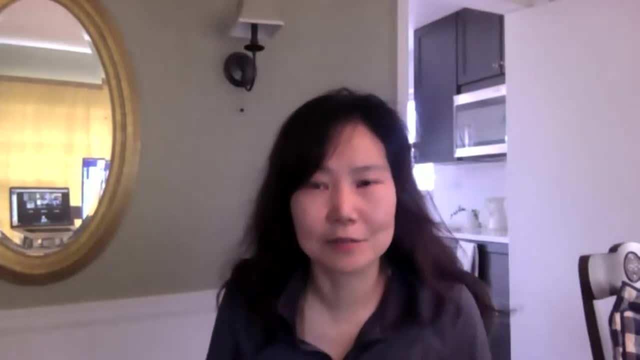 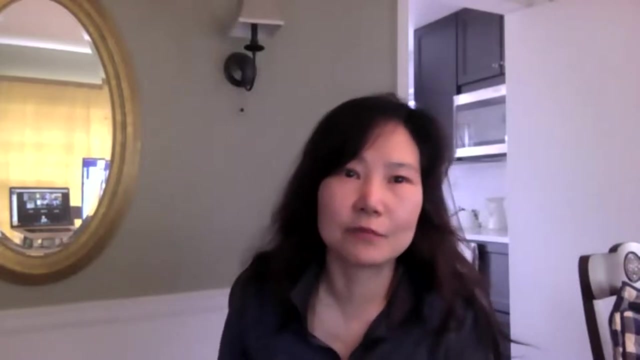 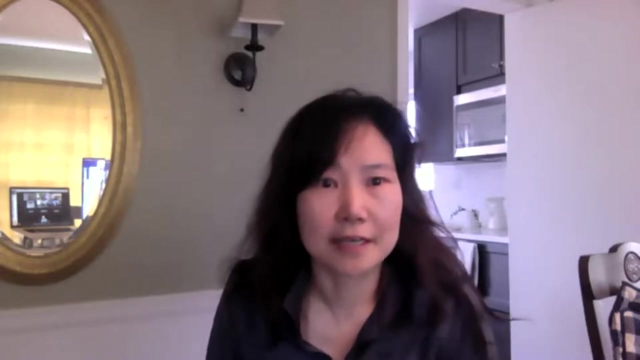 smaller compared to autonomous driving like in a highway. So highway is considered maybe an easier setting because it's clean, there are no people walking around, but they are moving. all the vehicles are moving at a very high speed, So if there is a collision there will be like a fatal accident. 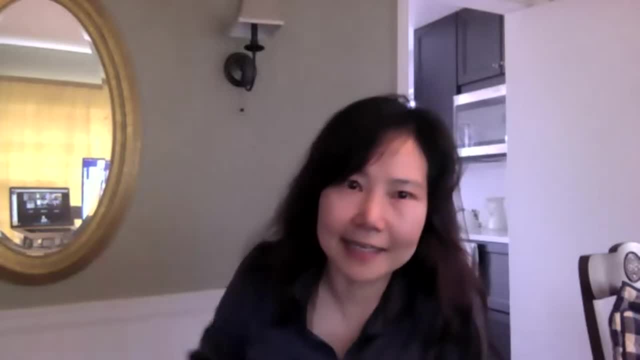 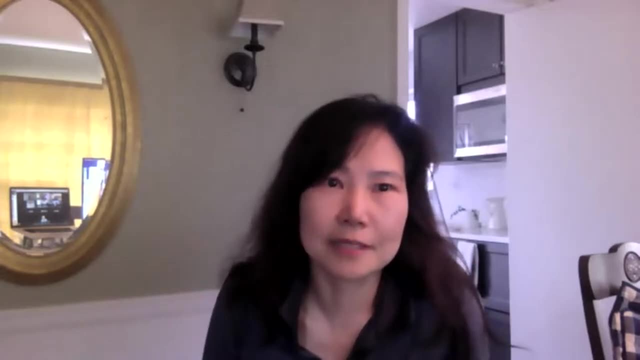 So that risk, because the risk is high. the safety concern is much more like an issue. But in pedestrian space, I think, because even if there is a collision we can get away and probably people may get hurt a little bit, But you know, not always. 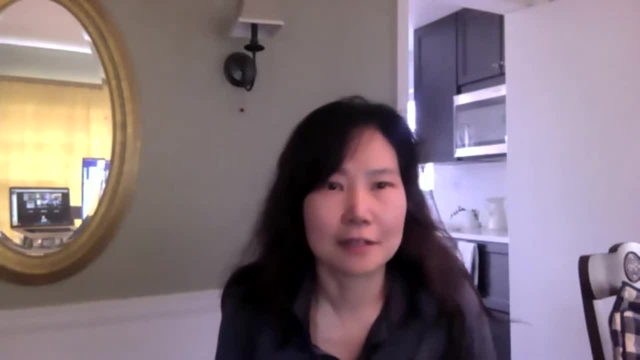 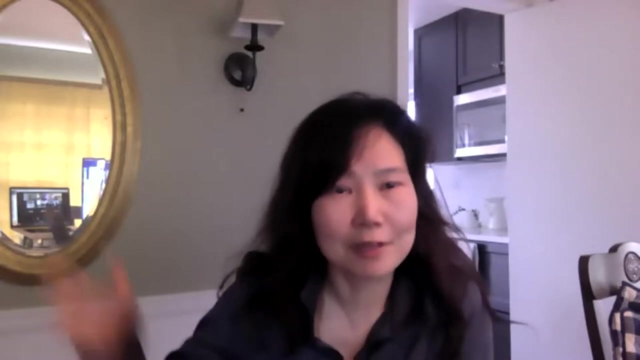 Yeah, Yeah, There's nothing fatal. So in that regard, maybe people are more concerned about the compliance and is the robot behaving naturally enough to mingle with the human population, But I guess. So that's one aspect And the other aspect is the explainability. 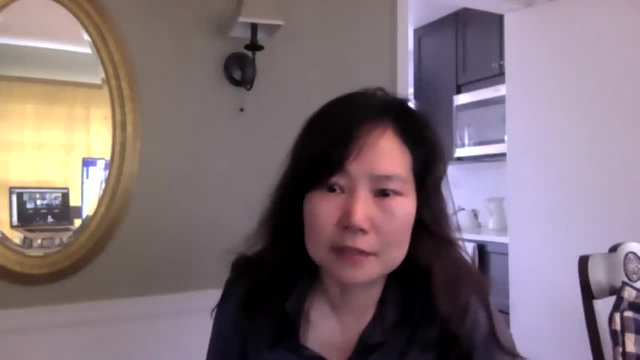 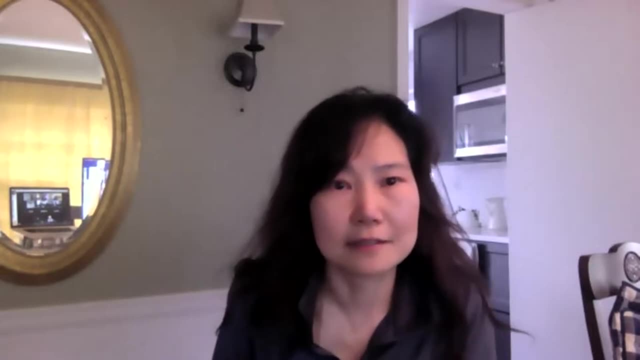 I think Michael was mentioning that And there was some And there was some discussion between explainable system versus competent system. So that's the airplane or other kind of systems that we have. this unexplainable trust is Because we know that the systems work pretty well and there are accidents, but chances. 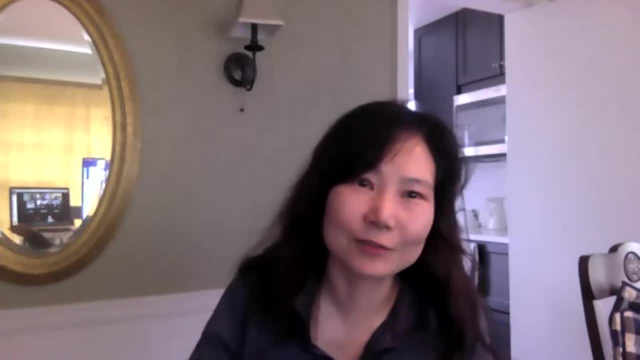 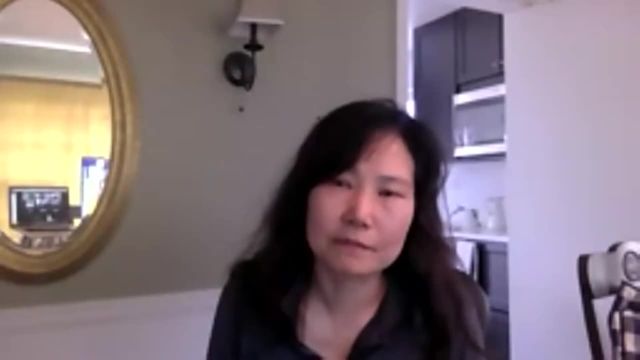 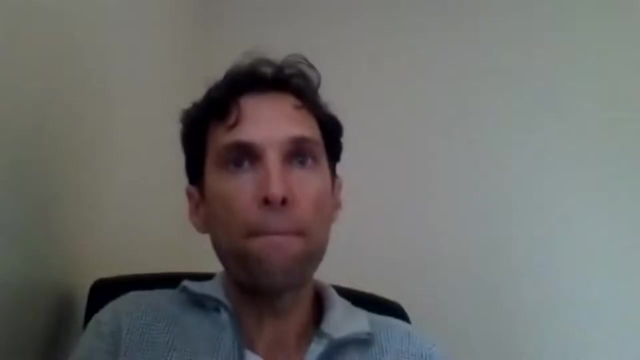 more So to that. that's the chance we are taking, Yeah, So I think people would much more prefer- I mean, to my personal opinion- would trust more competent system than system that is a little bit unreliable but it can explain. 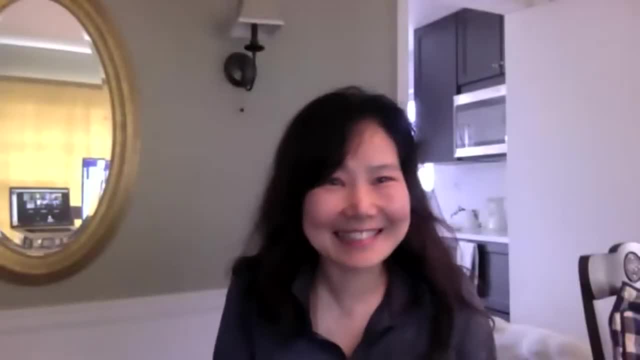 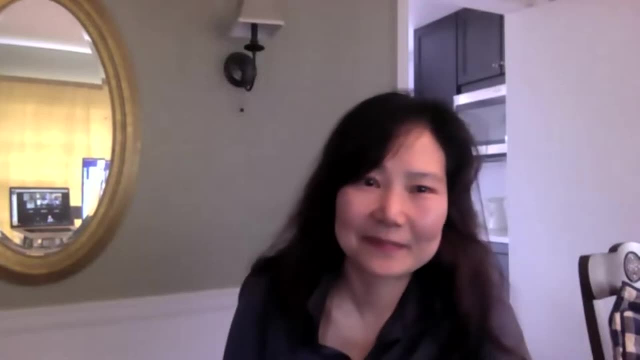 why it went wrong. So there is a trade-off between the two. So that's my personal stake on that. Yeah, That's a great point. Thank you, Thank you, Thank you, That's a great point. There's a lot of value in seeing something perform well. 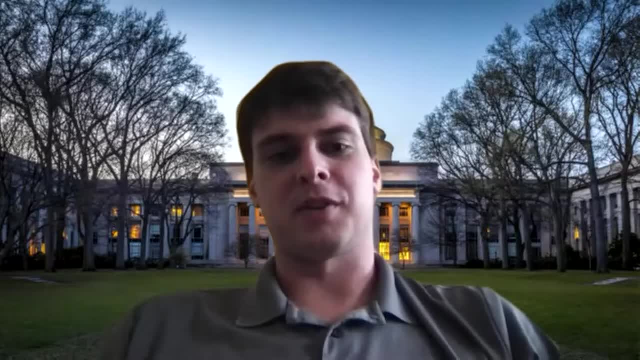 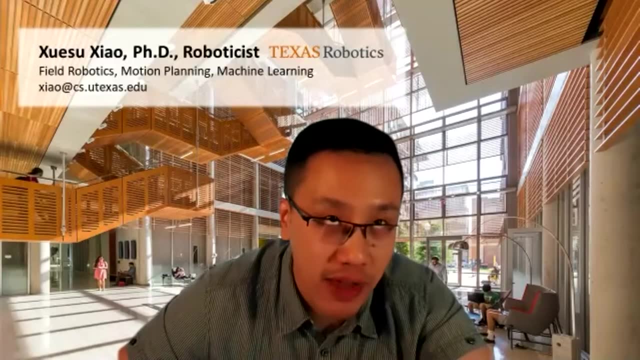 That gives you some confidence, even if you don't understand why it happened. I think that's a great point. So, Jing, what is your reason that you develop social navigation and just utilize all existing local planners? I thought it's for safety. 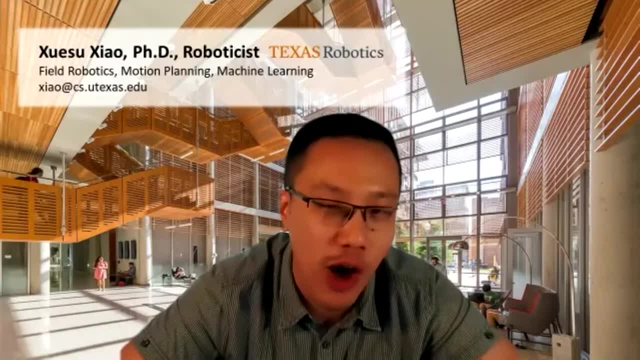 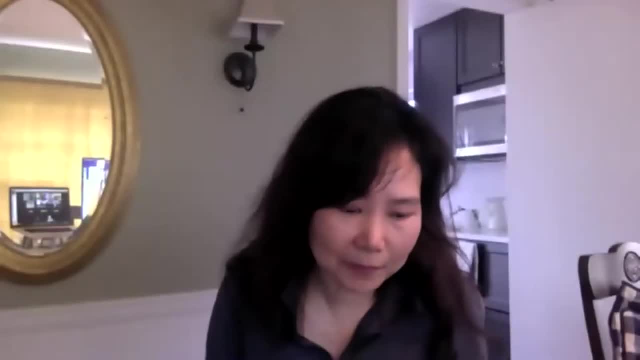 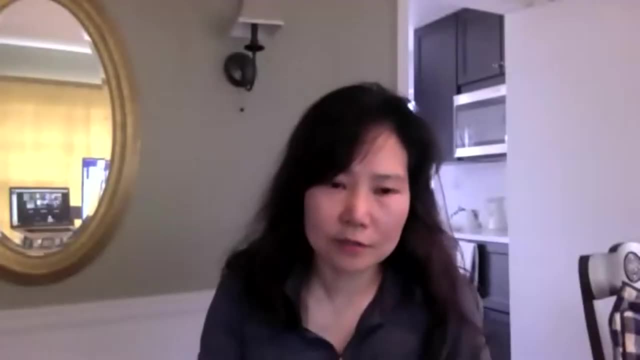 That's what I said in the survey. So that's the reason why you are just using classical local planners, but just try to learn a global plan. Yeah, So for that work, it's more for the general purpose. So there are socially compliant navigation is one type of behavior, but the navigation 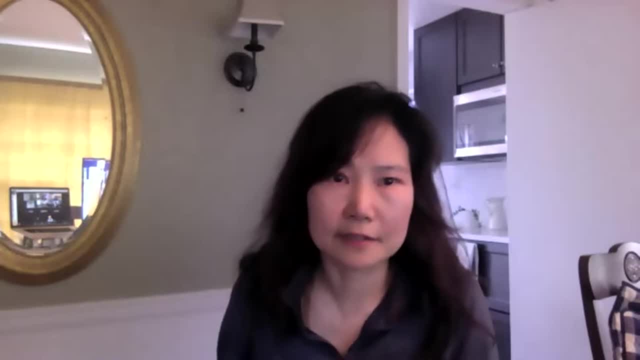 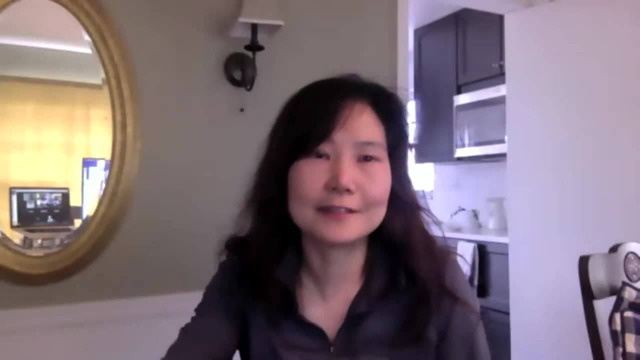 behavior can change depending on different contexts. So there is this level of a higher level reasoning going on to detect the context. So if it's a threatening situation, then you forget about the social context. Yeah, Yeah, Yeah. But if it's social compliance, then you want to be safe. 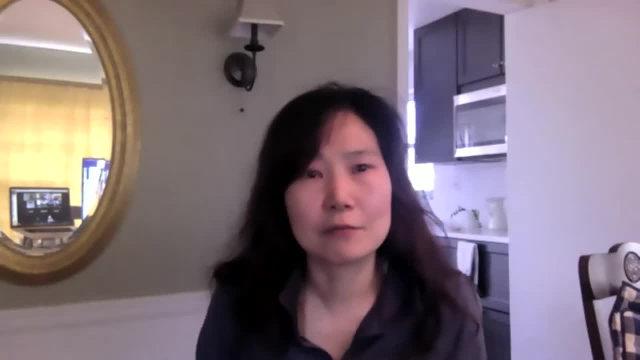 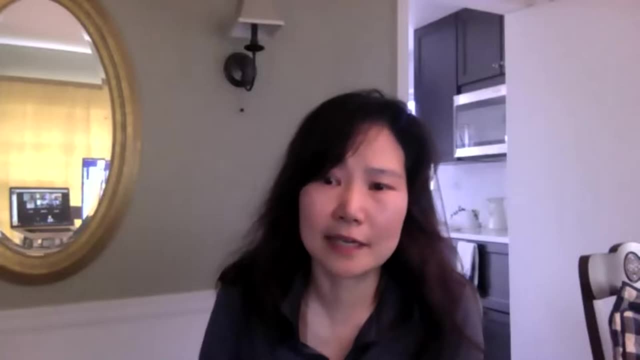 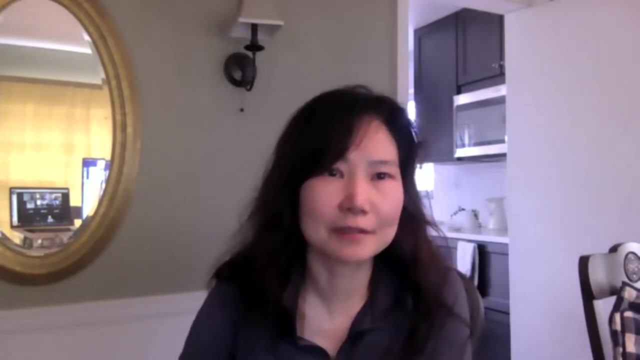 So how to do these context switching? That was more of the reason. And then for the safety part, actually we added a additional loss time in the navigation training so that the It's never guaranteed, but there is a little bit of a notion to avoid a collision. 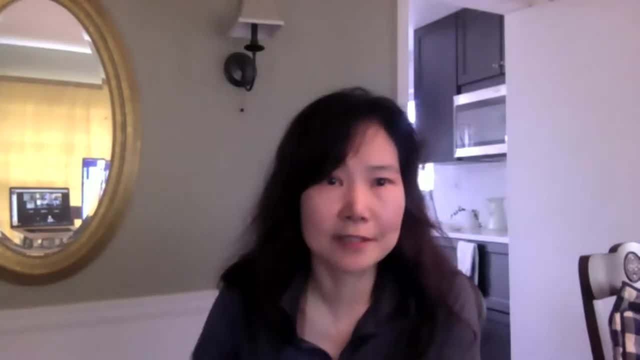 So the comparison to reinforcement learning agents that was actually trained to minimize a collision, it is still a little bit taking a risk, but I think just having that term was the factor that actually ensured the safety in avoiding collisions. because all the data driven approaches, it's very subtle. 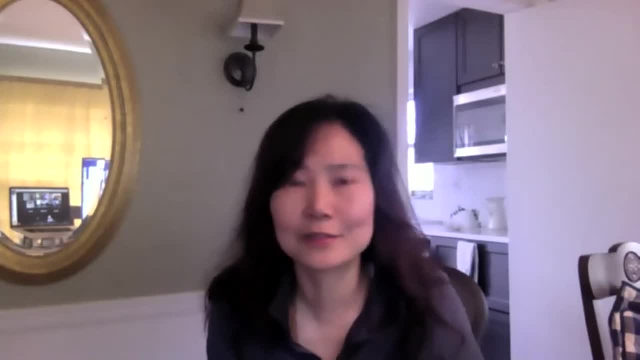 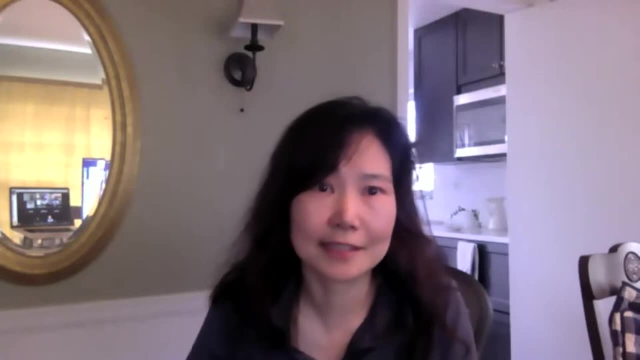 So in the training data there was no collision. so it is less likely to see that kind of behavior during the test time. But if we run just a lot of simulation experiments in self-play, we do see a lot of collision actually happening. 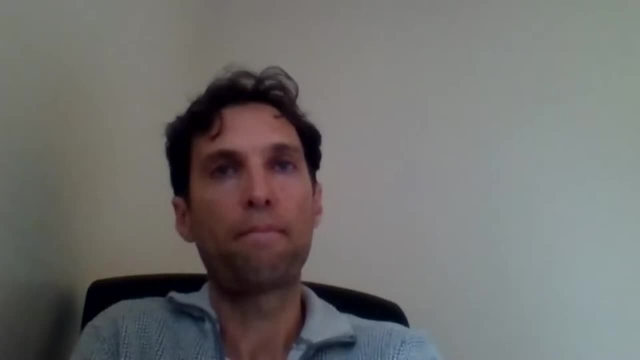 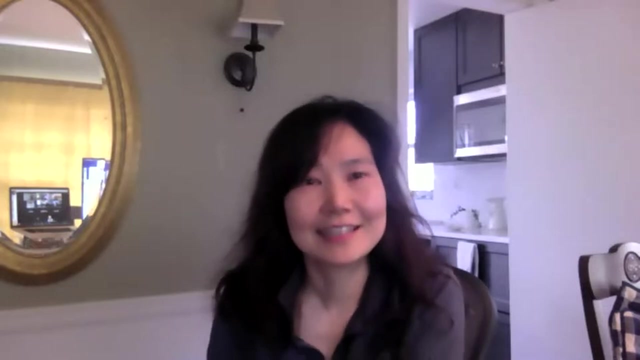 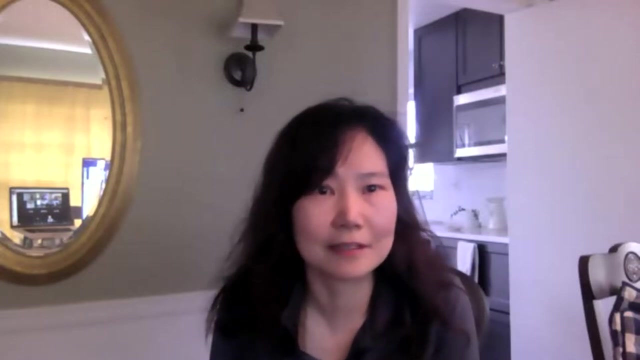 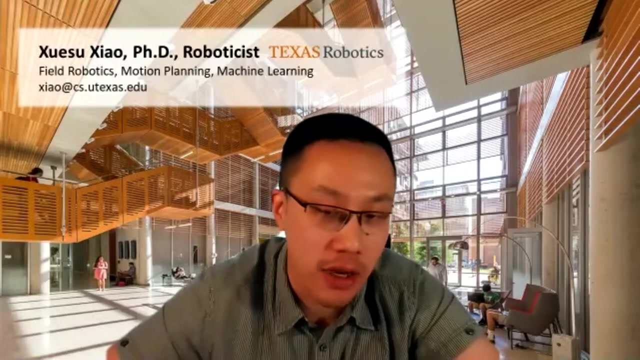 So there is no objective to avoid possible collision. So even if the learned behavior is not consistent, it's still a risk. So the learned behavior is implicitly collision avoidance. but there is no understanding of like collision is a bad thing, But if you are using a classical local planner, then the collision avoidance is taken care. 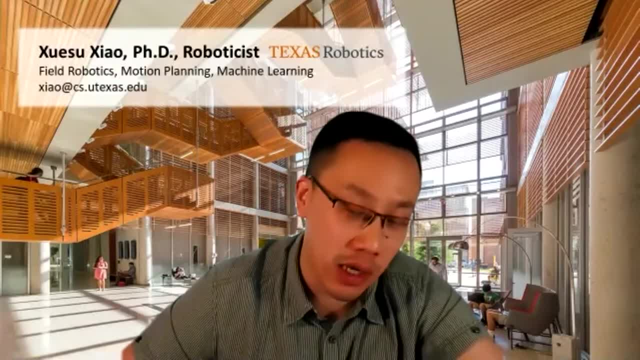 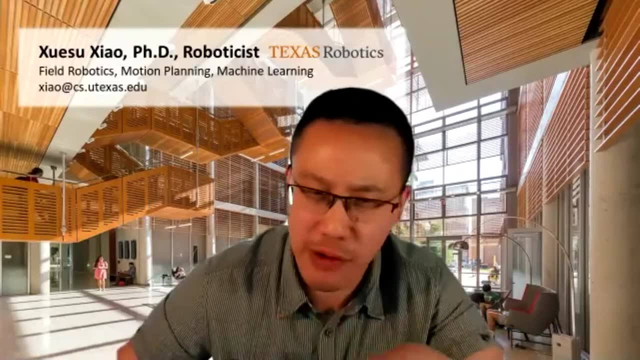 of by the classical local planner, right? So then, if it still collides, that's not the learning module's fault, It is the classical local planner is not well enough. Yeah, it's hard to kind of draw the line, Right. 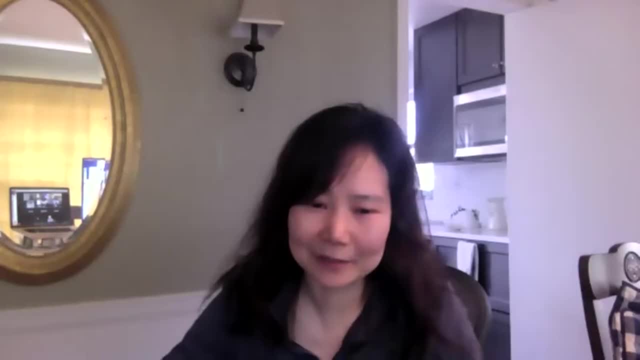 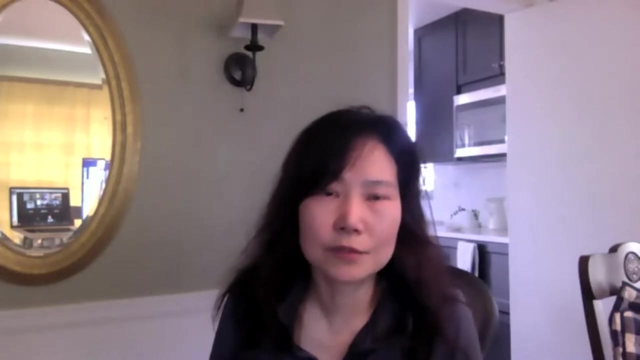 It's hard to explain what that is, because maybe the local planner thought that it would get away or avoid the collision, but maybe there is a localization issue, So there is a low level of autonomy that can cause that collision. Also, maybe the global level plan was barely safe. 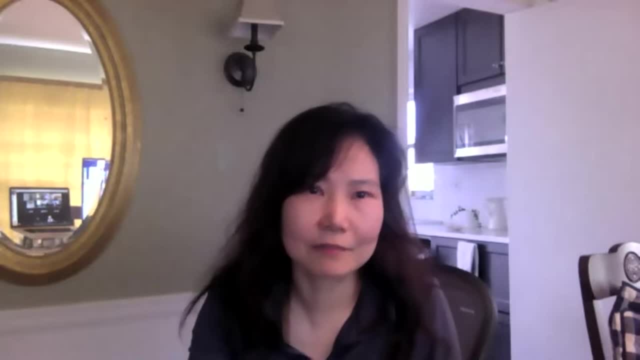 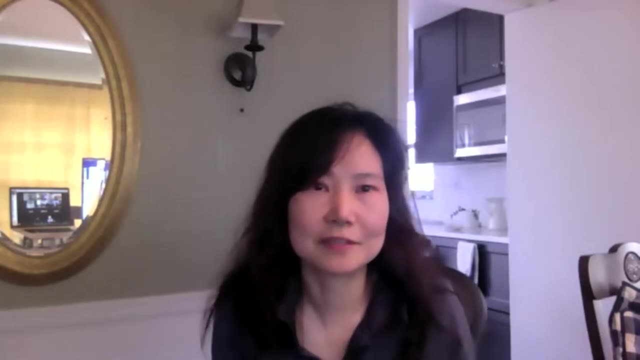 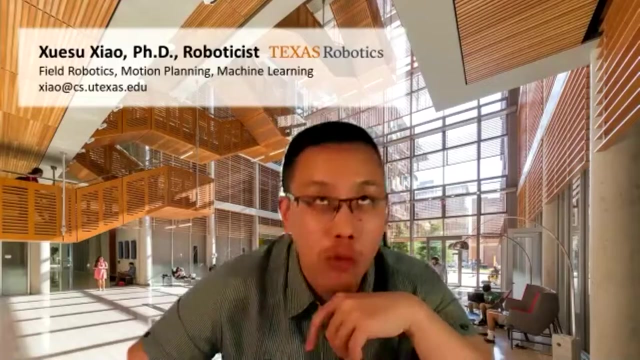 So there is a way to avoid the collision, but with the uncertainty lying in the background, in between like perception and local localization areas, it can happen. So I think it's a combination of. So what you're saying is also the global paths planned by the global planner is also somehow 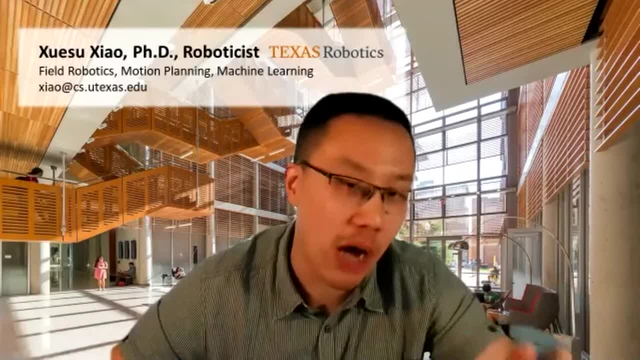 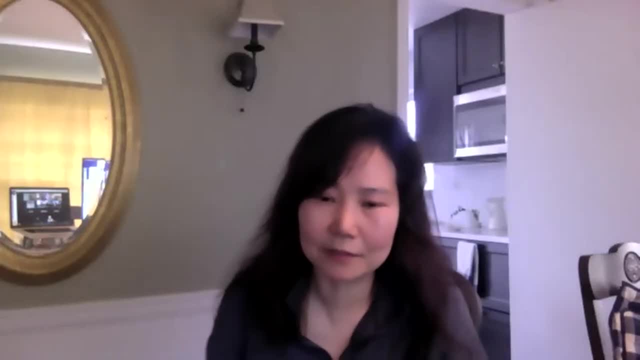 responsible for the collision because you assign the global goal too close to an obstacle. Maybe that's the reason why it's eventually collide. Right right, Because you know, maybe the global planner saw enough pathway, Yeah, Yeah, So that maybe the local planner will handle going through this narrow, cluttered space. 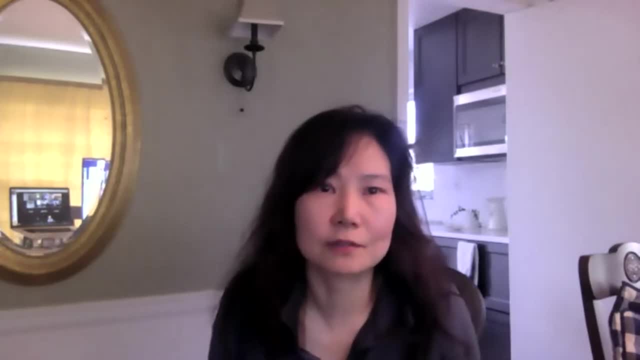 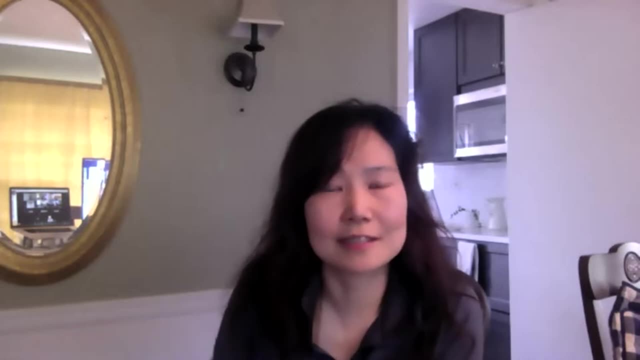 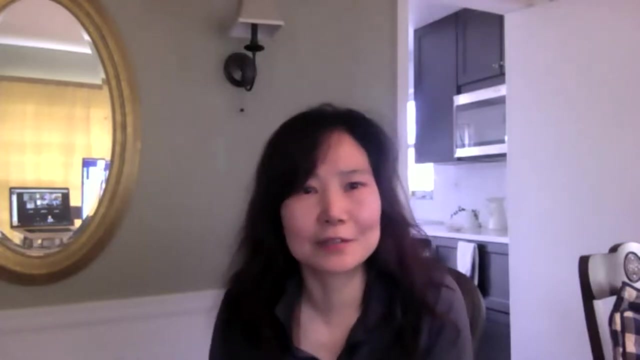 but maybe there was too much uncertainty. So you know there it could have made through. but also there is a high chance, high probability, that it might have been so, because it could have routed differently to maybe less cluttered but maybe less optimal looking path. 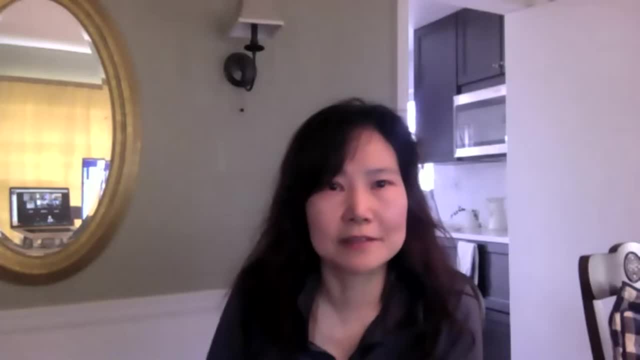 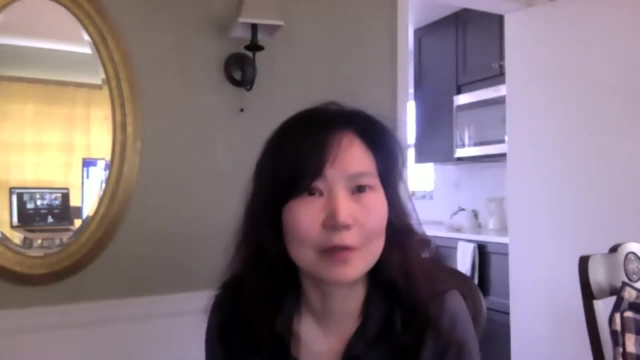 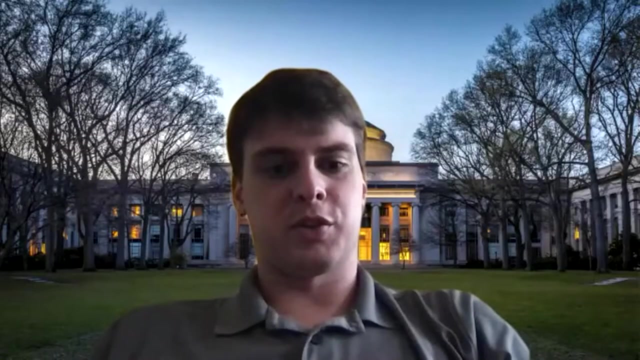 Yeah, Which is safer, but the global planners decision to let's give it a try on this narrow path. Maybe that was the part, part of the cause, That's. I like that where you described it, Jean. we just had a paper that was accepted. 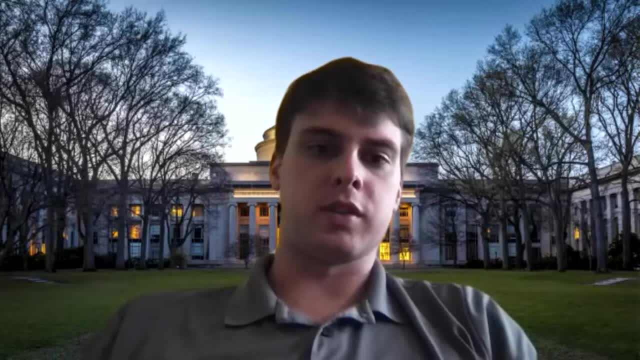 to Raul and IKRA and we basically do MPC for a local planner and we we try and learn a policy to select the global sub goal, So like. so you have some global goal, maybe a hundred meters away, and then the sub goal. 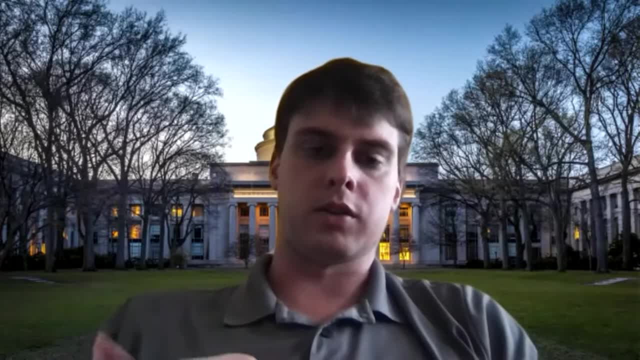 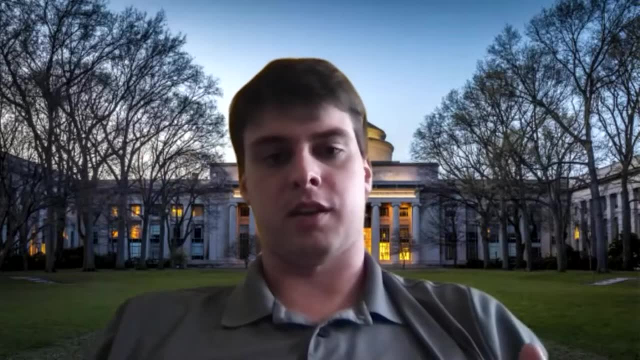 planner is learning how to place these carrots 10 meters in front of the robot so that we get these. you know I say in quotes: guarantees that the MPC is not going to collide with anything. You know, I say that in quotes because I don't really think you can guarantee those things. 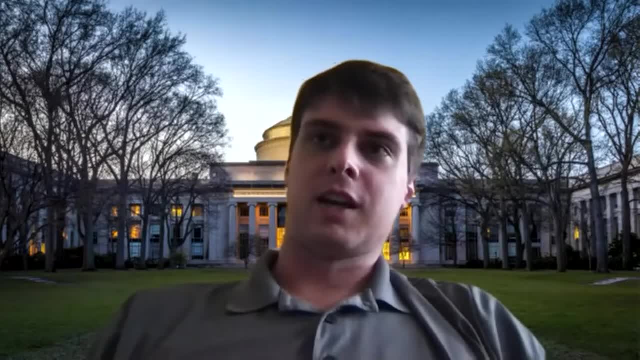 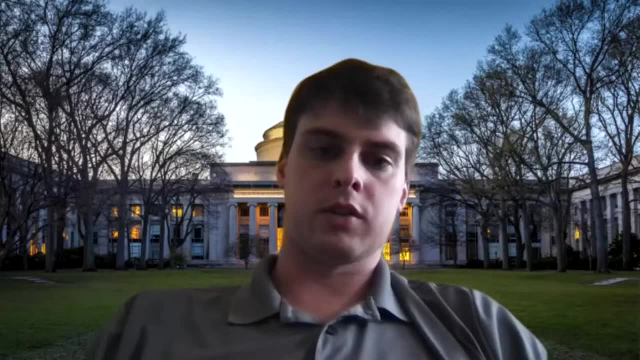 Even if you have hard constraints that you satisfy. but yeah, so basically there's a, an MPC that plans a trajectory to try and reach that sub goal. Yeah, Yeah, That's a sub goal, that's been learned, but then you don't really have to learn the local. 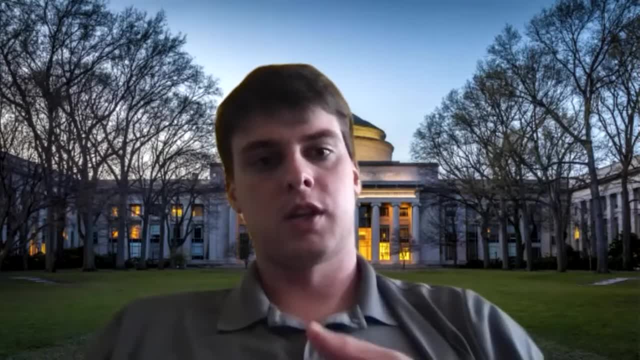 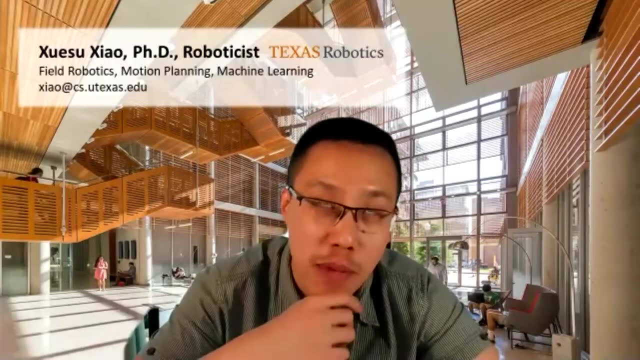 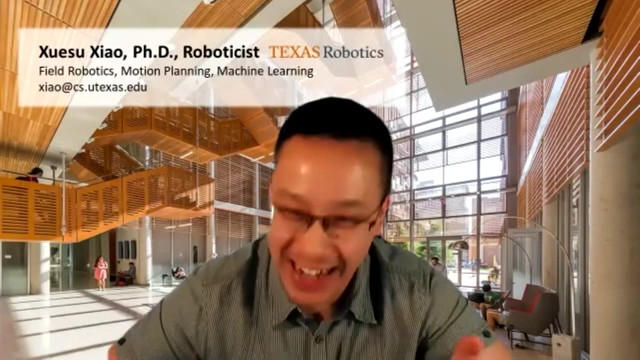 avoidance part of the problem, to try and try and bring those global and local planning ideas together. This conversation makes me feel like maybe we are too early to complain about the safety issues of learning because MPC is still cannot guarantee it Right. Well, yeah, I think it can guarantee. 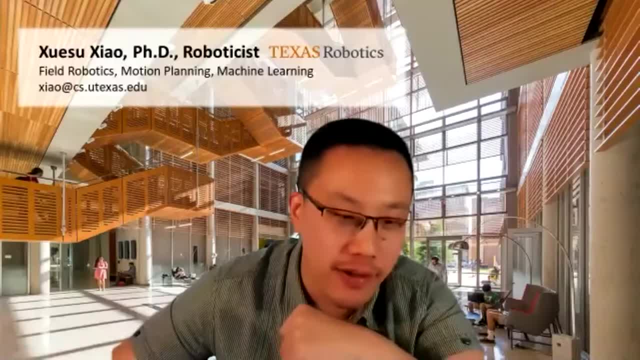 I think it's just. what does it guarantee? So, if you, you know, you have to make an assumption- Yeah, You have to make an assumption- of what other agents in the world are going to be doing into the future And you can avoid colliding with where you think they're going to be according to that. 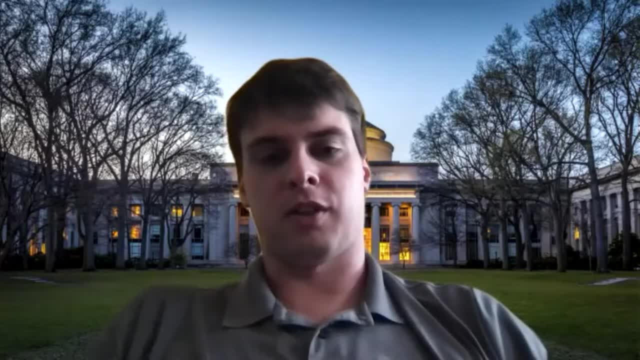 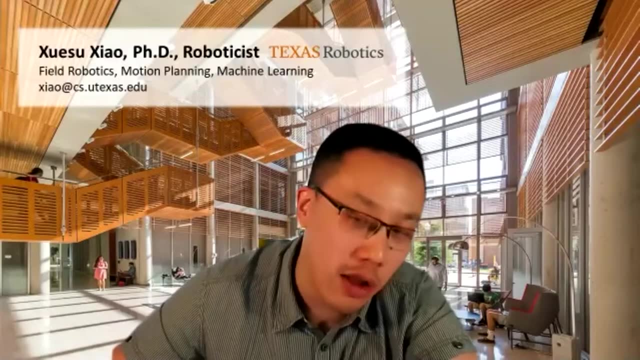 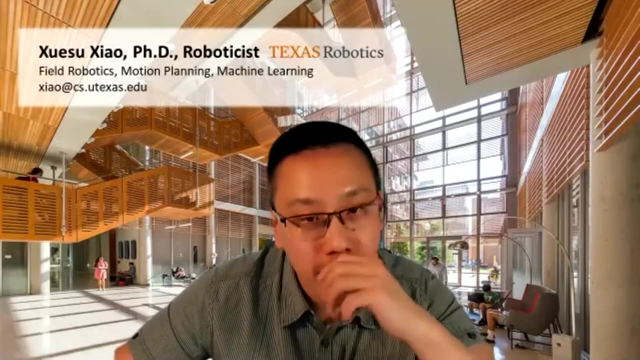 assumption, but they may not actually be there And so then you're isn't really that useful. Also, the assumptions of all the internal components, like localization, like all the noise, sensor, noise, all these things, Right, Yeah, Yeah, Exactly. 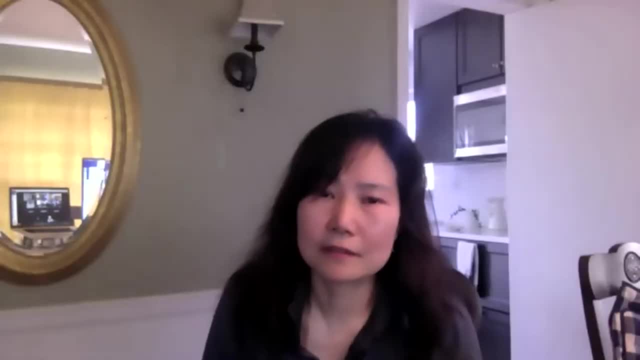 Yeah, And then as the population comes to that, you know the a lot of algorithms will fail because there is no feasible solution. So if we really go into a very dense population, then we also need to think about types of actions. 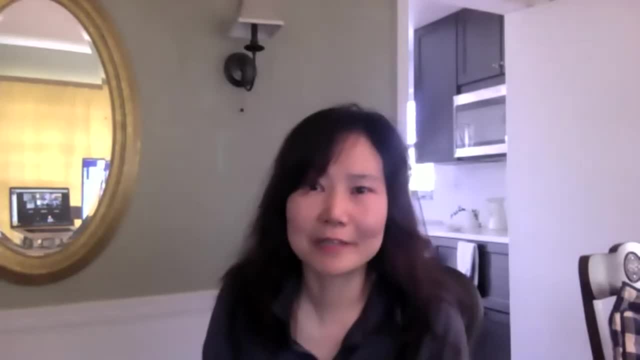 Just the mobility move around, but has different types of acts so that we can influence the rest of the population. So I need to go there gently, so maybe make a way, so using a conversational actions or showing a more legible behavior, so that people can understand. 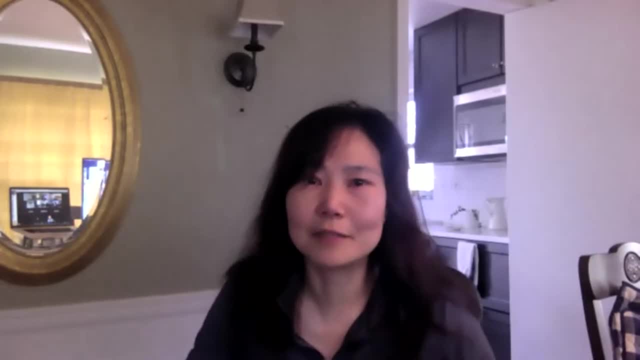 And so it's kind of implicit coordination. So that's that's the area that not many existing work have addressed. So there are other types of actions that we, the robot, can actually use, but all of these algorithms have been developed in this formulation. 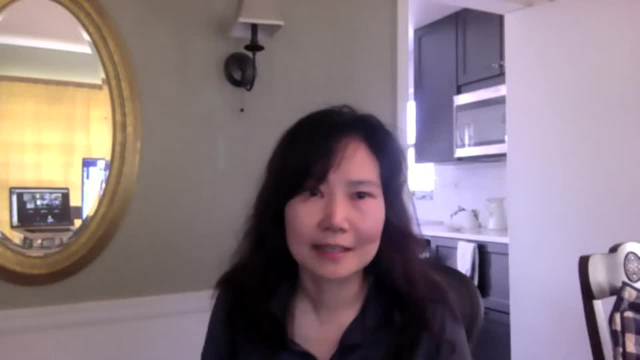 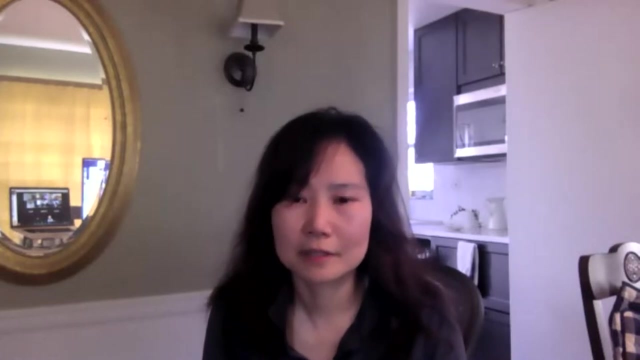 There are only moving actions, Right, And then we, we kind of only are thinking about the moving part, which is kind of a passive planning idea. So the environment, we will just choose moving actions based on what we have observed. But like, can we actually proactively change these agents because they can also move based 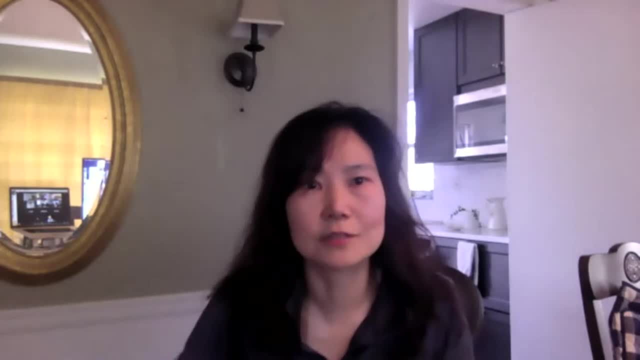 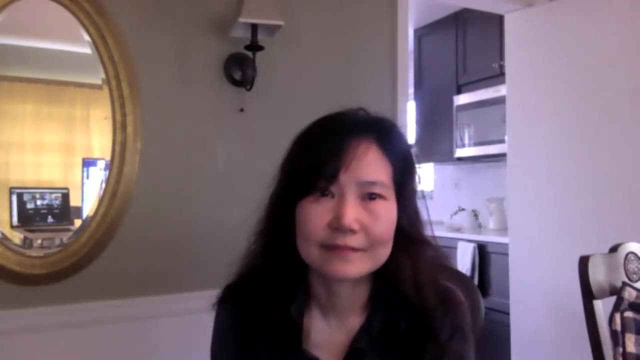 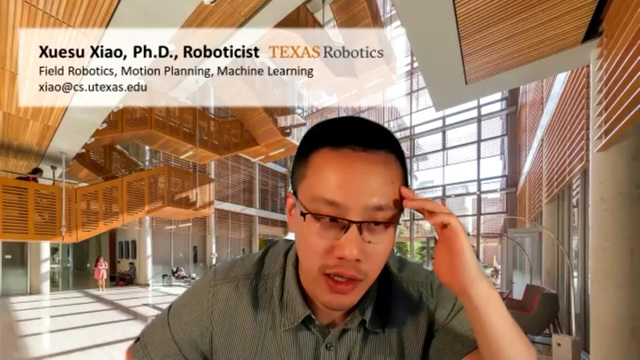 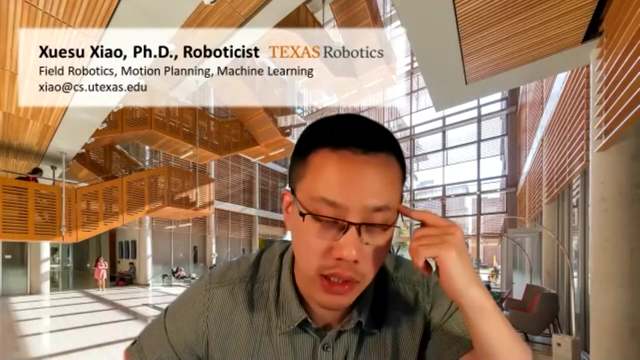 on my influence Or my suggestions or things like that. The other thing I want to mention, in addition to the planning or perception level, is the inclusion of implicit cues. We talked a little bit about this, like with Aaron, yesterday, So they have, like Justin has- a lot of work on this end as well. 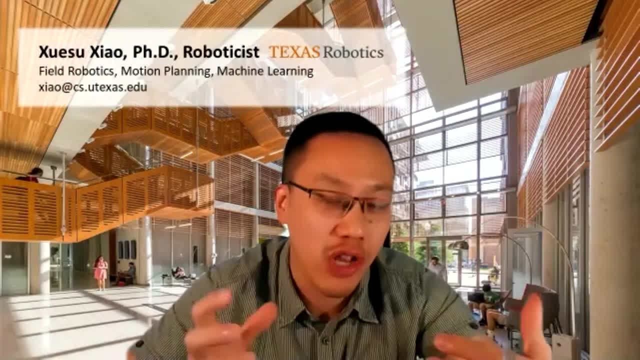 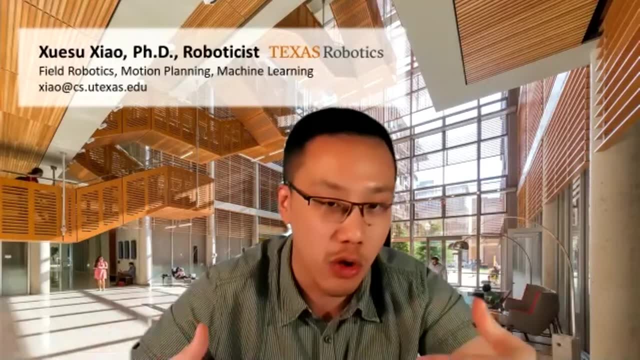 Right. So I just wanted to say that, like you know, when you interact with different social agents, it's not only about it's not only a metric or geometric sense, but it's also in terms of, like, your body, language, your gaze, your motion, your ability. 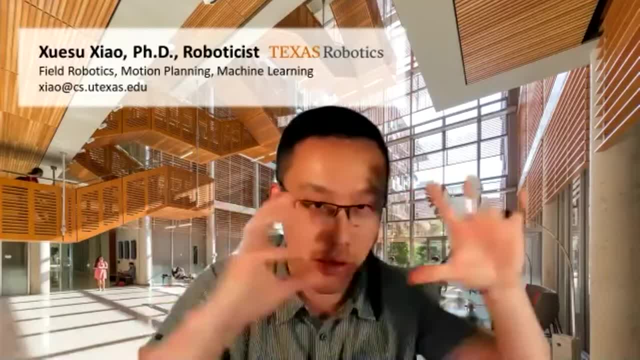 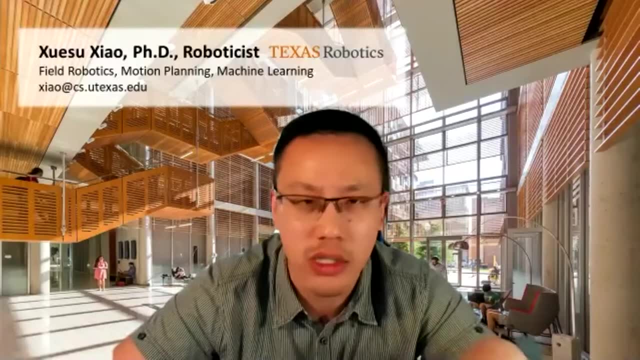 So Aaron has some work on mounting like a physical head and then doing the gaze and head rotation. So, Laura, when Laura was a PhD student with Aaron, she also did some research in this as well. Right, Also, I think I forgot her name. 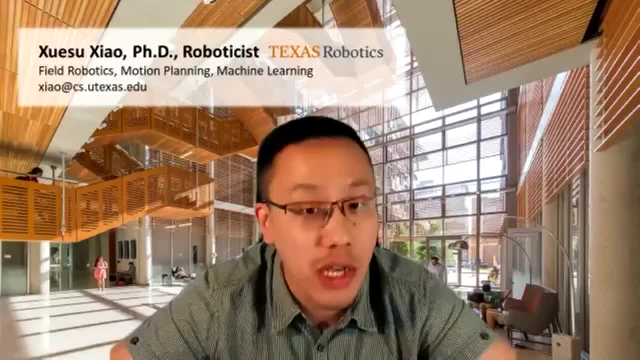 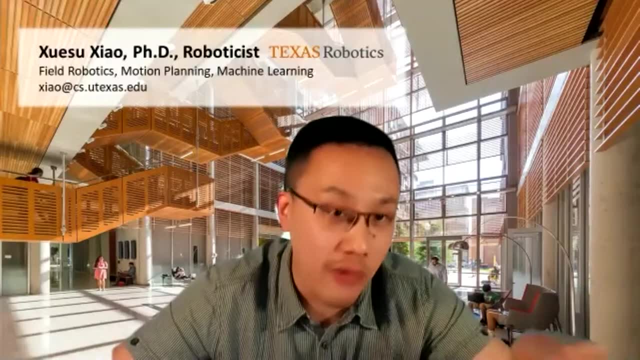 Aaron's: yeah, yeah, yeah, So she also has some work on this. Yeah, yeah, yeah, So yeah, I would say. eventually we probably also need to explore the other aspects of social navigation, adding those eligibility gaze, body language. 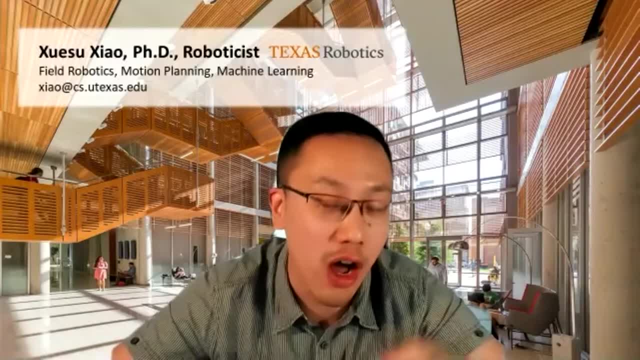 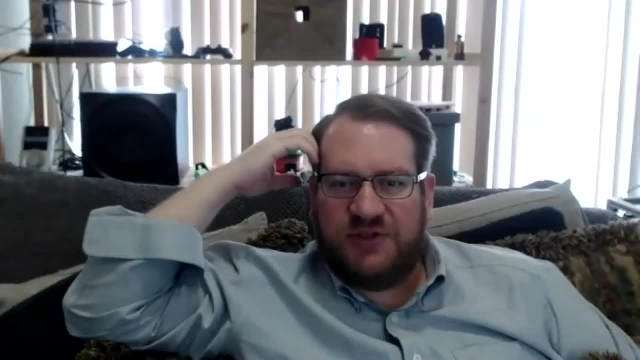 like these things, right? Yeah, Justin has lots of ongoing work on this. I mean, I've set up a set of sort of like parallel lab spaces over here at UT Austin. So I've got a lab in the computer science department where I've set up a virtual reality system. 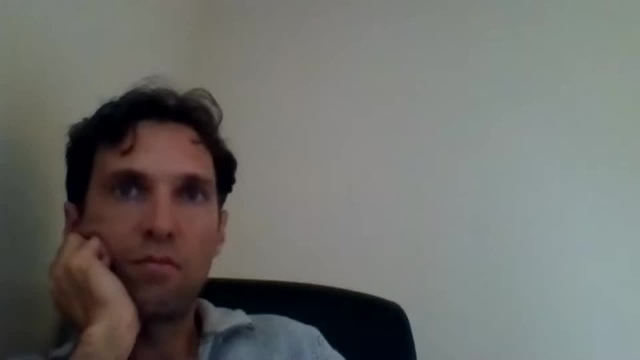 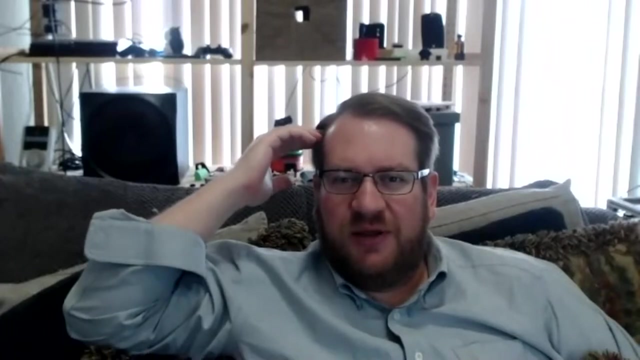 And the reason I've been using VR is because it's a little bit easier and faster to do experiments than, say, with, like a Vicon. But there are also very good VR systems that now have integrated eye trackers And so you can get integrated output. 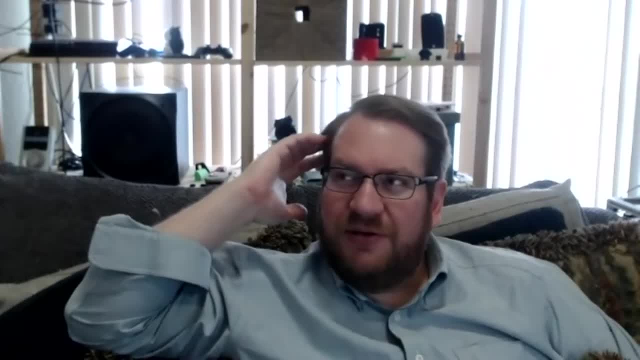 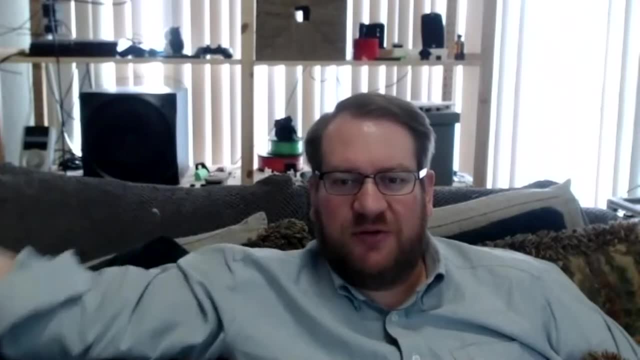 And then you can also get high fidelity tracks, maybe not at the temporal frequency of VR, of Vicon, but the spatial frequency and the angular frequency, yeah, And so our angular resolution, And so that's pretty good. And then you can also create: 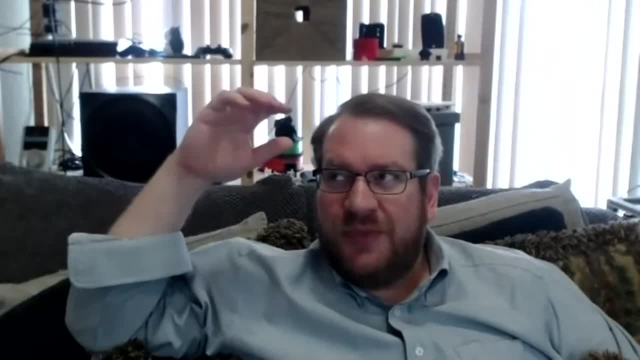 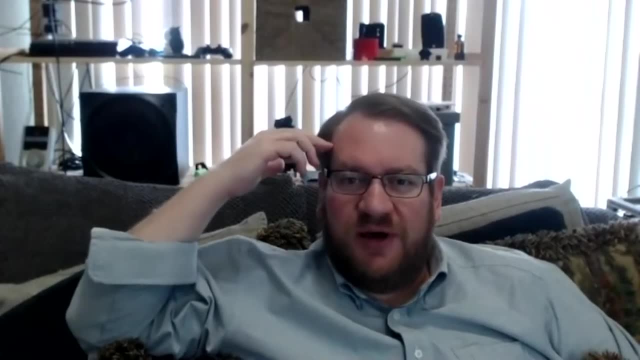 a good virtual environment for your study. So we've got a hallway that we've built in virtual reality with two people passing each other and looking at the exchange of gaze. We've got a paper that was accepted to ICRA by Bob and Halkar. 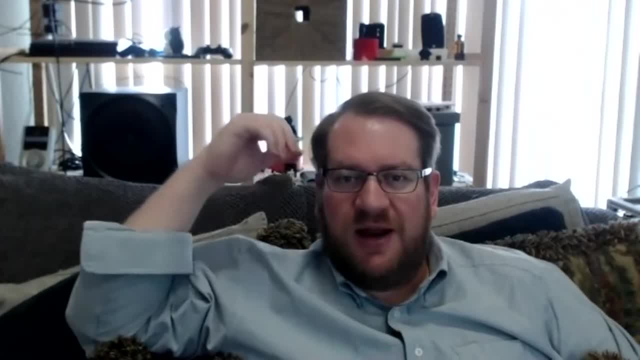 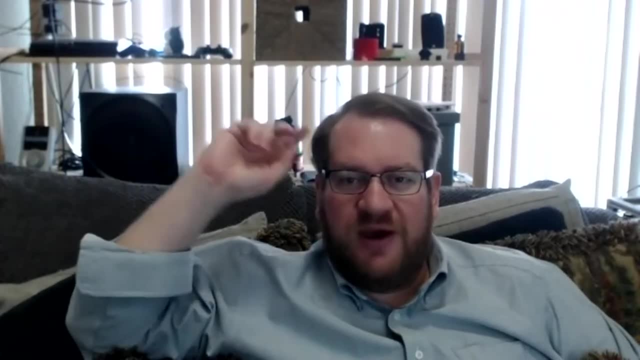 who has been at the symposium had a paper about like looking at your head angle and looking at that as a predictive cue for where you're gonna walk. We have one where it's gaze as a predictive cue where you're gonna walk. 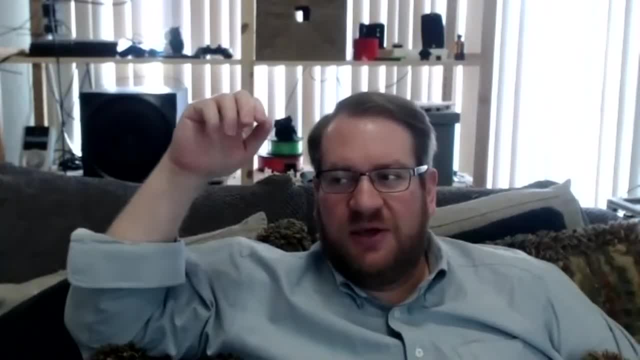 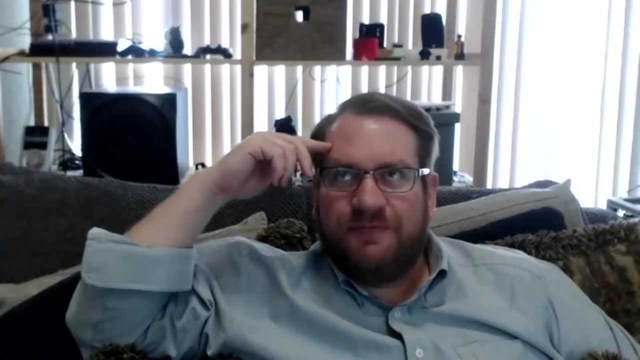 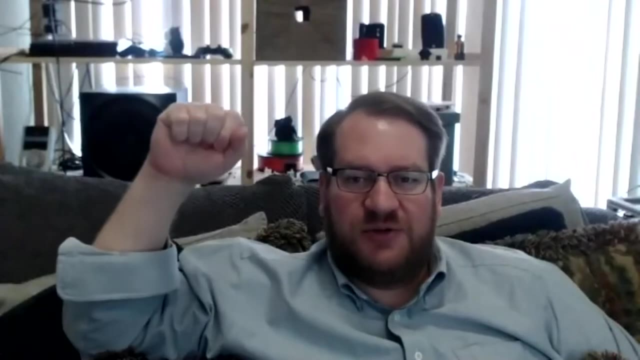 same sort of model, just with that, But now we're looking at embedding two people into that environment and then looking at the exchange of body language and also looking at things like torso twist and your shoulders, and are you forecasting what you're about to do and things like that. 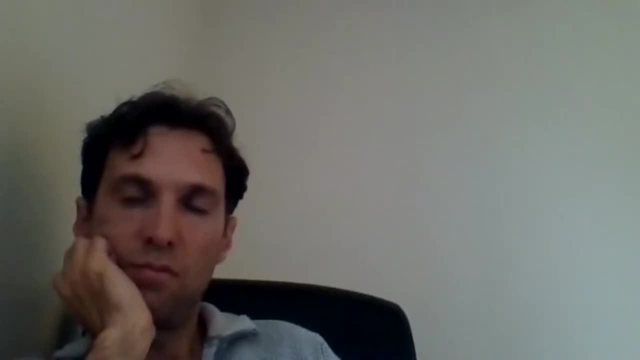 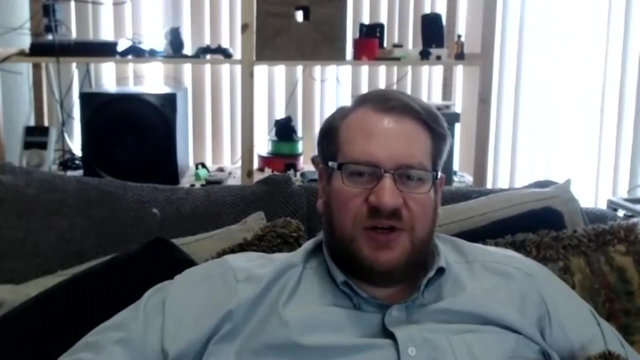 I think we're- I think we're probably gonna wrap up the forecasting type stuff where it's like, are you like twisting into a turn and that sort of thing this semester. And then we've got a similar setup where we built a hallway at a cubicle furniture. 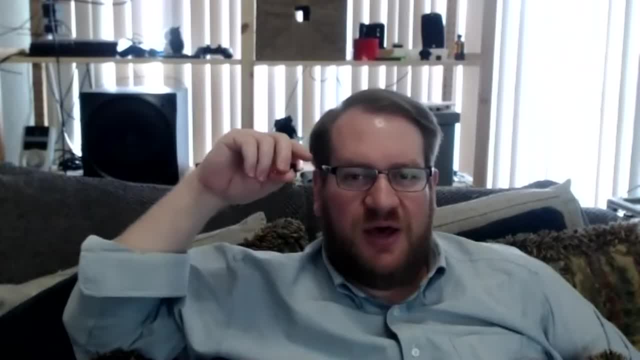 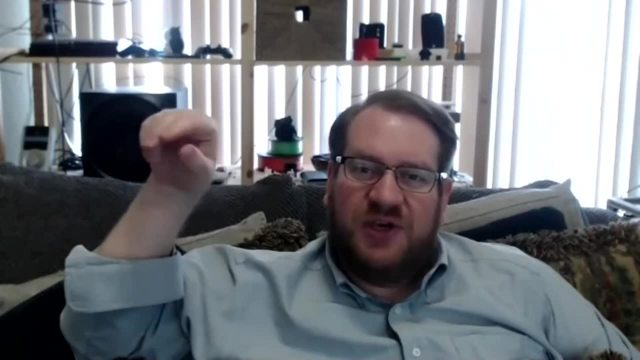 and we've published a couple of papers with like Zueschi was a coauthor on a paper where it's a robot with a virtual agent head and the head is producing a gaze cue. and do people read that cue? and it turns out yes. 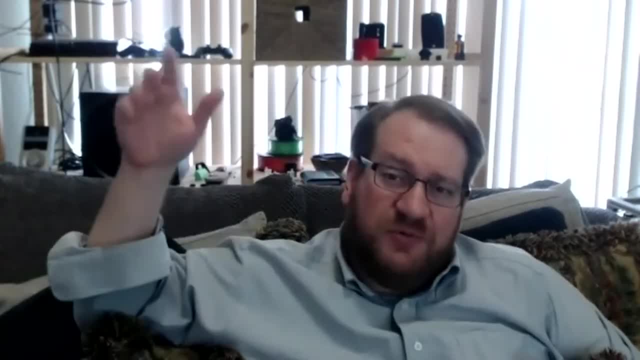 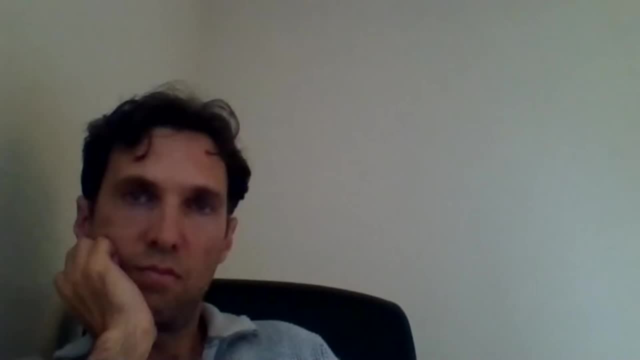 But the gaze cue isn't super realistic. So I've got a parallel group of people working on making better gaze cues And then but also looking at the same body language stuff and another instrument it set up with Azure connect cameras and having people actually walking. 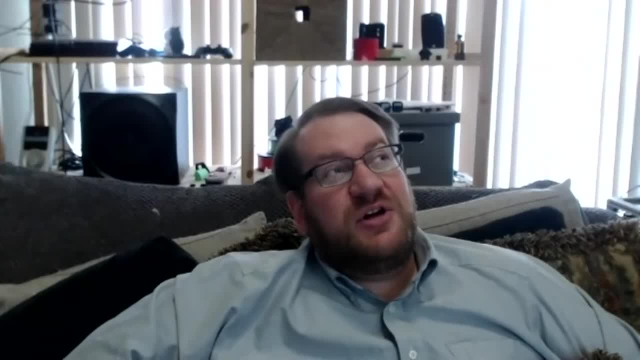 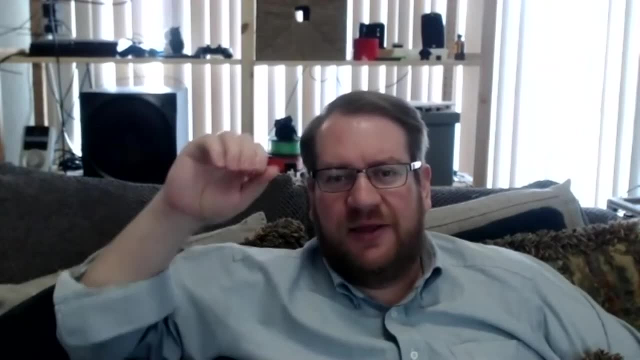 And then we've got another thing with it's, in conjunction with Peter and Joydi, looking at the same models, but on the robot, with a camera mounted on it. And then we've got another thing with it's, in conjunction with Peter and Joydi, looking at the same models, but on the robot, with a camera mounted on it. 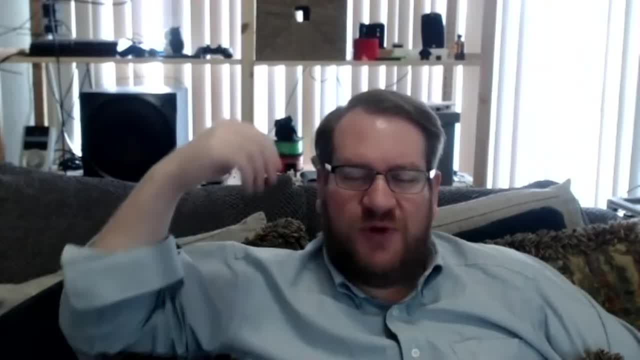 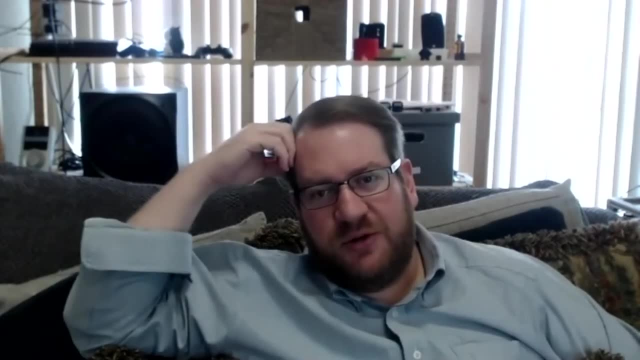 on the robot with the person tracker and reacting to the people and what they're doing and reading those cues, And so we're taking all the same data, putting them into neural networks to make predictions. Right now we've got statistical models that show that the predictions are. 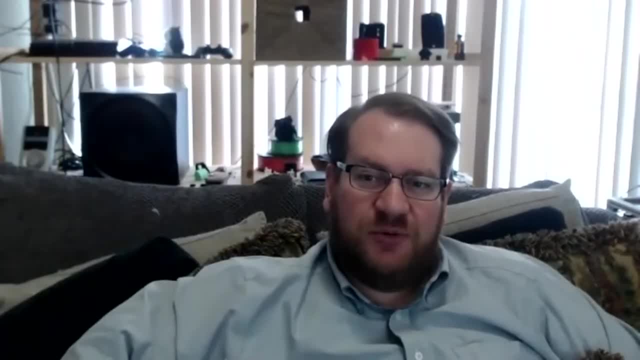 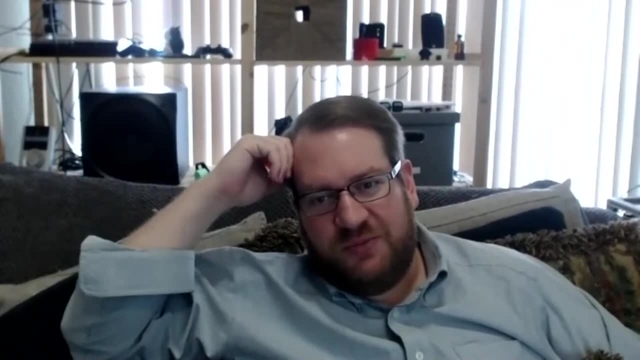 possible. but you know, building regression algorithms so we can put those into planning scenarios, So that's pretty exciting. So that's kind of like you know the matrix of what I'm putting together. as far as that's all concerned, You know we'll see how it all goes. So far so 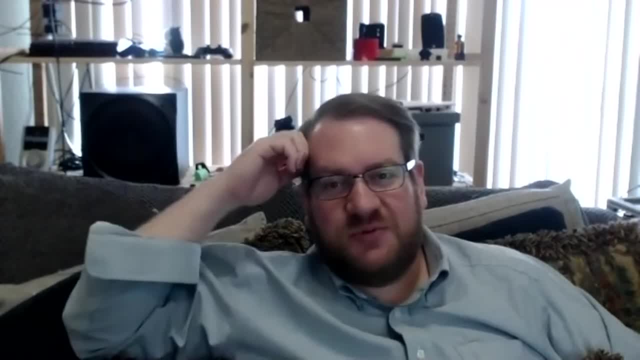 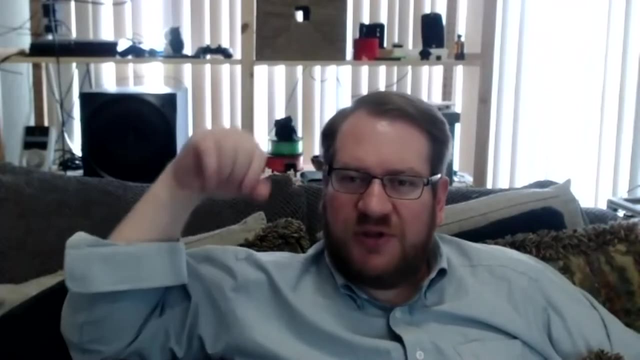 good, You know, yeah, But I do think that that's really important because, I mean, clearly, the exchange of implicit communication is, you know, plays a huge role here, And, you know, I think that it's like a lot of work has been done on the trajectory along the ground, more so than anything. 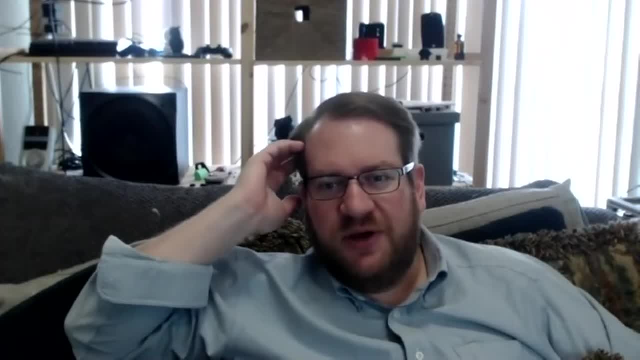 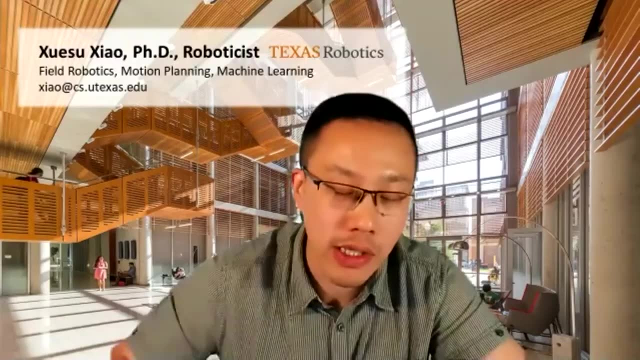 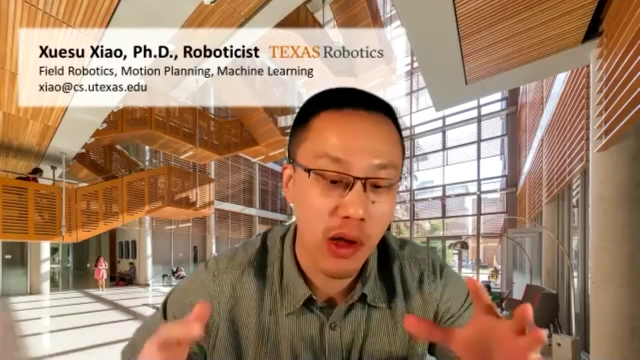 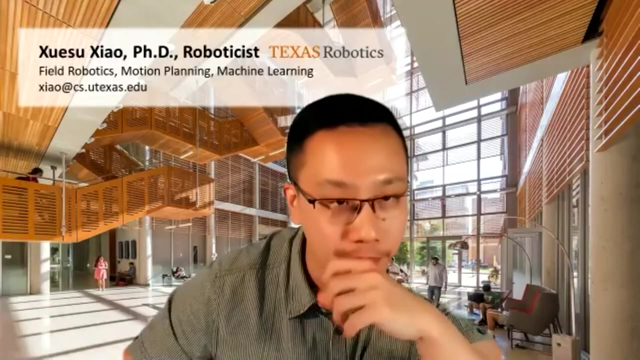 else. So I'm trying to- Yeah, definitely yeah, I will say that's definitely an orthogonal direction that need to be explored before we actually can have very organically, like robots, social robots, into human crowds to navigate things. Yeah, All right, I guess we are right on time. So 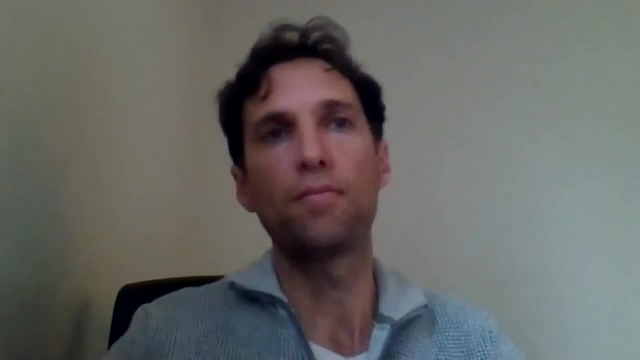 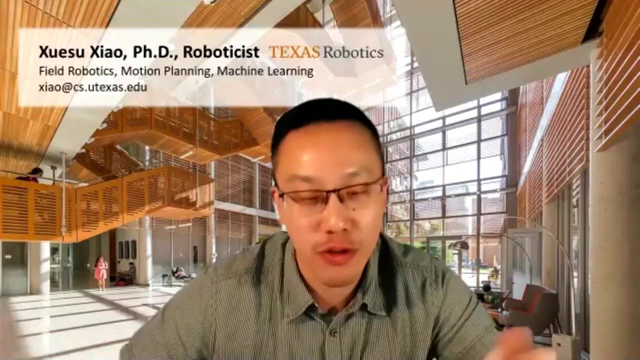 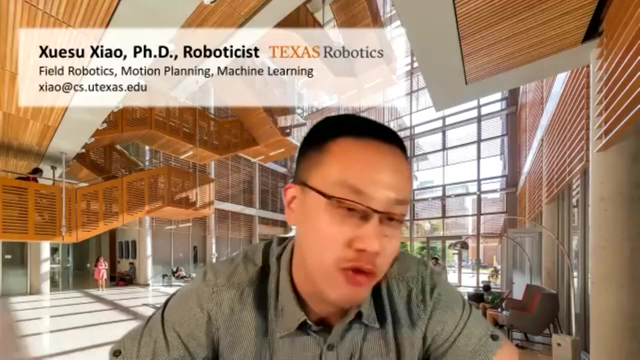 yeah, I don't have any like, Oh sorry. Okay, Thank you so much everybody for sticking around to the end and I think it's a successful symposium. I hope it's. I wish it's like a physical symposium, so we can actually see each other and we can ask the industrial partners to bring in their robots for us to demonstrate their capabilities.